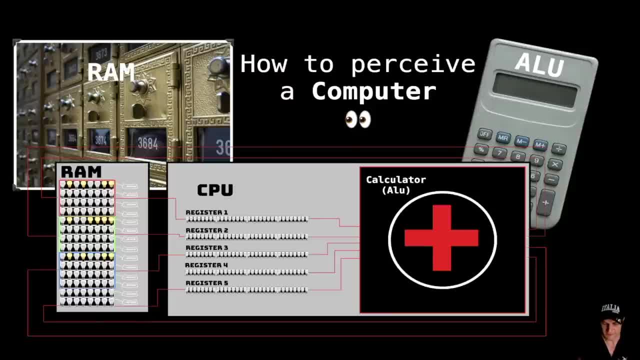 right: Abstraction is the key to collapse difficult, complex entities into manageable ideas. right: We want to collapse complexity into intelligible models. That's what we're going to do now I'm going to try to explain to you what is a computer in a nutshell. So 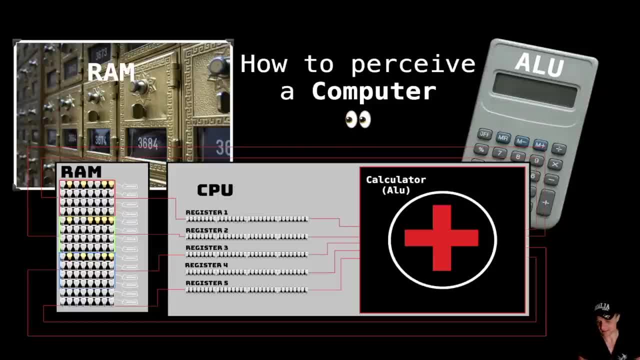 let's pretend an alien is coming to the planet and is asking to yourself: hey, how does your body work? What is going on there? Well, it's kind of a tricky question, right, Because there is a lot that is going on. You can start to explain to the alien. well, you know, we. 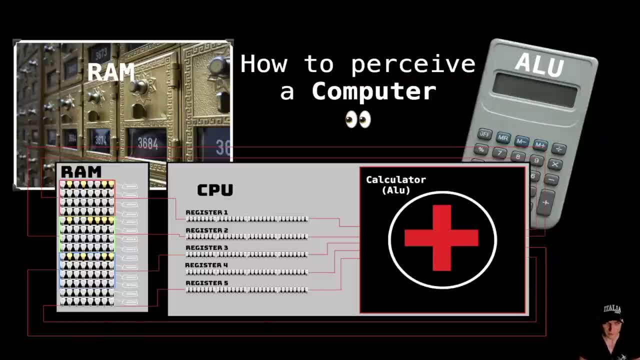 are made up of atoms, especially we are made up of carbon. We can consider ourselves like carbon machines: some hydrogen, some oxygen, some nitrogen and yeah, kind of complex, right, If you want to describe yourself in a Rick and Morty fashion, like saying every. 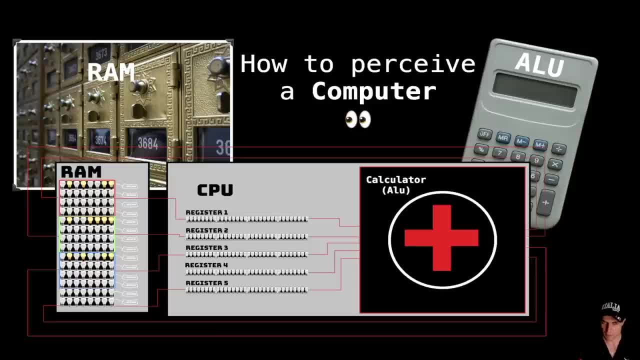 atom what is doing? well, I guess you're lost. A better approach, I would argue, is to tell the alien. well, you know, I have some systems inside myself that are providing some functionality. For example, I have the. 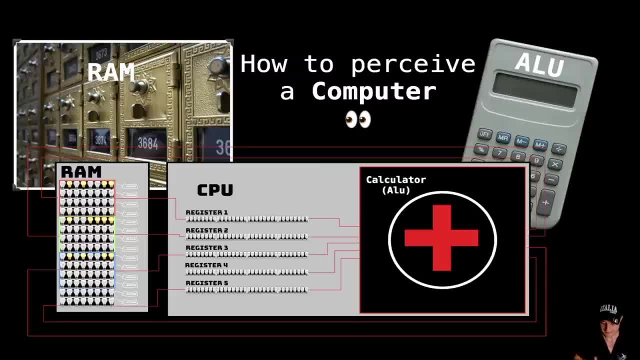 nervous system, which is composed of some organs. These organs cooperate together to process my reality, right? Something like that? In the same vibe you can say: well, I have a digestive system that is processing food that I take from nature, and this food is converted. 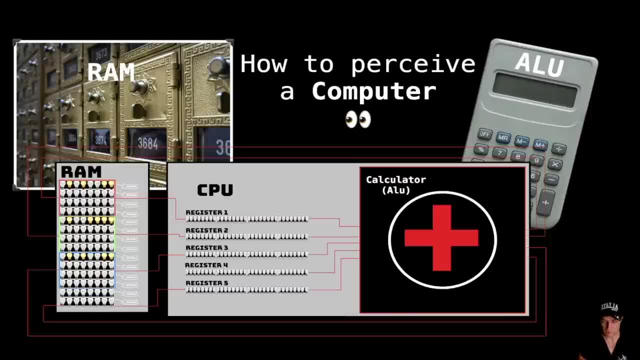 to energy, Energy that I can use for my nervous system to process reality, but I don't know as well for my muscles. Move around this body. You got the point right. You explain reality at a specific level. You don't want to explain from an atom level. right, It's too low. You cannot explain as 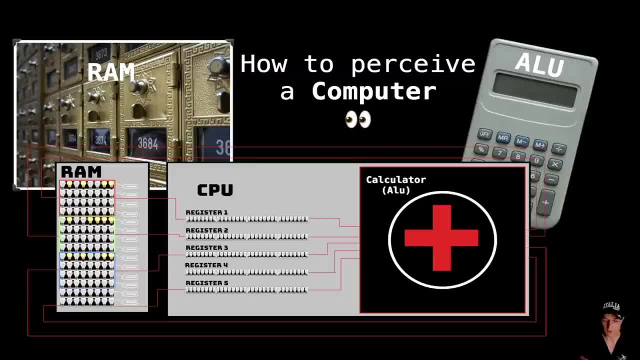 well from a cellular standpoint, right. Still too low. You talk on a level of systems, right? You simply say: I have this system that is providing this function, This other system that is providing this function. all together, these systems provide me. That's what is going. 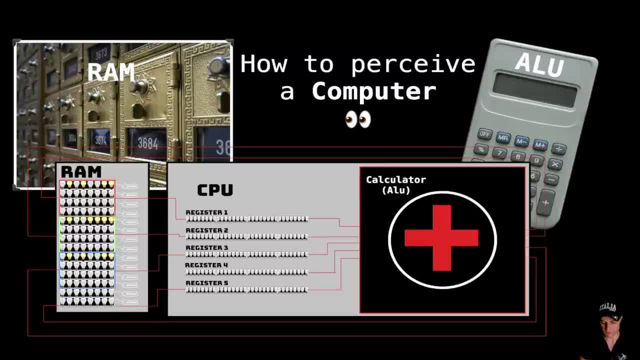 on In the same vibe. I want to explain to you what is a computer. At the end of the day, a computer is just a super fancy calculator, if you want. Especially when I code, when I write my C programs, I perceive the computer as just a simple arithmetical, logical calculator. 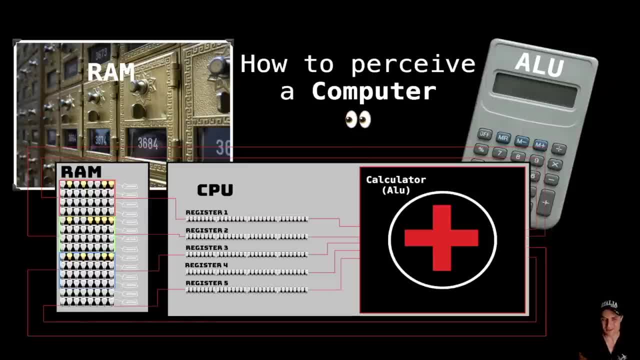 and a place in which I can stock all my numbers. So I see the RAM, the memory of the computer, as a big chunk of boxes with a specific ID. you will see in this video this is the gist of it- Addresses indeed Pointers. 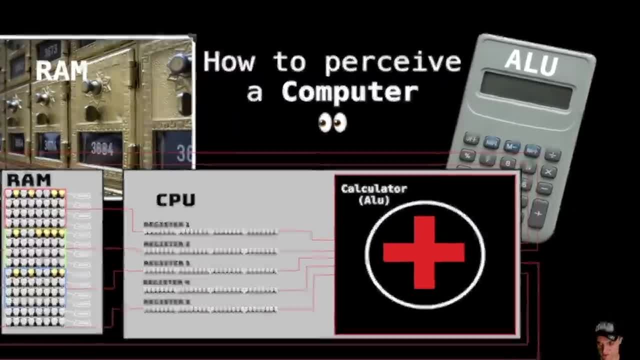 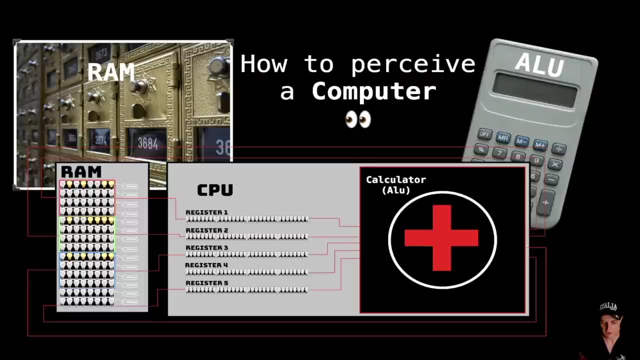 On the other hand, I see a calculator, A calculator which is an arithmetical, logical calculator that is able to perform, indeed, arithmetical and logical operations. Logical operations entails something like: is this number equal to this one? Is this number less than this? 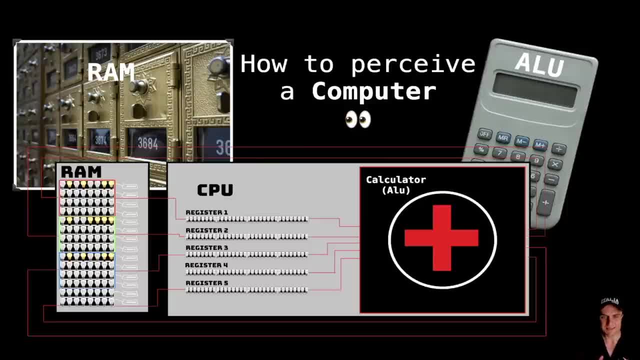 one And so forth, Very simple stuff. So that's basically it. That's how I perceive my computer: An arithmetical, logical calculator And a place in which I can stock numbers that will be processed by this arithmetical. 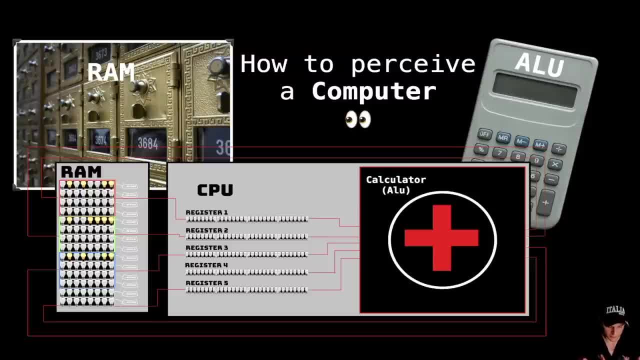 logical calculator. okay, Of course, in the real hardware I'm talking about the CPU, which is the central processing unit. You can see in the image that the CPU has inside the ALU, which is the arithmetical logical calculator. I was talking to you about arithmetical logical unit Inside the CPU. 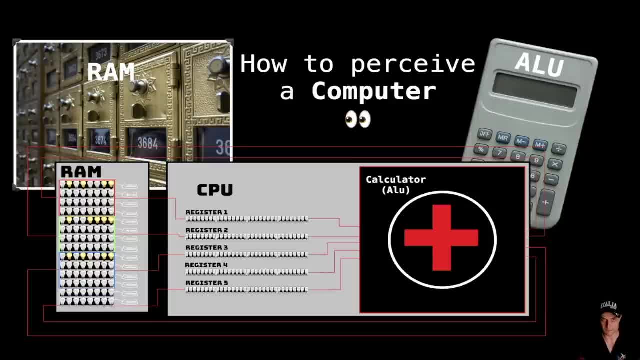 we have also the registers, which are intermediate places in which we perform the operations. We have a lot of places in which we stock numbers, And then we have the giant RAM, Giant, quote-unquote giant, because it can be 4GB, 8GB, 16GB and so forth. 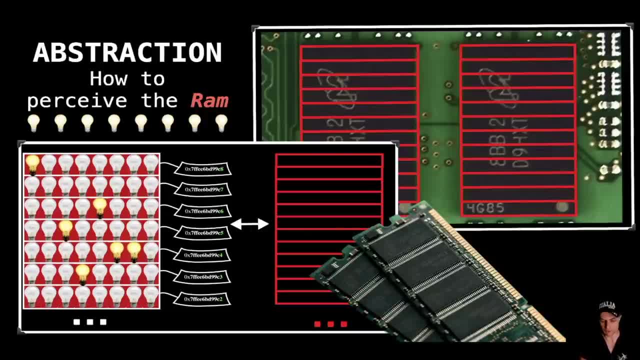 Okay, so let's dive into the RAM a little bit more. I told you that I perceive the RAM as a series of post boxes, essentially with a specific address. Every post box is a byte- okay, You know this stuff very well- And every byte is just a line of 8 light bulbs, As you. 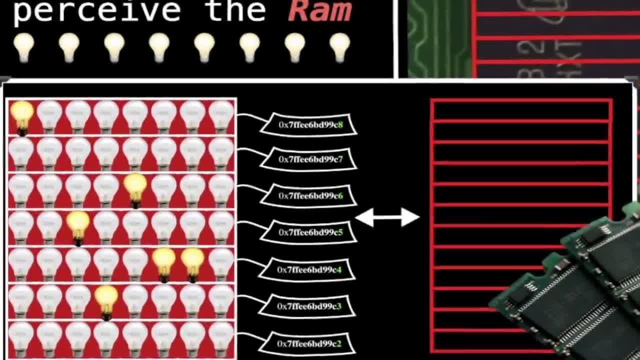 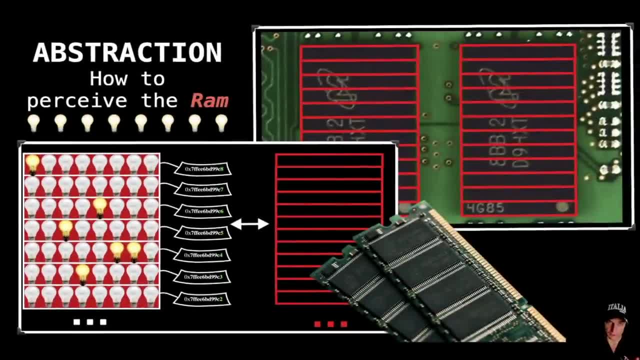 can see, every byte has a specific tag which is the address of the byte. so i have the physical view of the ram, which is a chip, and the logical view of the ram, which is my programmer perceived view of what this chip is offering me. right, a series of bytes, as easy as that. okay, so we have. 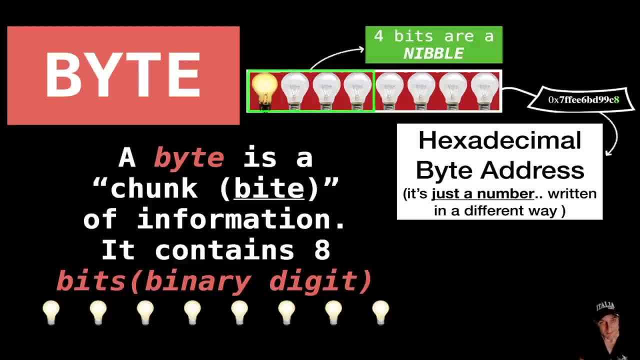 this view of what is the memory? so, inside this memory, i told you that there are these boxes. i told you that these are bytes, and what is a byte? a byte is eight light bulbs. of course, this is an abstraction for a transistor, but we can perceive like a light bulb that can be turned on and off. 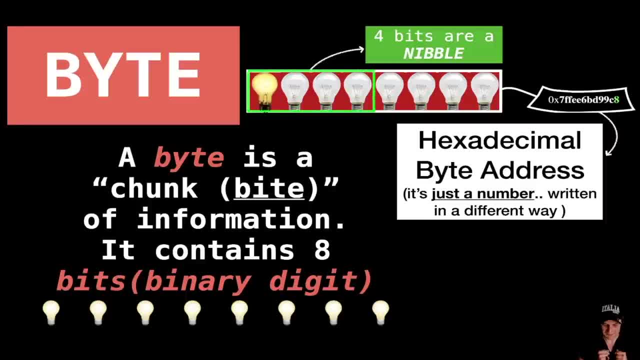 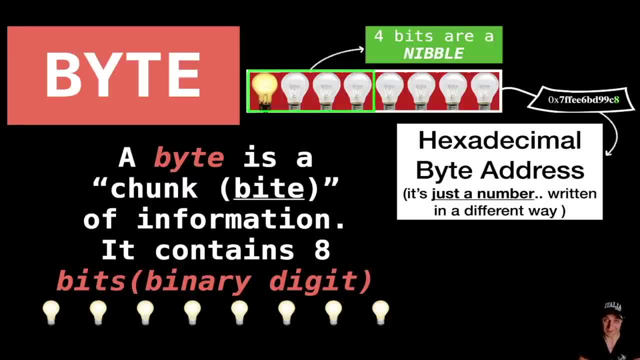 to zero to zero to two hundred and fifty five, of course in a binary way, in a binary base, because we are dealing with a binary machine, of course these light bulbs can be turned on and off in a binary fashion. the name byte is just a kind of joke, because four bits are enabled, so everywhere. 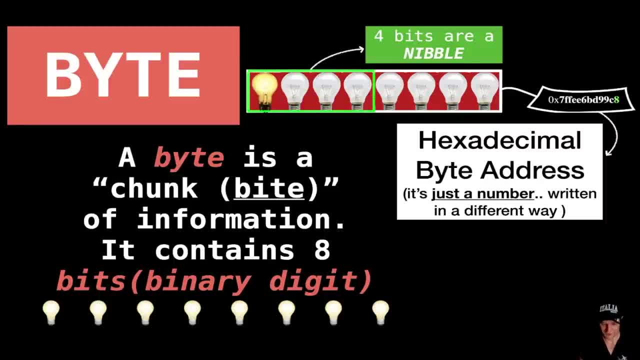 in computer science there is plenty of these kinds of joke. you will find out and as you can see, uh, here i have the, the address of um, the byte, which is a number. you see this strange number with symbols, but this is an hexadecimal notation. this is an hexadecimal. 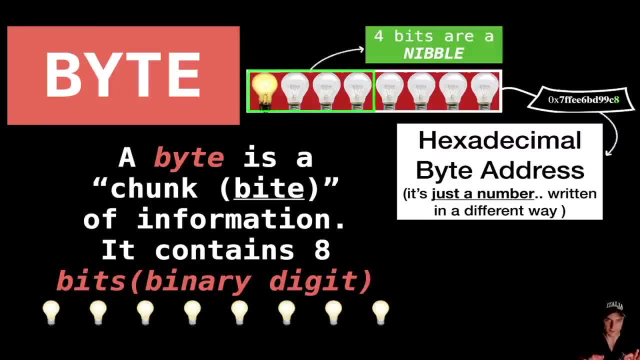 number. but keep in mind that this is just another way of representing a value. i can write the number 42 in hexadecimal, in binary, in octal. this is just a different way of representing the same thing. you can make a parallel, for example, if you say i privet ciao, all these things mean the same thing. 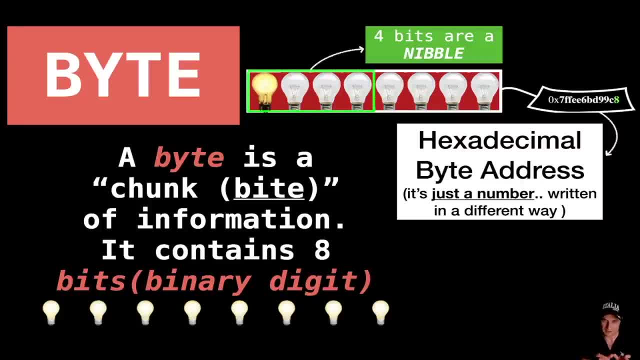 they mean i, but they are in different languages. so the value is the same, only the symbols are changing. so it's just a number. that tag is just a number, which is the address, the location in memory of this byte. so inside these bytes i can put stuff right, i can put. 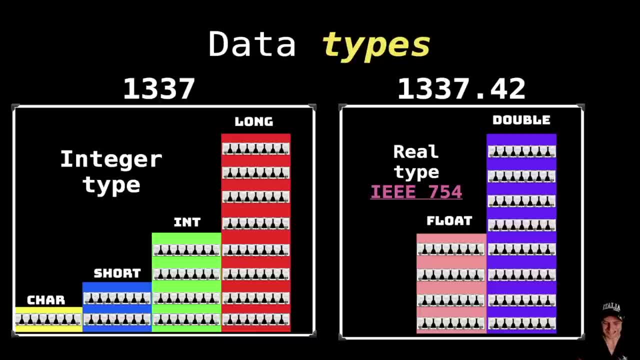 numbers. to be more technical, i can put data types. you can see i have these data types. i have char, short, int, long, float, double. to be more pedantic, uh, short and long are just qualifiers. they are short int and long int, but we can consider them like data types. 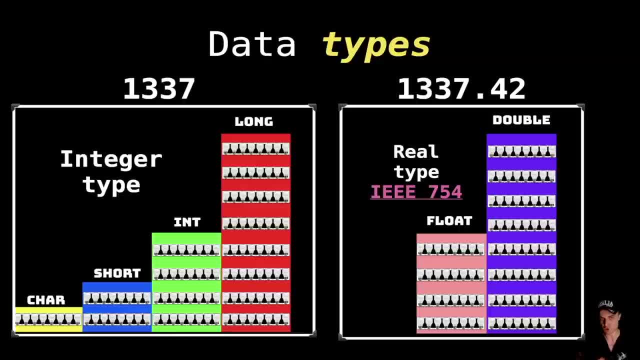 per se, right. when i declare a variable, i just use short and long. i i'm never right short int on long int, but this is an aside, this is not important. okay, from this slide you have to understand a few key ideas. so the data type is of a specific size, as you can clearly see from the image, you have a 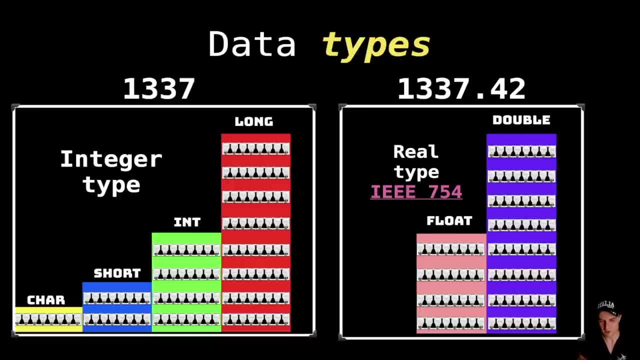 chart which is one byte, and you have a long which is eight bytes, generally speaking, depending on the machine. for example, in my macos, i have a long which is eight bytes, generally speaking. this is true even for you, i guess. so the data type is going to disappear and the data type is going to disappear. 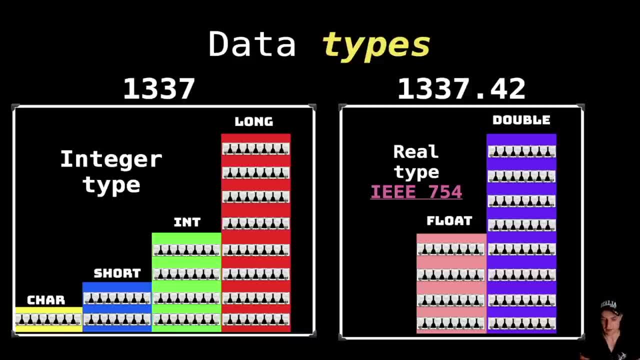 and the size that we're going to ask to our compiler in the ram. and, of course, the data type is going to discipline the way in which bits are going to be arranged. so we have two families, basically, we have the integer type and the real type. the way we stock data is qualitatively. 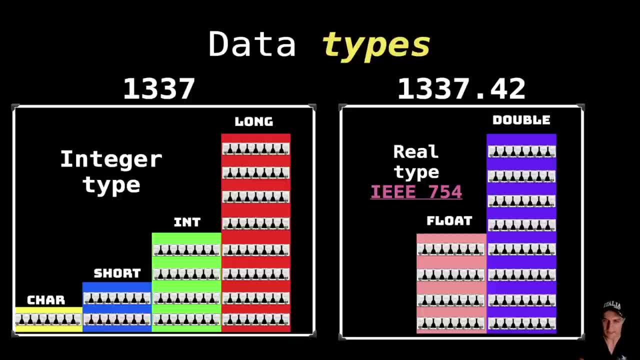 different. indeed, when we stock float, we have a different pattern configuration. when we stock real numbers, we have one bit for the sign, which is equal for both, and then we have some bits related to the exponent. so we have a qualitatively different configuration for the data type. 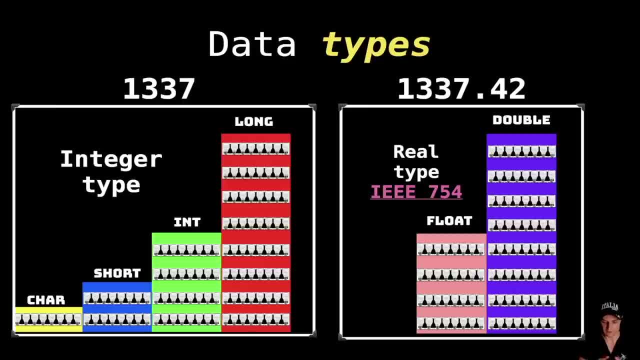 different way of stocking these numbers in memory. you will see later. we are going to dig a little bit about this idea. so key idea: integer types and real types have a different way of encoding in memory, binary speaking. so the bits are going to be arranged differently. you will see with a clear example later and depending on the specific data type you're. 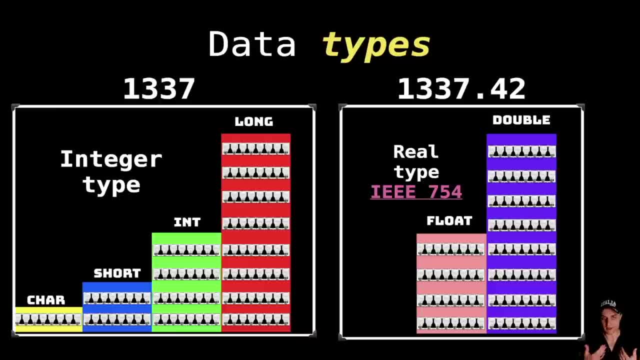 going to take much or less memory. okay, if i ask for a long, i'm asking for a big chunk of memory: eight bytes. if i ask for a chart, i just need one byte. indeed, in a chart. typically we stock charts but at the end of the day, a chart is just one byte, integer. it is an integer indeed. 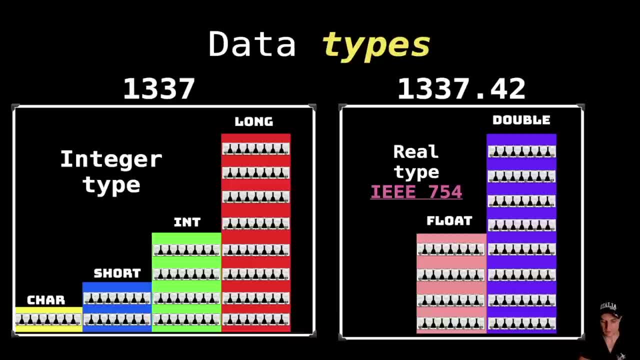 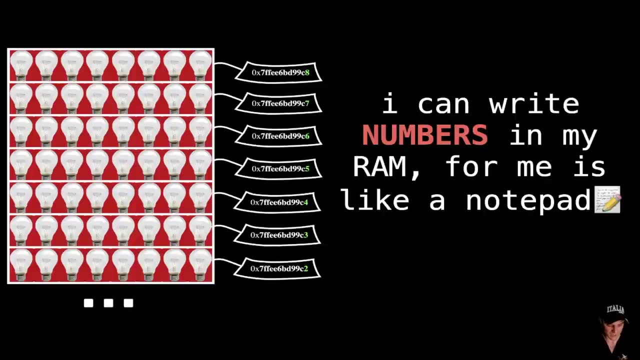 okay, so we have a ram. we can stock data inside this ram that can be in the real and integer form, depending on how big these numbers are gonna be. i'm gonna take less or more bytes. so, as you can see, i can write numbers inside my ram. to me, it's just a piece of paper in which i can write numbers. 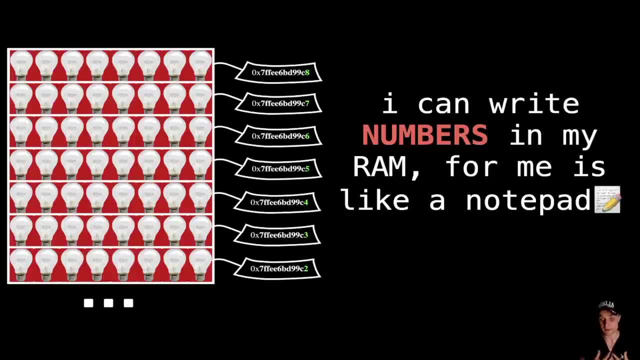 numbers that i will process with my algorithm. okay, that's all there is. i see the ram like a piece of paper in which i can write stuff. of course this stuff is going to be a number. of course this number is going to be in a binary form, because we have light bulbs that we can 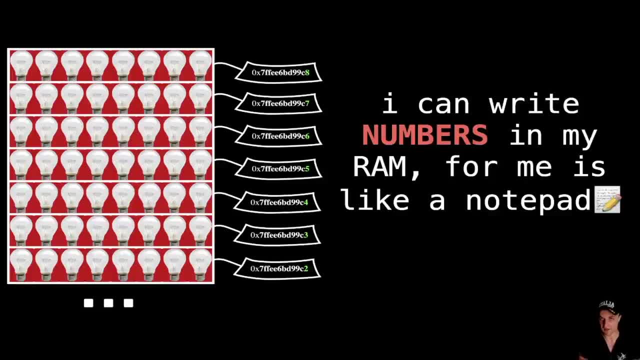 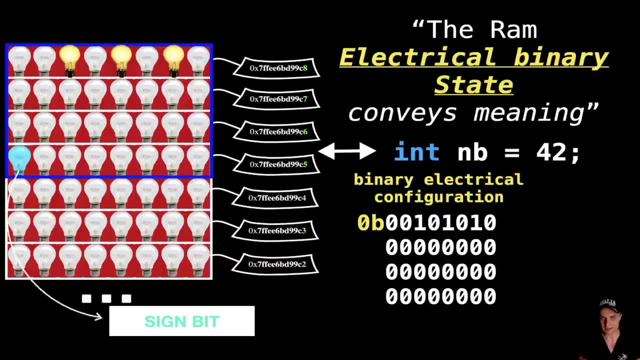 manipulate, but at the end of the day, with these numbers i can create everything. i can create this video that you're now watching. so let's make a clear example. the ram electrical binary state is giving some meaning, is conveying some meaning. in this case, i have declared the. 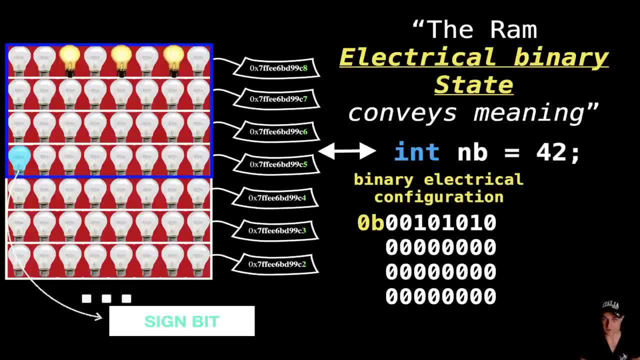 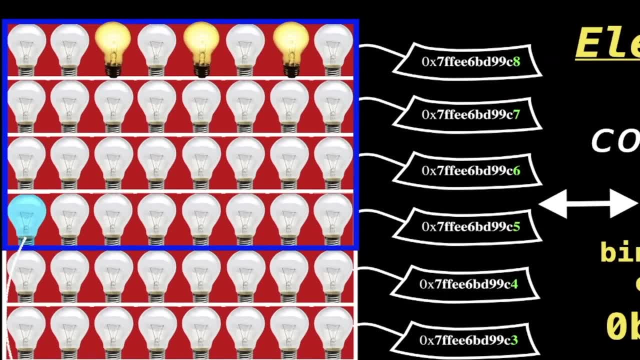 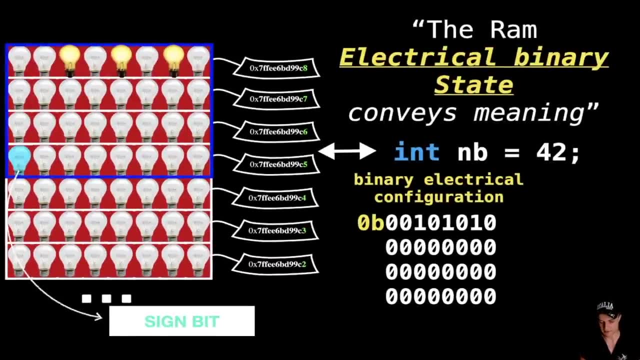 value of the number 42 to this variable, which is nb, and i assign the value 42 to this variable. as you can see, the bits are tuned accordingly. right here i have a one zero, one zero one zero. this is indeed the binary configuration of the number 42. i hope you know how to translate. 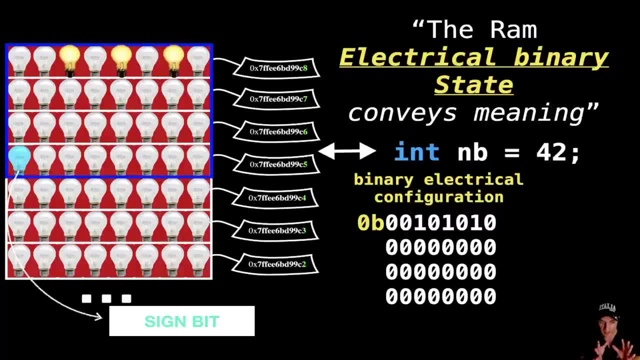 from binary to decimal. if you do not just watch a video, it's very simple. so here i've written in a space in memory, which is a that specific address, the value 42.. the specific configuration, the specific details by which numbers are stocked, is called endianness. if you want to search, 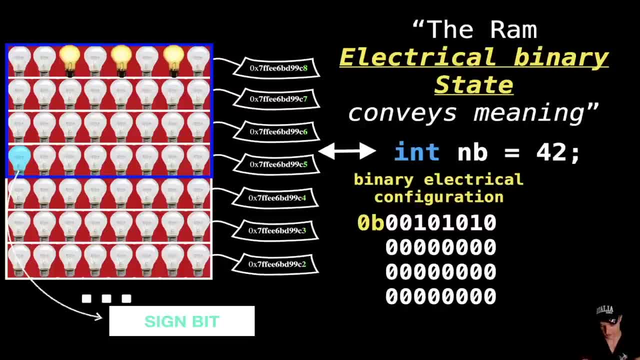 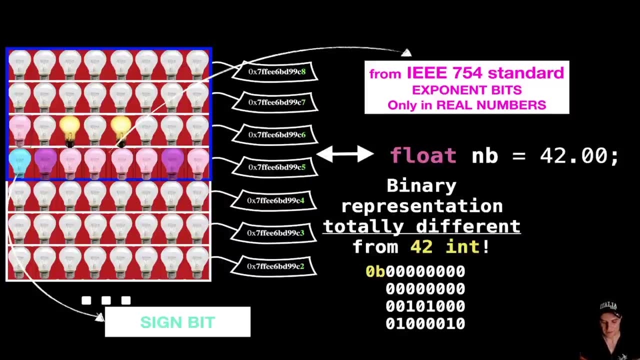 difference between little endian and big endian, but again, this is not related to our topic. let's focus only on the number itself here. as you can see, we have a binary configuration that is conveying the number 42. cool, now let's watch the binary configuration of the number 42.0. as you can see. 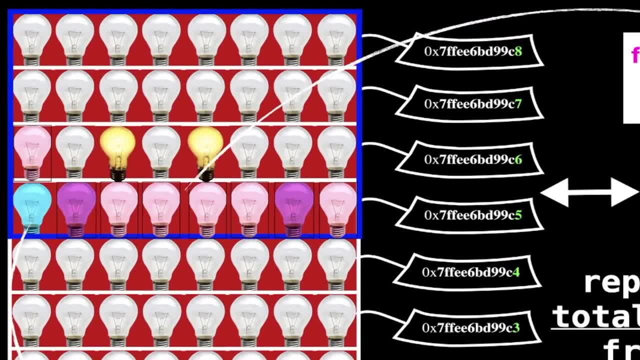 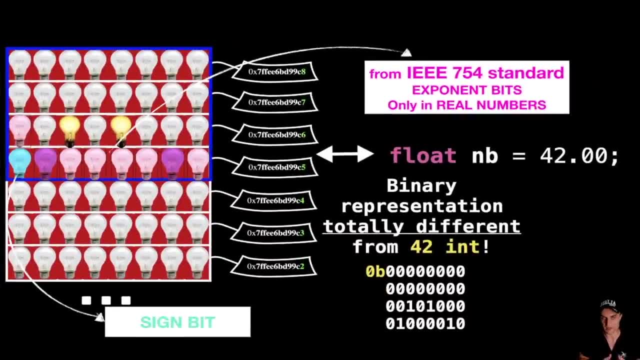 it's totally different. it's totally different because, as i told you, we have a standard that we're following. basically, engineers gathered and decided that, okay, this is the best way to stock a float number for various reasons, and we have these eight bytes that are the exponent for floats. now, 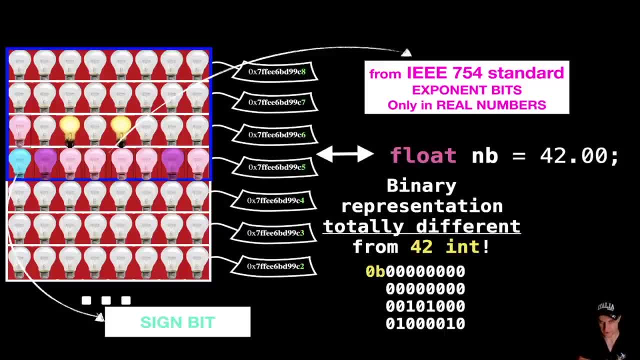 the idea that i want to convey to you is that the bits are totally different. keep in mind this idea, because it's going to be useful in the video, where we're gonna just do some pointer manipulation. so to make a tldr of this introductory part. by now we haven't talked about pointers at all. 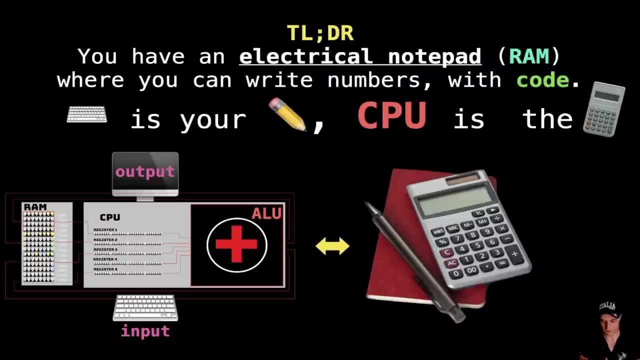 but we're going to do some pointer manipulation so to make a tldr of this introductory part by now. but i think it's useful to have this introduction to be everyone on the same page. so we have an electrical notepad, the place in which we stock numbers. the keyboard is my pencil. 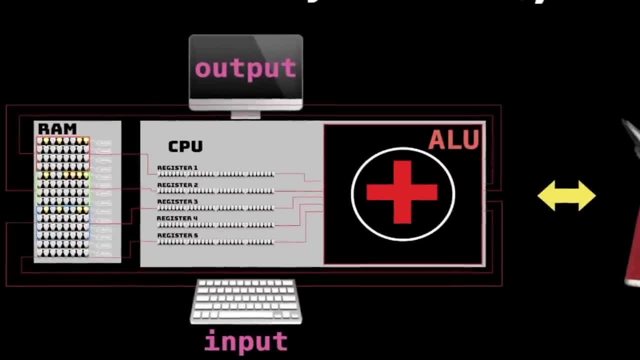 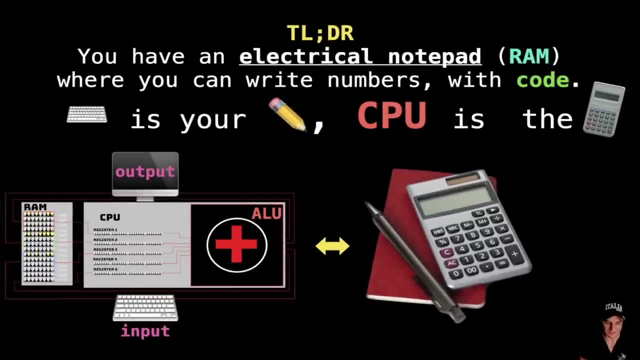 right is my electrical pencil. i input inside my ram the numbers, thanks to the code i'm going to write, and the cpu is my arithmetical logical calculator. every time i say if a equal b, or if i say printf a per b, well, all these operations are going to happen inside the central processing unit. 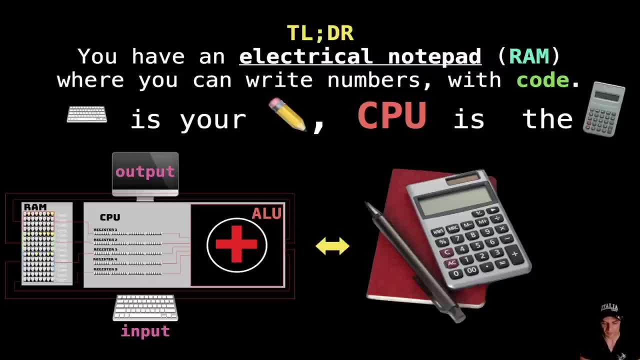 which is just a place in which processing is happening. so keep in mind this view: you have a place in which you can give the input to the computer, a place in which you stock number, a place in which you process number and a place in which you see the results- a super fancy calculator, my. 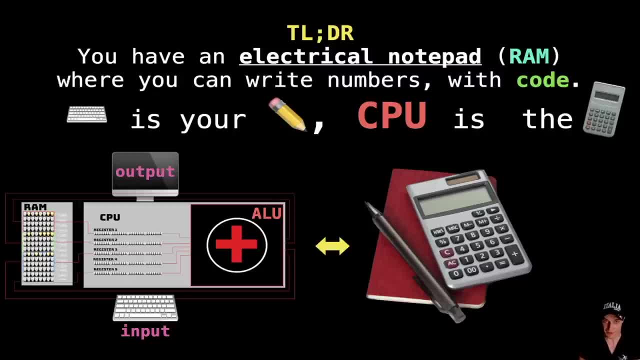 friend, you see, you can do this stuff analogically right with a calculator and a piece of paper, or you can do with computers that are much, much better, much, much faster. and you, you can do, of course, algorithm with computers, so to make a computer that is much, much faster. and you can do. 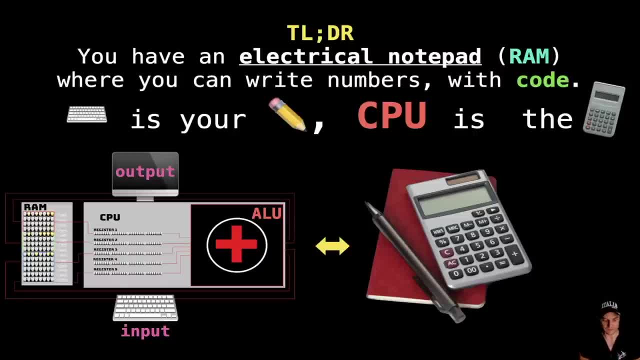 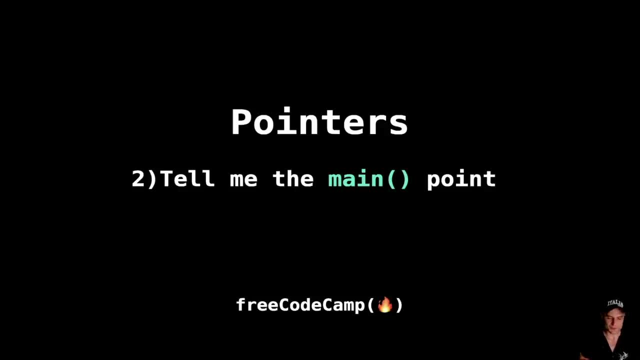 calculations automatic. so this is the intro, this is the view um which i think it's fairly useful to understand pointers, and we are ready to go okay. okay, this is all cool, my computer is a fancy calculator and a piece of paper, but go to the point, cut to the chase, and indeed i will. now we 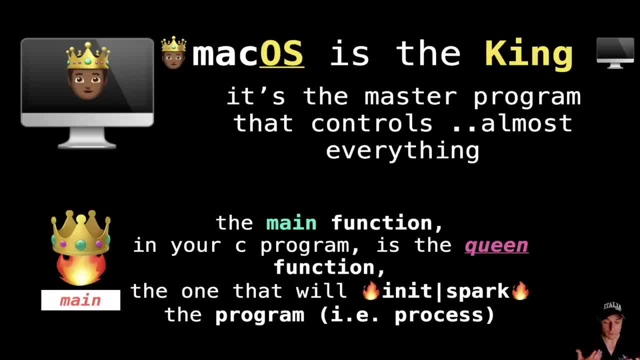 are going to talk about the main point, namely the main function. you surely know that the operating system is the master program that is taking control of all the resources inside your computer. right, it's the king is the medium between me and the bourbon hardware. this is a super complicated program. 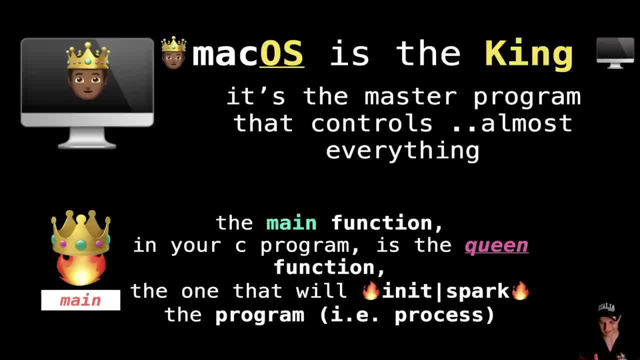 that is able really to control the machine at the lowest level of reality. every time i create a program i'm asking the operating system to give me some computer resources. inside my programs i have a special function, which is the main function. i call it the queen function because it's gonna be the first one that is gonna spark, that is gonna. 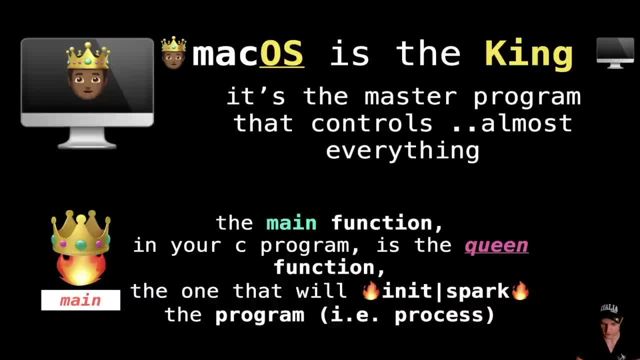 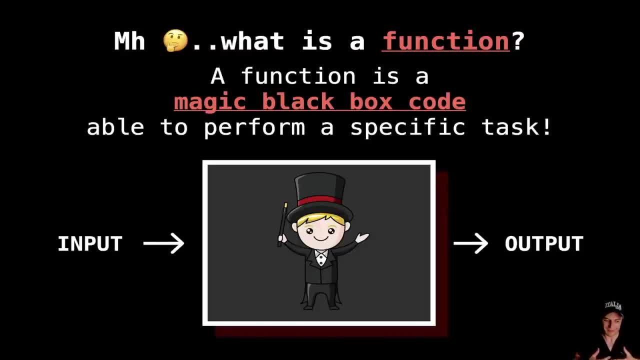 init all the process. a process is a fancy word for referring to a program that is running. so first of all, let's clarify what is a function. well, at the end of the day, a function is a black box magic is a piece of code that is able to perform a specific task. the best example i can think of: 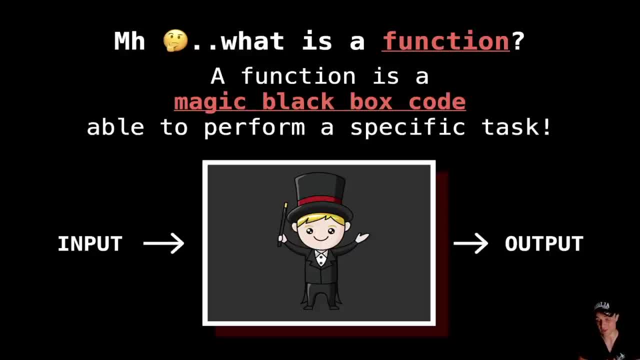 is the printf. how many times you have used the printf function without knowing absolutely anything? you have a piece of code that has been written by someone else you can use, including the output, and boom, you have in the terminal the string hello world. you don't know a line of the. 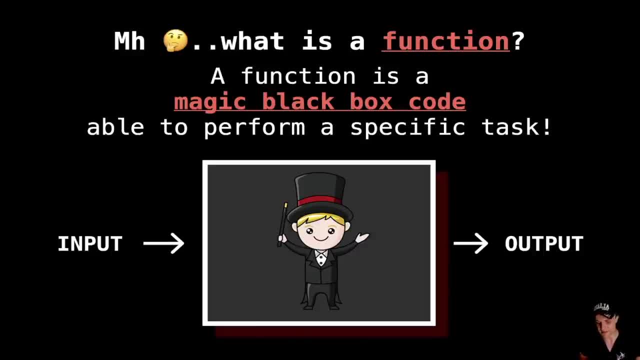 implementation of printf. nonetheless, you use on a daily basis. that's the power of abstraction, that's the power of functions. so to me it's a black box. i have an api that has been given, in which is written which are the specific inputs that i have to put inside parentheses and the specific syntax. 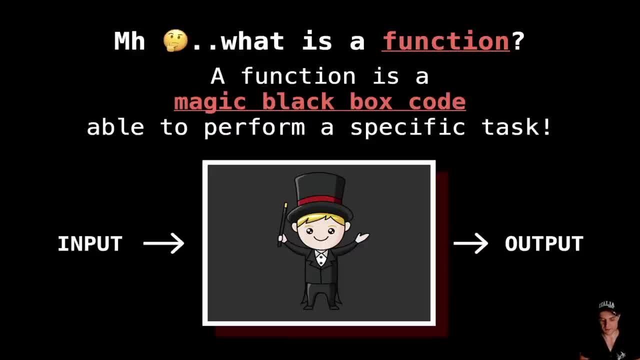 and given that i can use the function very easily, of course i'm talking about black boxes referring to others people code. if you have to implement your own functions, of course you know what is going on underneath the wood, right? the thing is that with code, we generally leverage other people code already written, so 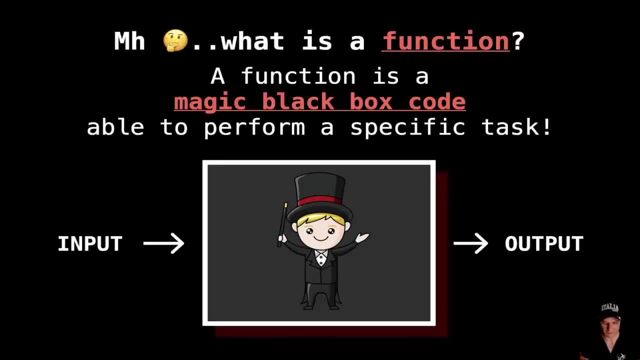 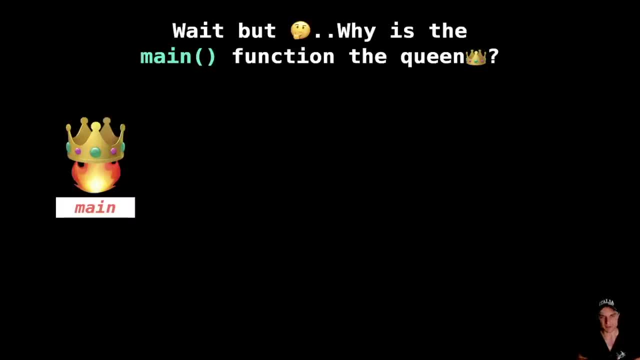 for us, the black box magic is a really good metaphor. so now let's clarify why the main function is the queen. well, every program can be composed of many, many functions, for example- i don't know- facebook. facebook is composed of many, many functions. for example, low world is composed of 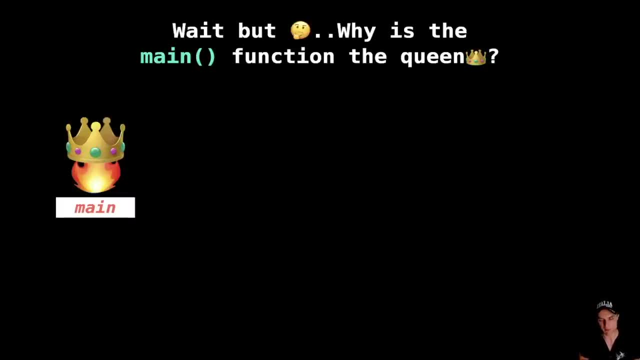 the main function and the printf- two functions, so a very simple program. generally speaking, we can think about a process composed of many functions. so we have this situation here: we have the main function, that is, calling another function as well as calling another function, and so forth. many, many 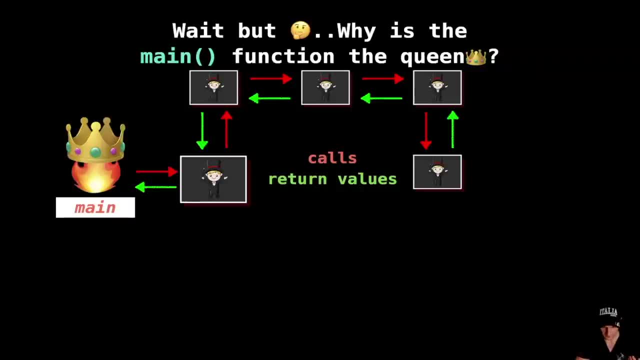 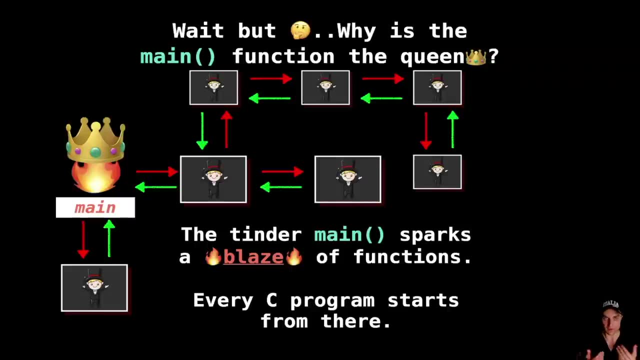 functions calling one each other. then of course i'm gonna have the return values for all the functions to perform a certain task- superior operation. so we have a giant calling of functions one each other. so we have all these black magic boxes that are cooperating when each other to perform a specific. 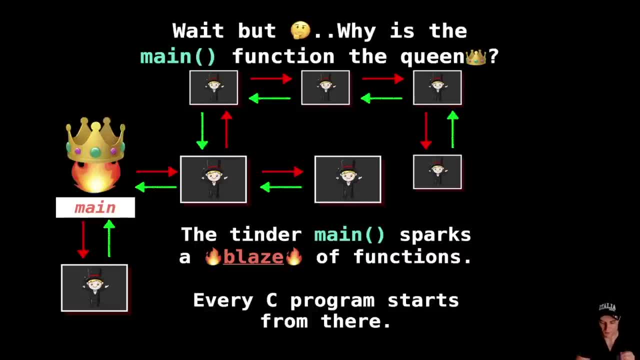 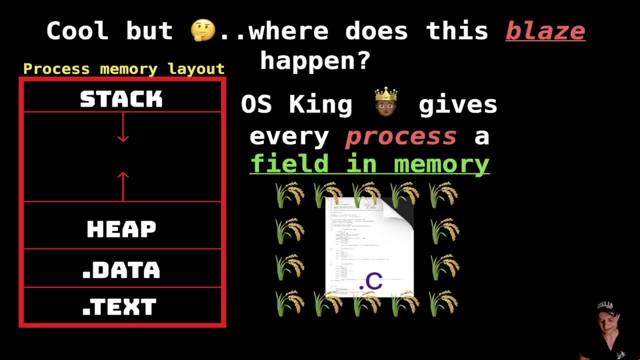 task to perform a specific application right. the main is pretty important because it's the tinder, is the one that is gonna spark all these madness of functions calling one each other. okay, pretty cool, but where is all this action? well, again we have to ask the operating system for resources. 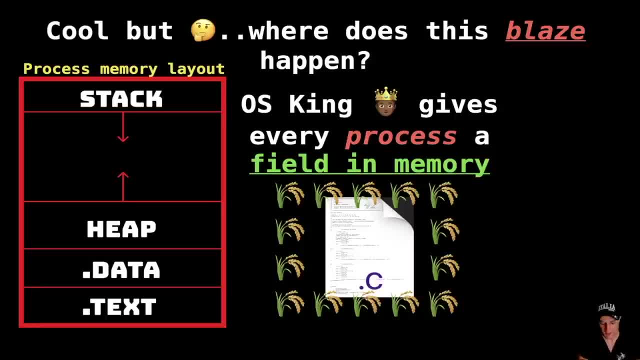 your process. we ask the operating system for some memory and that's what we're gonna get. we're gonna get um so-called process memory layout, which is this very strange um arrangement of memory. we have a stack heap the data and text, so these are sections that are going to contain pieces of 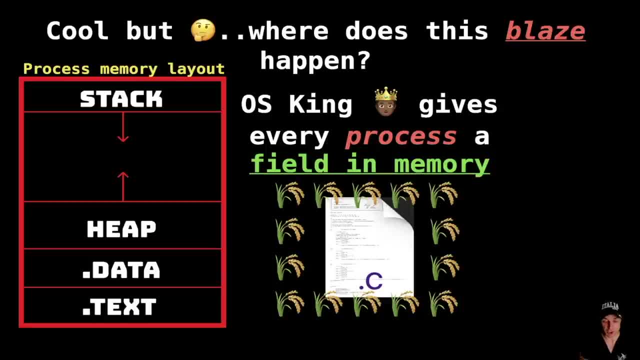 your process. for example, in the text you're going to have machine instructions. in the data you're going to have, for example, global static variables. in the heap you have the memory which is going to be allocated dynamically or at the runtime, and in the stack is where all the action is taking place. 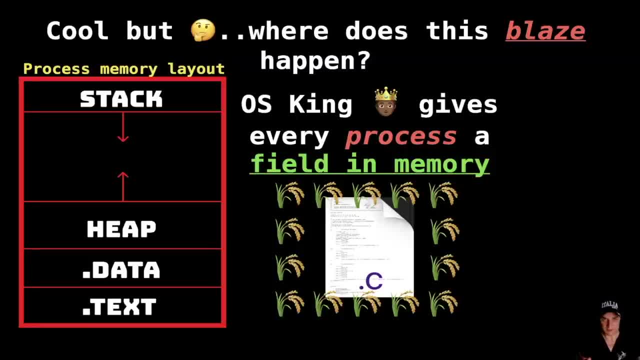 so, to make it very simple, the operating system is controlling all the ramp, all the resources, and is saying, okay, i have this process. i need to give him a specific spot in memory because he has to perform his stuff. so he's going to say, okay, take this field in memory, do your stuff and then give. 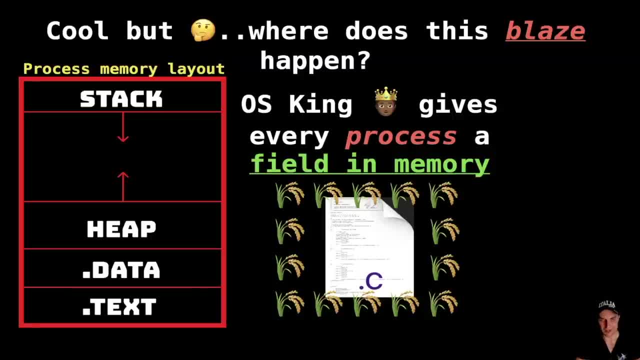 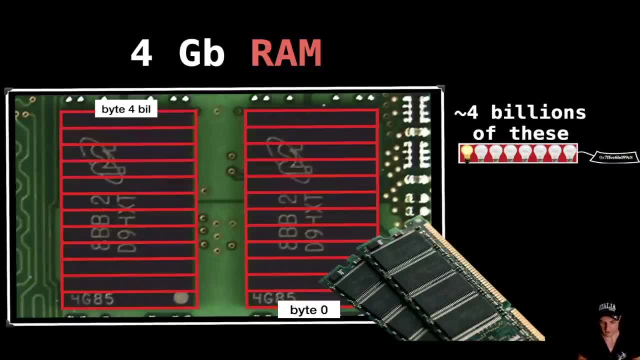 me back. i need the control back. that's what is happening. so let's zoom in a little bit and let's try to understand better what is going on. this, my friend, is the ram is the place in which you stock your numbers. you can view the ram as a chip or you can view as a programmer. the ram has a logical 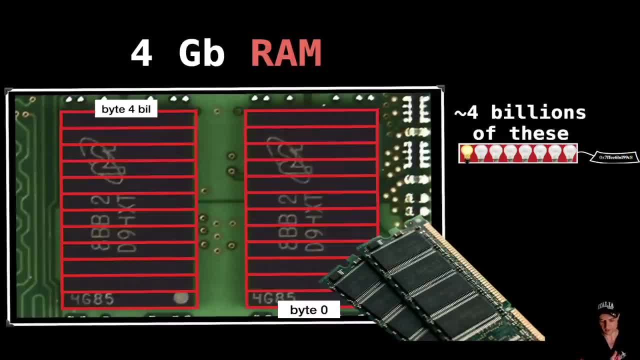 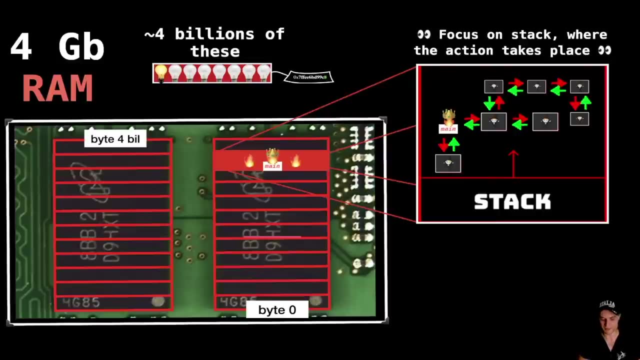 contiguous series of bytes. here is where your process is gonna take his piece of memory to perform his calculations. so if we zoom in, what do we see? well, we see something like that: your process intake is taking this slice of memory. of course, this is a super mega abstraction. this is more complex. 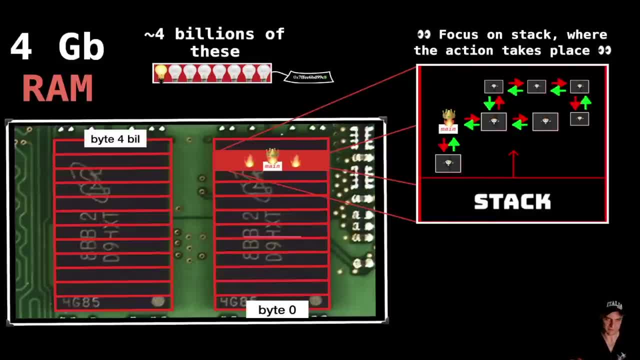 than that. it's not all contiguous and, yeah, you know, this is from. our reality is always more complex, but we want to grasp the principles. so the idea is that we take a slice of memory and inside the slides, all the action is going to take place. of course, we're going to focus. 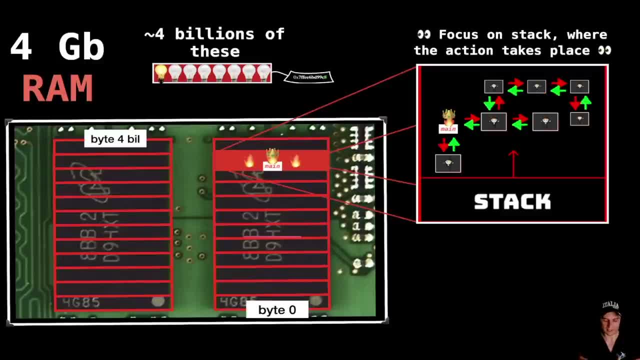 our attention in the stack, because here is where all the action is gonna take place. right, we have the main function that is calling another function that is calling another function forth. you can have call to malloc, so we have also the heap that is involved and other details. but 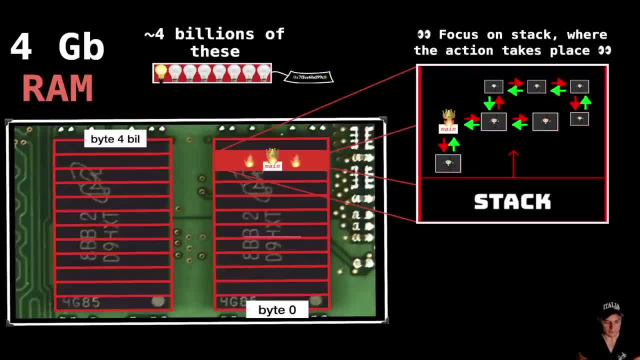 initially we're gonna focus on the stack, so i think you have already all the tools to understand what is going on with pointers. everything is happening in the ram. your process is a living being that is calling functions one each other to perform a specific task. every thing has a specific 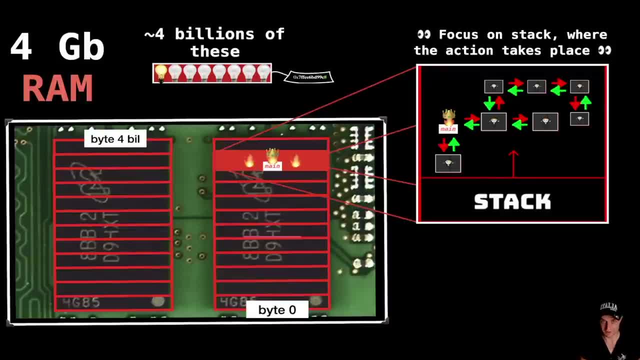 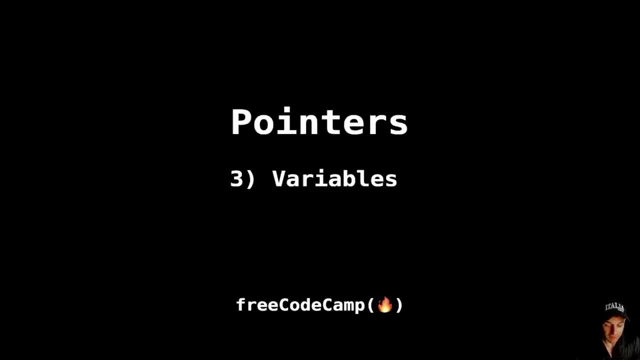 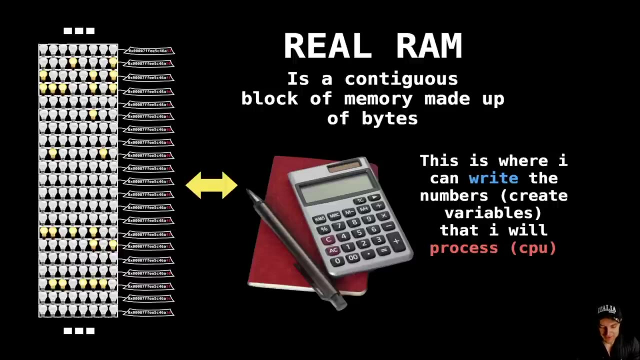 address. okay, these addresses are pointers, my friend. so now we go deeper. okay, my friend, we are ready to start our journey into pointers and we are gonna start with variables. of course, pointers are just addresses to variables, so we have to understand super well this concept. now we have this frame of mind that the ram is just a fancy, uh notebook right in which i can write. 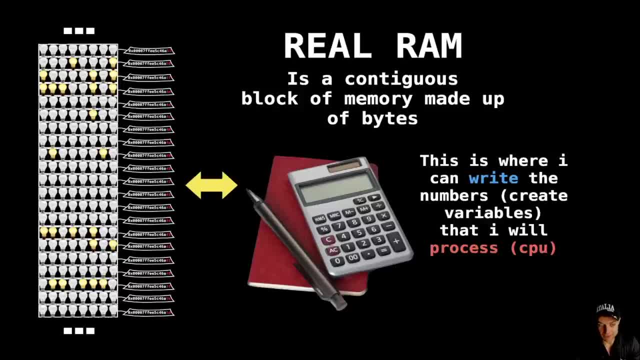 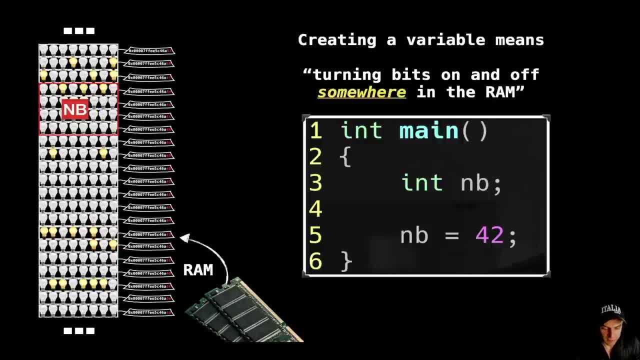 stuff in a binary fashion, because we are dealing with electricity and with binary entities, namely transistors, that here are just light bulbs. now let's make a simple example. as you can see here, i have a little main program that is gonna declare a variable and b and assign the. 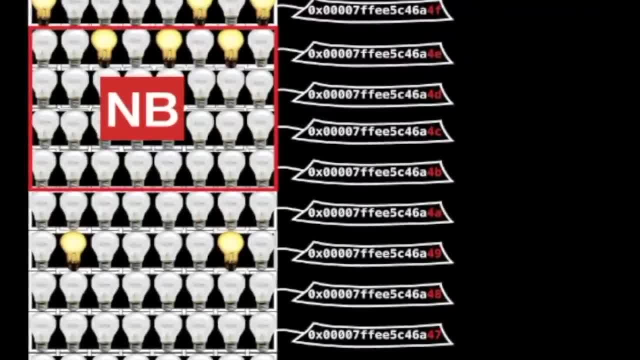 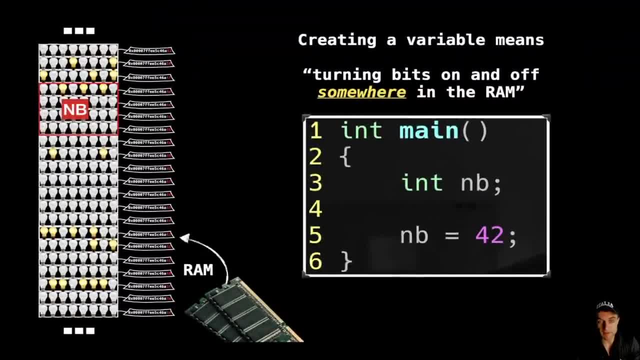 value 42.. so what is happening here with this code? very simply, i'm going to write somewhere in memory, in my ram, this number 42, so i'm gonna turn on and off the bits accordingly. for the number 42, i have one zero, one zero, one zero, as you can see here. four: 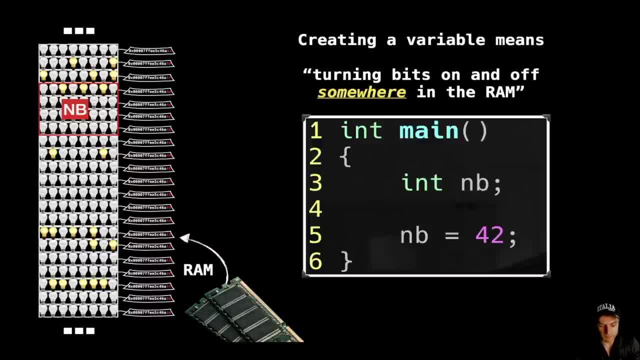 from the least significant bytes. okay, so i have, long story short, four bytes, depending on the machine, but generally speaking, it's four bytes allocated and i have the value one zero, one zero, one zero, which is inside these four bytes, and b is gonna be the tag for us, for humans, for programmers. 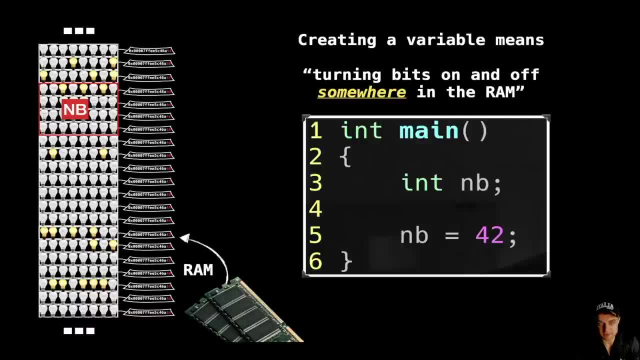 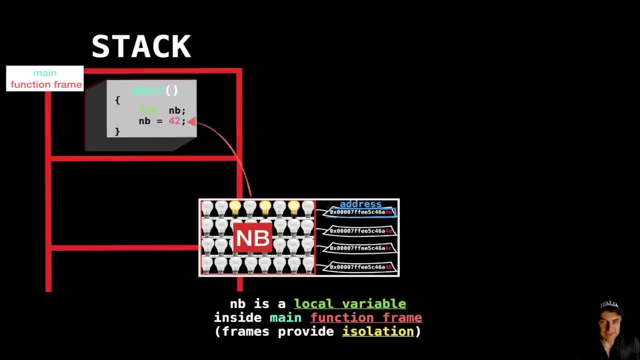 but from a computer standpoint we have only addresses, of course. so tldr, we have somewhere in my memory some bits which are turned on and off. now let's watch a second this little program from a stack perspective, because you know right, when i have a process i have 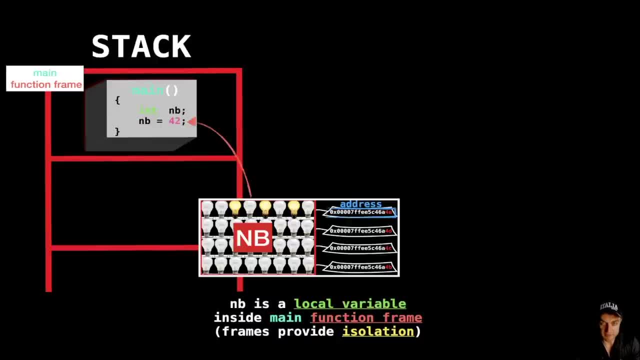 my operating system that is giving me a space in memory, the process memory layout, and all the action is going to happen inside the stack, the heap, the data and the text and all the segments that i showed you in the previous video. so the stack discipline, namely the allocation and the 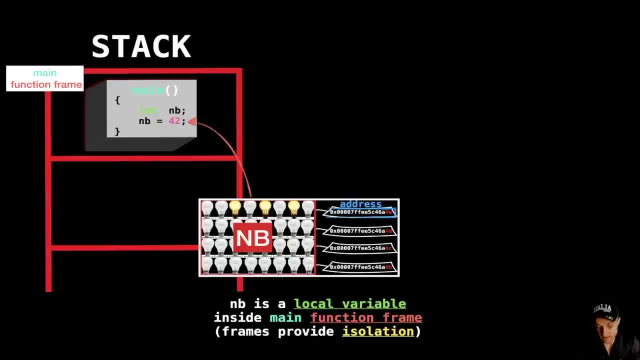 allocation of all the functions inside my process happens inside the stack, of course. so here i have allocation of my main. inside my main i have the creation of this variable and b, so i have a local variable which is inside the function frame of the main function- a function frame in this case. 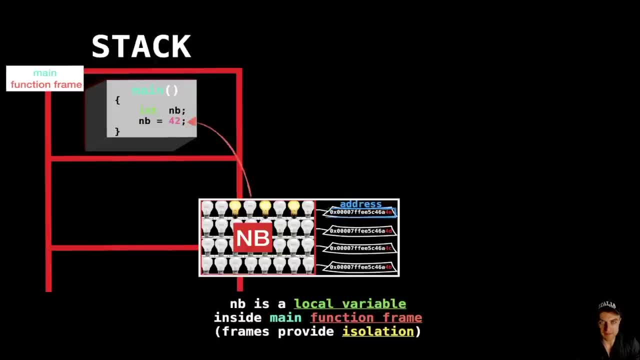 the main function frame is the specific space relegated to the main function. so the main function has this specific frame to perform its stuff. so inside this function frame i have the creation of my variable and b. okay, let's zoom in a little bit so we can understand better. 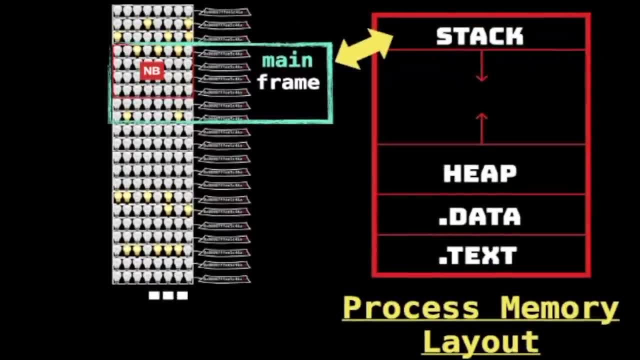 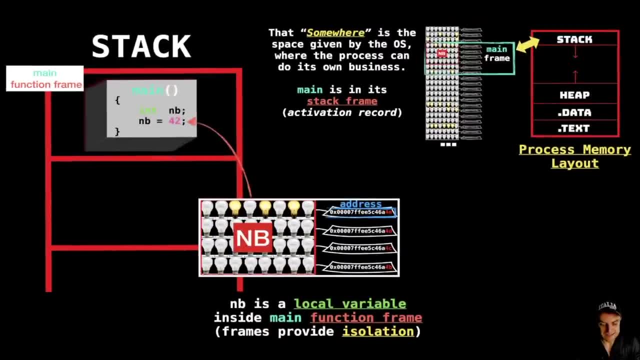 here i have my stack, and inside my stack i have this frame in which my main function lives, and inside this frame i have some bits which are turned on and off so that somewhere in memory is the space given by the operating system where the process can do its own business. of course now 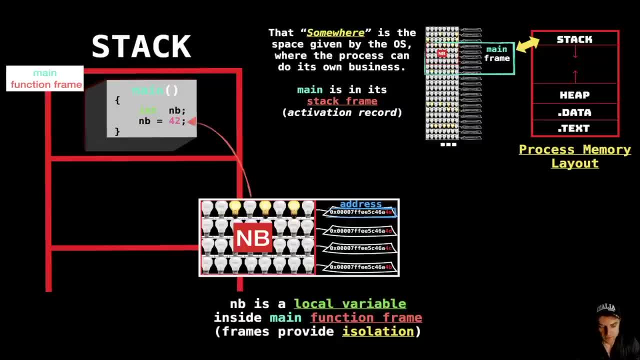 we are inside the main function frame because we are inside that function. now you see that the variable and b has a specific address, right? i want to stress out that this is not a real deal. this is not the real address, physical address. this is not what you find inside your real ram. indeed, this is. 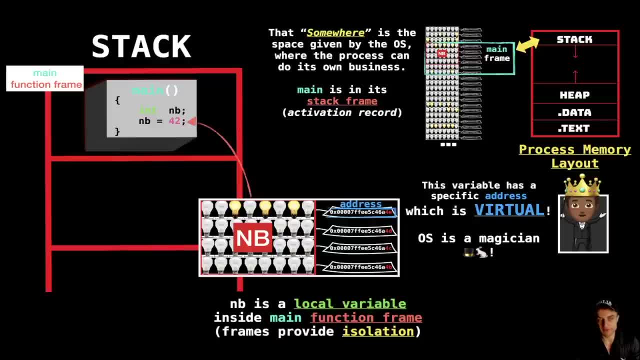 a virtual address. basically, we have the operating system, which is a juggler, is a magician, is doing all the tricks to optimize performance. as long as we are concerned, we don't really care for us programmers. this is the address of the variable. then we have some other pieces, like the memory. 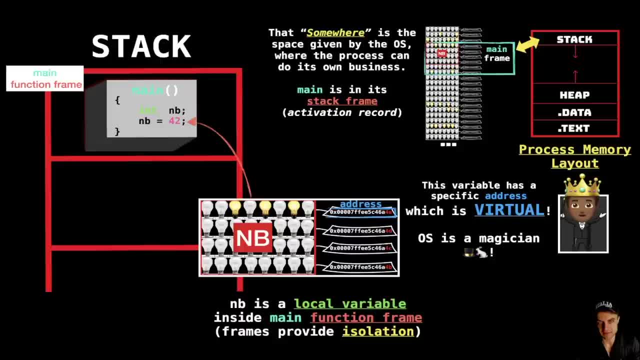 management unit that are going to make all the necessary computations to match virtual and physical letters. but we don't care, we don't care. we work on a higher level of abstraction. our process really thinks that has unlimited memory thanks to this magic of the operating system. but let me repeat to you, we don't care by now. we want to stick with principles. so an 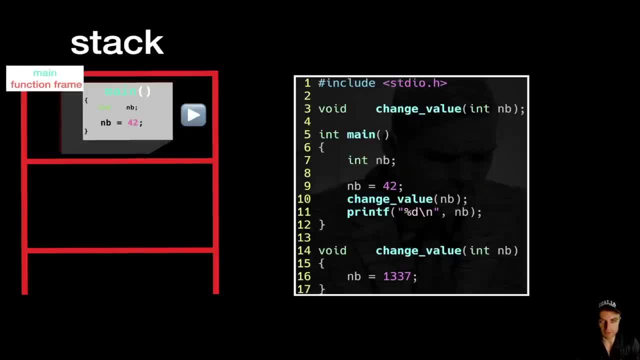 address is an address. now let's watch together a little program so we can really observe the stack discipline and what is going on inside the stack. so here i have a stupid program made up of a few functions. so i declare in my main the variable and b, like before. you just saw right, so our program starts. 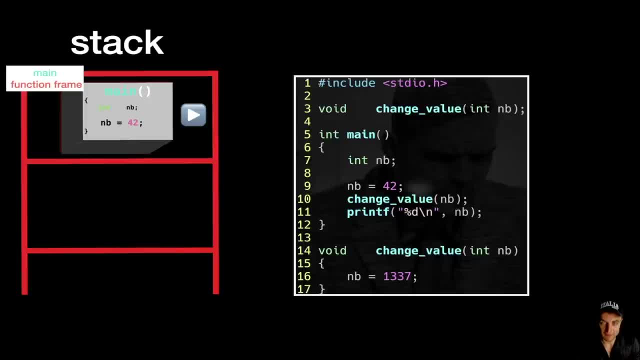 of course, from the queen function name is gonna declare and assign the value for two to the variable and b. so we have four bytes in memory that contain the value for two, one zero, one zero, one zero in binary. and then we reach the point of change value. so we have a function call change. 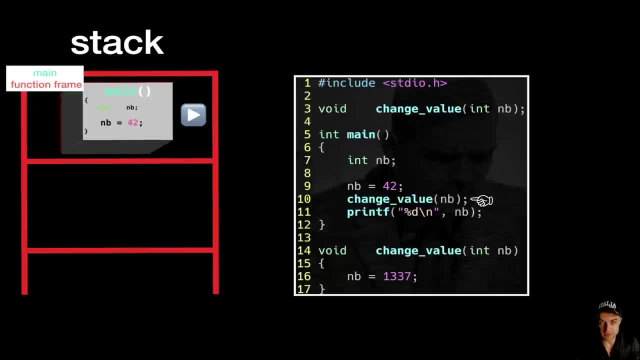 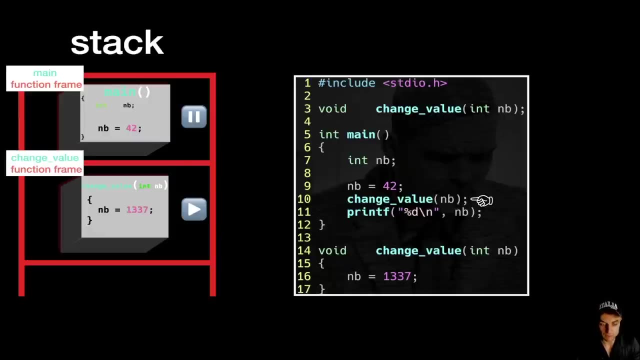 value is a function that essentially tries to change the value of the variable. let's see what happens here. so once we reach change value, we stop the execution of the main and we allocate space for the change value function. as you can see, the stack has grown and now we have. 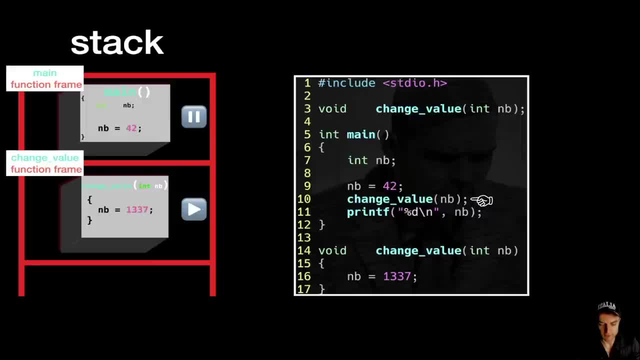 this new allocation, the stack counter-intuitively grows from top to bottom for historical reasons, but this is indeed a growth. so we have the main function that is stopping, and now we are playing the change value function. what is happening here? we have this function that is taking as an input. 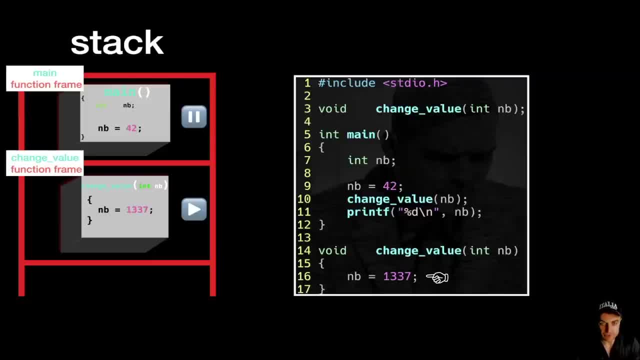 and b. okay, so our variable inside main, and it's trying allegedly to change the value of nb to another value, which is 1337. okay, what do you think is going to work, this little program? can the function change value, indeed change the value of nb? well, let's try. 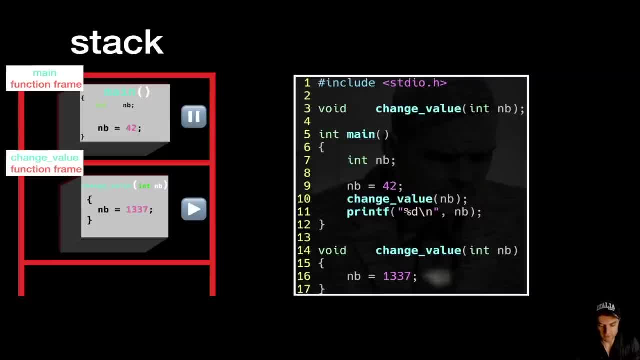 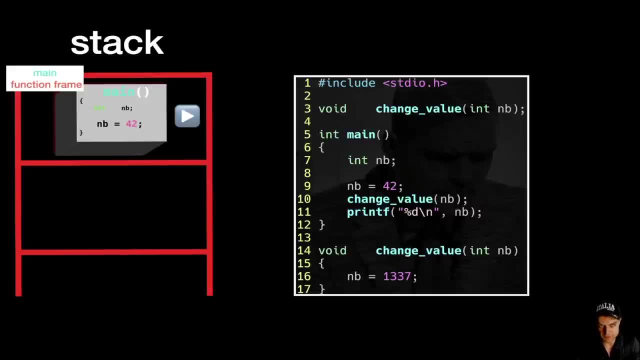 so we have the execution of nb equal 1337 and then we have the, the allocation, of course, of the function, because we have finished. a function finishes when we reach the final closing. curly brace, cool, now we are back to the main, we can play again the function. and now we have the call to 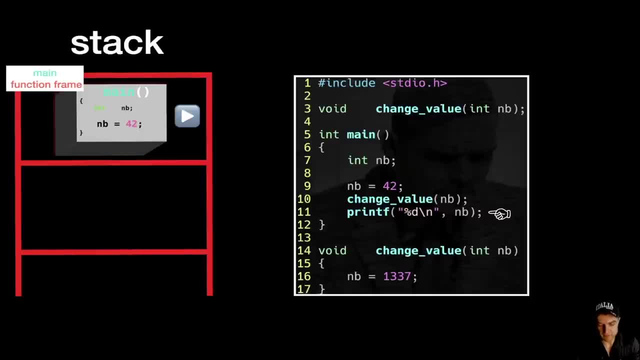 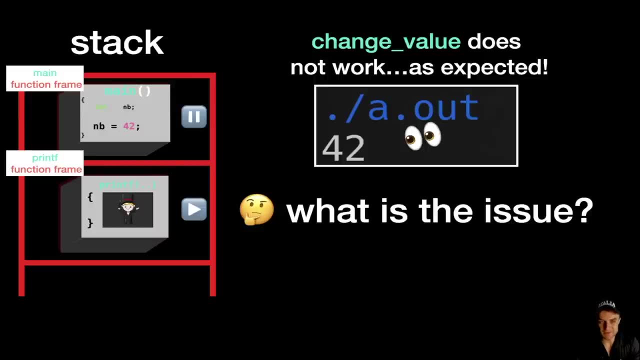 the printf function. the printf function, you know very well, has to print the value of nb. so we call the printf boom, we have the allocation, but now, as you can see, the printf is printing 42 again. so my change value function hasn't worked, or is it? namely, the function worked, but maybe i didn't quite. 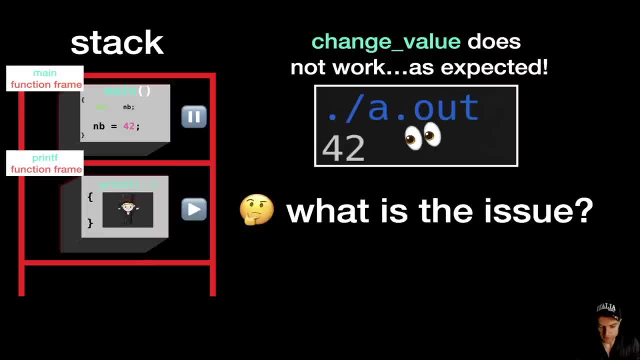 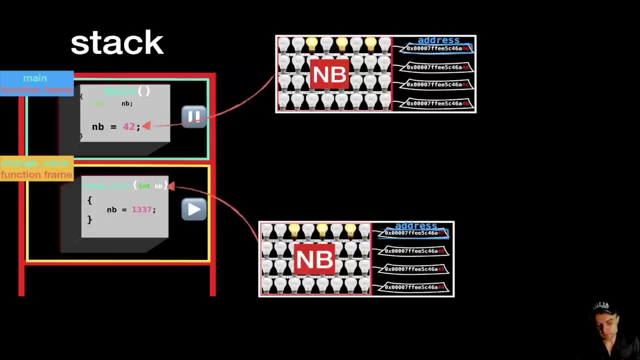 understand what was going on, right. so what is the issue here? what is the problem? let's try to understand and deconstruct this issue. so now we stop at the moment in which we were calling the change value function. so i have my main function frame and then i have my change value function. 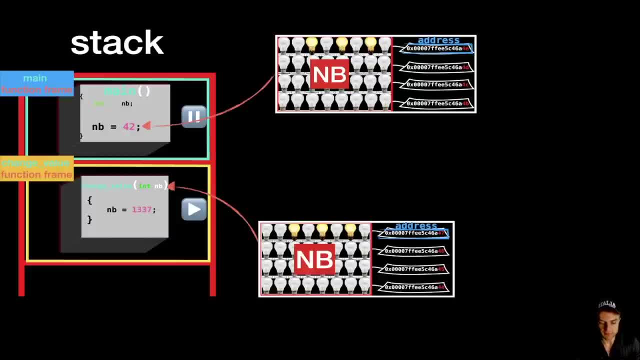 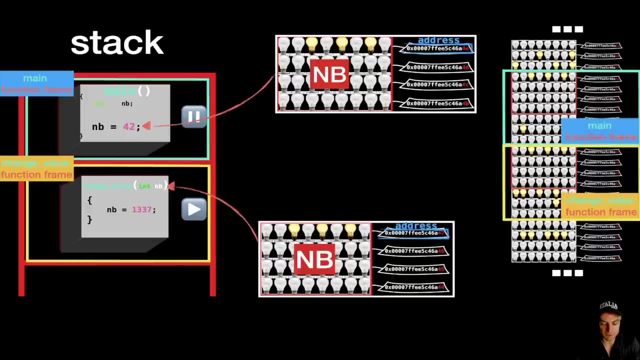 frame, as you can see. so i have my variable and b both in main and in change value. but let's watch more carefully what is going on here. so i have my function frame and my change value function frame inside the stack. as you can see, i have nb both in. 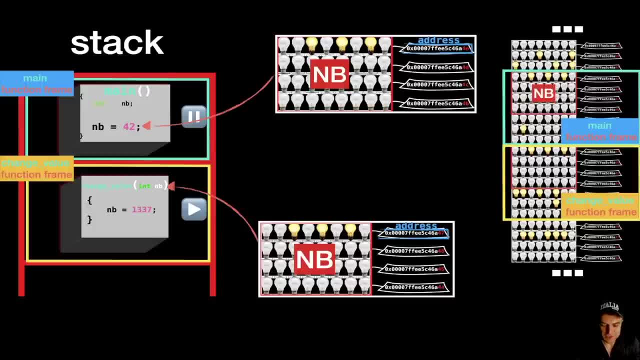 main right. and then i have also nb, which is in my change value function frame right. so, immediately, what can i understand? well, i have two variables. they have the same value, the same name, but they are different. they are in different spots, in different places in memory. so nb in main is a. 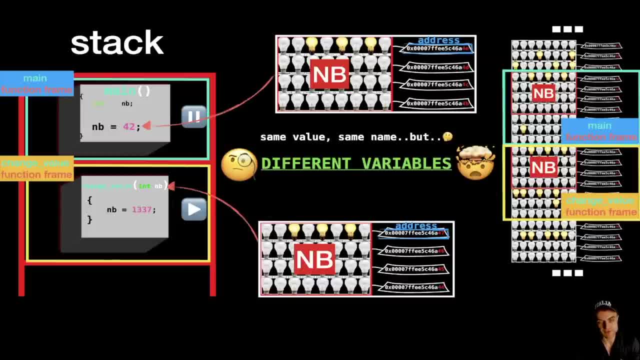 different variable, respective to nb, which is in change value. and this is tricky right. same name, same value. they are the same. nope, it is not the case. the thing is that when we call some functions, the arguments are passed by value, as we say in c. pass by value is a fancy way of saying well, 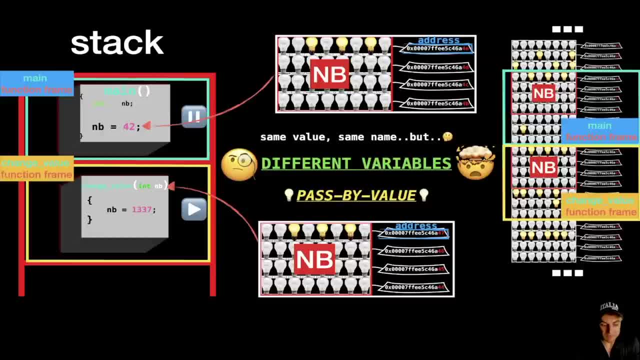 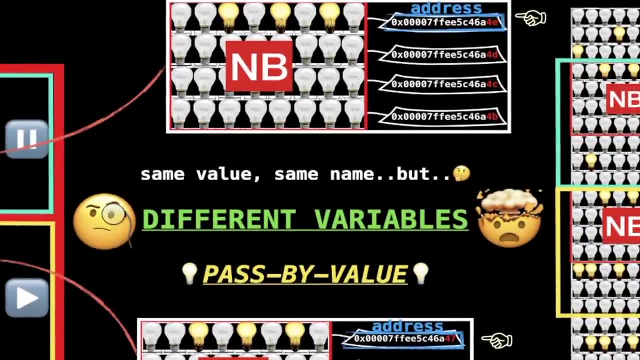 the variable is going to be copied. so what is really changing change value is a copy of the variable. it is not the variable which is in main. you see, and if you watch carefully, we have the addresses which are different. they are pretty close because they both live inside the stack and one function is just calling one another. so they are very, very close. but 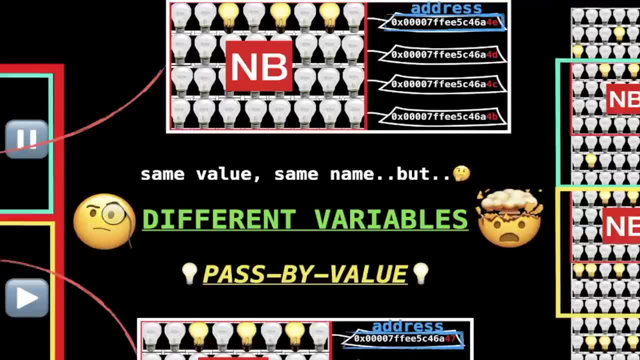 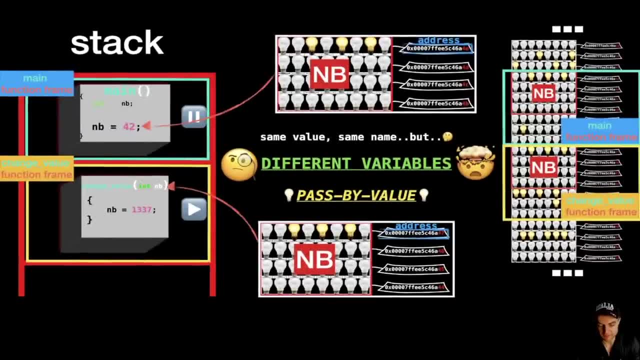 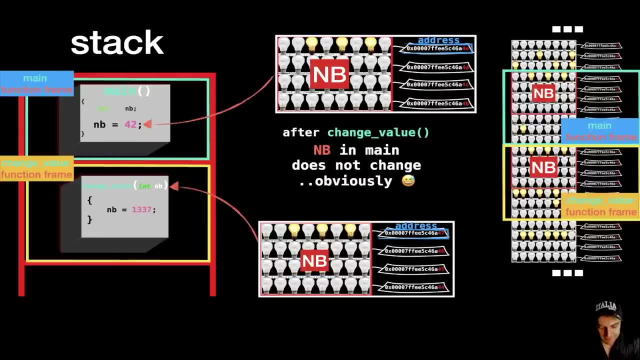 nonetheless, they have different addresses. that's the main idea. and to make it clear nb, in change value the argument name and b could have been different, like, for example, foobas. we don't really care because they are different things. so what is happening here? when i change value nb 1337, what is? 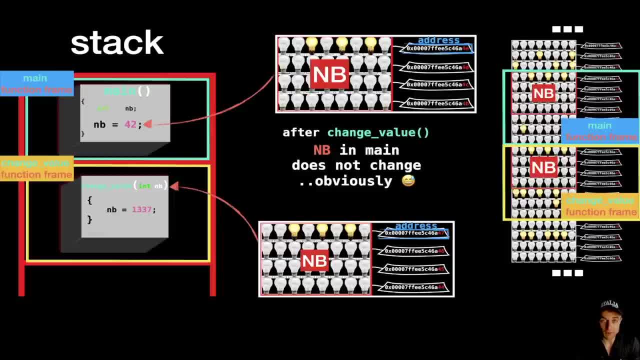 really happening? well, the function is changing the value of its own copy and it's not changing the value of nb, which is in the main function. you see, that's the catch. so let's watch what is really happening. we have our variable in change value. that boom is changing its value, as you can see. 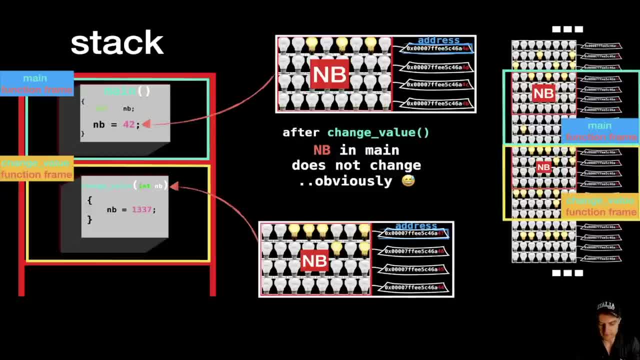 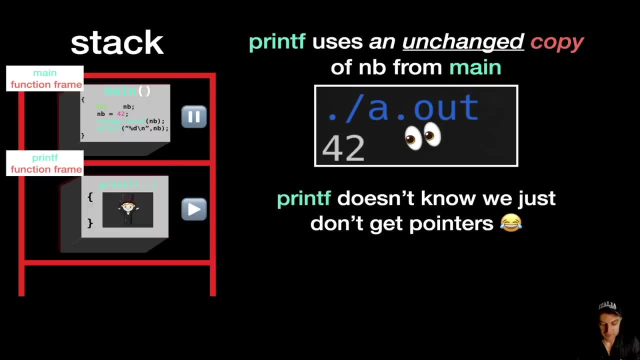 i've changed the binary configuration. now this binary state is representing the value 1037. but then what is going to happen? well, we have the location of the function change value. so boom, and in the main function i call again the printf. but the printf is getting the old 42 right, because i've changed the value which was in another stack. 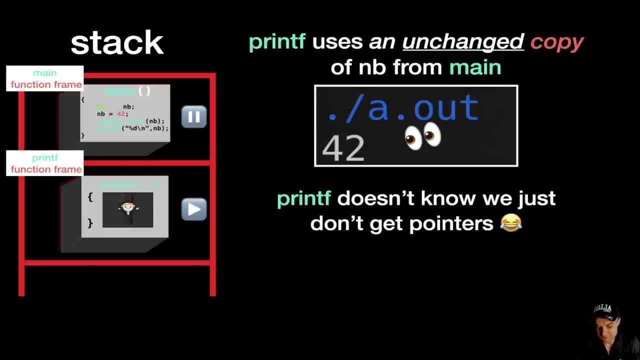 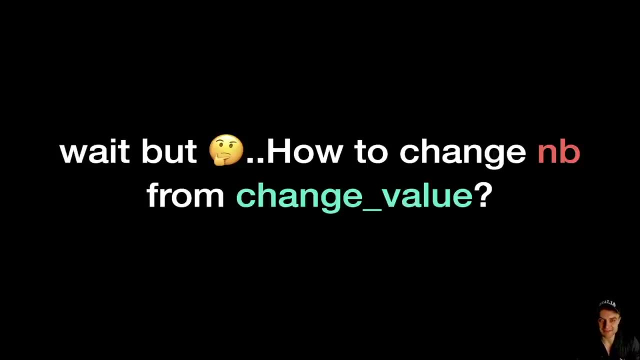 frame. so nothing really changed. so printf simply keep using the usual nb42 and the printf is not aware that we don't understand pointers, my friend. so what can we do if i want to change nb, which lives inside the main function frame? what is the trick here? well, my friend, that's where pointers come handy. you see, let's. 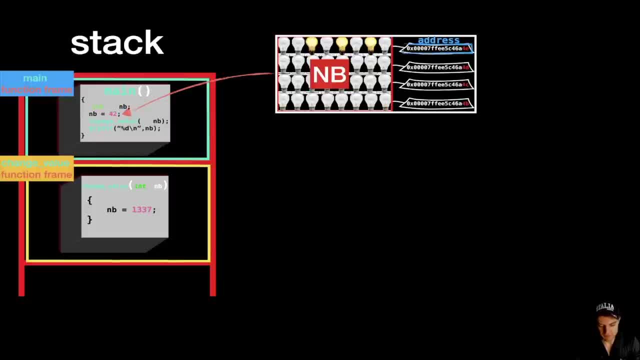 re-watch again the animation. i have my main function. inside the main function i have the variable nb. then, instead of calling change value with nb, i'm doing something different. i'm using the ampersand operator. this ampersand operator is giving the address of the variable. 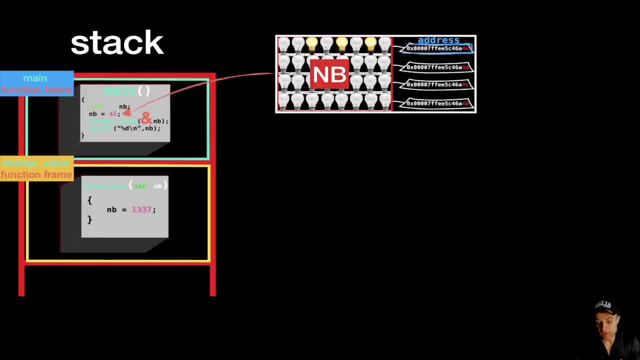 to the called function, in this case change value. so i have to change also the change value, because this time we are getting different kind of inputs. carefully, change value is taking this time. a pointer to nb. we use the asterisk operator and as well, nb equals 1337. we have to change a little bit. we have to say at and b, so i'm gonna. 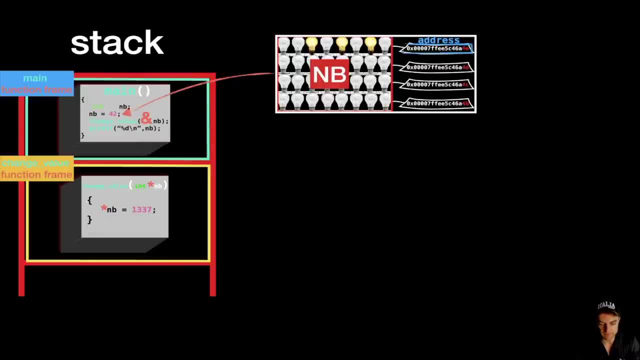 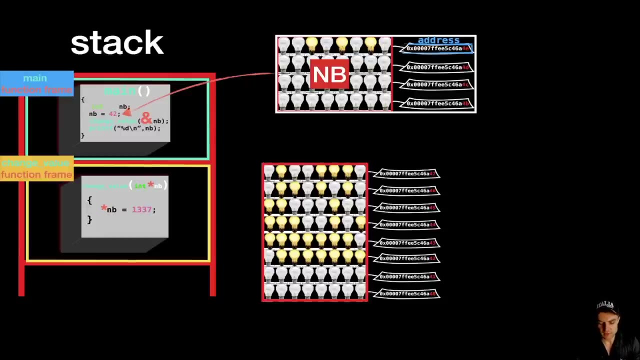 dereference. this, indeed, is the reference operator we will see later. so this time the input, the data type that change value is taking, is not anymore a variable, but it's a pointer. it's this big boy here. he is eight bytes generally speaking, but depending on the machine, that is able to point indeed somewhere. so this: 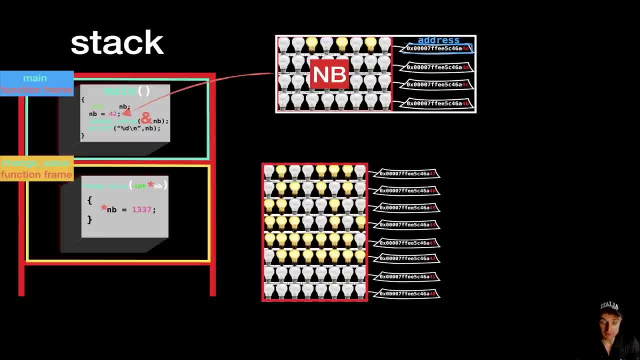 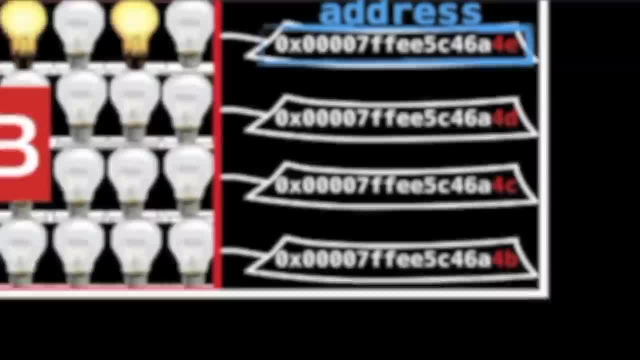 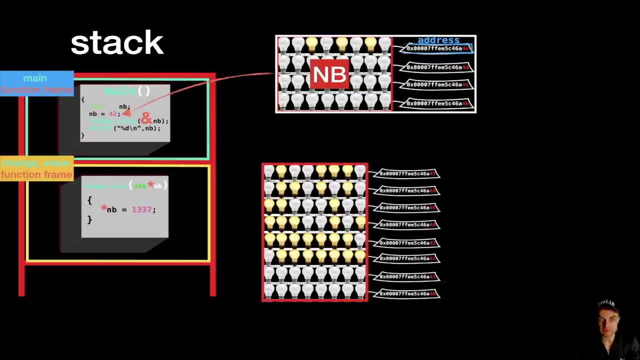 variable contains the address of another variable and if you watch carefully, you see the binary configuration of this variable, which is exactly the address of nb. so this pointer is a special kind of data that is able to point somewhere in my memory. we can make, indeed, reference to something which is not here, not in my 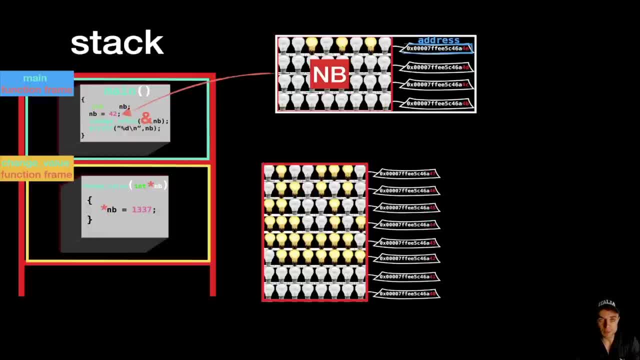 local frame, not in my local function frame. indeed, when we say dereference, we are meaning reference to something which is not here, which is far. think about the word I don't know, deportation. bring someone far. that's the idea here. we'll make you reference to something, far the reference. and when I say star and B, I'm 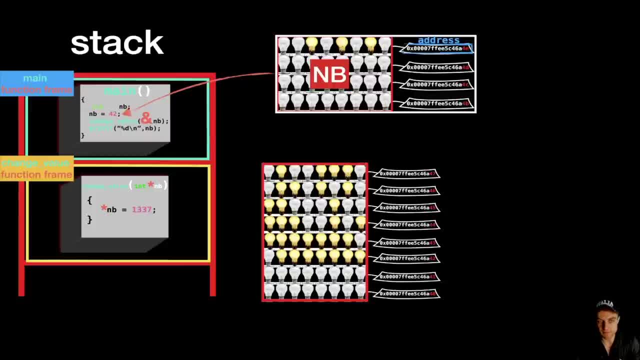 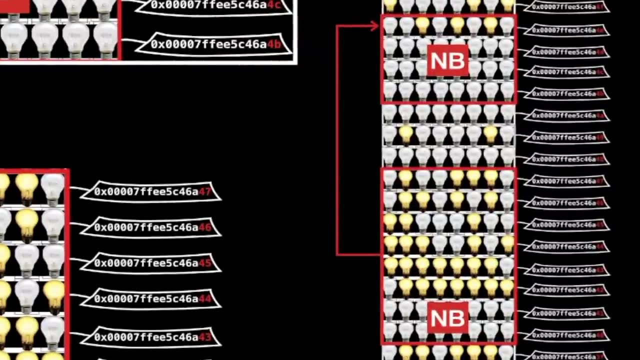 saying a, go in the address pointed by on B and put a there the value 1337. okay, so we have this condition this time. let's watch the stack frames. as you can see, I have NB and both NB, so I have my main function frame and then I have my change value function frame. but this time, thanks to 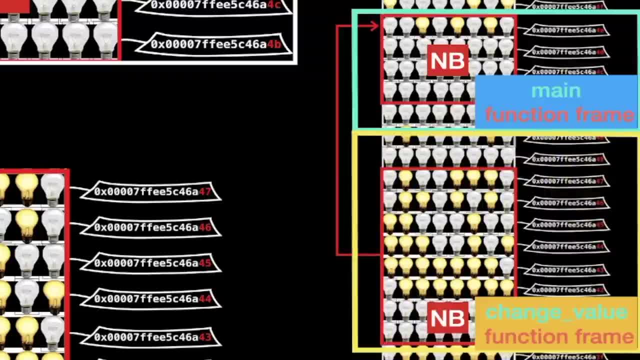 NB and I'm gonna do and gonna dereference this pointer. boom, so I can access the NB which is in the main function, and then I just do. at NB I can read in this fashion: asterisk, asterisk, asterisk, asterisk asterisk can be is equal to 1337. now look here for the what is going to happen? boom, I'm. 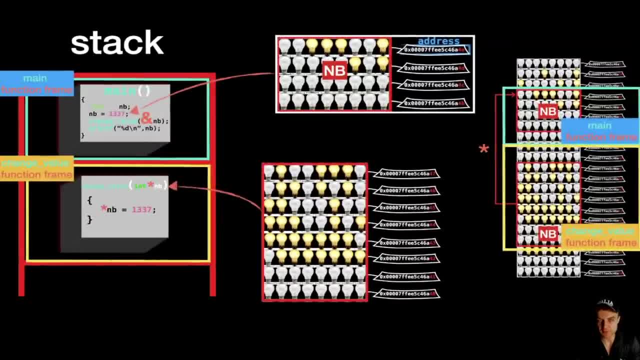 gonna change the value there, okay. so thanks to the magic of pointers, I'm able to go somewhere else and change values. this, my friend, is called passing a value by reference. not by value, but by reference. so we give to the function a specific address, a specific place to watch if we want to do its business. so 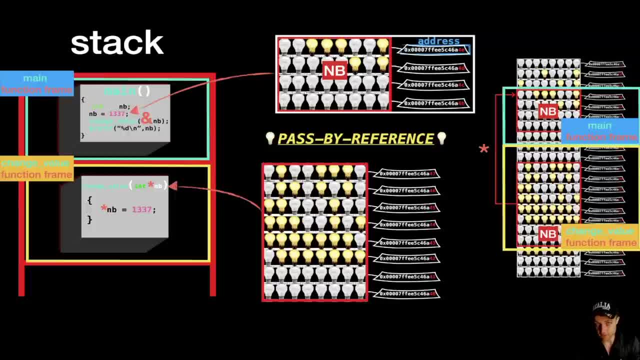 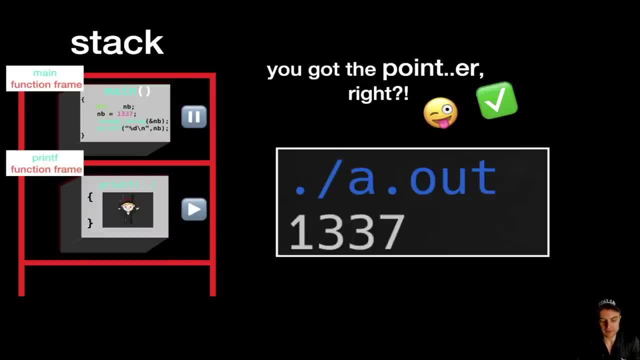 which is very different from passing an argument by value. right, you just saw. so we have the change value function that gets the allocated when we reach the final curly brace, and then we call again the printf. this time the printf is getting as an input and b, which has been changed, you see. 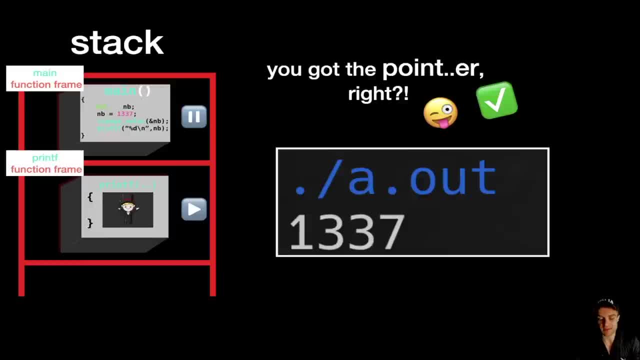 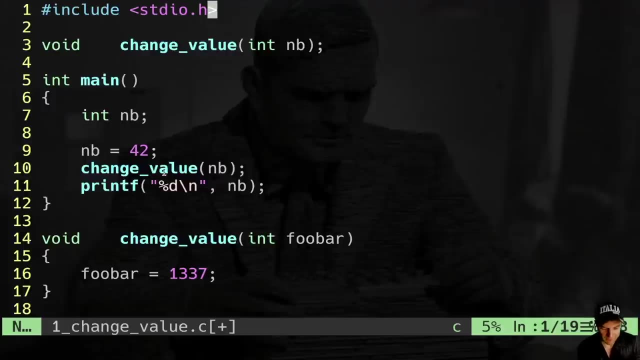 i have 1337, so everything works. thanks to the power of pointers, thanks to the power of dereferencing- making reference to something which is not in my stack frame and we're ready to rumble- you have the tools to understand everything about pointers. okay, my friend. so here, my friend, i have 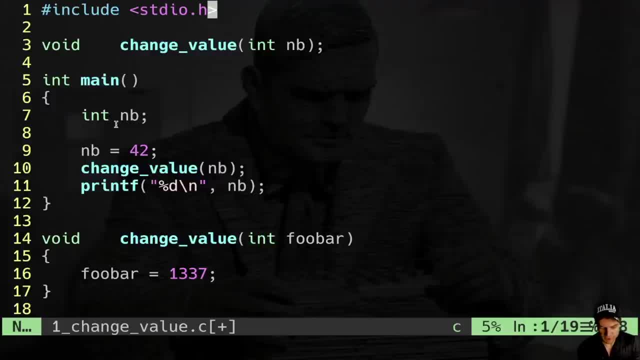 the actual code, as you can see, my main function, in which i declare my variable and b equal 42, and then i call my change value, the, the function you just saw. i call my change function. here i call the variable and full bar. just to stress out that this is gonna be different. this is gonna be a copy of 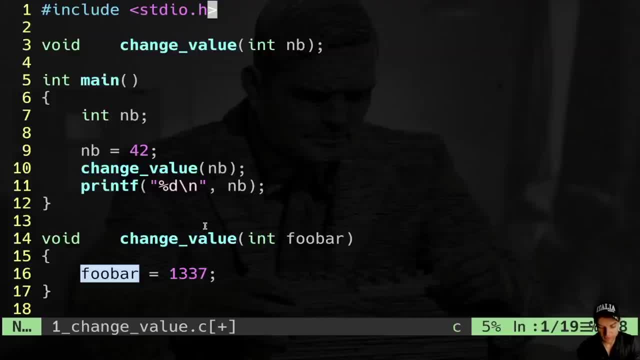 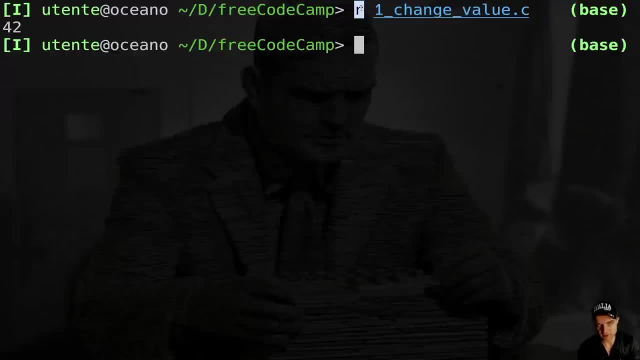 nb and you just saw that this program doesn't work. let's try out. so i'm gonna run my program and i get 42.. as you can see, r is just a function that i created. it's just compiling, doing all the checks and so forth. it. 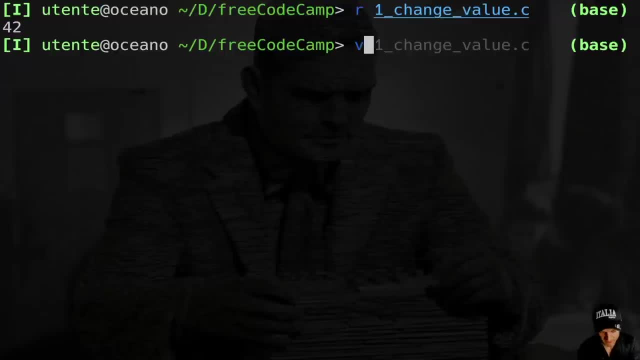 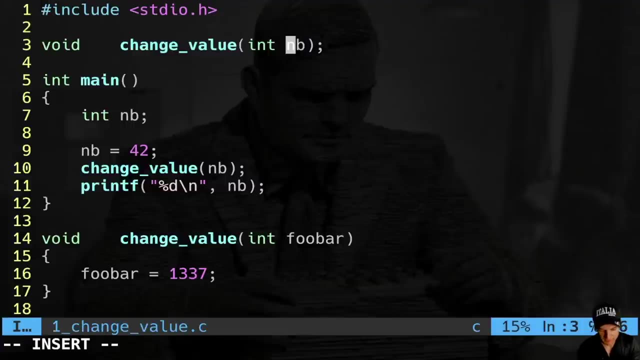 is like gcc and then launching it out. it's the same. so we watch again the code and this time we're going to tweak a little bit. first of all, i'm going to tweak the prototype so the function is taking an address as an input, so i have to use the star. i will explain later why. here i don't have 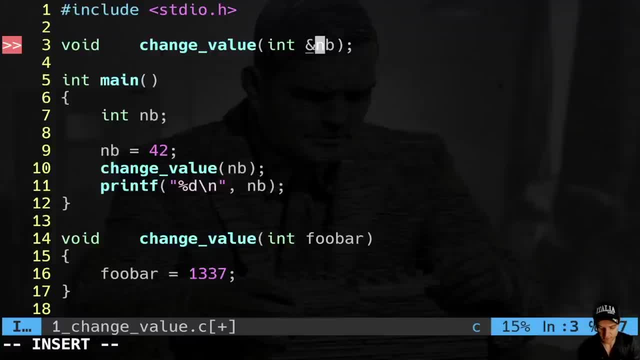 the ampersand, because this is a little tricky. the syntax of pointers is kind of tricky. i will explain. so here i have a pointer, here i give as an input an address, so ampersand on b i'm giving the address of mb and here again i have to use a pointer. here and here i have to dereference the difficult. 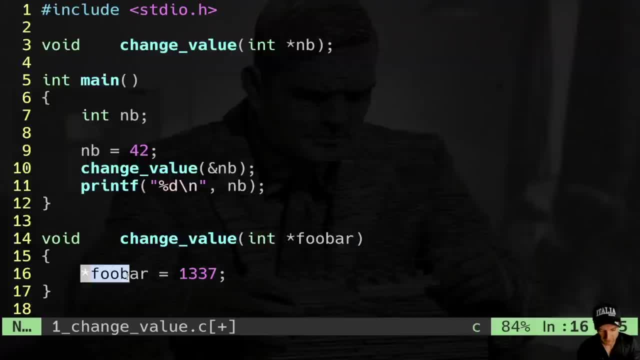 part, in my opinion, is that declaration and dereferencing are the same right. we have the same syntax. this is tricky, but no, not really. i will explain to you now. we're gonna run again this program. so i'm gonna run and you can see. this time i have 1337.. it works. 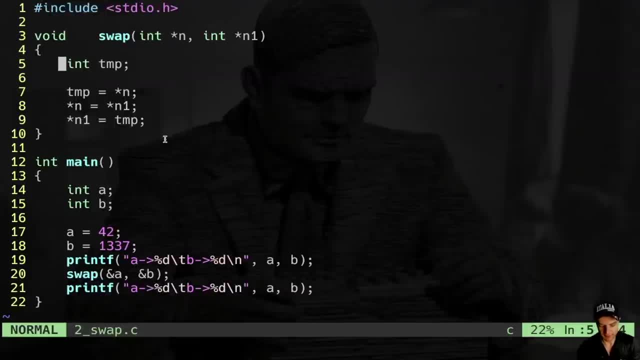 now let's watch again the classical example of um using pointers, and this is the swap function. right, i have two variables in my main, which are 42 and 1337. i'm going to print their values, then i call the swap and then i'm going to print again. as you can see, this is what the reference to the 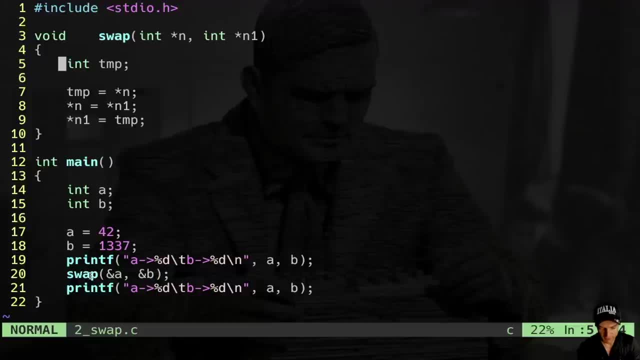 two variables, ampersand a, ampersand b. so my swap is receiving the addresses of a and b, as you can see from here the signature of the function. right, i have as an input two pointers, pointer n and pointer n1. then i do my swap routine, which is just making a temporary variable in which i can stock. 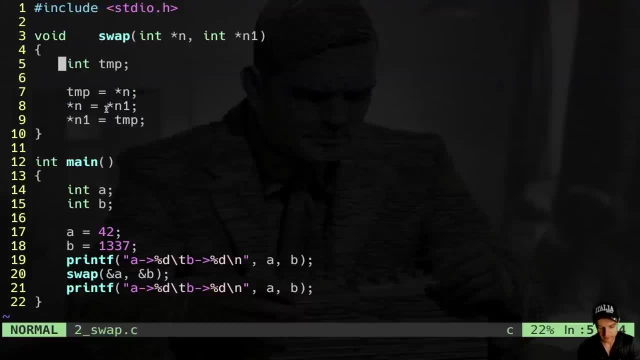 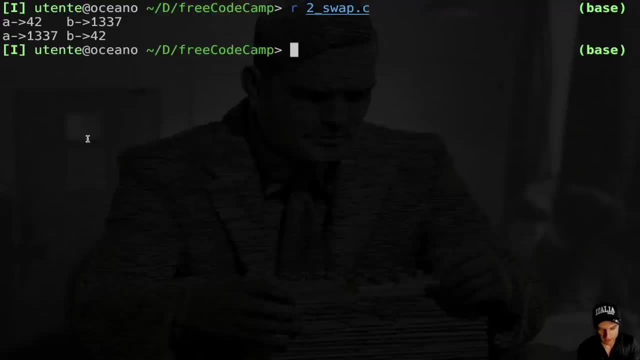 the value of n. then i say at, n is equal to at and one. basically, this is a stupid swap algorithm. so let's try to launch this and you can see that it works perfectly. so you understand super well by now what is going on. right with this um pointer. 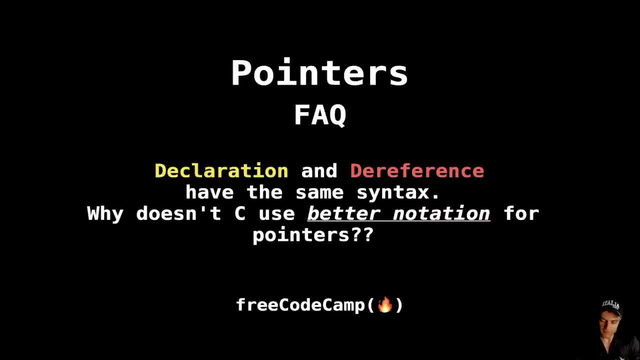 so now the tricky part: uh declaration and the reference have the same syntax. why doesn't c have a better syntax for doing this, namely a different syntax for the referencing and uh, uh respectively. another different syntax for declaring. this is confusing. initially it was for me a little. 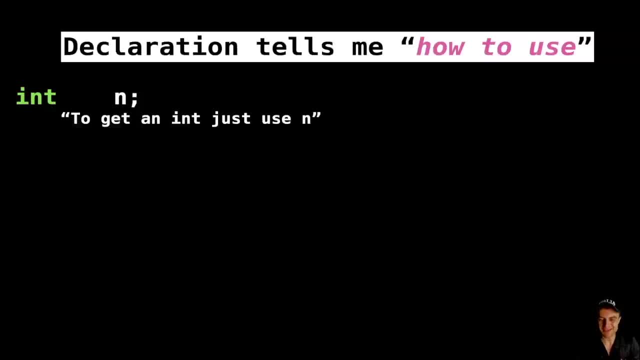 confusing. keep in mind this principle i have. that declaration tells me how to use. what does it mean? well, let's try to understand together. i have here a declaration of a variable, int and right, a classic declaration here i read in this fashion: to get an integer, just use n. that's why 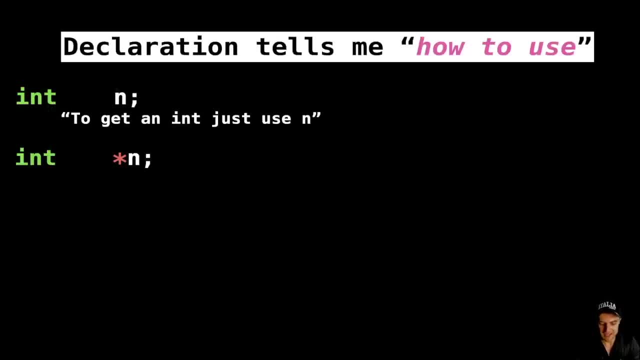 i read even this declaration. let's try another int star n. what is written there? well, it is written that i have a pointer to an integer. so i read: as a programmer to get an integer, just the reference n. you're starting to understand, i guess. right here i have n 3, which is an array of three integers, but 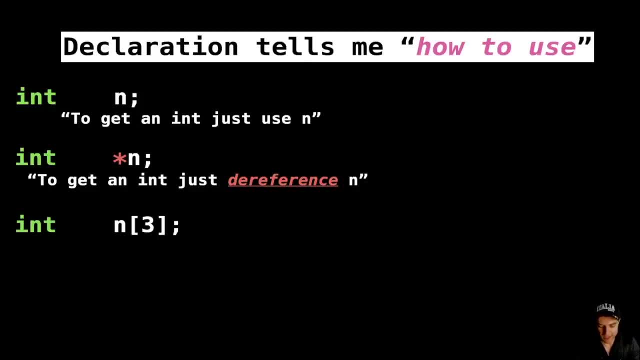 here i read in this fashion: to get an integer, you have to index inside this array a value. so in an expression and square bracket, 0, 1, 2 is gonna yield an integer. the last example is a function. for example, we have a prototype, foo, int n, float n1. what do i read? well, i read that to get an integer, just call foo with. 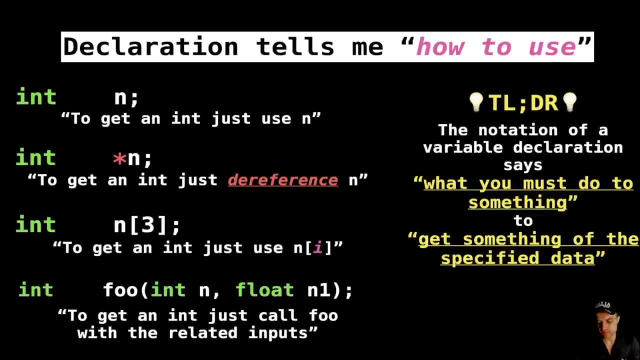 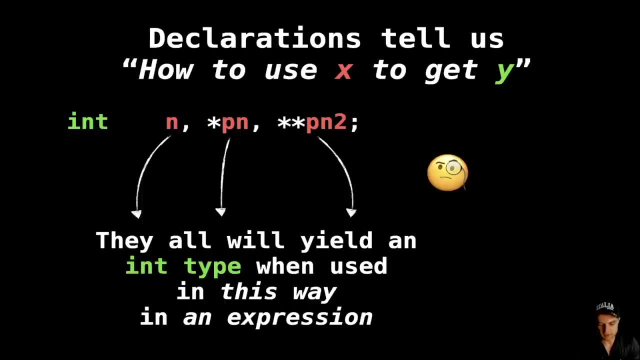 the related inputs. so tldr. uh, the notation of a variable declaration is telling me what you must do to something, something of that specific data type. let's apply this principle to pointers. here I have a declaration of different pointers and you can see I have int n. 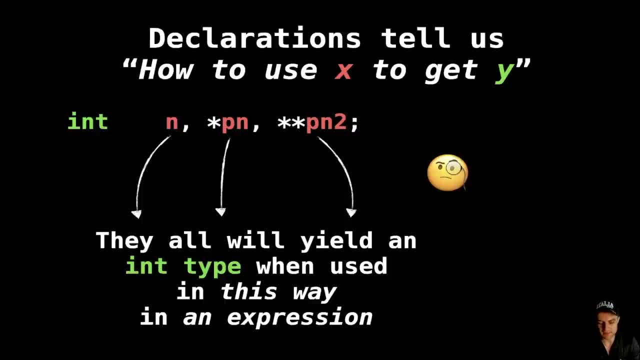 this is just a variable. then I have star P n and then a star star P n. what do I read here? well, I read: to get an integer, use n, use the identifier, the variable identifier n, or you can use star P n, or you can use star star P n. they all will. 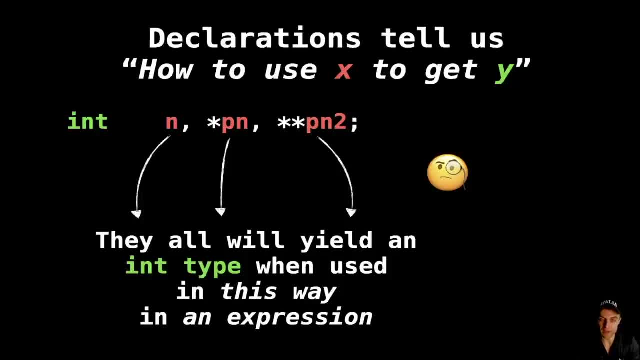 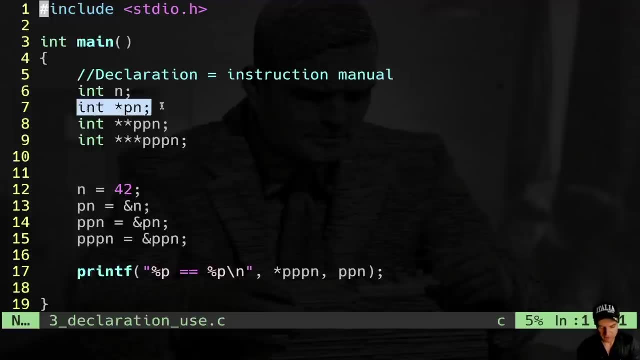 heal an integer type when used in this way in an expression. so in my view, in my mind, and declaration is an how to use, okay, to get a specific data. so here, as you can see, I have many different declarations for different declaration. so I declare here a pointer, a double pointer, a double level pointer and a. 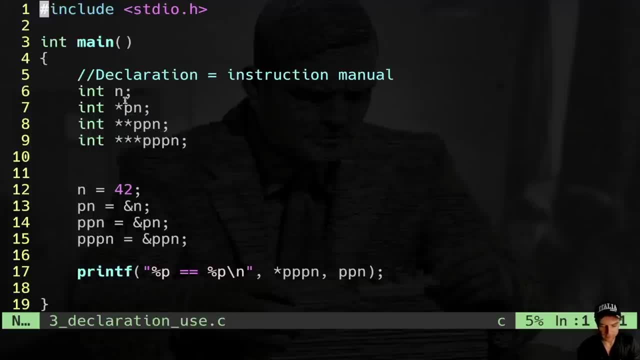 three level pointer. okay, here, given the principle I just told you, I see that I have to use this identifier variable, identifier variable, name, call as you want to get an integer. here I have to use star P n to get an integer, and so forth. right, here I have to use three times to start on this P, P, P and to get 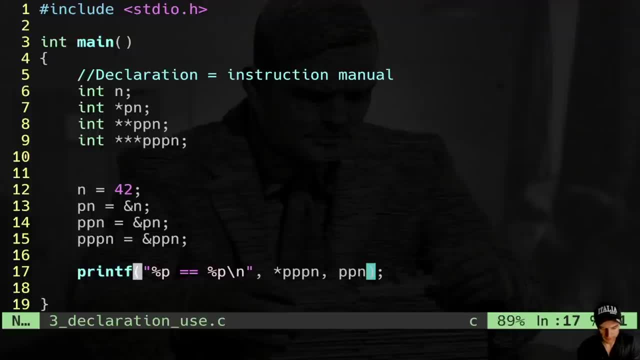 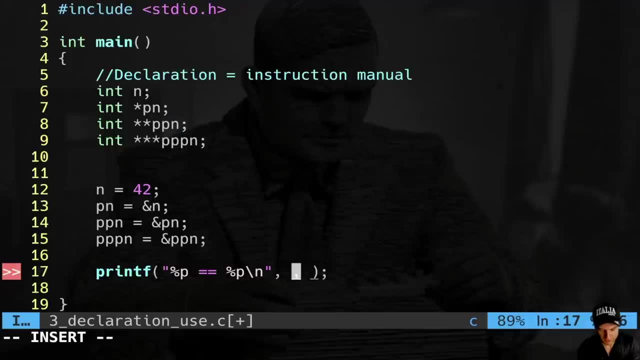 an integer. so if I want to get, for example, an integer from this, what shall I do? well, I have to use two times the let's delete this and let's do that print tough person. the new line I have to do to this boy: here you triple the reference pump, pump, pump, but a triple the reference P, P, P, n, like that. 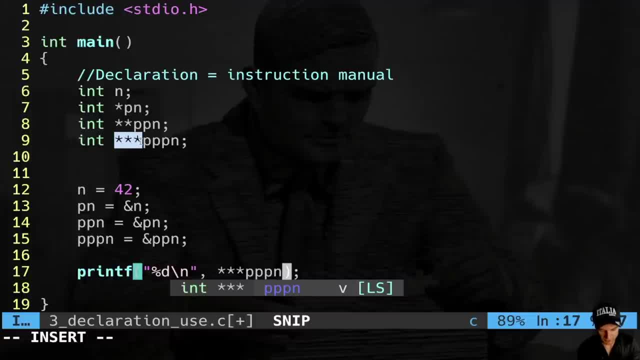 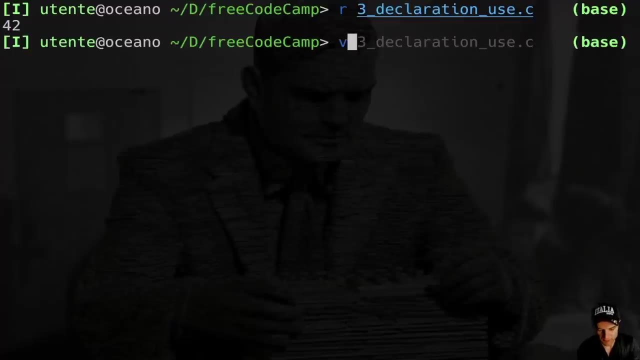 and this is gonna heal an integer, because here is written: if you triple the reference this boy, you get an integer. if you single the reference this boy, you get double pointer to integer. you see, you get the catch. let's try if it works. so I run the code and, as you can see, I get 42. I get the number 42. 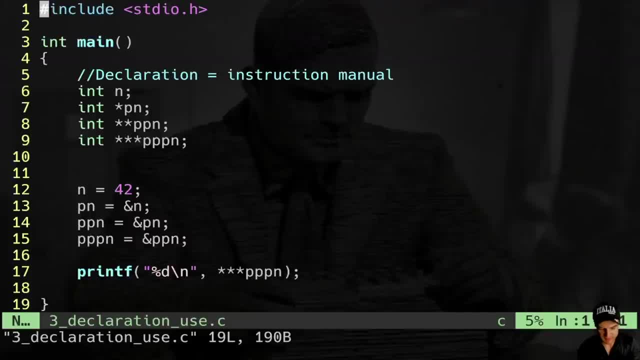 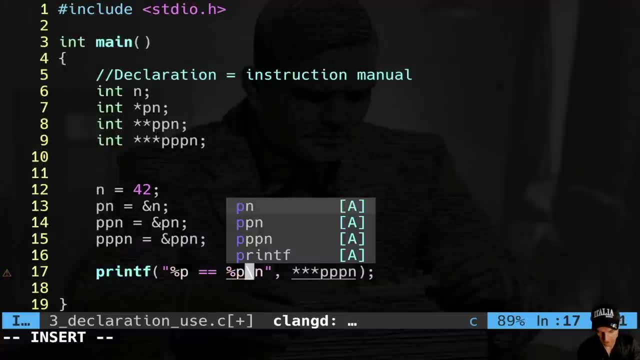 perfect, because I triple the referenced this. now, if I do something like that, I do P. the standpoint pointer is equal to p, another pointer. so what do I do? I double the reference this. why a double reference? well, because if I double the reference, this boy, I get a pointer to an integer and the. here I use P, n, which is: 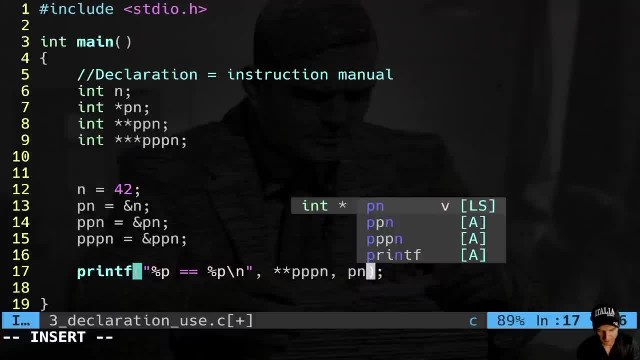 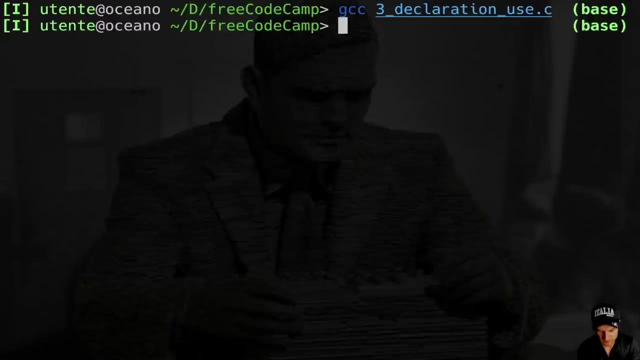 what a pointer to an integer, so I'm gonna use directly. we know the referring because these, if I use these, I get a pointer to an integer, I'm not the reference. you see the, the catch- my friend let's watch works. okay, here i have some controls that i made, so i'm gonna do like that gcc and then launch boom. 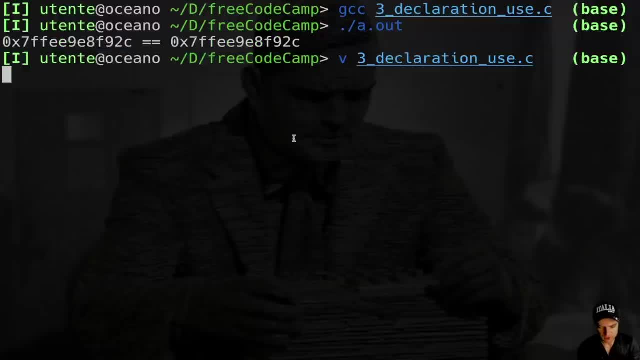 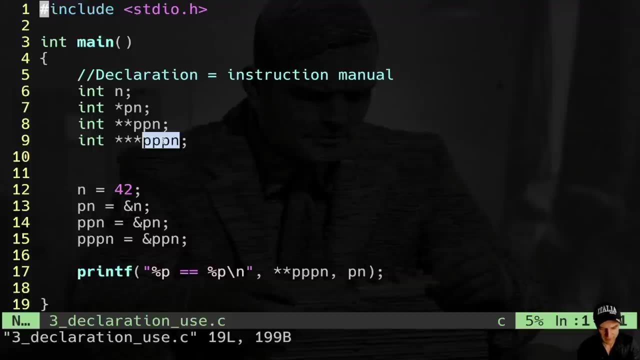 as you can see, they are equal. they are the same right. so just keep in mind what i told you. this is an instruction manual. it's telling you how to use this uh ppp on to get a specific data type. if you do a triple d reference, you get an int. if you do a single, you get a double pointer, and if 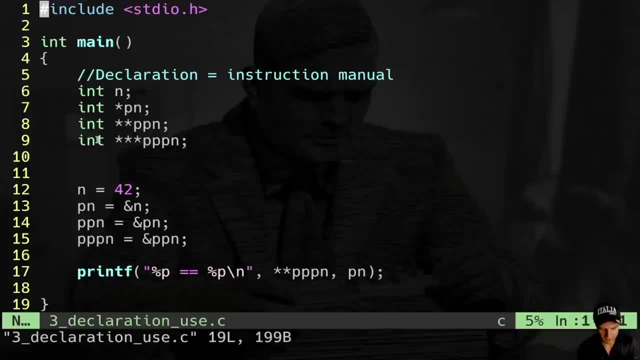 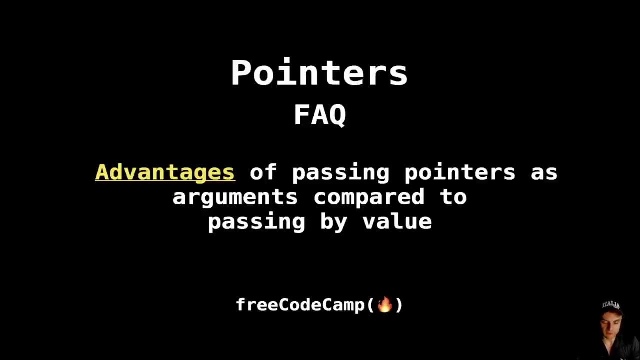 you do a double the reference of this, you get a pointer to an integer you just saw here. that's the idea. okay, my friend. so i guess, uh, these declarations are not gonna be difficult anymore. now another question: which are the advantages of passing pointers as arguments compared to passing? 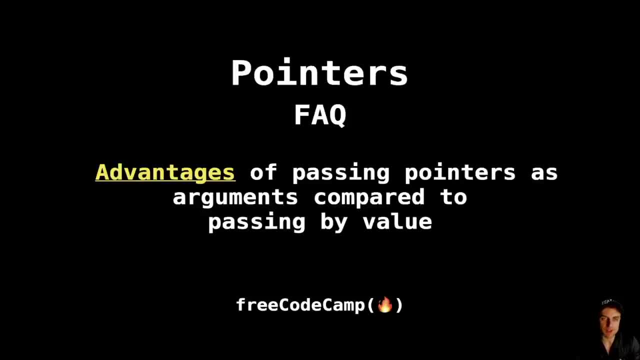 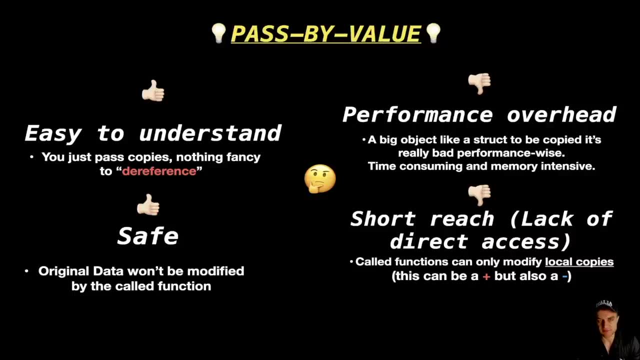 by value. this is a good question, right? let's watch some pros and cons. of course, everything in computer science, like in life, has some pros and cons. so we start by passing by value, of course, passing variable by values. i recall to you that they were just copious. it's easy to understand. 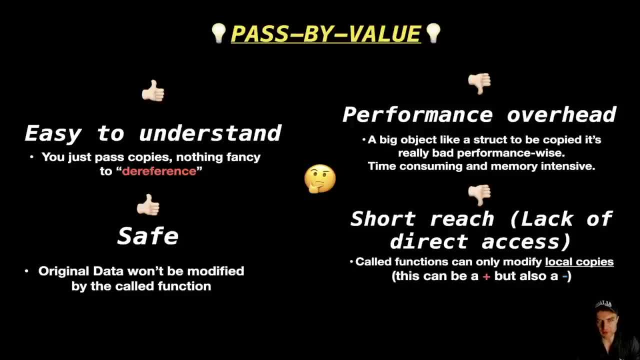 right, it's super easy: you pass a variable and the other function is doing its business to that variable, to that copy, and i have nothing to the reference. super simple. of course, this is safe because passing only copies is going to prevent some other functions to change value somewhere. 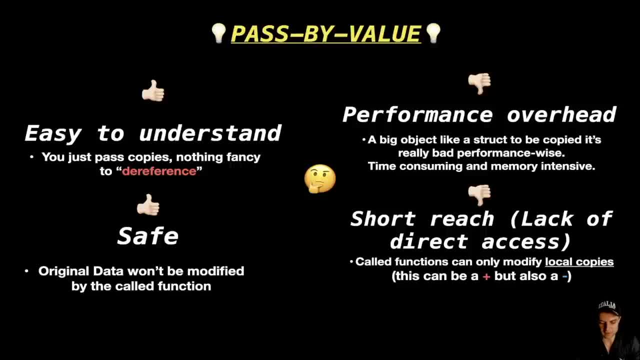 else and making the code overall unreadable. and yeah, you are sure that the cold function is not going to mess up your variables in your local frame. the bad part is that we have some performance overhead. of course, when i pass an object by value, this object has to be copied, so keep in mind if the object is 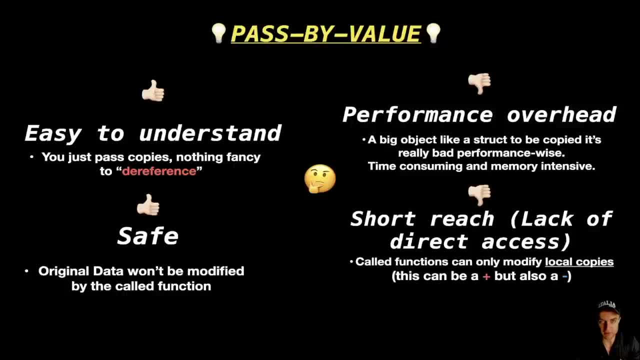 very, very big. you have a very big memory overhead. now we cannot really pass arrays by value. they are not copied because we have a phenomenon which is the array decay into a pointer. i will explain later the relationship between pointers and arrays. but if you have a struct, 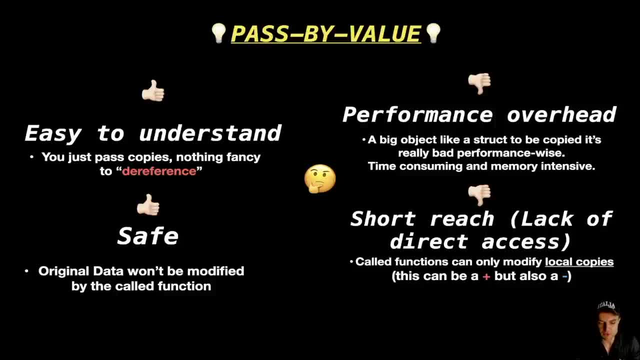 to be copied. so you have every time to every function to copy this big boy. you can very easily understand that this is a big overhead. so another negative part of passing by values is the short reach right. you cannot do what with pointers you can, so this can be good, of course. 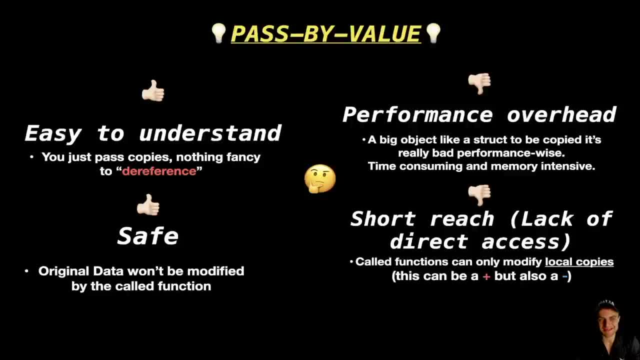 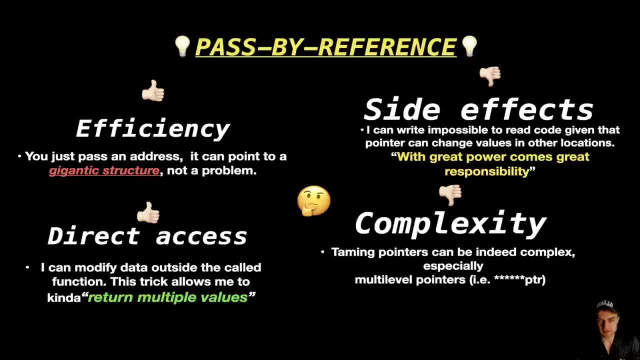 because you have safety, but can be also bad because you're tied to your local frame. so this can be a plus or a minus. passing by reference is, uh, efficient. so you can pass big to data structures, for example, a big struct, and you're gonna pass only a reference. so in the 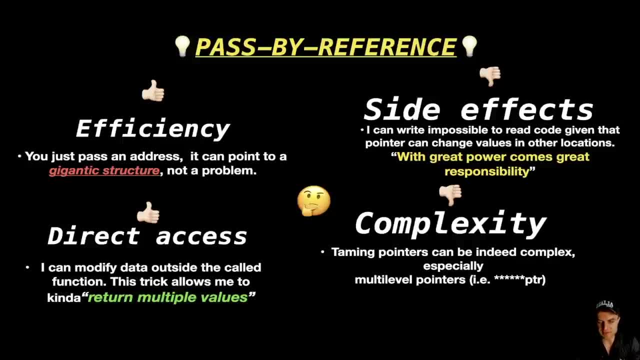 call function. you don't have to copy everything. another plus is that you have direct access to other places in memory. you just saw with the swap function that we can go to change stuff in other places, and this is useful if you know what you're doing. and yeah, this is a way to return. quote unquote. 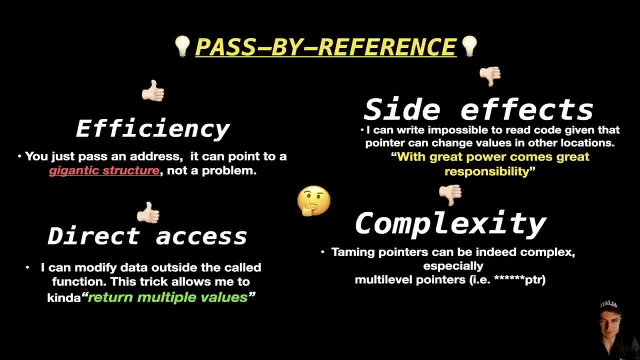 return multiple values, because with the function you're tight to return only one value. right, you have return the value. here you can see that you have a function called return value and you can see that you have a function called return value. here we are able to change stuff in other places. 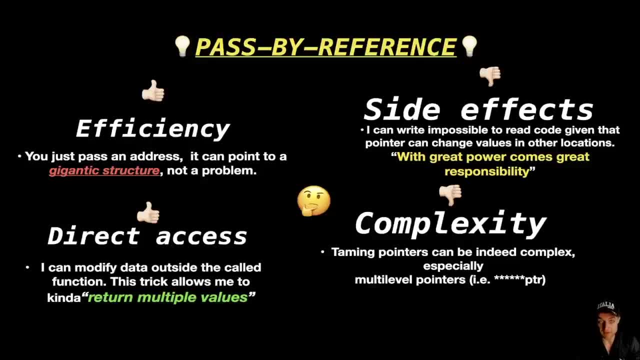 so we can make functions that have a lot of functionality. side effects, of course, is the one i just told you before- is that you can mess up a lot of your code. you can create code which is impossible to read because you have many functions that are changing parts of other code and, overall. 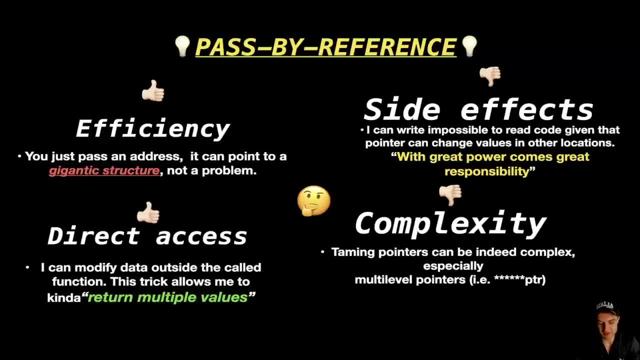 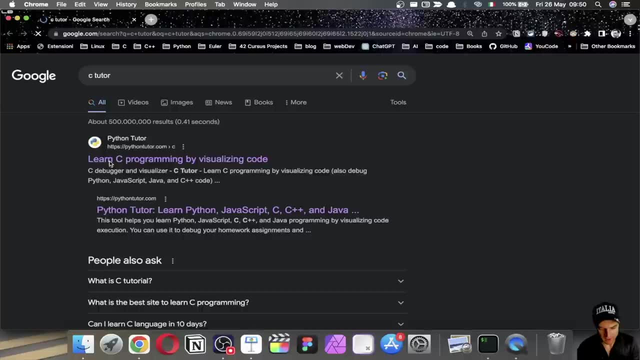 can be a big overhead to have many pointers if you write bad code and, of course, this is complex. taming pointers is indeed very complex and, see, this is one of the most difficult, if not the most difficult, arguments related to c programming. so now, my friend, we are going to a website which is very, very useful. 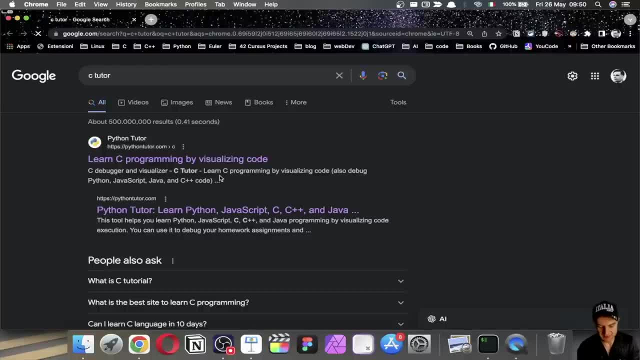 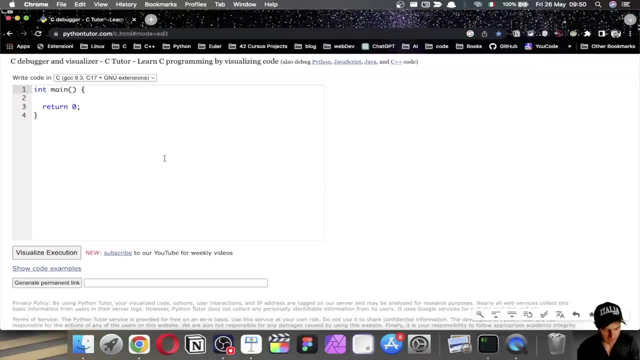 especially if you want to learn pointers, because this is a visual tool that allows you to visualize directly pointer. you just type c tutor on google and you go into this website. then you just pass some code like, for example: here i have this sample code that now we are going to check together, so 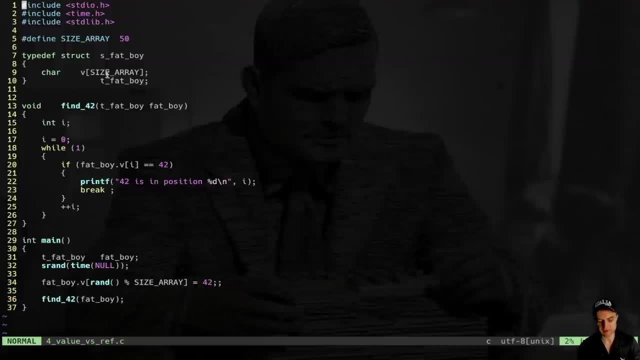 let's watch in the terminal. so we have color. first i have created a little struct which is fat boy. it contains a big array, a big array of 50 elements, so not that big. and here i declare: uh, one instance of objects. right, so i have my fat boy. 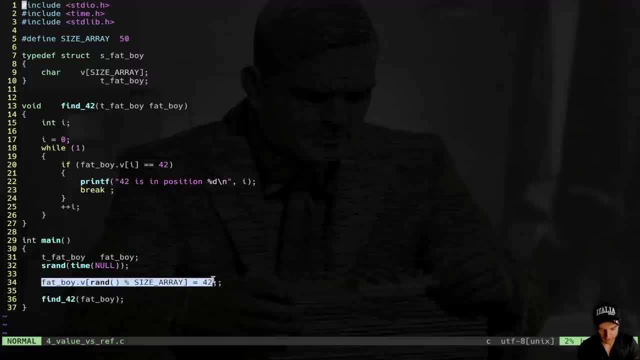 then i just put somewhere randomly in my array the value 42, and then i need just to find this 42 in my fat boy. okay, so i call the function find42, passing as an argument, fat boy. you see, so my, i have my fine 42, that is taking. 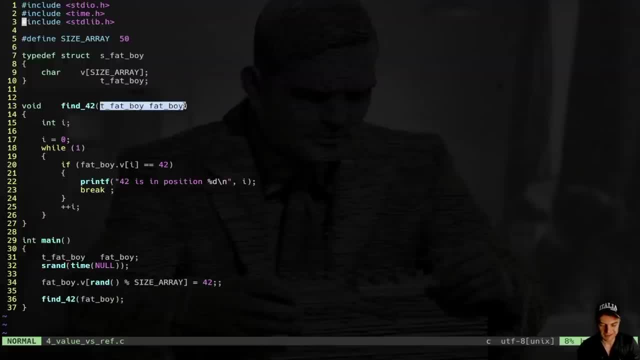 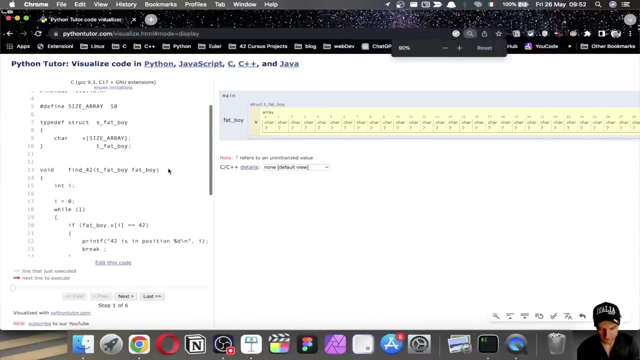 what well he's taking a copy of that boy. you see he's not taking a reference. these are passing by by value and then i have a simple routine that is searching the position of 42. so he's searching where in my fat boy 42 is okay. now let's watch here the execution in ct user. as you can see, i 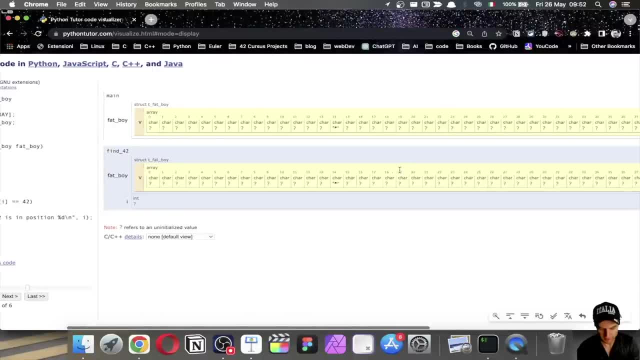 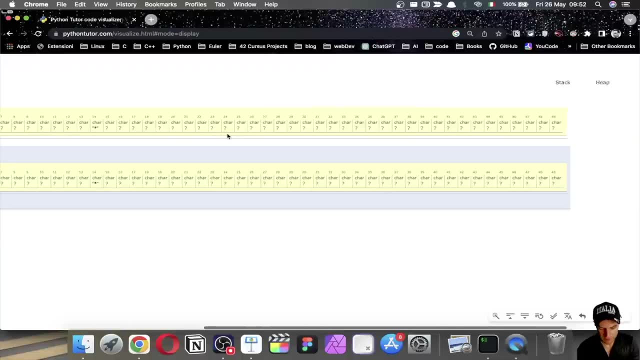 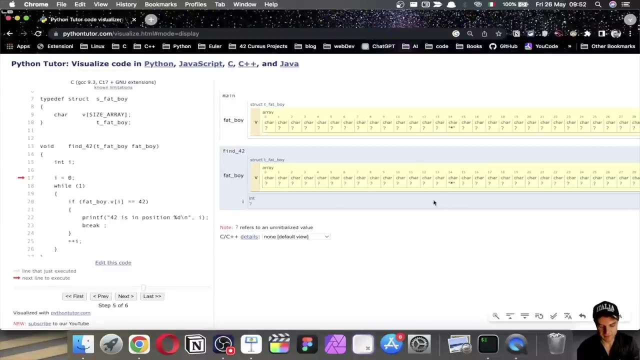 have this big boy here, fat boy. that is a big array. you see a big struct, and when i call find42, i have this. so i need to pass the entire copy and this is bad, right? just keep in mind that you can have many, many functions. this, of course, is going to impair performance, because if you have to copy, 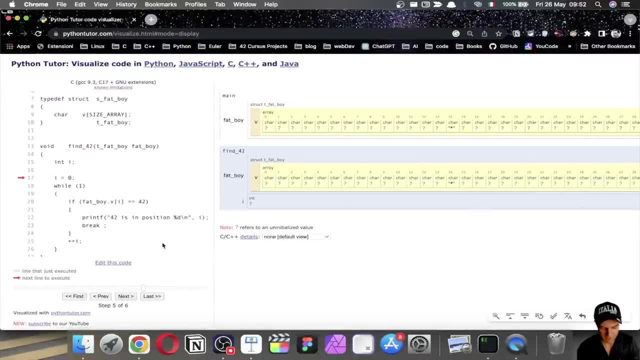 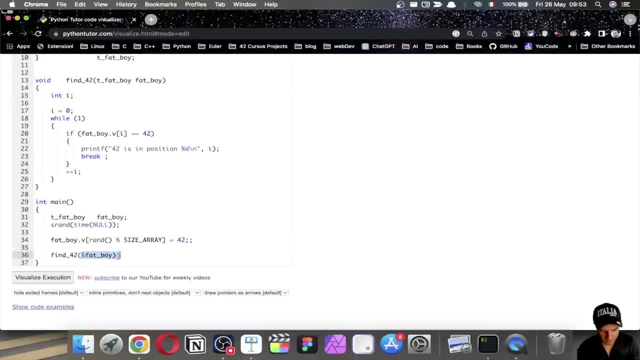 every time all the thing. it's going to take time, even though computers are really fast. now let's tweak a little bit the code. i'm going to change this. so i'm going to use ampersand fit boy here, as you can see. so i give an address to destruct and here in my fine 42 i'm taking a pointer. 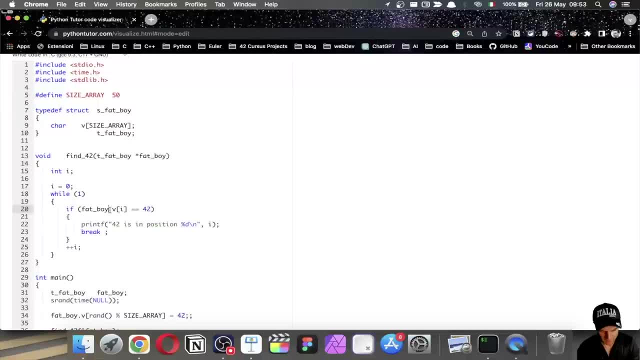 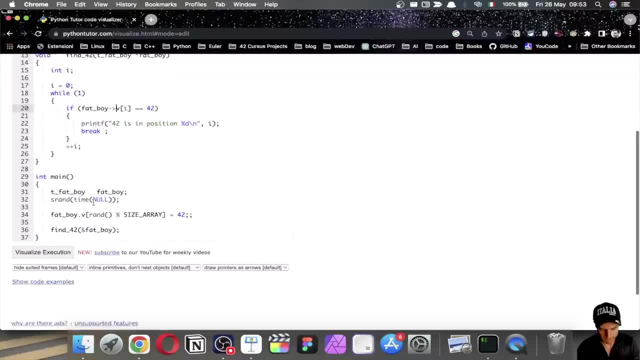 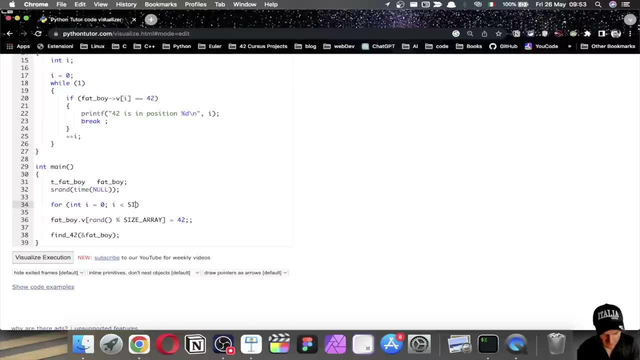 so here now i have to tweak a little bit even near the code. i need to use this special operator. this is for struct, but this is not important now. and here we are. now i just use a loop inside: equals zero i minor. that's dense size array plus plus i. i'm gonna do fat boy v in position i is equal to i. okay, this is just a. 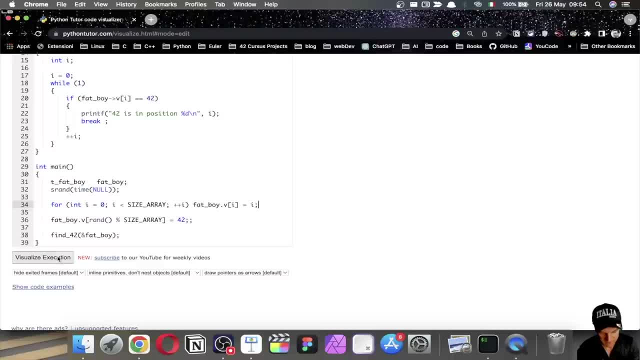 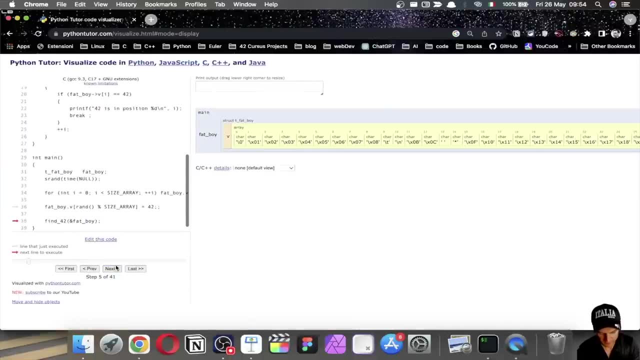 simple uh loop to put some values inside all the cells. so let's run it here. as you can see, i have some random values. then i call the um find42, giving as an input the address, and then i call the function boom. now look carefully, this time you. 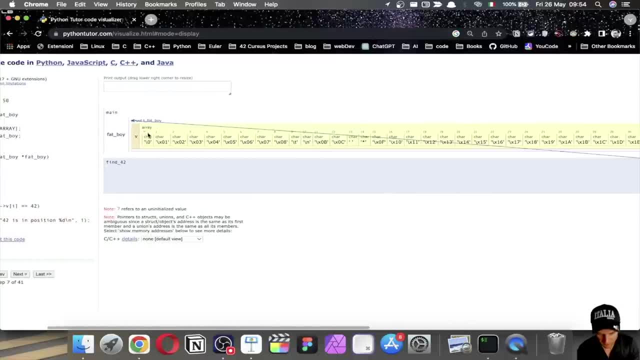 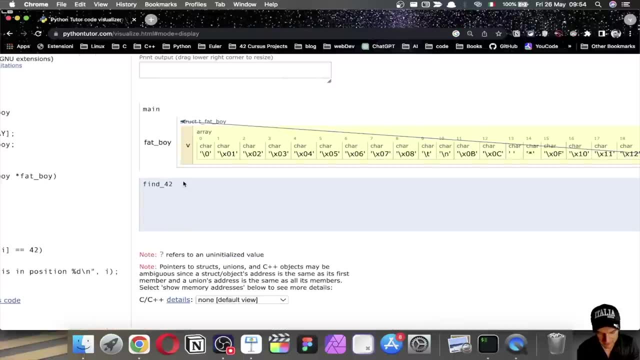 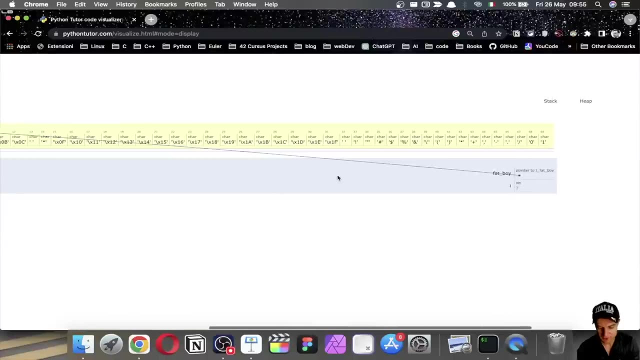 see, i don't have the copy, i just have a pointer. i have a pointer to my big array. so my find42- here my function, doesn't really need to have an entire copy, it just have a reference. so my find42 can be a reference to the main function frame. so it's not in its frame, it's somewhere else, it's in. 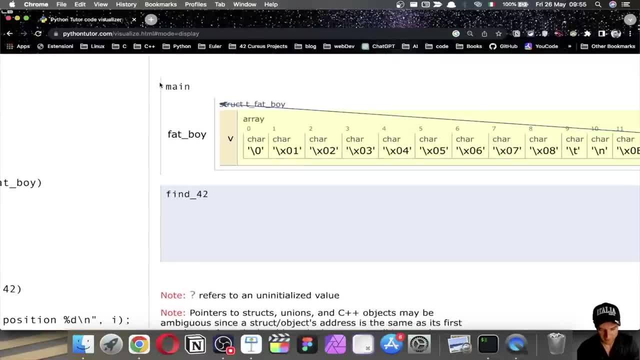 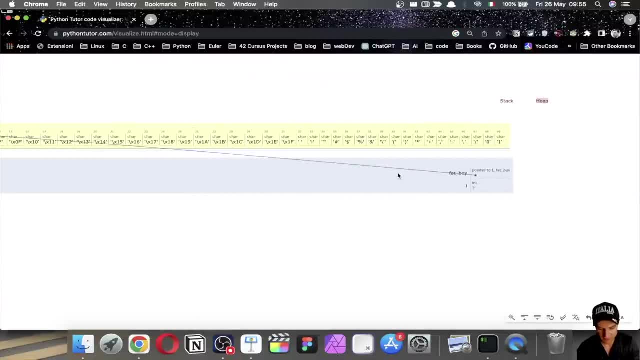 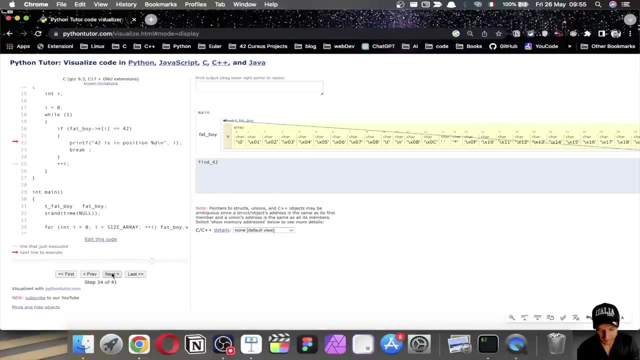 another place. indeed, it's in the main function frame. you see, here with this website, you can clearly see the stack and the and the heap, uh. so here are the functions allocated in the stack. so it's gonna do its algorithm uh in uh, its own frame, looping inside the variable which. 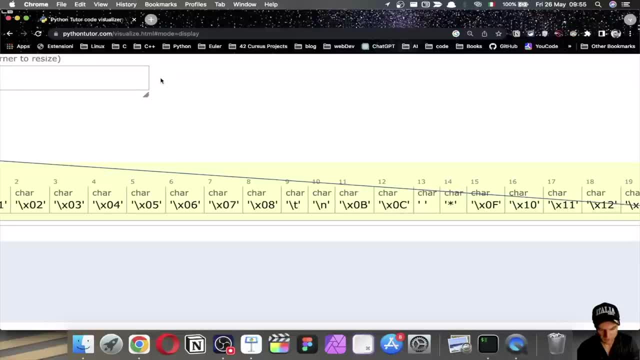 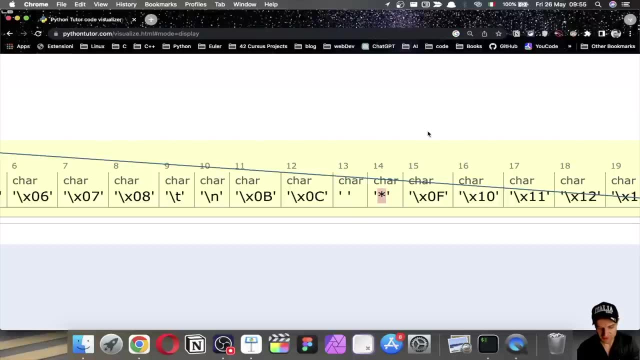 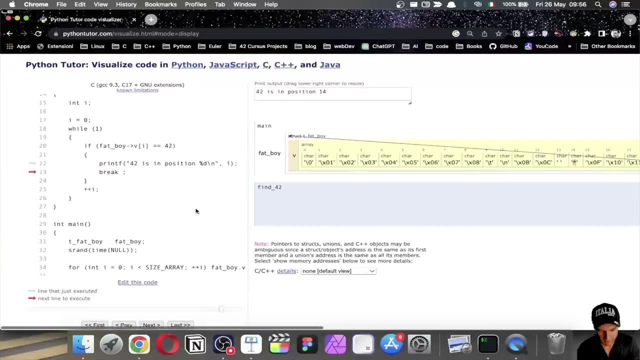 is in the main, a certain point is gonna find 42 in position 14, which is this one. of course, this is um a star, just randomly. 42 is also a star because if you watch the ascii code, you will see that 42 is indeed a star and, my friend, you understood why um passing a value by reference can be. 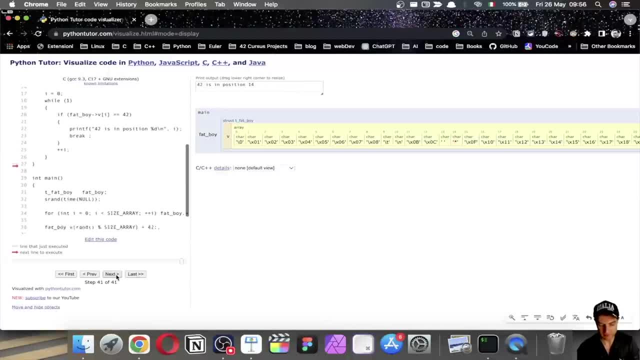 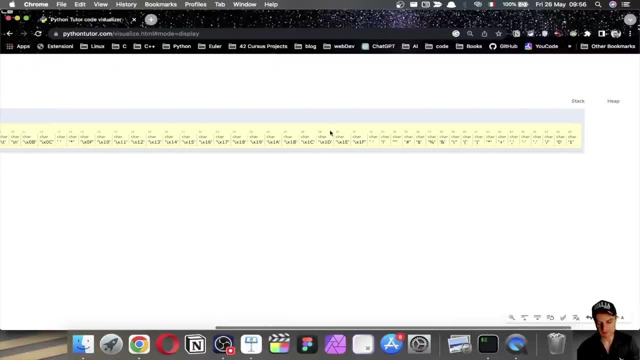 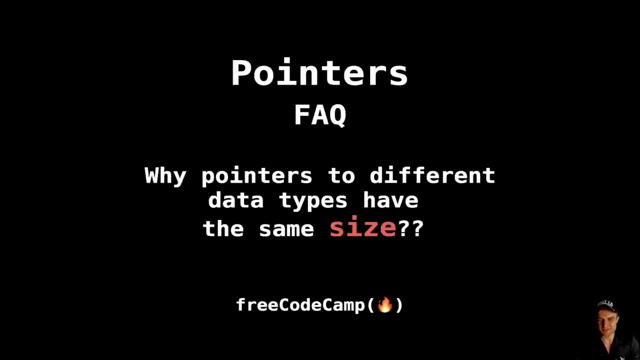 more efficient. well, you don't have to copy all the stuff all the time. okay, these, of course, make more sense once you have big structures, for example, fat boy here, which is a big structure, relatively big question why pointers to different data types have the same size. this is a good question, right? 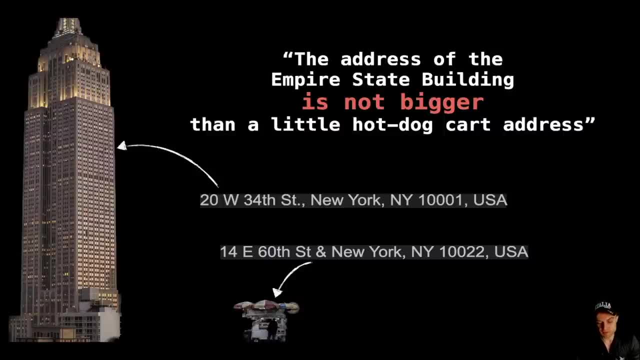 now i'm gonna propose to you a little parallel which is illuminating in my opinion. so if you want to search the address of i don't know the empire state building, or if you want to search the address of a random dude selling hot dogs at central park, you're gonna get a bigger address. if 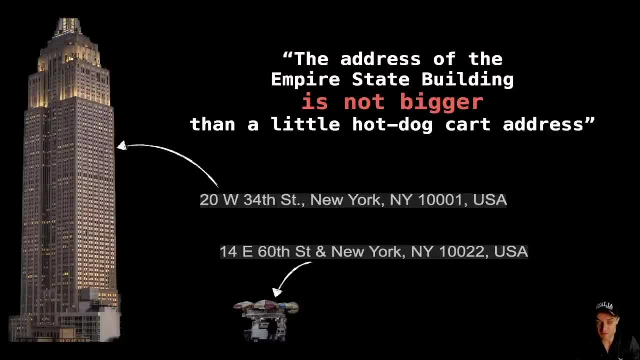 you want to go in the person building, given that this is much, much bigger than the selling hot dog art? well, of course. no, my friend. an address is just an address. this is something that is telling where something is. it doesn't hold that the object pointed by this address is big or not. 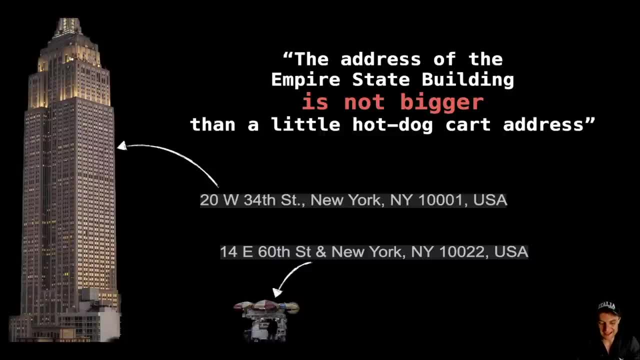 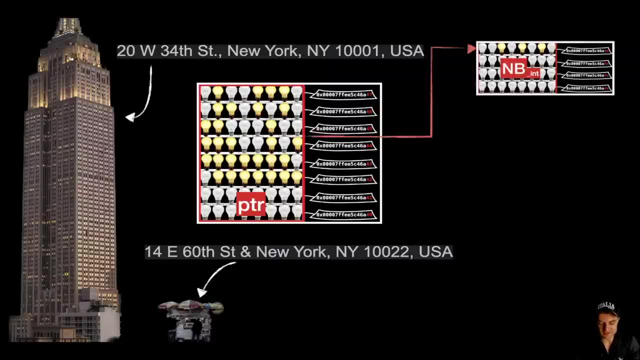 this is not the point of an address. so this is the idea of pointers. if we are pointing something in memory, that can be, for example, an integer for bytes. generally speaking, depending on the system, we have an address of eight bytes in my machine. if we want to point to 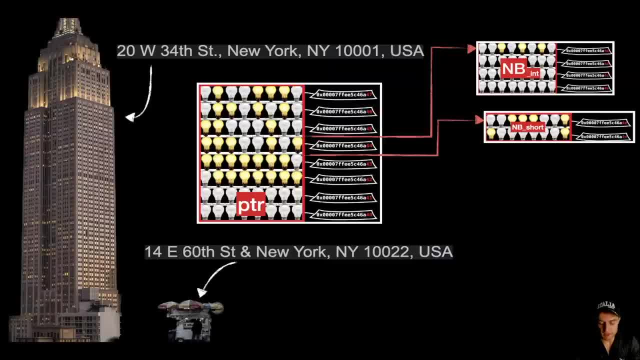 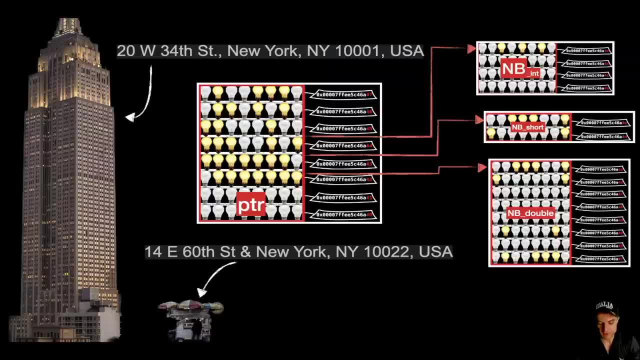 i don't know a short. we still have a pointer of eight bytes. if i want to point to i don't know a double, which is pretty big, uh, it's eight bytes as well in my machine, i still have the same pointer. i still have the same size of my pointer. you get the point, because all the data have an address. 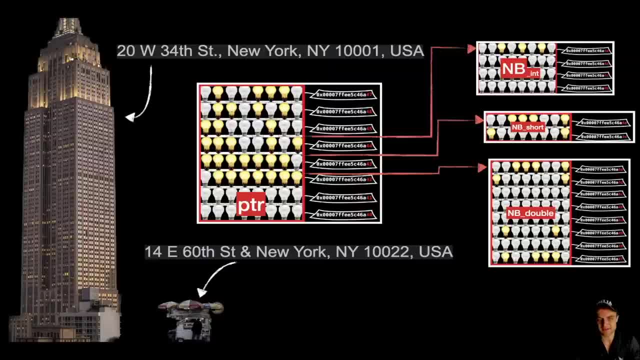 which is of a specific size. so keep in mind this parallel that i made with the empires that building and the selling old dog dude cars. let's start the video, let's go ahead and go ahead, and same idea. okay, that's the same principle. so here, my friend, i have a little program that is showing. 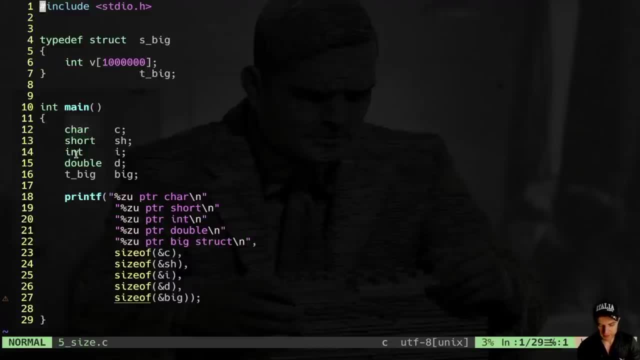 you this: i have a char, a short, an int, a double, and then i have a type, big, which is just a struct that contains a big array. here i have three, six, one million um integers, so i have, uh, four megabytes, okay, and here i simply print the size. of this is an operator that is giving me back on any bytes. 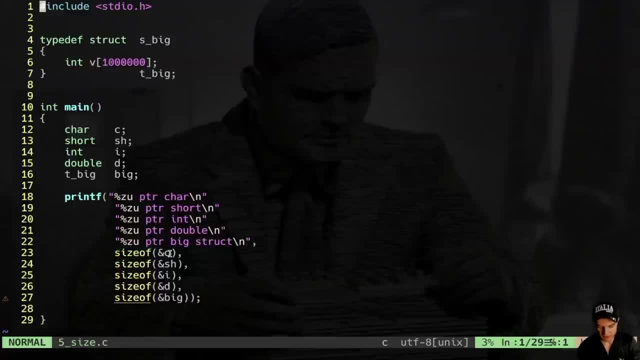 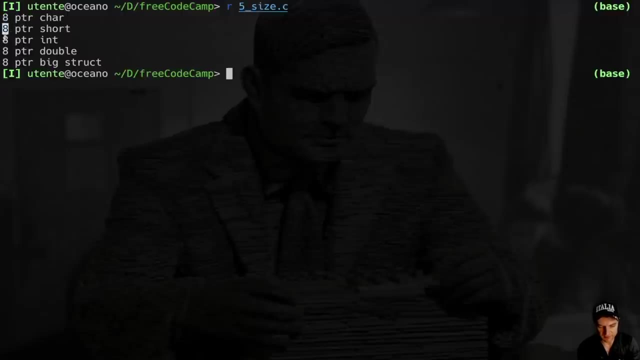 something is big of the address of uh, c, of ch, of i, d and big so the address, while pointers do these objects here. all right, let's try to launch this code. i have eight, which is the size of the pointer, to every data type, to a chart, which is the smallest, to big struct, which is the biggest i have. 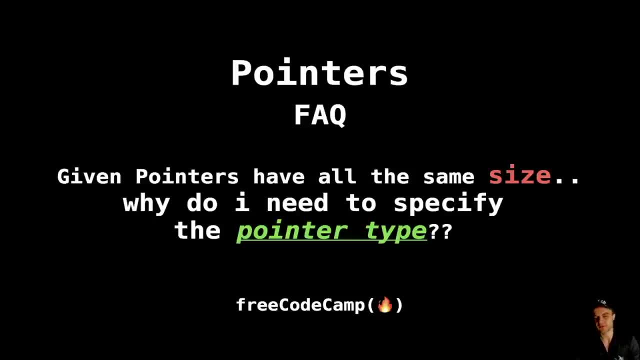 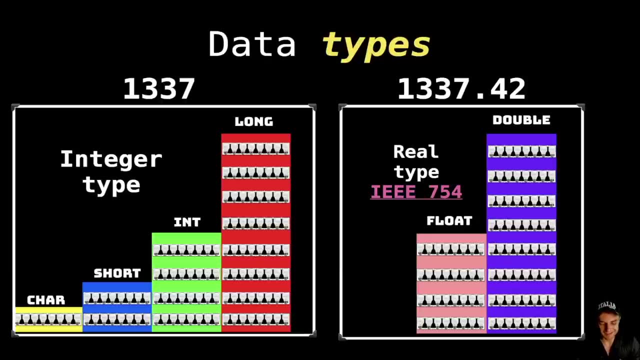 all the times eight. now another question: given pointers have all the same size- we just saw that- why do i need to specify the your type? this is another good question, right? indeed, when i declare a variable, i'm telling the compiler: hey dude, i want, uh, an integer. so give me in my machine four bytes, or i want long, give me. 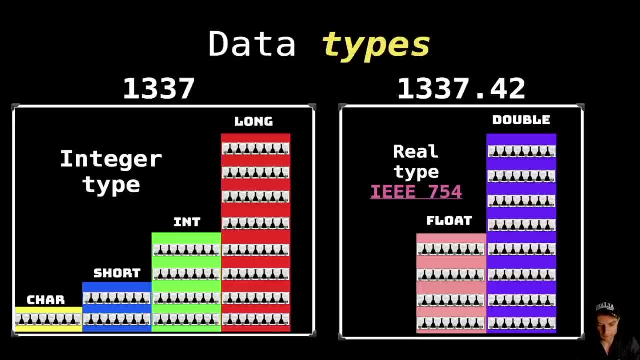 eight bytes or i want to charge, give me one byte. they are all integers. at the end of the day they are stocked in memory as an integer. so here i'm just saying, hey, i want eight bytes, or i want one byte of the integer type. i can do the same line of reasoning with floats, but you got the point right. 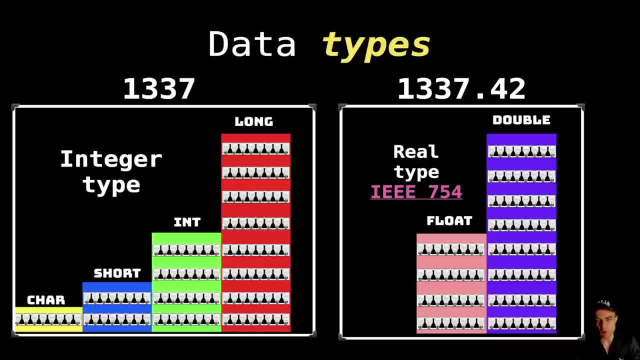 so the type is, uh, telling us even how big an object is. of course, this is a simplification. at the end of the day, is the compiler that is deciding how big an object has to be. but anyway, just linger on the principle: you decide the data type depending on the size. for example, if i want a very little number, that 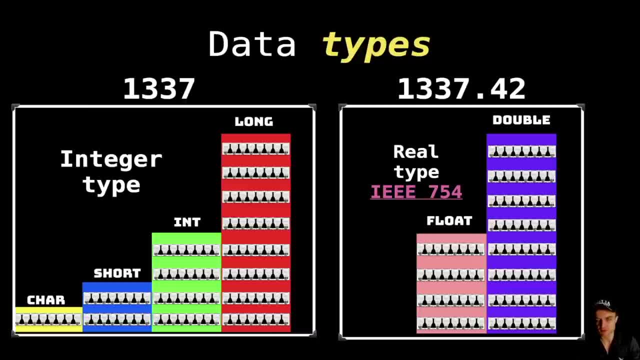 is ranging from, i don't know, from 0 to 100, i can use a chart. i can use a chart as a one byte integer, not only for charts. this is an integer of one byte so i can really use it for a little number if i want to use. so i can very surgically with data types decide: uh, how much memory i want. 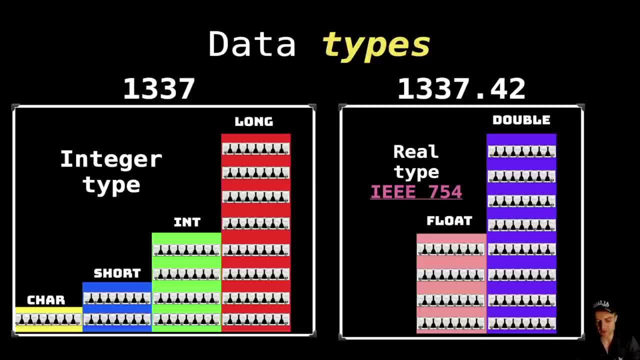 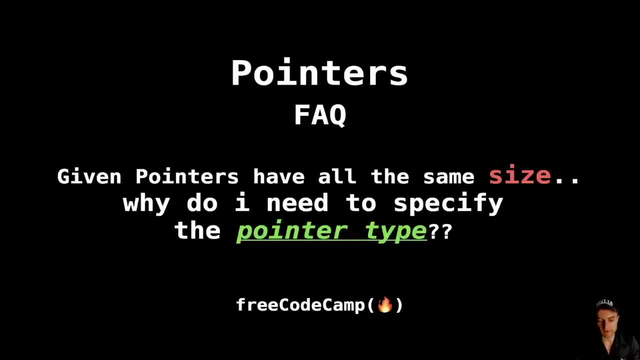 to use. this is pretty useful, right when you want to have a super control of what is going on. indeed, the c programming language is giving you super powers in this domain. on the contrary, you have pointers that have all the same size. so what is the point of telling me: okay, this is a pointer. 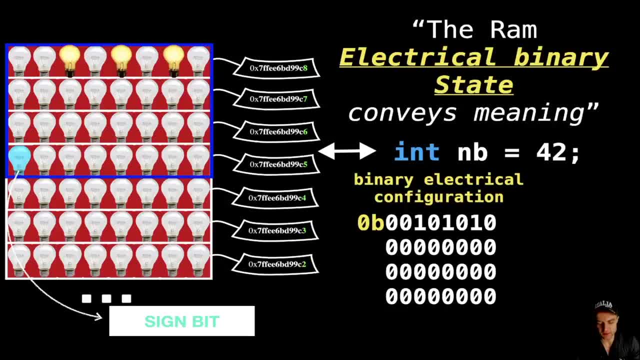 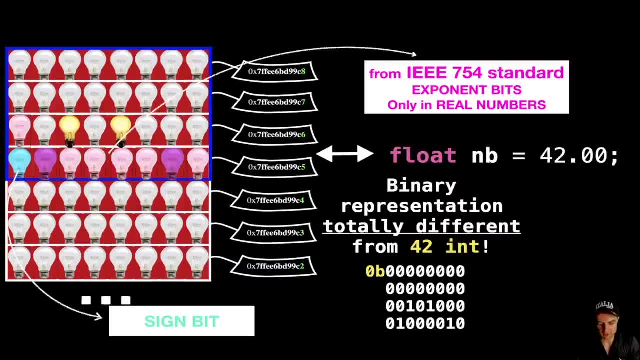 to an integer rather than a pointer to a chart. so here i want to repeat to you again: this point that i want to make clear is that the configuration of 42 is very, very different from the binary configuration of 42.0, float right, because we have a different encoding of the binary. we have 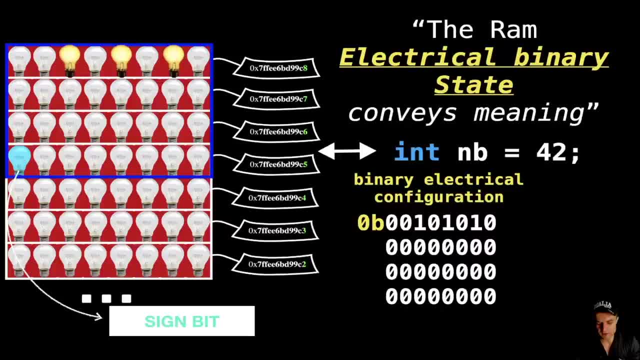 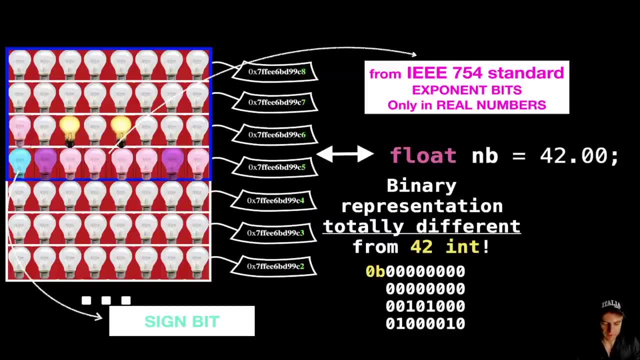 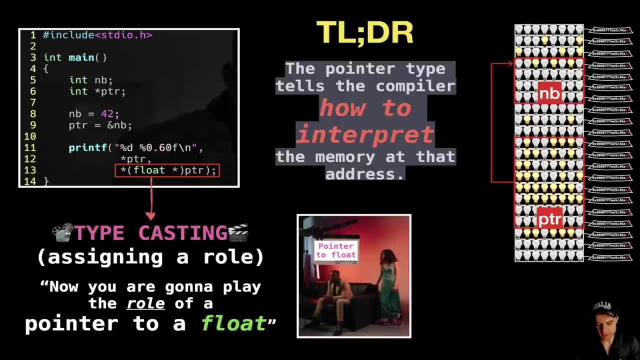 exponents, bits, uh, in the real data types, on the contrary, on the integer data type, we don't have this kind of accounting. we have simply the number in a choose- complement fashion. so keep in mind this, because we're gonna do a little trick related to this idea. so now i have a little program. 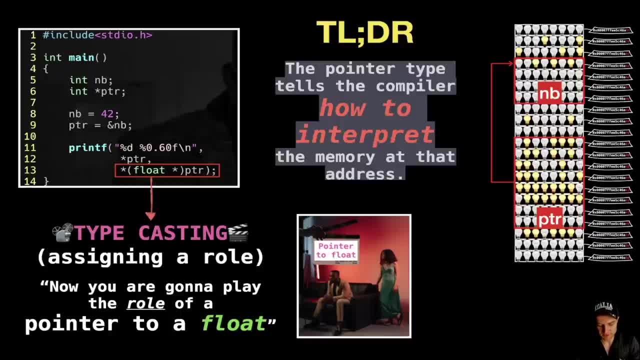 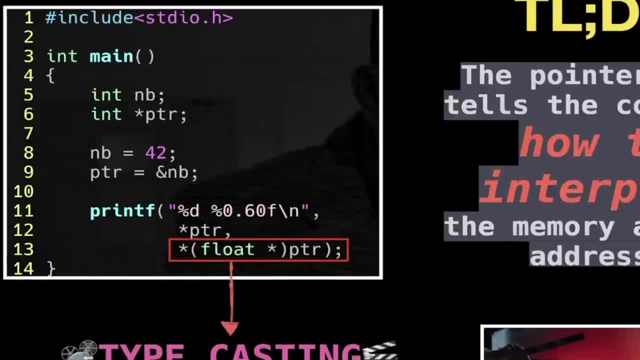 that we're gonna check to understand why a pointer has a specific type. i have a declaration of a variable which is an integer- int and b- and then i have a declaration of a pointer. you can see int, star, ptr. this means that if you the reference ptr, you get an integer and b gets the value 42. 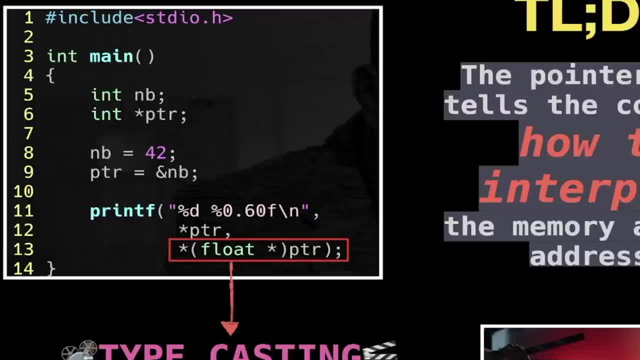 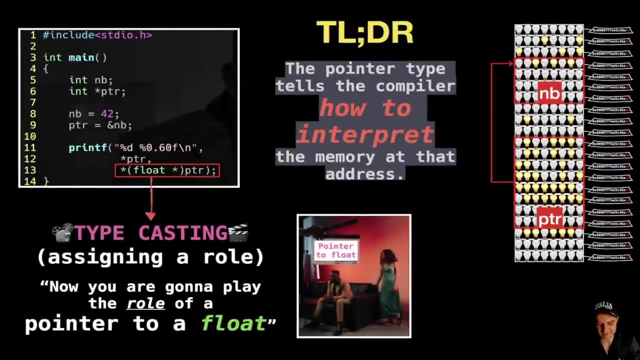 and ptr gets the address of nb, then i call my printf, so i want to print the, the value pointed by ptr, and then i do something peculiar, which is this casting: okay, i'm gonna cast ptr to a float star float pointer. what is this casting thing? well, the best analogy that came to my mind is: 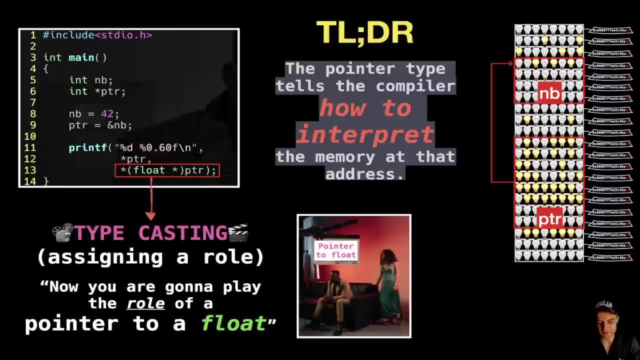 like the real casting when we want to decide which actors have to play in, uh, in our film, right, well, that's basically the same idea. when we do a cast, we are assigning a role to a pointer in this case. so we are assigning the role of a pointer to a float to my pointer. so here i'm. 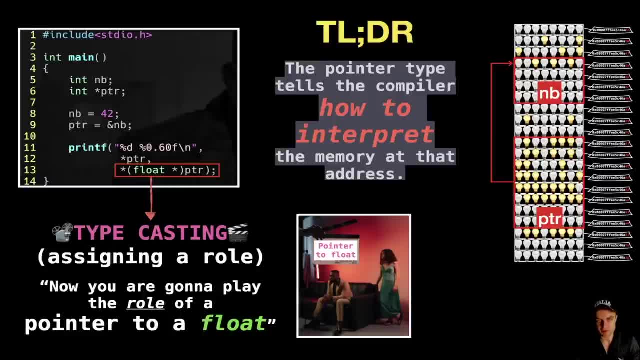 telling to ptr: hey, dude, i know that you are a pointer to an integer, but you're not going to. but in this time you're going to play the role of a pointer to a float. so we're going to do another chuck and we're going to reference again the pointer, but this time of a type float. so here, 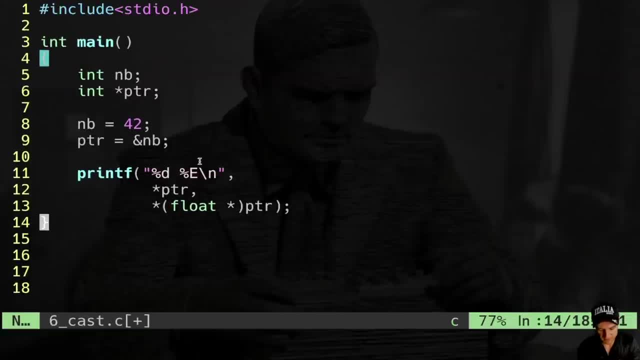 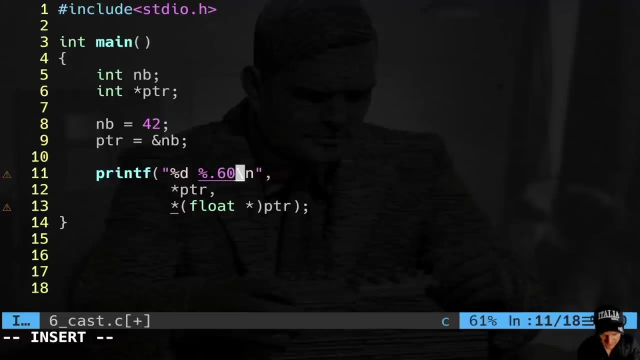 you come. my friend, this is the actual program. as you can see, i have the thing you just saw in the slide. the only thing is that here i have an e because i want to see in scientific notation, otherwise the number is going to be too little. but we can also do like that: um 0.60 f. 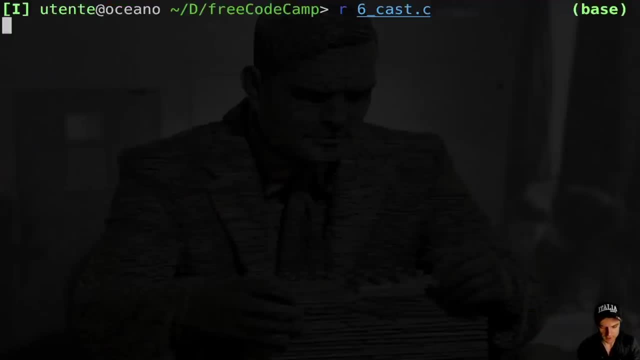 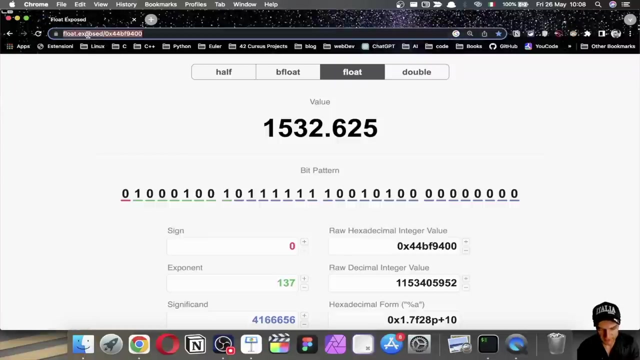 okay, let's try to launch the program. so i'm gonna launch. look what happens. i have these 42, and then i have this zero, zero, zero, zero, and then i have this value. what is that value, my friend? so you just go on this website, which is uh float exposed, in which you can uh play with floating numbers. 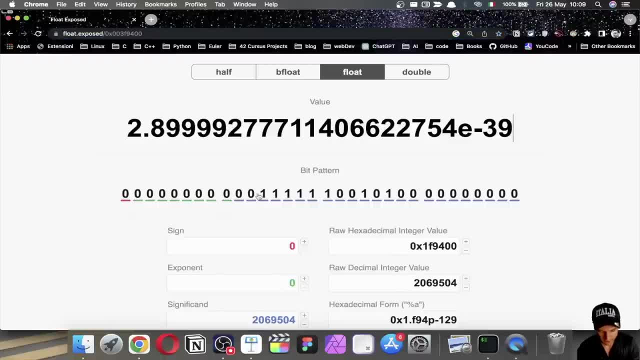 so now let's try to do something. i write 42 here, in binary of course, which is 1, 0, 1 0, 1 0. of course, you can buy it, which is this one. so i have one zero, one zero, one zero. do you see something that? 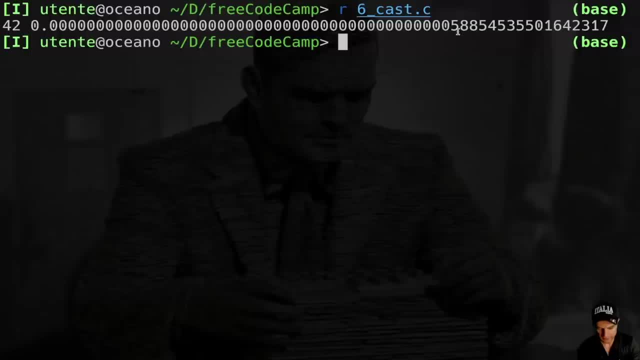 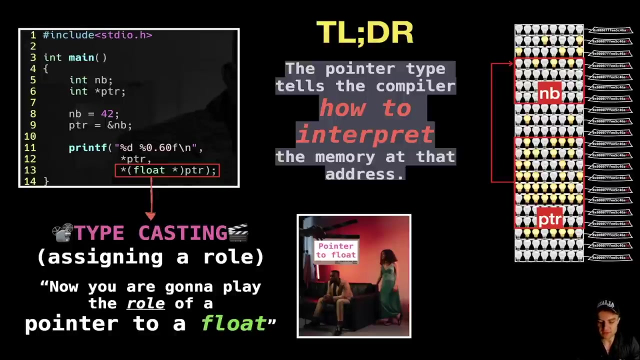 you just saw five, eight, eight, five, four. what do you see here? five, eight, eight, five, four, five, three, five, five, zero. five, three, five, five, zero. hmm, so you see what's happening here. my friend, here with this cast, i'm telling a pointer: when you're gonna be the reference, read those binaries as a float. 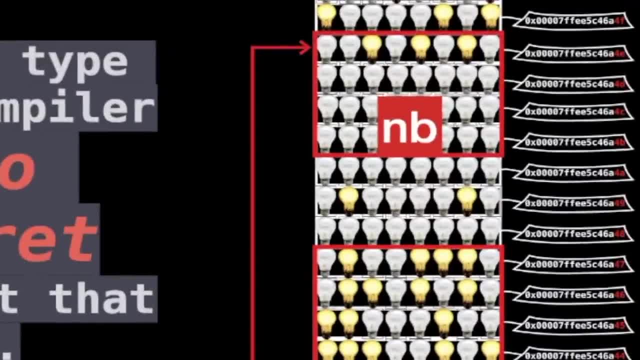 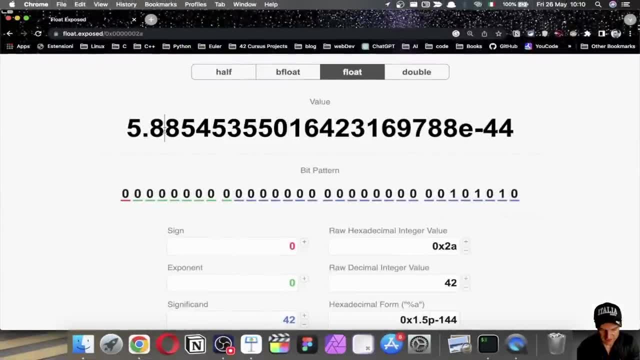 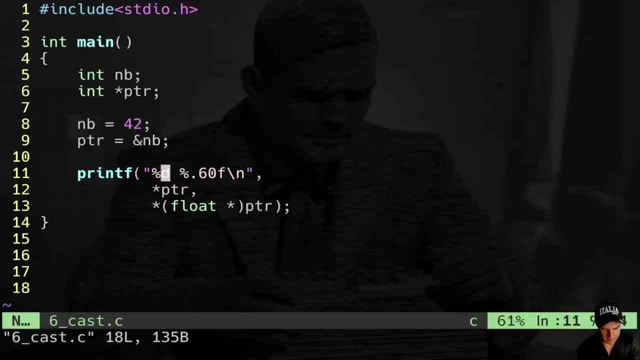 not anymore as an integer, so you're pointing to a float now. you see, so that one zero, one zero, one zero is the referenced. in this fashion, it doesn't see any more 42, but it sees this very little number, which is this five elevated to minus 44.. here we can do in scientific notation: 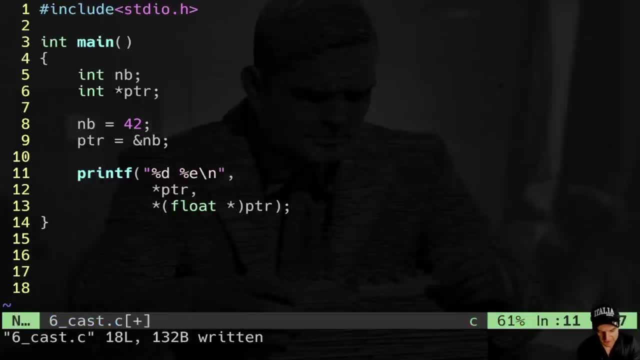 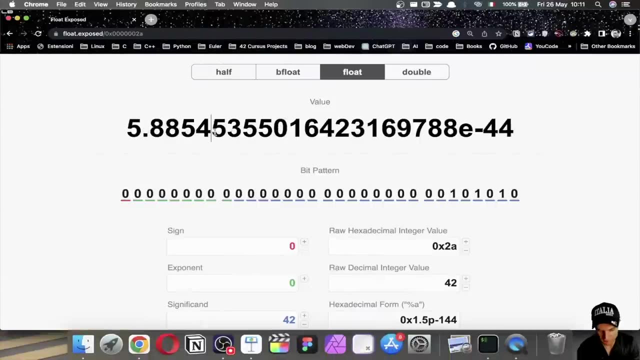 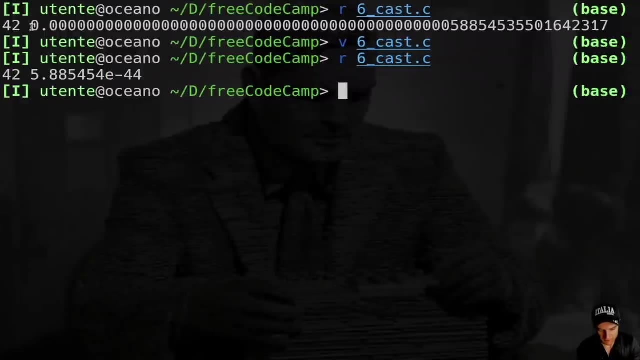 essentially like i did before. like that and you will see the exact same value. just you don't see all these zeros right. five, eight, eight, five, four, five, four. of course, here you see a four because we have um, the value rounded and then elevated to minus 44. you, that's why you have all these zeros here. but anyway, you get the point, the pointer type. 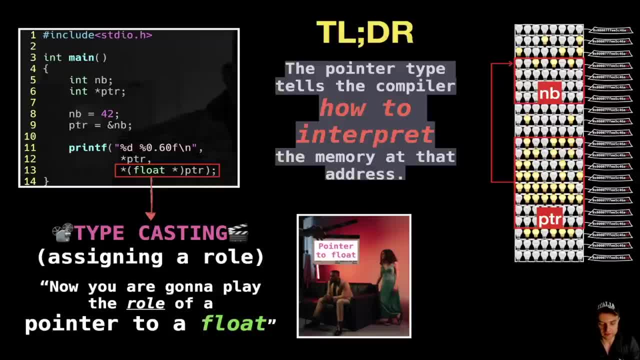 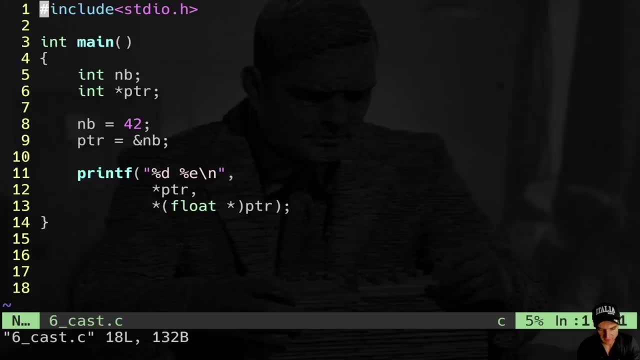 tells the compiler how to interpret the binary, the spotting memory that is pointing to. so that's why we have a data type for a pointer. this is crucial all the times you want to get a specific value. let's play a little bit with this code so we can have a super good understanding of what is going. 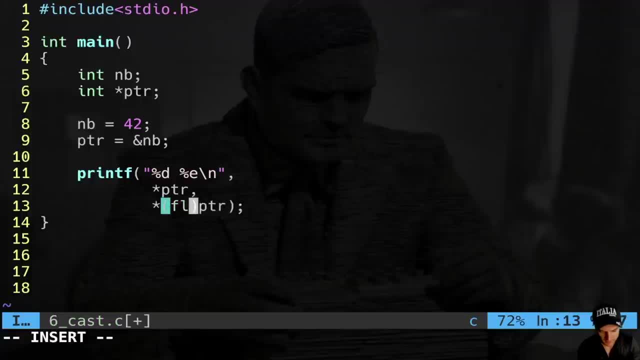 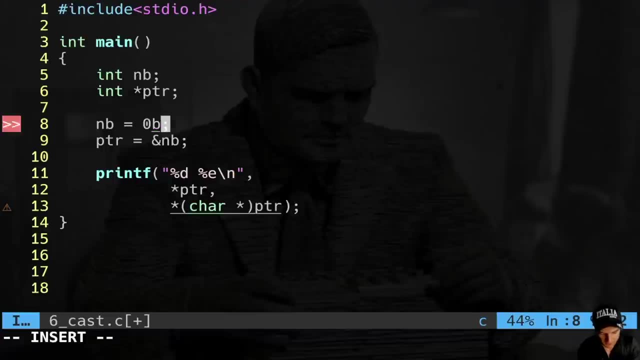 on. this time i'm gonna do um a charm, for example, i'm gonna cast to a chart and um, um, here i'm gonna write directly in binary: we do, we can do that in c. we do one and eight zeros. one, two, three, four, five, six, seven, eight, and here i write c. what is going to happen in your opinion? 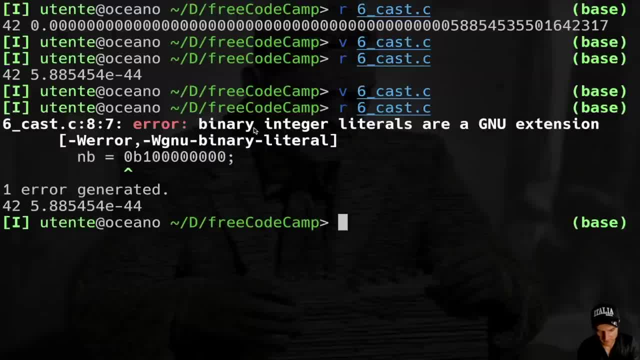 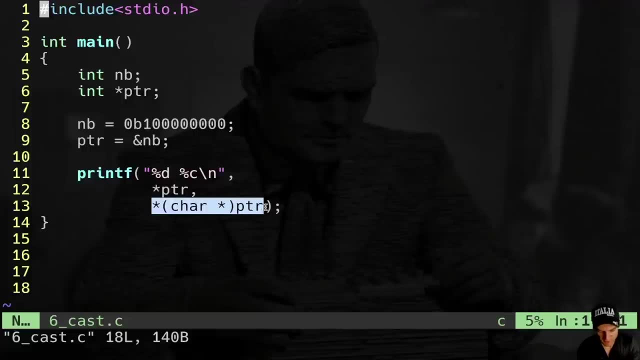 let's close, let's run, okay. uh, i cannot do, because this is binary search, but i can. these are just controls, flags that i put. okay, i launch, i get the value 256, but i don't see any char. why is that? well, when i do reference this pointer, what i'm gonna see is only the least significant byte. 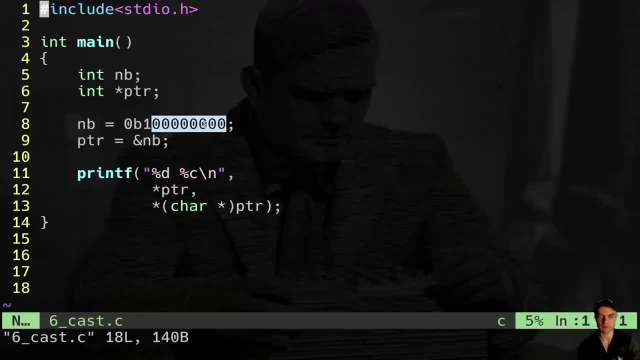 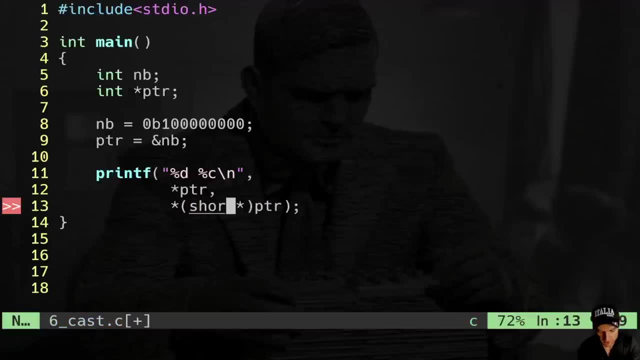 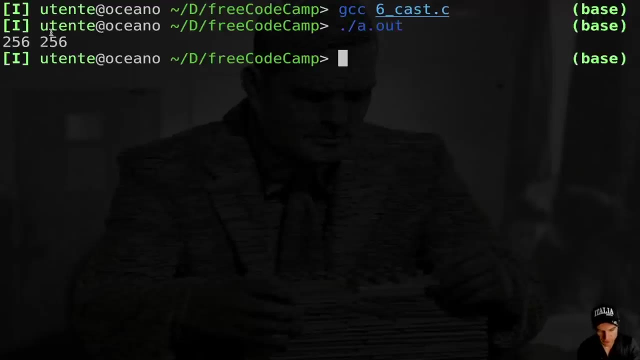 a charge is one byte, right. so when i reference, i get the zero, the null char. so that's why i don't see anything here. if it was i don't know- a short, i short uh, and here i just put uh, d, so you are gonna see 256 as well, because when i do reference this pointer, this is gonna see uh, these second byte. 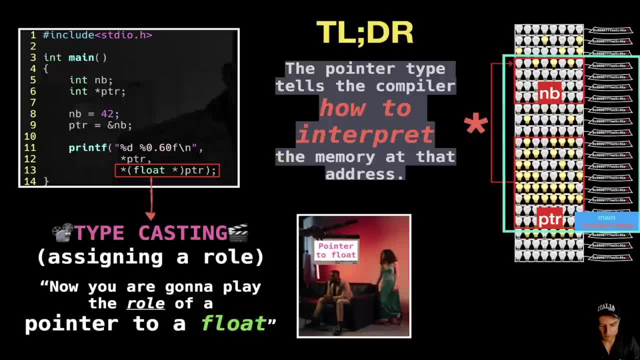 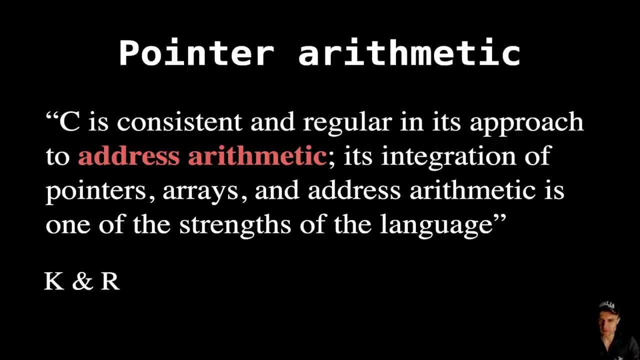 want because a short is two bytes. depending on the data type, we are gonna read the bytes pointed by the pointer differently. this is not the full story of the data type of pointers. indeed, we have c that is very consistent and regular in its approach to address arithmetic, its integration. 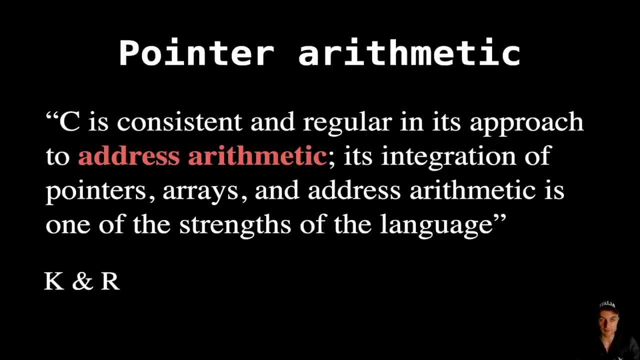 of pointers, arrays and address. arithmetic is one of the strengths of the language. you will see later that there is a big integration related to arrays and pointers, making it really tricky to differentiate between arrays and pointers. you will see, but keep in mind that ears is written. we want pointer arithmetic to be equal to index addressing of arrays, so let's make a stupid. 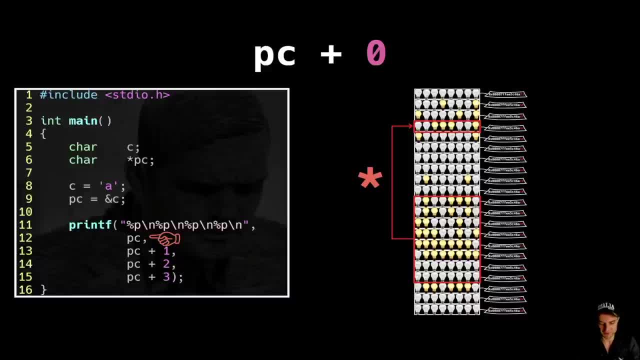 example, don't pay attention to the binary configuration of the ram. this is just random. i want just to make a point here about pointer arithmetic. so i have my pointer pointing to a char, a pointer to char, and then i'm going to print every time the value of this pointer, mainly the address. 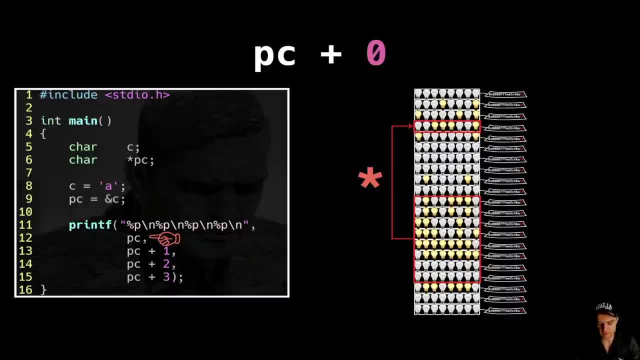 doing some arithmetic, as you can see. initially i want to print pc pointer to char its value, so i'm going to print that. then i'm going to do pc plus one boom. so, as you can see, i advanced the pointer by one. now the pointer is pointing one position more. then i do. 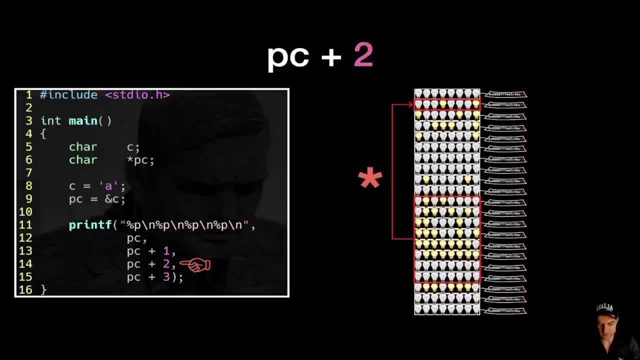 pointer c plus two. so i advance another position. and then pointer c plus three, i advance another position. now we say, well, that's easy, right, i have the pointer. that is indeed advancing one position. but this is just the case. the case is that a char is big one byte, so that's why we are advancing one byte at. 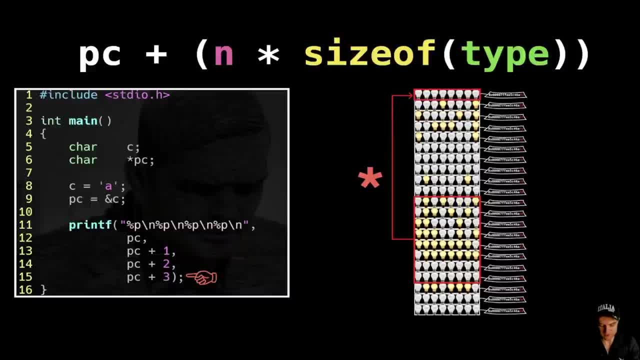 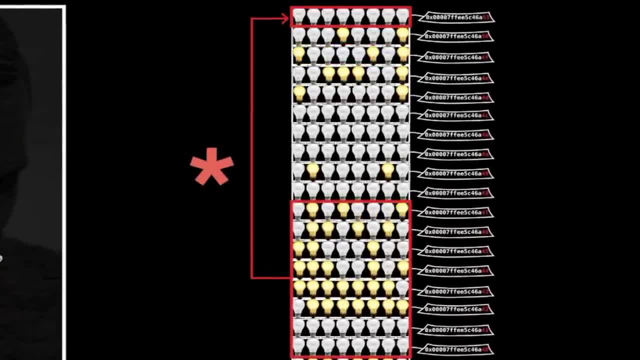 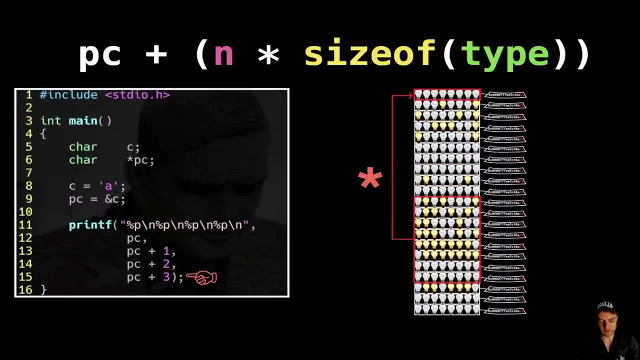 the time. i want you to pay attention to the fact that a pointer is just a variable. as you can see, the binary configuration of the pointer is changing, as i do pointer arithmetic, because this is just a value that can change. okay, so the formula to make pointer arithmetic is this one. i am 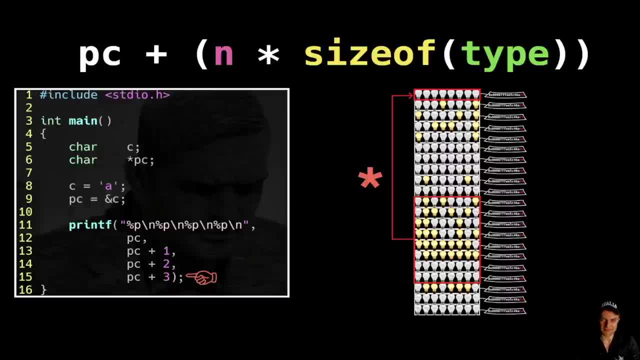 going to change the value. so i have the pointer plus and per size of type pointed. so that's why it's important to know the type of the object pointed. this time i have a chart, so it's easy, and let's say: is three, the size of char is one, so i have the address plus three. okay, now let's watch. 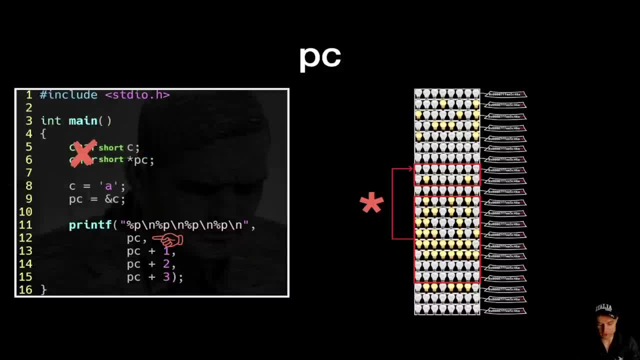 another case. this time i'm pointing to another data type, which is a short, for example. we're gonna change a little bit the code, we're gonna change the value, and now what is going to happen this time when i add one to pc? so look carefully, i have this boom, i have the advancement of two bytes and not only one. why? 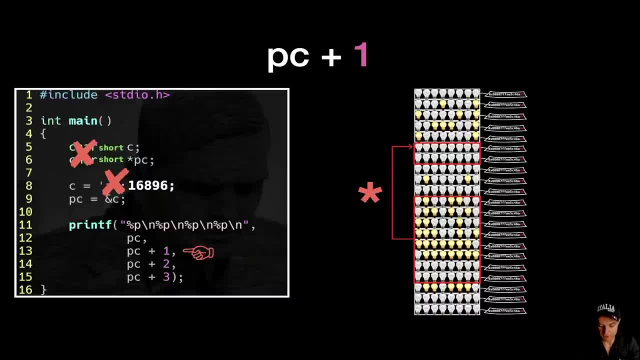 is that well you understood, because a short is two bytes. so when i say pc plus two, i get boom, an advancement of other two bytes, so four bytes respective to pc. so that's what is going on, my friend. you understand super well that the data type is important, also when we do pointer arithmetic. 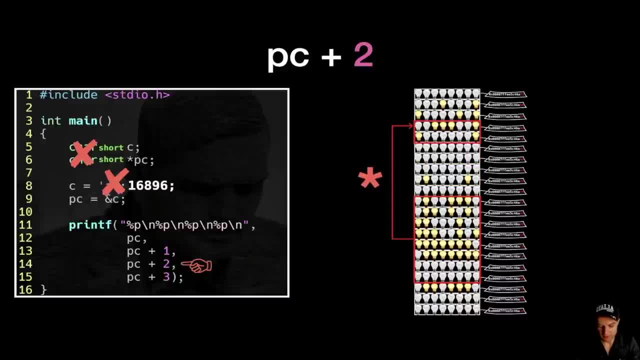 you see. so this is gonna discipline, it's going to work, and you will see that this maintains a highly consistent parallel between pointer arithmetic and array indexes. indeed, it's like i'm taking the object at position x. so this is just a code that you saw. we are going to start, for example, with an integer. 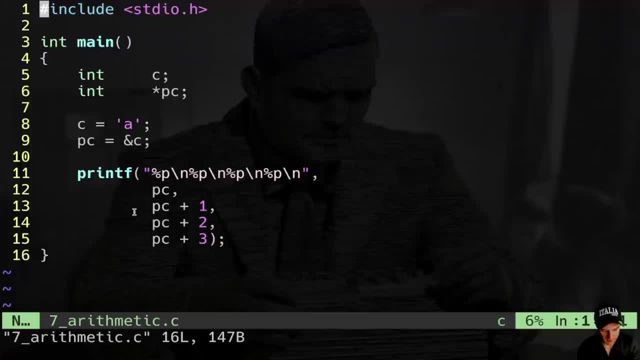 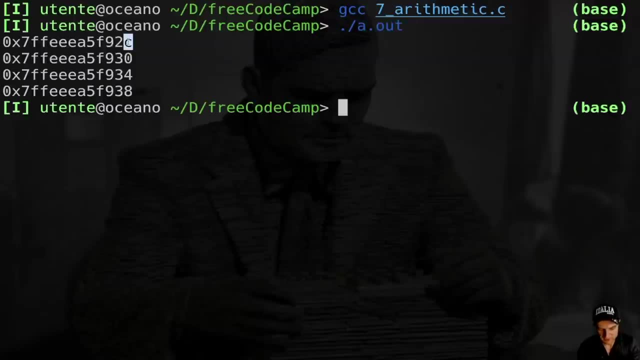 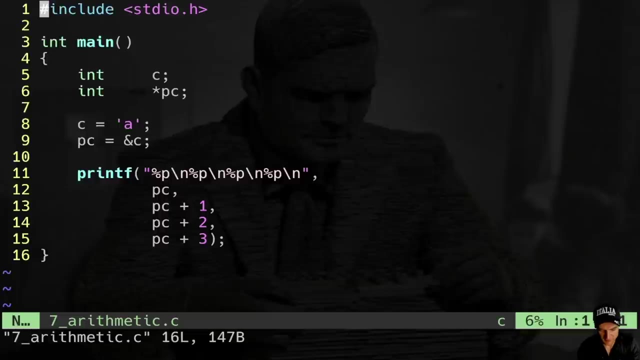 this time i have a pointer to an integer and we're going to perform arithmetic with an integer pointer. i'm going to compile and then launch. as you can see, we have an advancement of of what? of four right zero four eight. okay, why is that? well, you understand so very well. now, 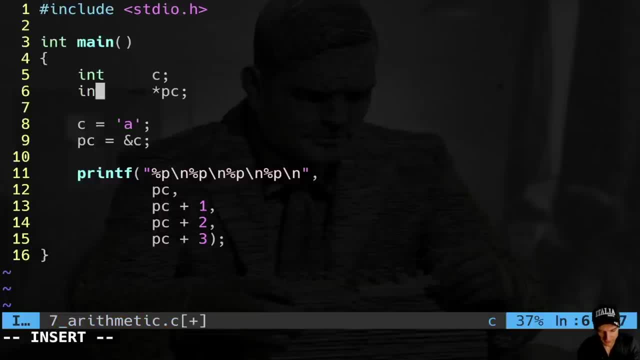 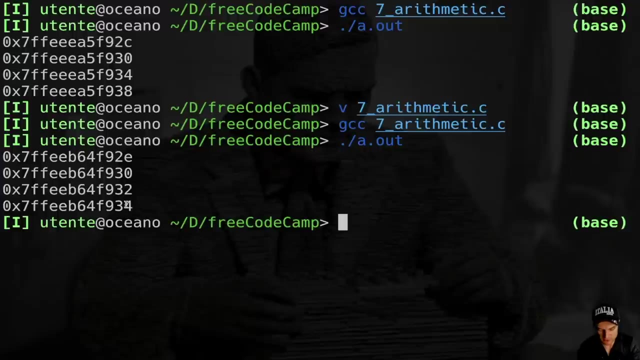 because an integer is uh for byte entity. if you do your uh short, like uh in the slide, so we change here to short, what is going to happen? well, you already know. i'm gonna launch. i have an advancement which is from two to two zero two and four. that's all. there is my friend. other question: void pointers. 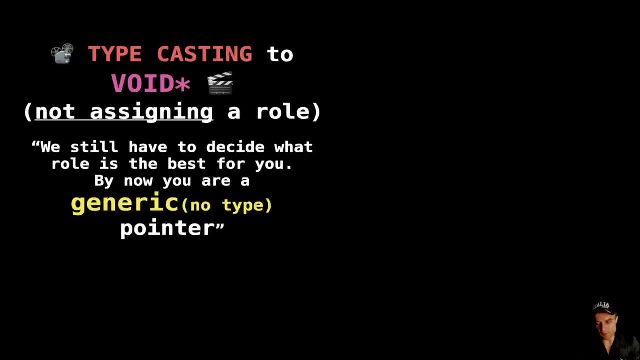 confusing. hmm, let's dig a little bit. when i say that a pointer is a void pointer, what i'm really saying? well, i'm not assigning, if you want, a role to my pointer. i still don't know which is the best fit for this specific pointer, so we can say that void is a generic pointer. you should definitely. 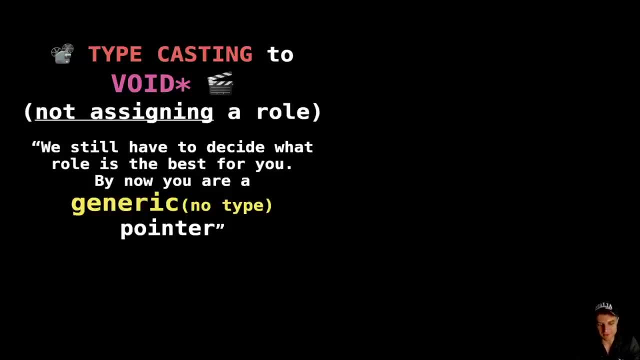 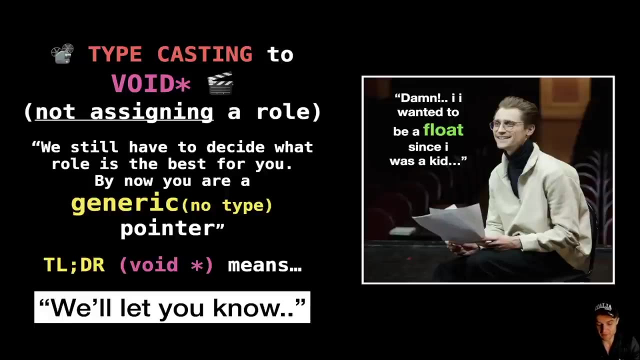 change the word void to generic in your mind when you see void. just keep in mind that this is a generic pointer. so tldr, void, star. void pointer means we will let you know. right, that's what happens with actors when we don't know which is the best role for them. you can keep this. 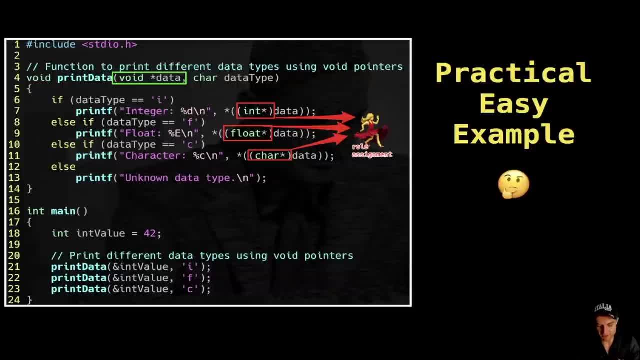 parallel in your mind. it's pretty useful. now let's see a practical example here. i have a stupid program that is going to declare in its main a value, the usual value 42, and then i have a function that is called, which is print data. so this function is able to print that specific data. 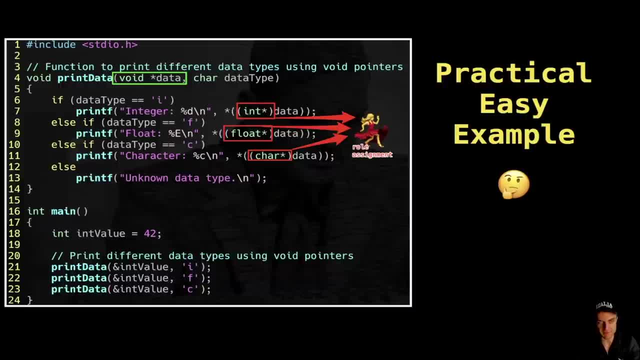 given a specific chart, for example i, f or c for integer fraud, or char. the print data function is taking as an input a void star data. so we have a generic data that we're going to interpret inside the function. so if we have the char i, we're going to interpret the data as an. 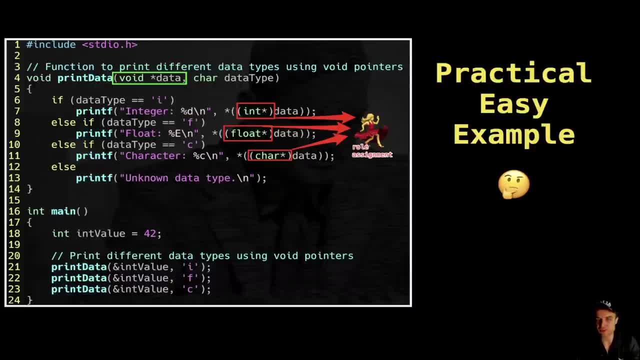 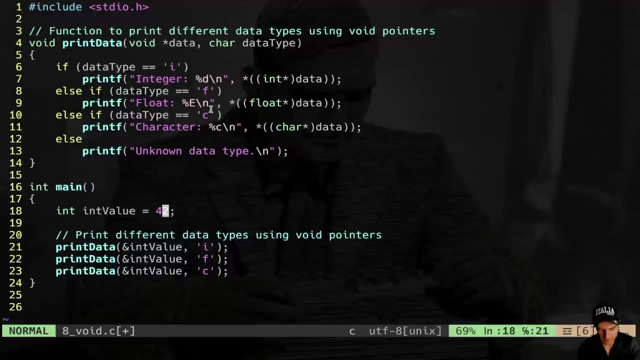 integer f as a float chart is a char. so you see that inside the print data function, i'm assigning the role to the void generic pointer. okay, let's watch the code. okay, here we are. as you can see, i have my integer value here and then i just print the value every time i assigning the role to my 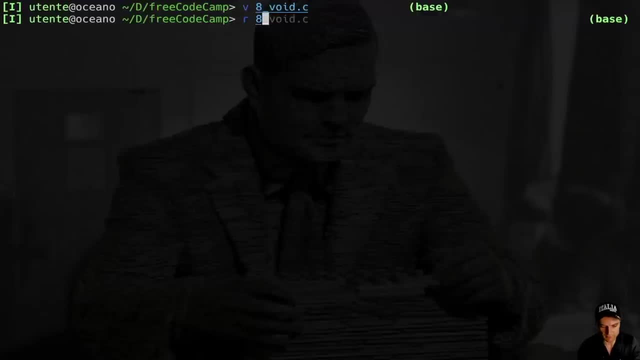 generic data pointer. so i'm gonna run the code and, as you can see, i have 42. if this pointer is pointing to an integer, i have the value which you saw before, which is the binary configuration of 42 if it was a float, and then i have the star if it was a char. you understand everything related to 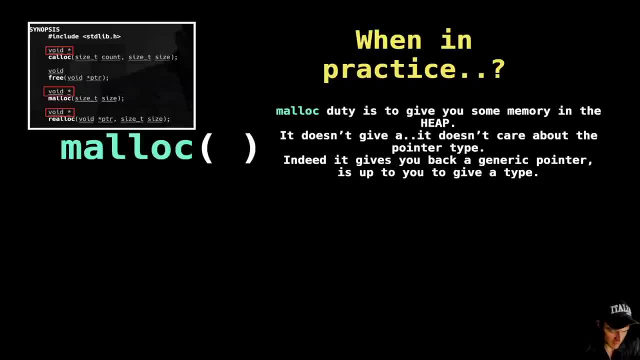 this topic, i guess now when, in practice, we stumble upon these void pointers. well, when you use the malloc function, you see how many times you have used the malloc, namely requesting at runtime some space in memory. well, the malloc is returning a chunk of bytes in your memory, but it doesn't really care about. 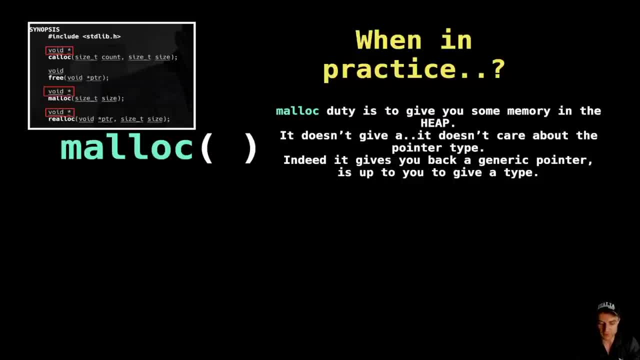 the data type. that's up on you. you are going to decide the specific data type, the specific role that the pointer has to play with a casting right. every time you use the malloc, you're going to get a void pointer. now, my friend, given that we are talking about the malloc, i want to show you. 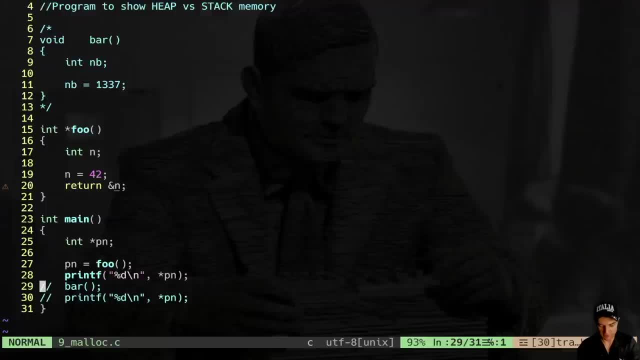 another little program which can be illuminating about the use of pointers. so here in my main i have a declaration of a pointer right to an integer and then i assign the value to this pointer. the return value of fu. foo is a function that is returning a pointer, as you can see here. 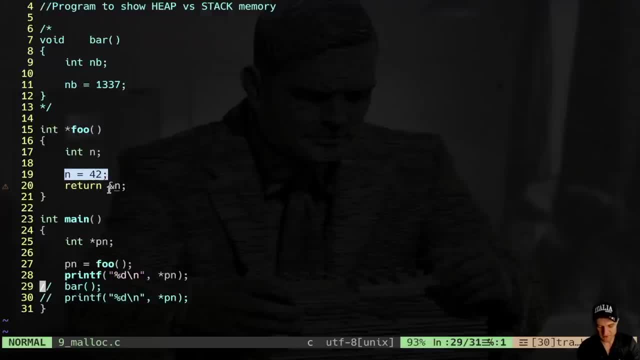 and essentially is returning a pointer to a variable which is a local one, is returning the address of n, which is a variable. inside that, the. what i'm gonna do? i'm gonna use tuff to print the, uh, the value pointed by the pointer. okay, what do? 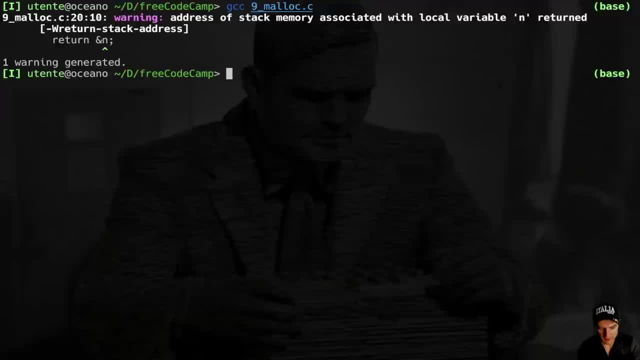 you think this program can work, let's watch out. so i compile and immediately you see that i have a warning. i have a warning address of stack memory associated with local variable and returned. this is tricky. then i'll launch and it works. so i have my 42, but now let's try to change a little bit. 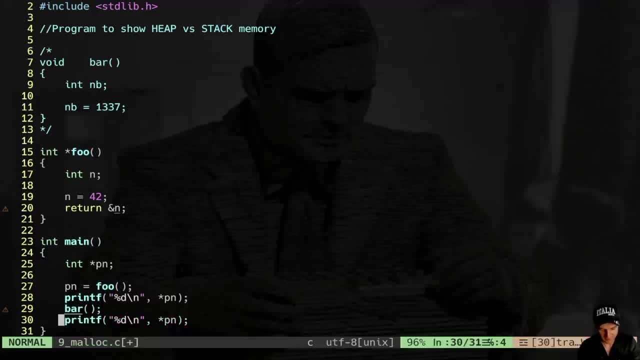 the code. i'm gonna uncomment this other function, which is bar, and this function, very simply, is going to declare a variable and assign a value. that's all there is. that is going to happen in this code. let's try to launch and then try to deconstruct. so i'm going to compile and launch. 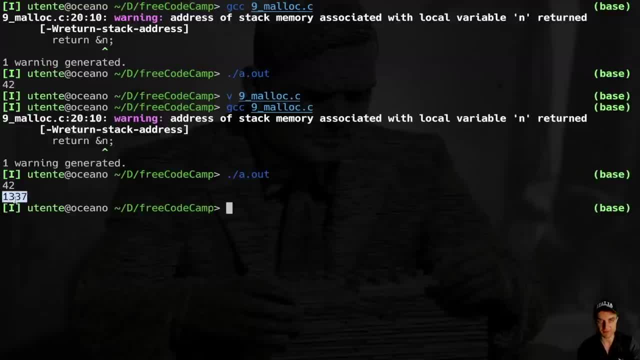 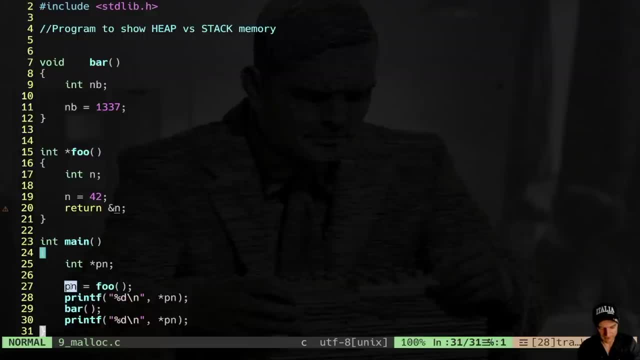 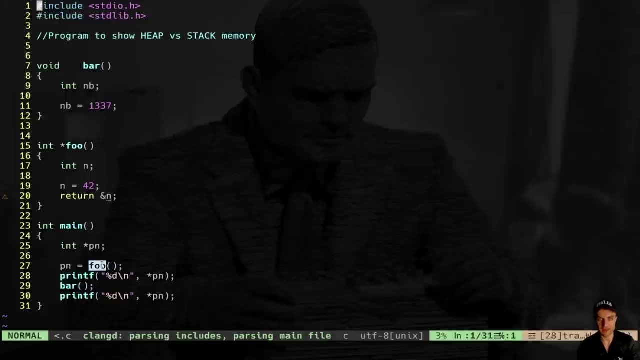 i get first of all 42 and then i get 1337. what happened i mean here? i never changed um the value of the pointer, right, it has always been the same. now, my friend, the issue with this code is very simple. so when i call the function full, i have the allocation in the stack of this function, right? 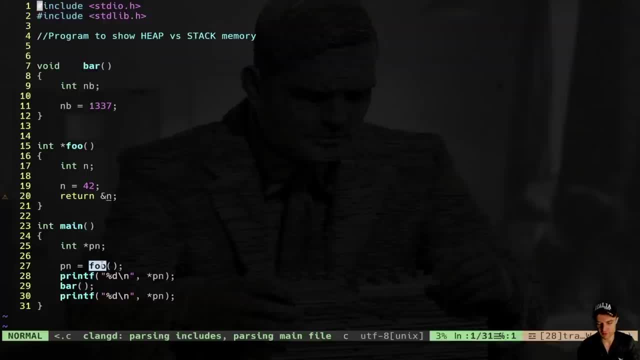 so. so my main function is going to stay idle and then foo is going to perform stuff. essentially, it's going to declare this variable 42 and then it's going to return a address to that variable. cool, after that, what is going to happen? well, i have the full function that gets the allocated 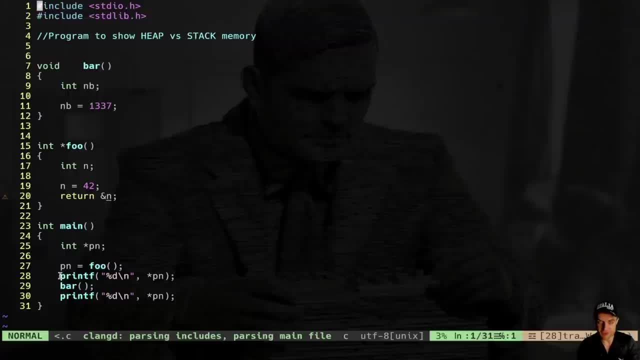 from the stack. so i have a variable which is in a place in the stack which is not allocated anymore. is the allocated. then i call my printf ever. i have 42, because that place in memory is not overwritten by other functions. and then what do i do? i call the bar function. so i have another allocation just above the main, like 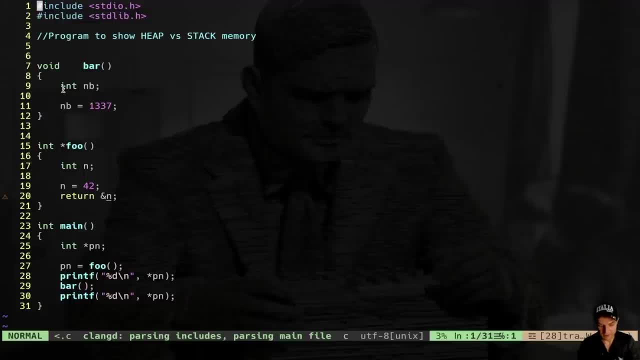 the foo before and the bar function this time is declaring another variable, is declaring this variable here and assign another value. so the address that is the one of the previous variable and which was in full now is the same address of nb. just by chance, right, because we know how the 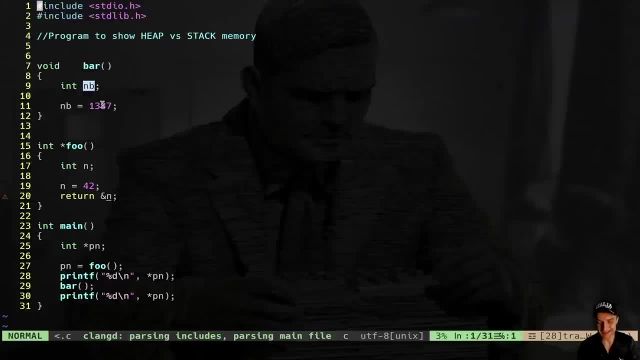 stack routine, the stack discipline works. we can, in a knackish way, assign a variable to the stack, assign another value to the same address. so that's why in the second printf, if we print from the same address, we get this other value here. so now you understand very well what is going on here. 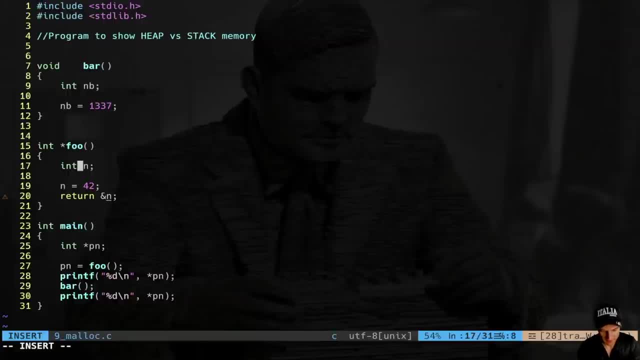 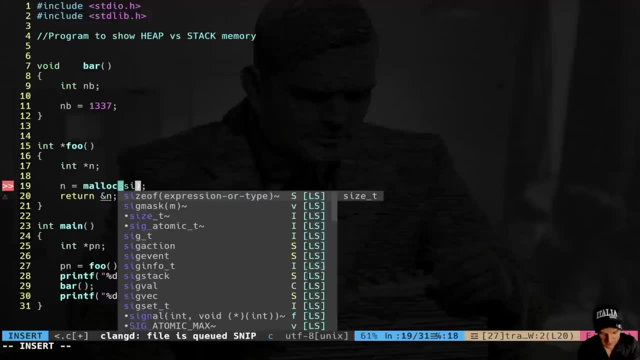 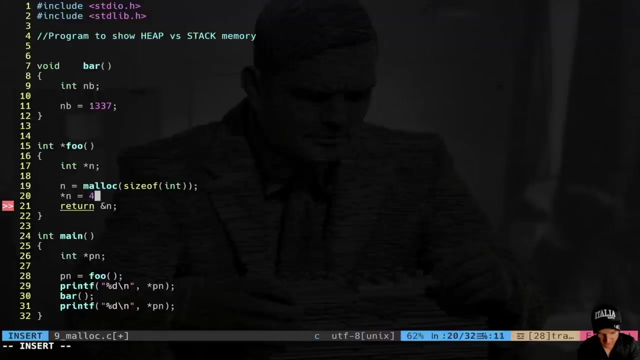 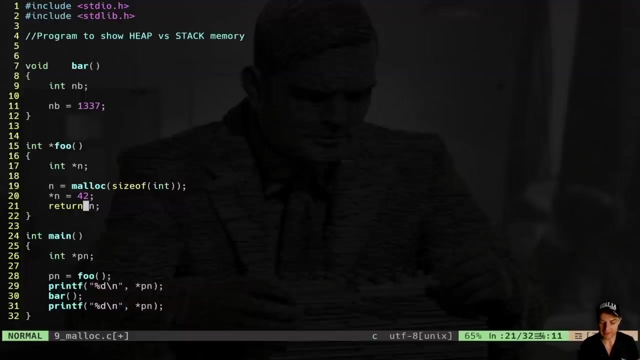 so why the malloc? um, i'm gonna say int pointer. i declare a pointer to an integer and here i do: n is equal to malloc size of int. okay, and then i say at n, so id reference this address. i say 42 and then i simply return n. i return a pointer, so this data now lives in the and it's. 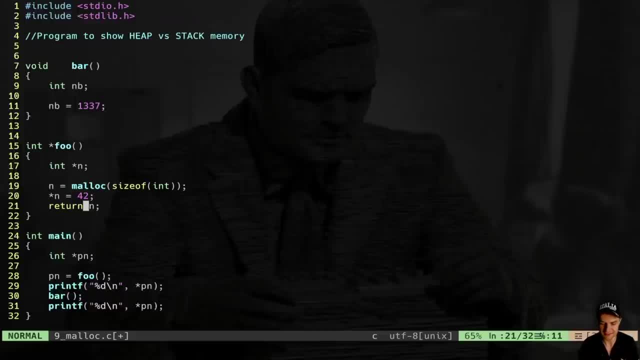 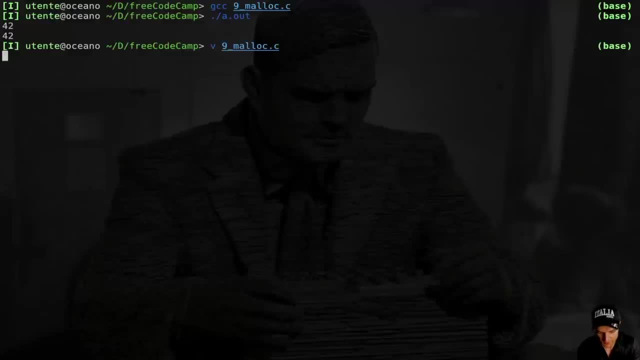 not going to be overwritten, because in the heap we don't have a nip uh, discipline, we don't have an allocation and the allocation of stuff. so let's watch again the code, and this time i'm going to get 242s, of course. right, i think that here it's useful to see visually. so we're gonna. 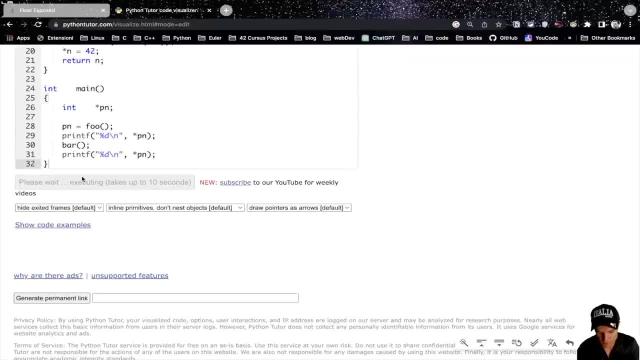 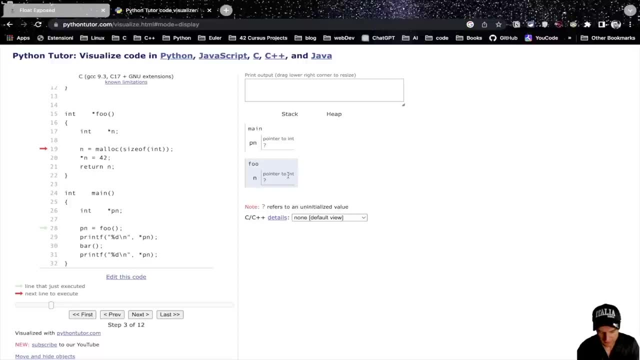 copy this and past in ctutor so we can see what happens. so i'm gonna run. i call this, call my function foo. as you can see, i have another um stack frame and then i call my malloc. as you can see, now we live in the heap. we're pointing in uh, four bytes which are in the heap. 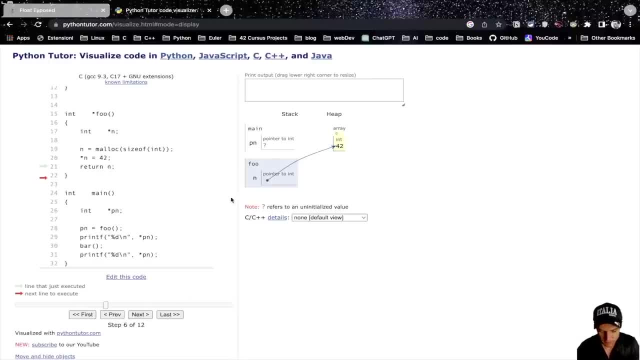 assign there the value 42 and then i'm going to return this pointer. as you can see, i have this pointer in the heap that gets returned to the main function boom. so now i have a reference to my 42 and when i say print what is inside pn, i'm gonna print 42. when i call the function bar, 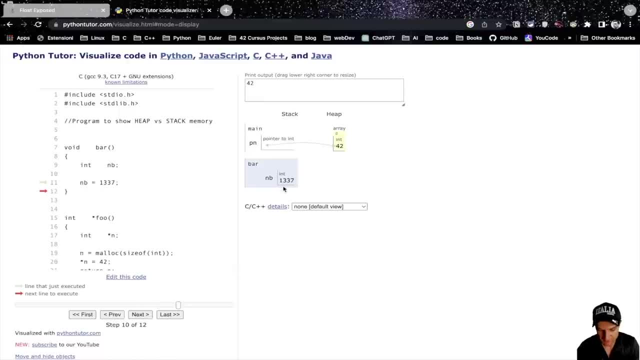 here and i get the variable declaration. i don't have any arrays of previous values like before. right, i hope you understand this point. but no, nothing, because the heap is there, idle, nobody's touching it, and here we go. so the second time you're gonna print again 42. 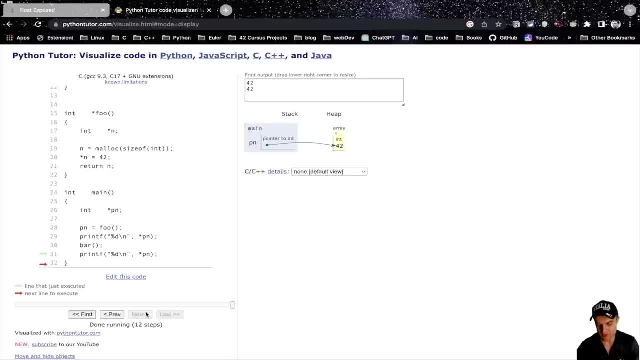 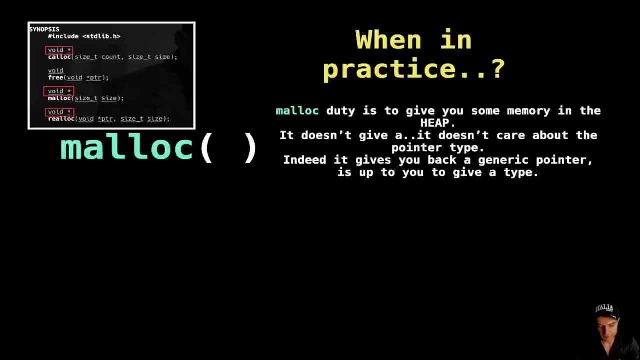 so that's all there is, and this is a thing by which the memory in the heap is useful, because this is memory that is leaving idle by- uh, the stack madness that is happening, allocation and allocation stuff. okay, so this is a silly example of the malloc function. now, if you watch manual, 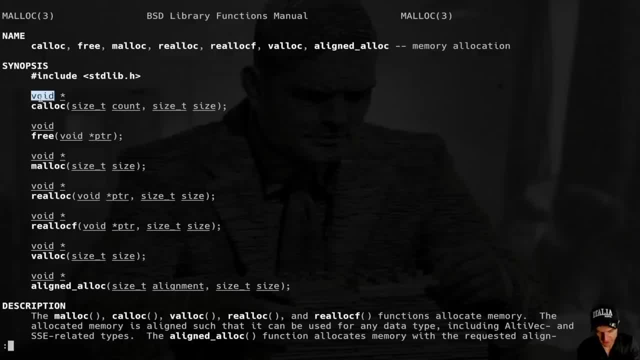 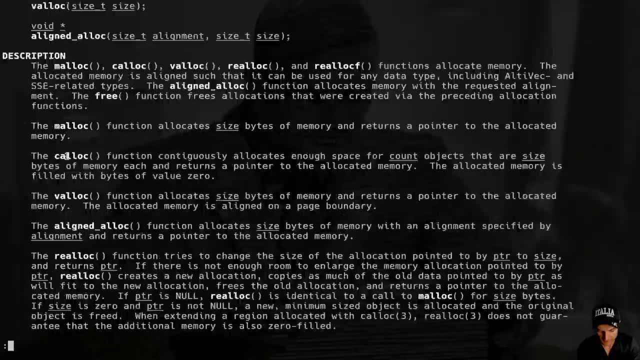 malloc. we are gonna see what i used to tell you that every time we are gonna receive a void pointer from malloc, then it's up to us to cast it to the specific value we want to have. okay, another important thing that you have to keep in mind is that you cannot, of course, dereference. 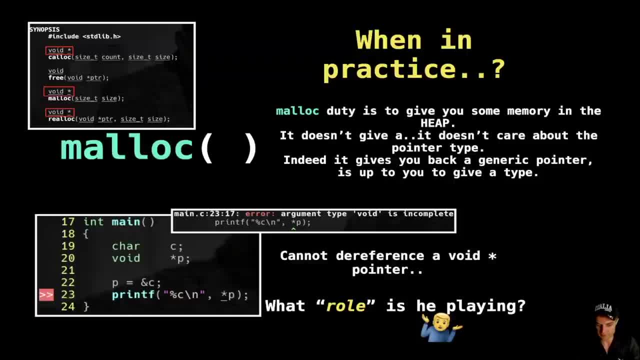 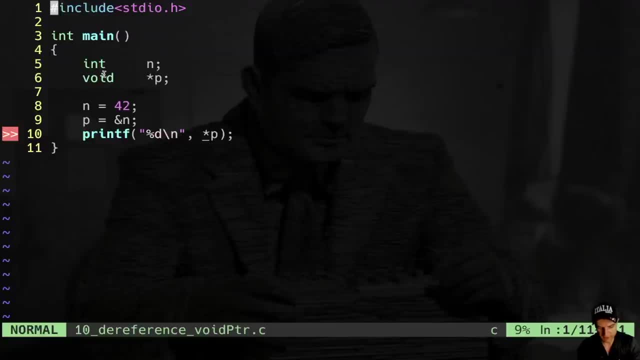 so look at this example. i have an integer and and then i have a void pointer in which i assign the address of n, but when i try to reference it, you see i have a mistake. immediately it's gonna say: hey, i actually don't know which is the data type pointed out. shall i read the bytes pointed? 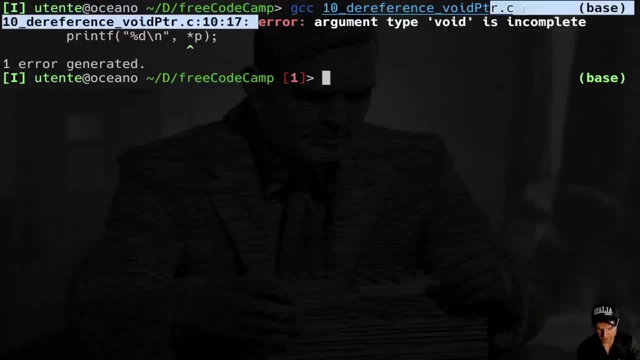 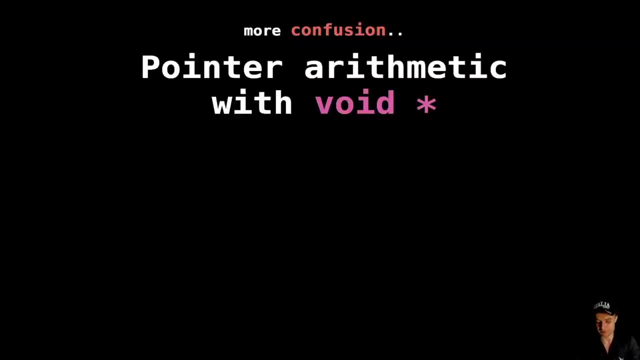 so if we compile, i'm going to get an error. argument type void is incomplete, of course, and you understand super well by now what is going on. now i want to add some more confusion to your life. okay, with these pointers- and this is the question of pointer. 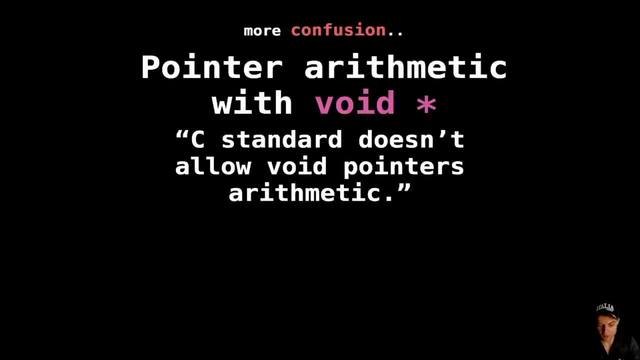 arithmetic with white pointer. do you think it's feasible? well, c standard doesn't allow. what pointers are in magic void, indeed, is a no type. so it's kind of tricky to understand how to handle arithmetic right, because you know that arithmetic depends by the size pointed. if i'm pointing to 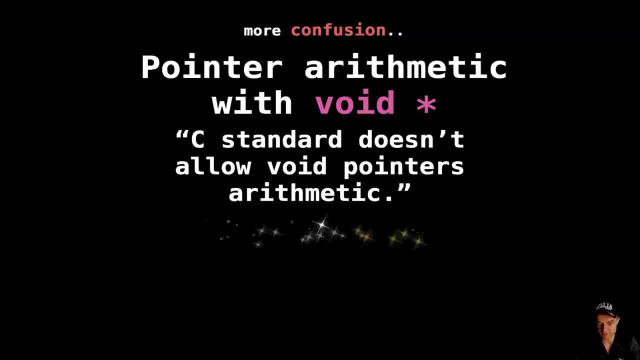 a short, i'm gonna jump two bytes by two bytes. but it's kind of tricky to get the size of a no type, because void is a no type. long story short, we can, long story short, we can. do pointer arithmetic with white pointers. what is going on here, my friend? well, we have a GNU extension. let me explain better. 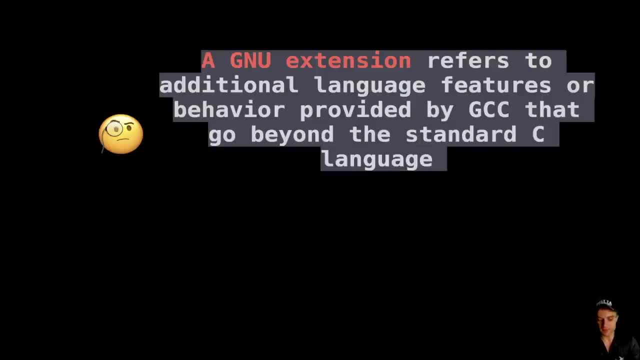 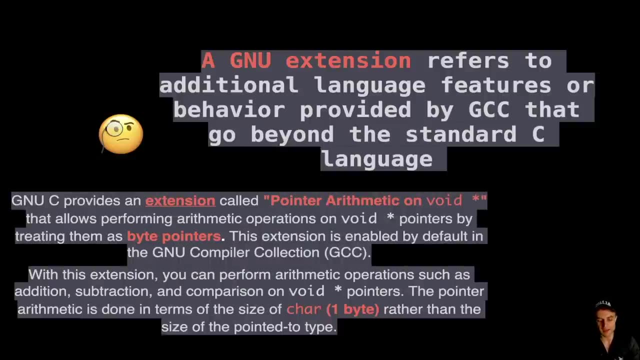 a GNU extension refers to additional uh stuff that you can do, additional features you can perform with the language beyond the standard, beyond the standard c. in this case we have an extension which is called pointer arithmetic of volume pointers. long story short, we are gonna treat about point. 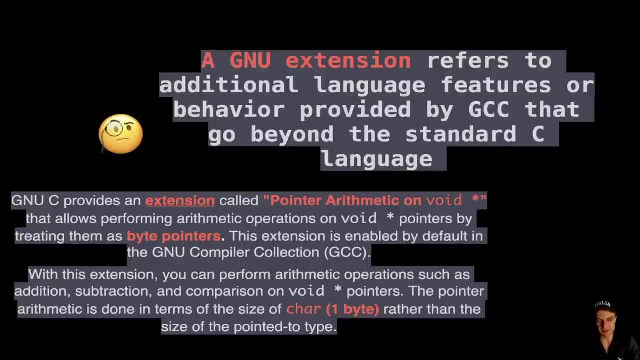 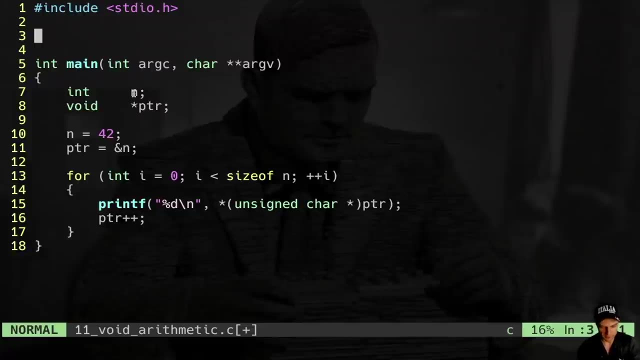 as a pointer to a byte. this makes sense, right? because when we have a void pointer, we are implying that, uh, we have a pointer to a byte. i just have a generic pointer to a byte, so to prove you this: uh, pointer, arithmetic, avoid pointer. so i have this little program, my usual variable, uh. 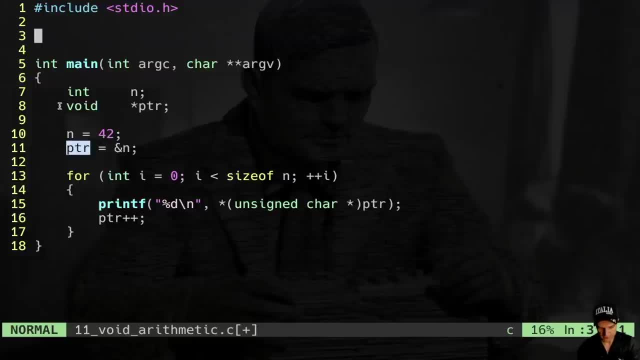 42 and then assign the address of 42 to ptr, which is a void pointer. then i do some pointer arithmetic so i'm going to print the, the value pointed by the pointer. here i do a typecast just to make the reference possible, because i cannot the reference avoid pointer. so i'm gonna do. 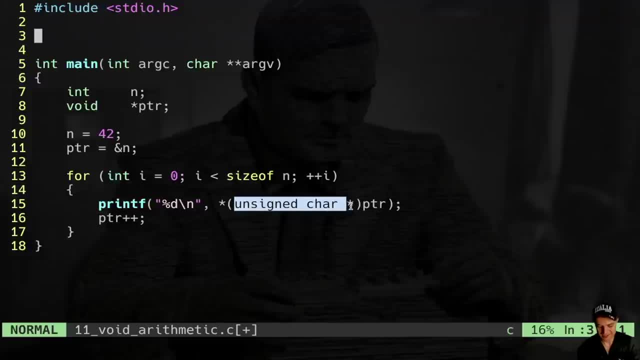 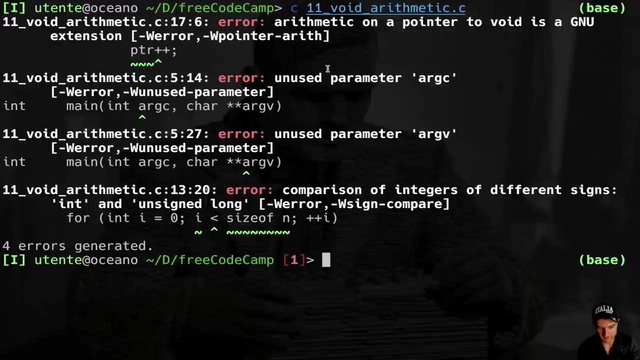 reference as an unsigned char. why is that? well, because i'm unsigned. char is a byte, if you think about that. and then here the magic i'm gonna do: ptr plus plus. so what is it feasible? ptr plus plus. let's launch the code here. i'm going to compile with all the flags that i have, as you can see. 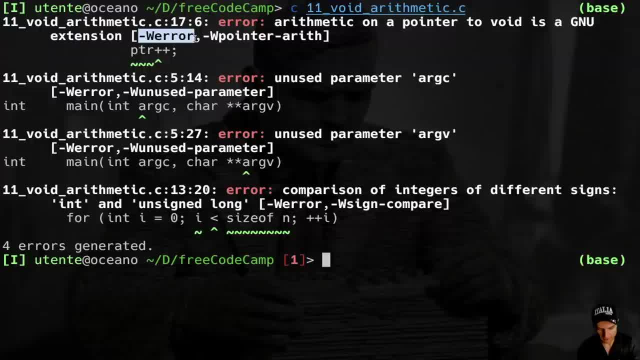 i'm I have error because I'm using the flag W error. This is going to make of every warning an error, but this will work. I have arithmetic on a pointer to void is a GNU extension. Basically, it's telling me: hey, this is something more. 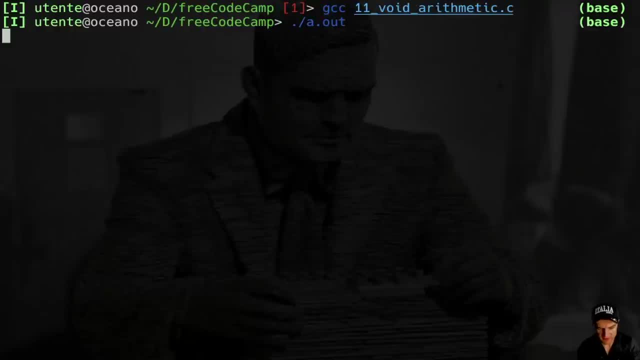 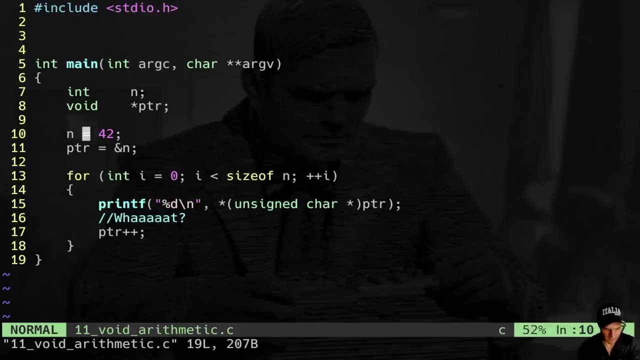 This is not the standard C. Now I compile, void arithmetic and then I just launch. So you can see it works. I have just the values that are printed. Let's do, for example, 256.. I will get 0, 1, 0, 0. 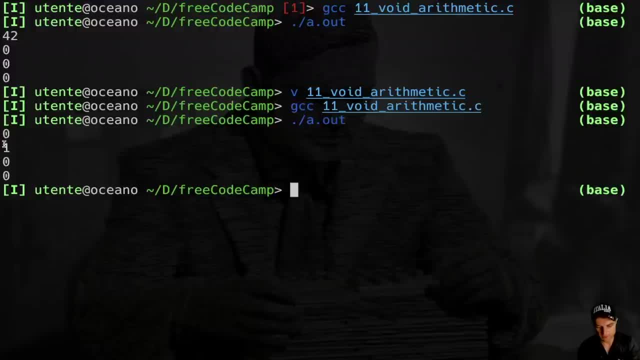 Let's watch it: 0, 1, 0, 0.. You see, You understand why I got 0, 1, 0, 0? Because I have only 1, 1, which is the ninth bit. 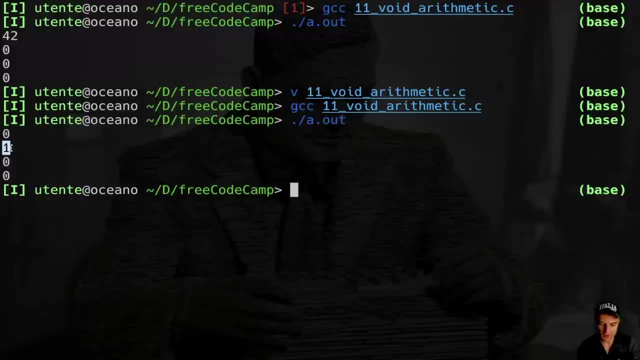 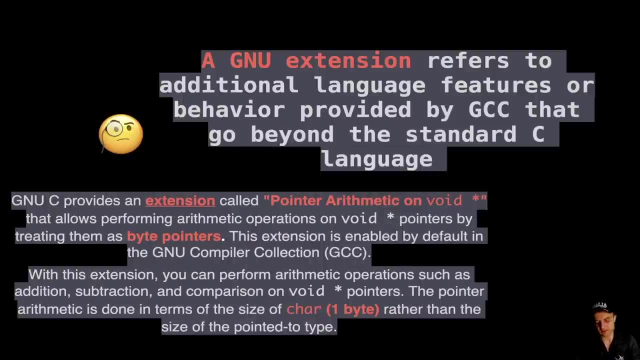 The ninth bit is the least significant bit of the second byte. I hope you understand this point. So with this GNU extension it is feasible. but it is not a standard C So it is not suggested to use. But now You know that you actually can. 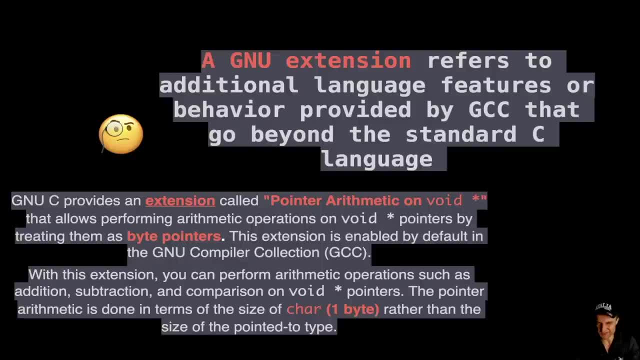 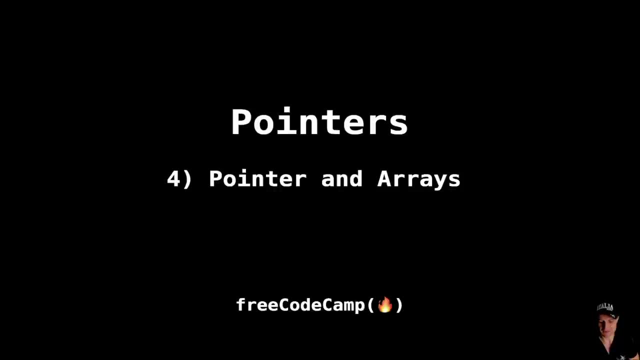 Okay, We already covered a lot of questions which are kind of tricky right, And now we are going to go a little deeper. Okay, My friend, Now I think you have a very good understanding of what is a pointer. Basically, it's just an address of a variable inside your ROM, inside your memory. 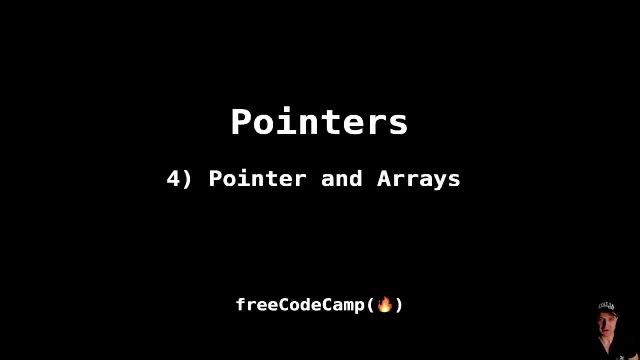 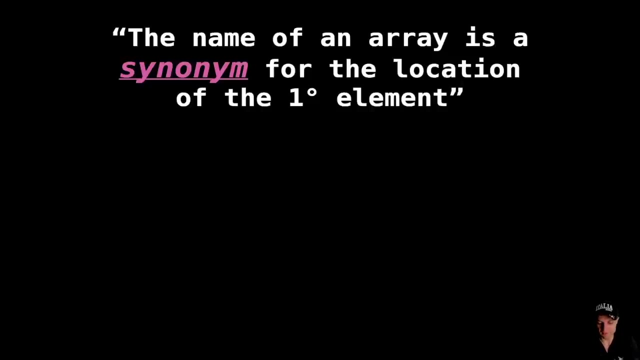 Now we enter a little bit in murky area. Indeed, we have to understand what is this correlation between array and pointers? This, in my opinion, is the trickiest part related to pointers. So let's start from this definition. The name of an array is a synonym for the location of the first element. 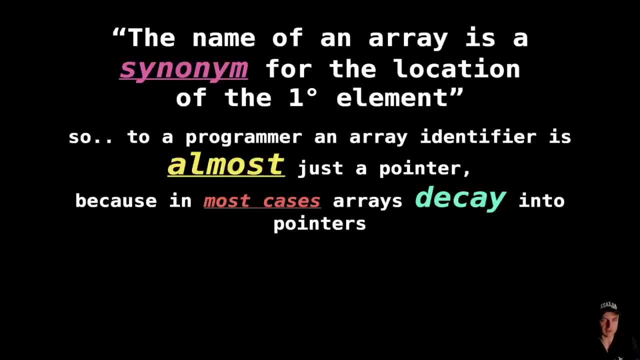 So basically the name of the array is an alias. So to a programmer, an array identifier is almost- and this almost is very big- just a pointer, Because in most cases arrays decay into pointers. Decay is a fancy word that means loss of type and loss of dimension. 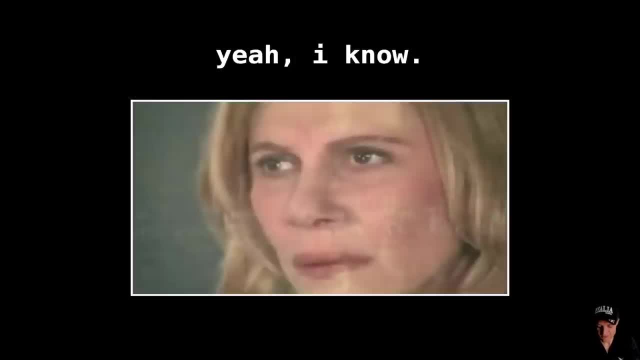 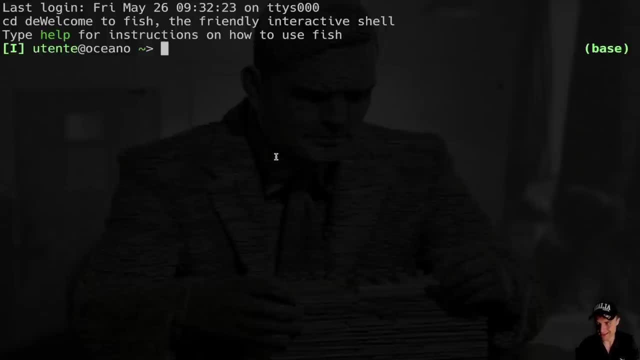 And yeah, I know my friend tricky, But uh, I'm going to try to make it simple, I'm going to try to make all of these as easy vanilla as possible. So what we are going to do now, we are going to create a program that um is going to be self explanatory about this dance between array and pointers. 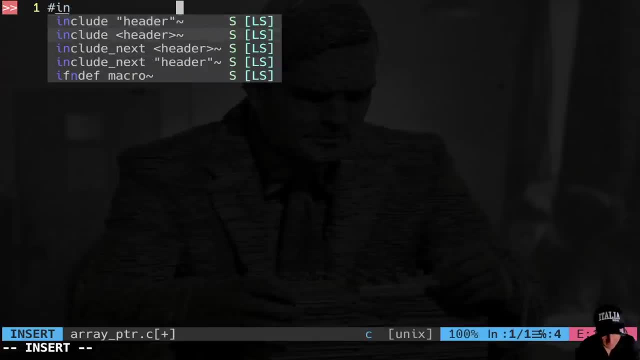 So the usual boiler plates so include, uh, standard input output and then, as usual, my main function, So int main. okay, You perfectly know that to create an array, you just do that right. You just say, for example: let's: 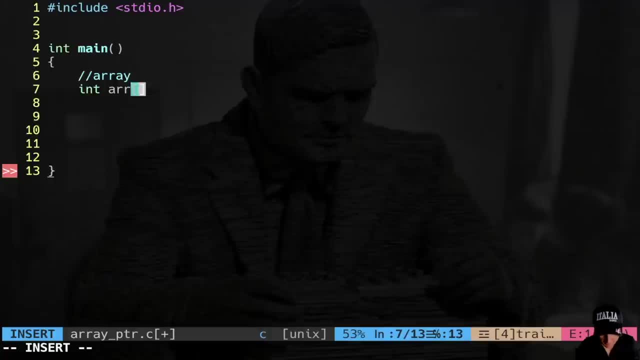 Pretend we have an array of integers. We say int array, which is the name identifier of the array, And you can say 10.. So this is gonna uh create an object of 10 integers inside your run, more precisely, inside your main stack frame. 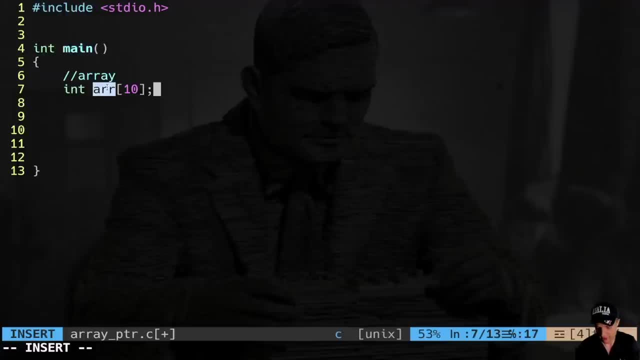 Now I told you that at the end of the day, the name of the array, the array identifier, is basically a pointer to the first element. If I do something like that, pretty tough, Be new line, And I say R, I'm gonna get the address of the first element. 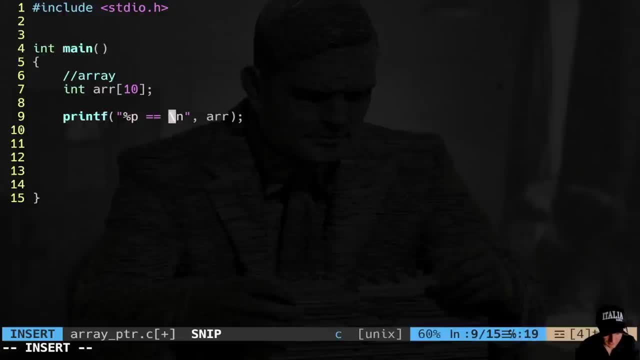 So to make the proof, I can say: B is equal to B and I use here the address of array, The first element, array zero. Do you agree? This is the same right. This is equal to this. Let's try to launch this program. 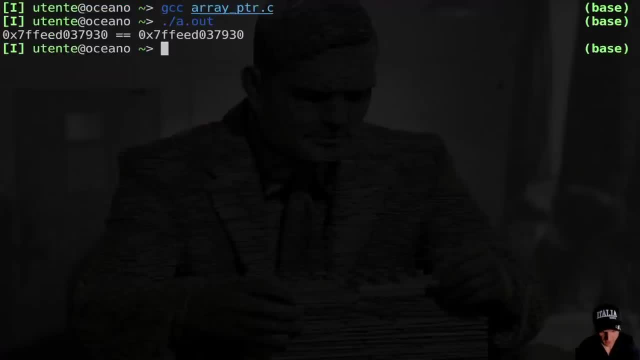 So I'm gonna compile a very pointer and then I'm gonna launch. as you can see, they are two addresses and they are equal. So the name of the array is this one And this is the address of the first Element. So you can see that they are exactly the same. 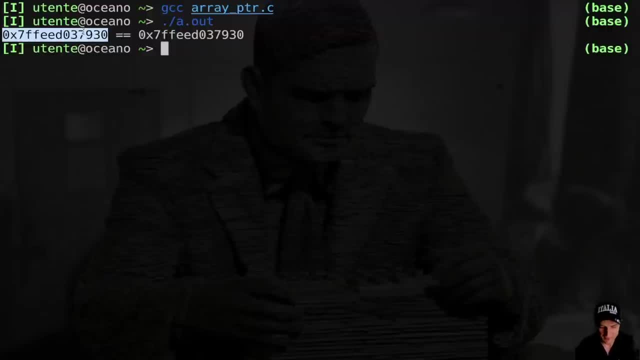 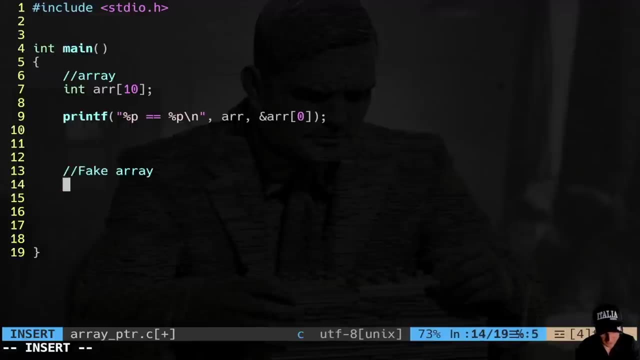 If I say the name of the array, I'm implying the address to the first element. Cool, So here I want to create my fake array using only pointer notation. Uh, so first of all I have to create a pointer. So in PTR, like that: 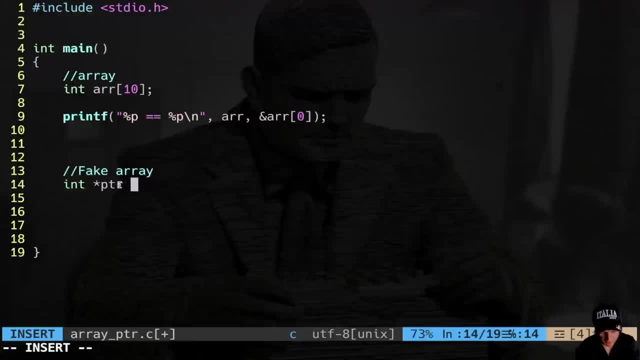 So this is a pointer and um, what shall I do now? So this is a pointer to an integer essentially like array. Now the key difference- that it's immediate- Is that when you use these uh array notation, you are allocating in the stack some memory, right? 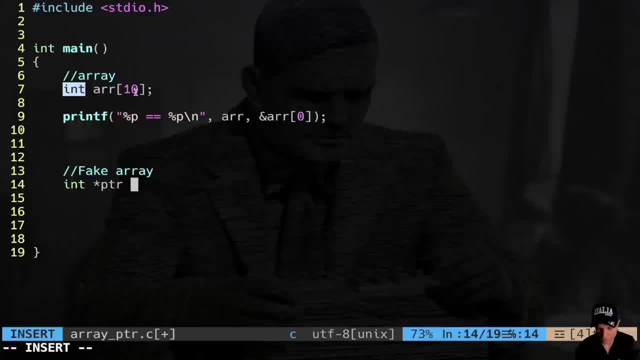 You are allocating essentially 10 per four, So you're allocating 40 bytes. This is an object of 40 bytes. This is not happening with a pointer. right, I have a pointer that is pointing to an integer or random integer, So we don't have a location. but we can have a trick to to to do that. 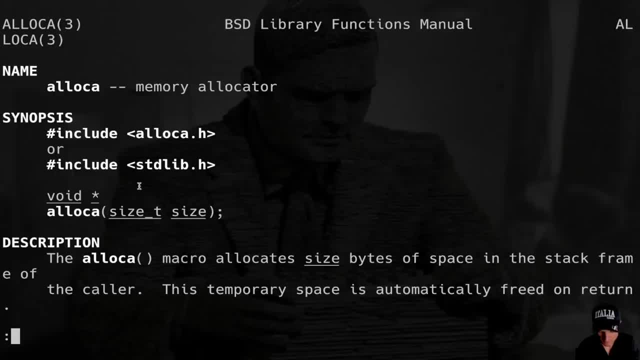 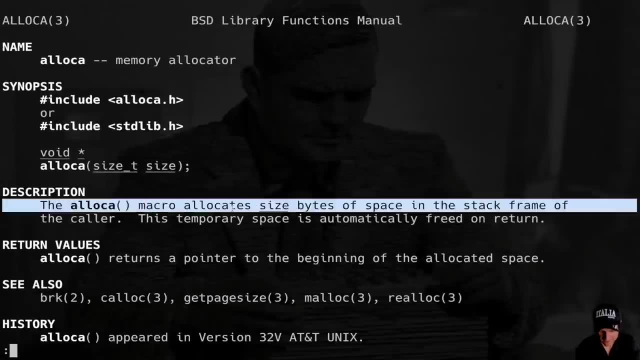 We have a function in it which is called a locker- Not a lot Used because it is not, uh, suggested, but it exists. So the aloka macro allocates bytes of space in the stack. So you see, that's the key difference between a malloc and a locker. 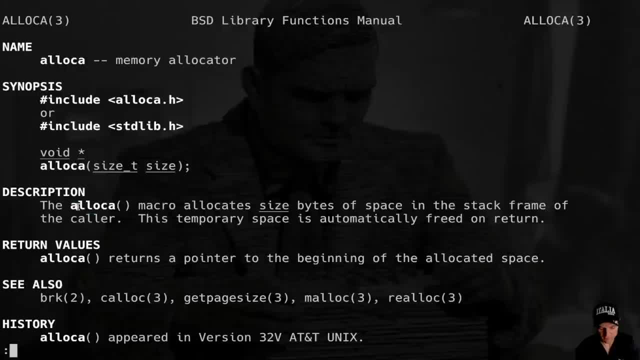 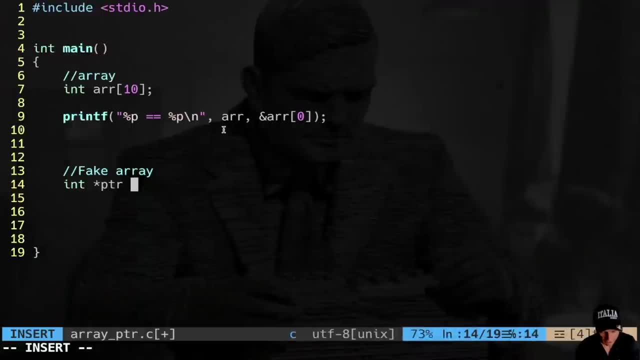 We are in the stack, We are allocating in the stack, So we have this function that is able to allocate some space in the stack, essentially like an array, right? So now I can do something like that, I can do a locker. 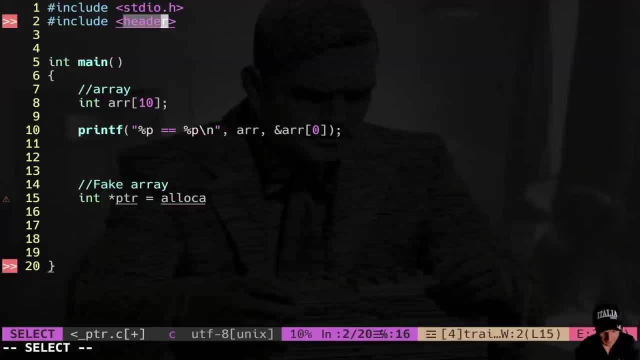 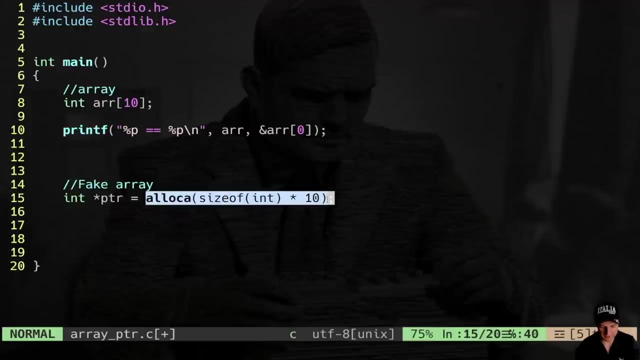 Of course I have to include uh, my Uh standard library. I call a locker, of what size of int per 10.. Okay, So a locker is going to allocate in the stack 40, uh bytes, essentially the same thing that is happening here. 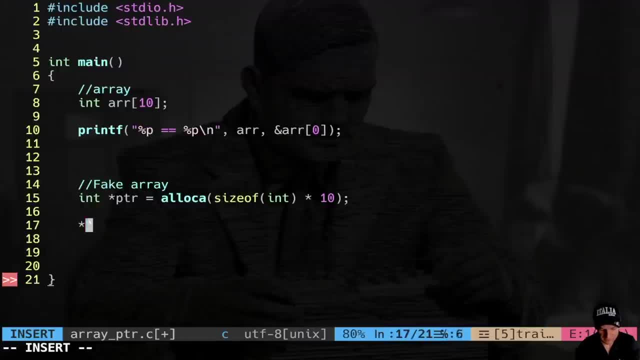 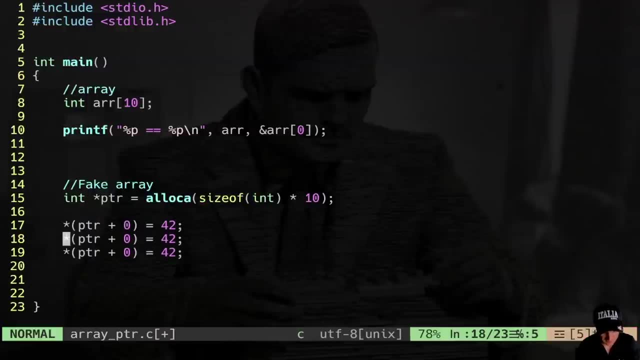 Cool. So now I can say: um, at PTR uh plus zero is equal to 42, as well as some other examples. So I can say: at PTR plus one, Okay And uh. and at PTR plus two is equal to another number on 337 and minus 21.. 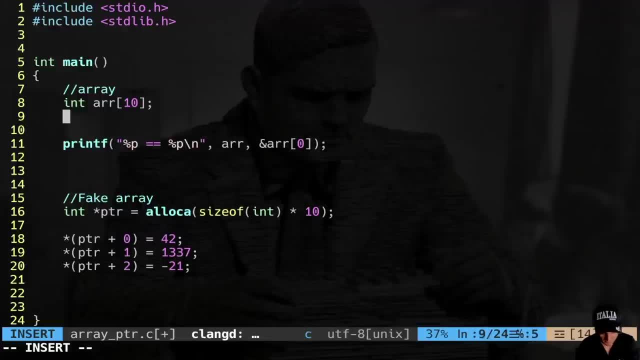 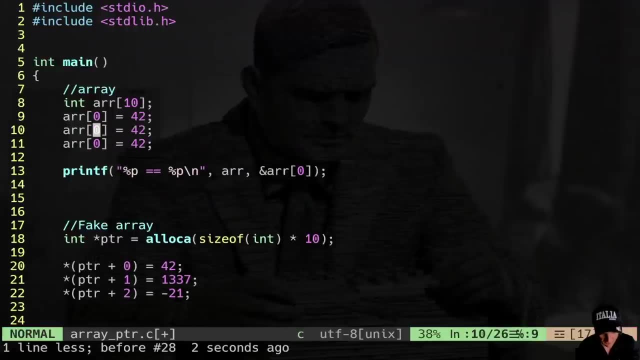 Let's do the same with the array, with the array notation that you know pretty well. we have array zero equal 42.. I'm going to copy this and past, and then I do: array in position one is equal to the same value. as well as for the last. 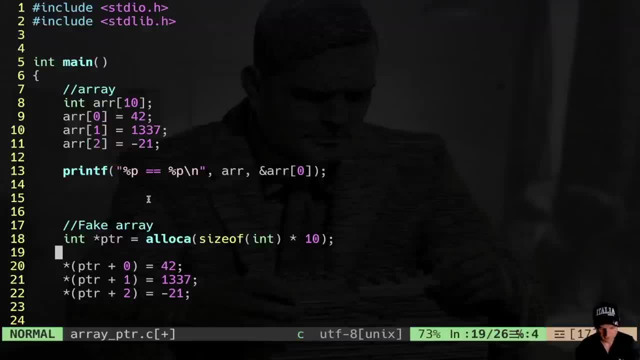 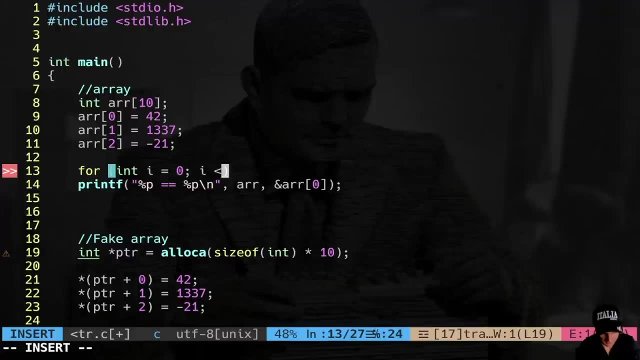 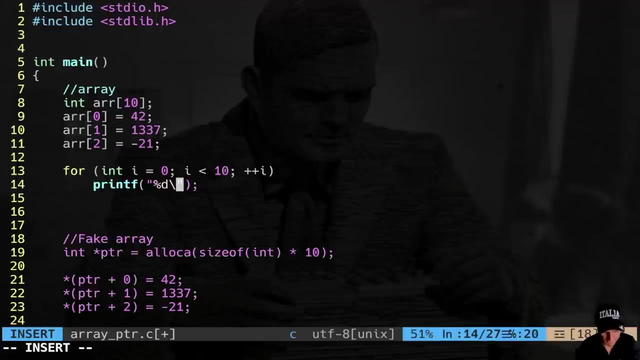 Okay, We have something which is, uh, almost equal, Do you agree? now Let's print The values. So I do a loop for entire whole, zero, eight minor, then 10, and then plus plus I. we are going to print, um, the value which is in the relative position. 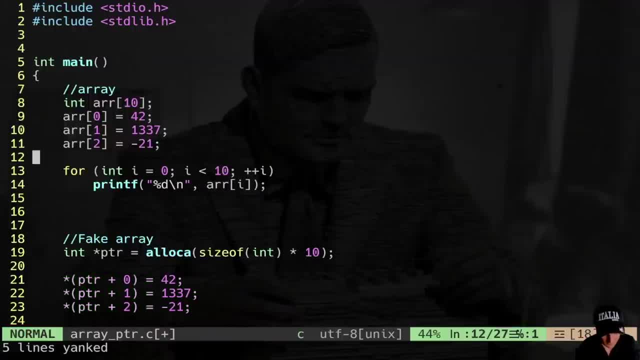 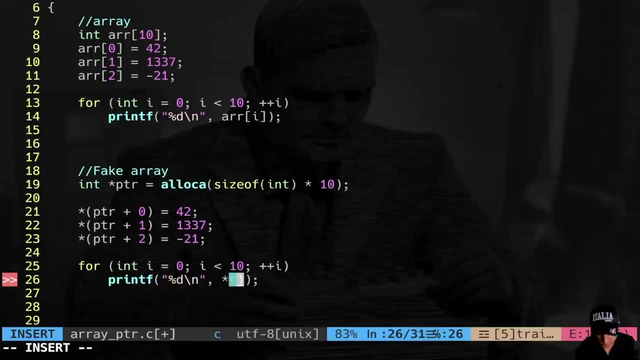 Okay, So we have array in position I. we do the same, essentially for my fake array, Only I use pointer notation. So at uh PTR plus I. okay, Of course I have only uh three numbers. The other numbers are going to be. 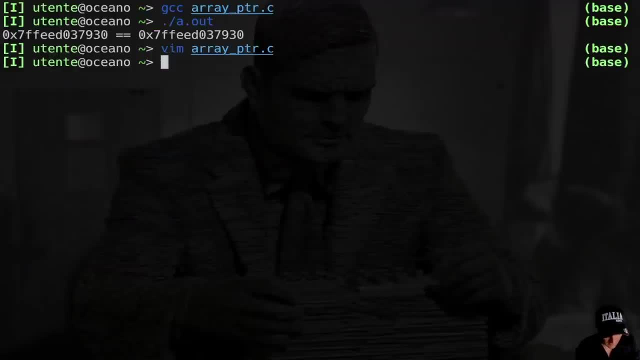 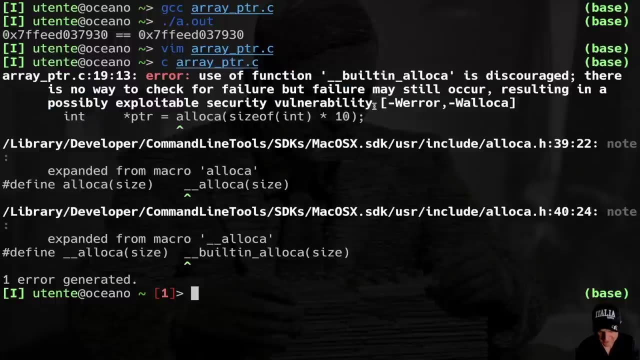 I'm going to use a little bit of a random, but we don't care, Let's try to launch this code. So I'm going to compile with all the flags. Uh, and, as you can see immediately, I have, um, this warning. that is telling me Aloca is discouraged. 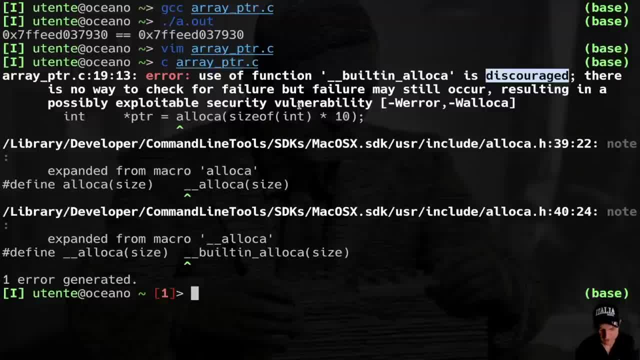 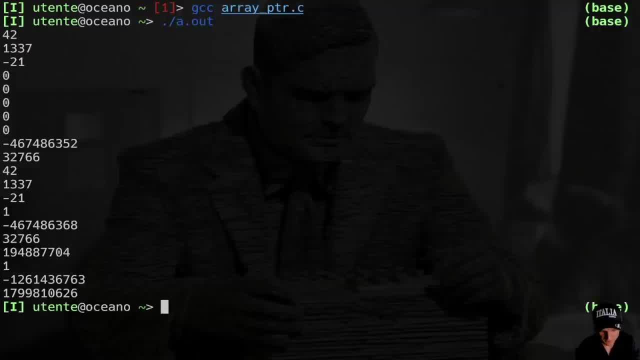 There is no way to check for failure and some other details, but we don't care. This is just um a sample to understand principles, So I'm going to compile normally and then adjust launch. You see, it allegedly works. Now let's make the code more clear in the middle here. 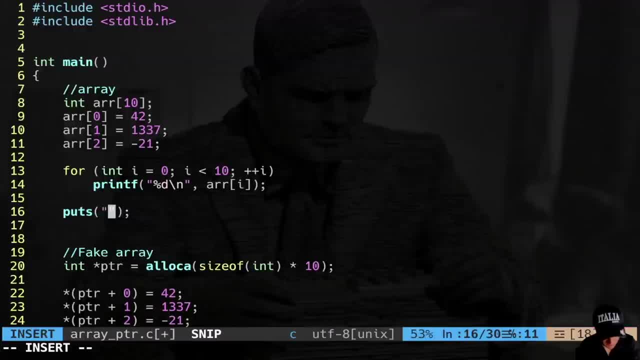 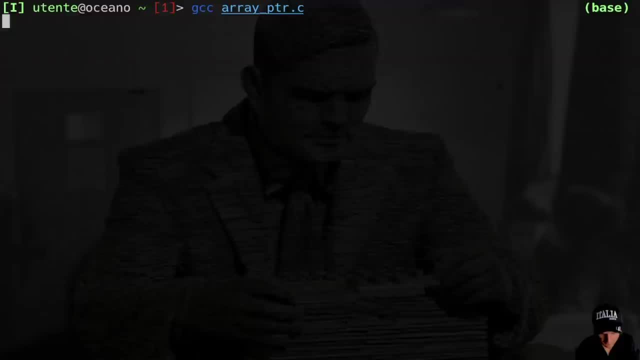 I'm going to put Some spaces to make the code more readable. Okay, Put string: two spaces Plus the one from put string is going to be three. Okay, So I'm going to compile normally and then I'm going to launch. 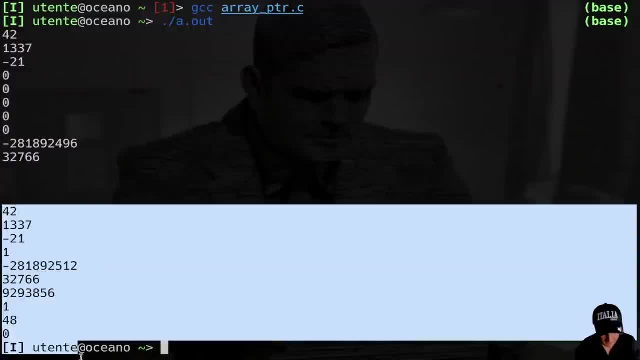 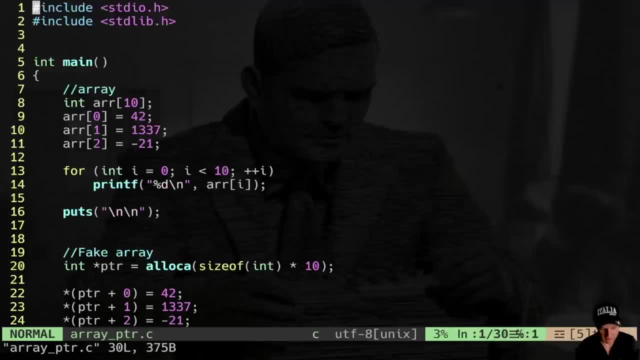 So here it comes: I have my first array and then I have my second array. So, as you can see immediately, the first three numbers are the ones essentially like the real one. Cool, Now it is kind of the same. Let's try to find some differences here. 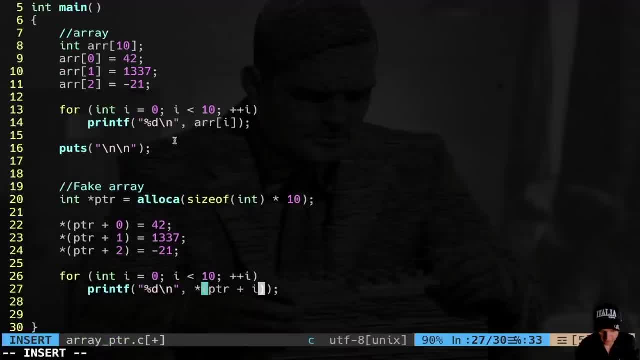 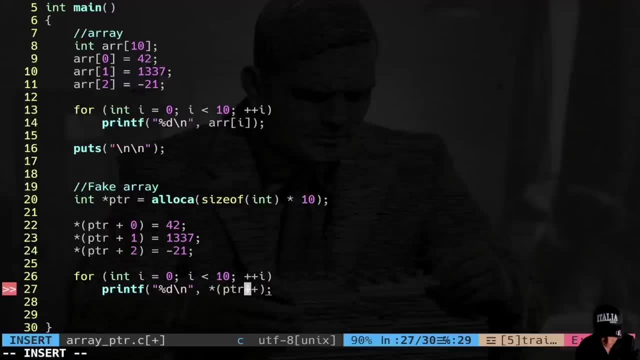 First of all, I would like to increase Direct Lay PTR. PTR is just a simple pointer, a simple variable that I can change, So I'm going to do directly: PTR plus plus. I can remove the braces, Of course, they are not necessary. 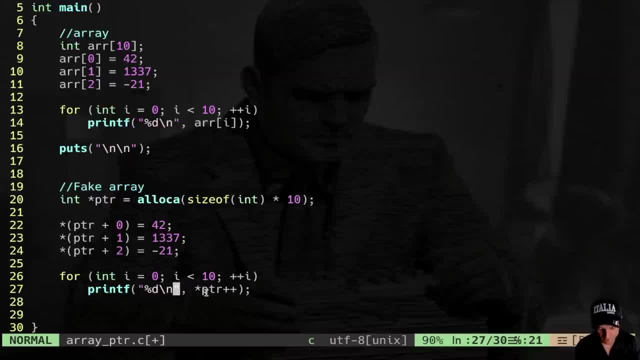 So I remain with this expression. here, Of course, I have these operators. The plus plus is going to be performed before, because I have associativity that comes from right to left when we have a unary operators. But nonetheless, here I want to do the same. 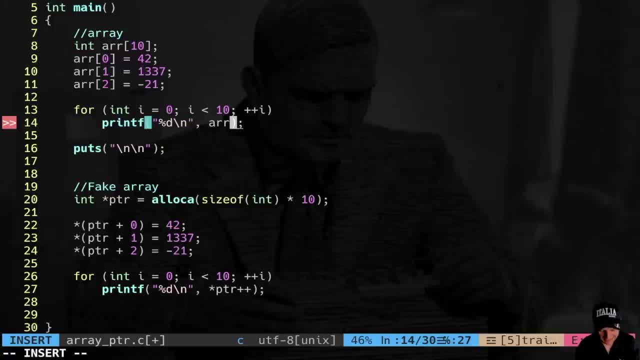 So I'm going to do not array I. I would like to try to increment This and the reference, because we know that the name, the identifier of the array, is equal to the pointer, to the first element. We just saw that. 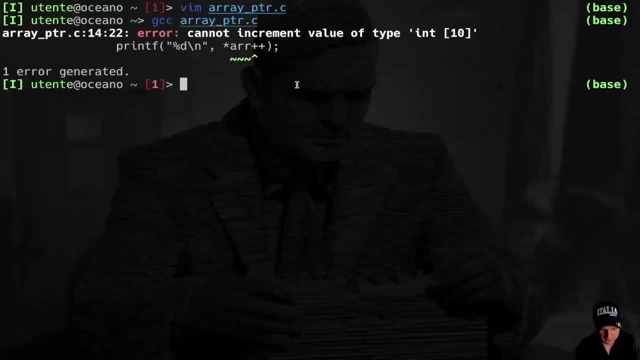 Let's try. So I'm going to compile and immediately I get this mistake: cannot increment value of type array of integer of 10 elements, So I cannot increase directly the value of this identifier. Strange, given that this is just a pointer, right. 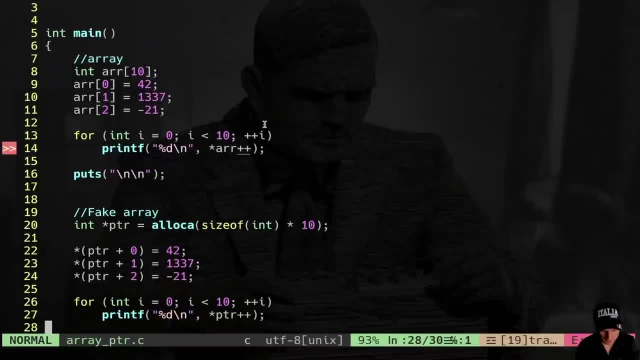 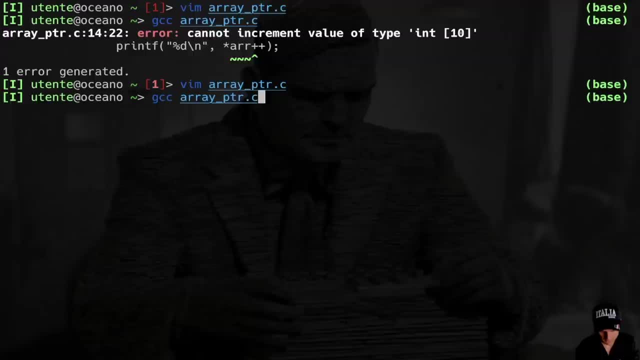 So this is one key difference between these two. I cannot do that. On the contrary, um, on the contrary, I can do very easily, right. So with pointers, let's try to compile a launch. as you can see, it works correctly. 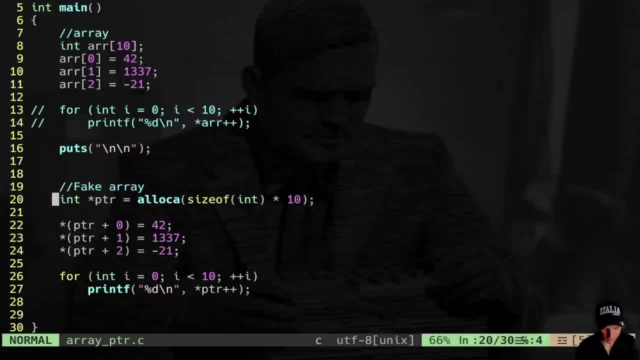 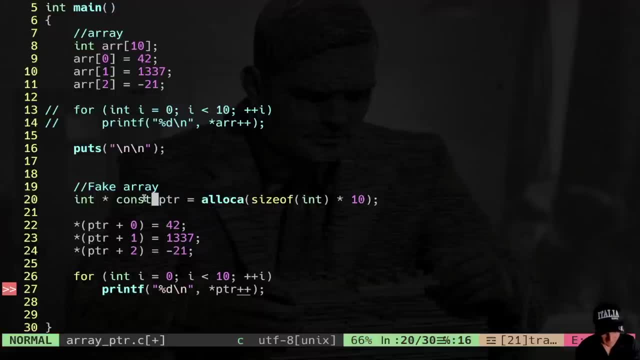 No problem. So to make it, uh, more equal, I'm going to try to do something. I'm going to say: this is a pointer, but this is a constant. Okay, So here is written: This is a pointer, constant to an integer. 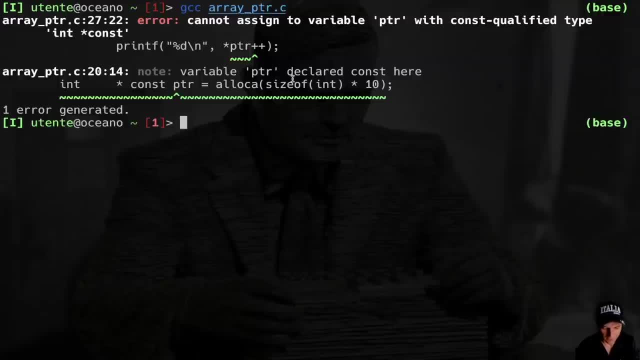 Okay. So now if I try to compile I would get almost a similar thing right Because I have the constant qualified type. So basically I cannot perform pointer arithmetic directly on the pointer itself. Basically I cannot change the value of the pointer. 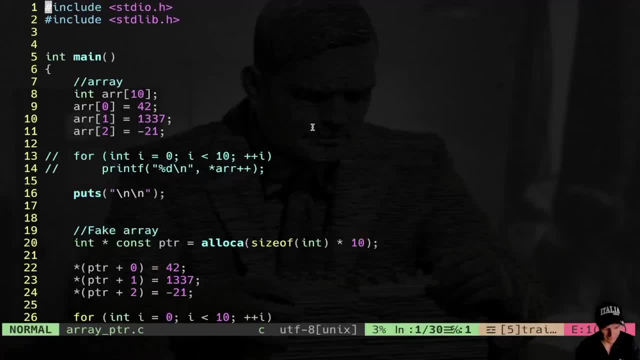 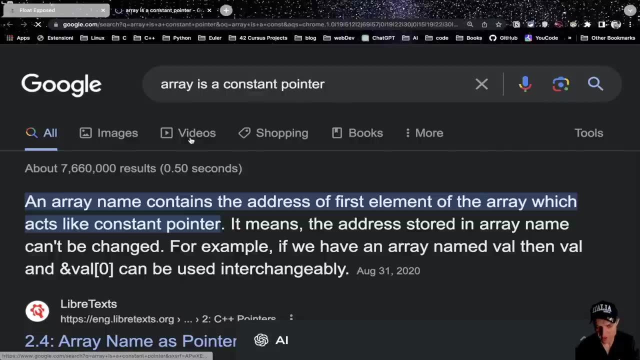 Okay, So we managed to get a similar behavior. If you want, Indeed, when you search online, for example, is an array just a constant pointer? you will find many people that will argue: Yeah, essentially, uh, an array is almost like a constant pointer. 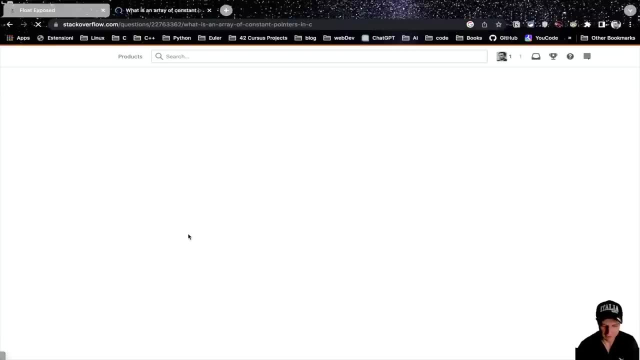 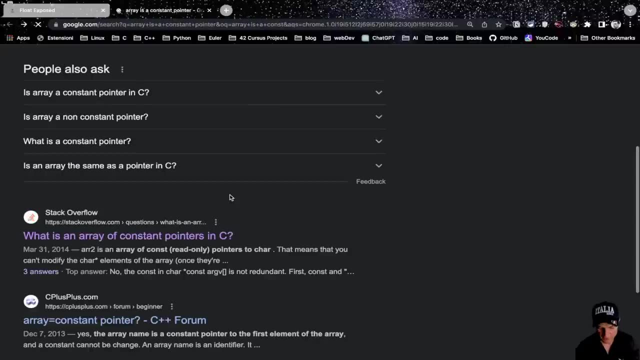 It is not the same, but you can consider an array like a constant pointer. Of course, the answer Is not the case, right? If you want to go deep, they are not the same thing. but search by yourself. uh, is an array a constant pointer, and you will find some good information. 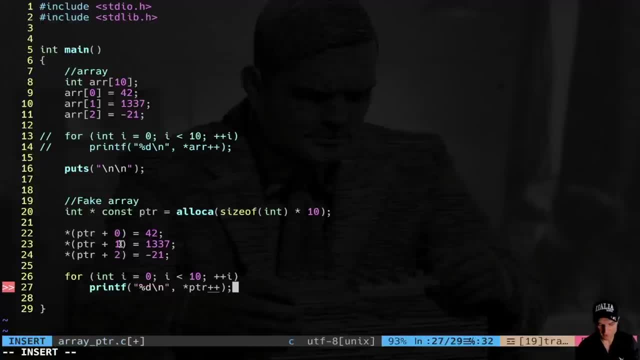 Now people is telling that an array is just a constant pointer. because of this you have this uh similarity and that's legit in your mind. You can consider um the name of the uh of an array just a constant pointer. 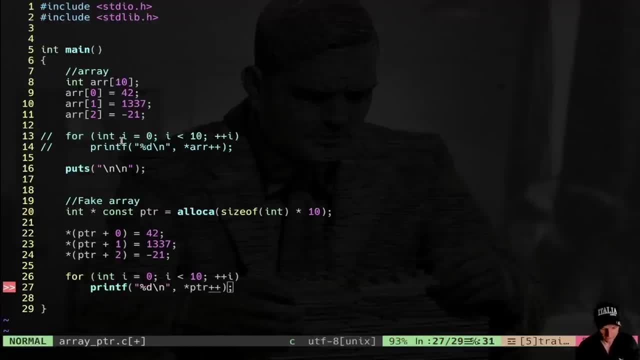 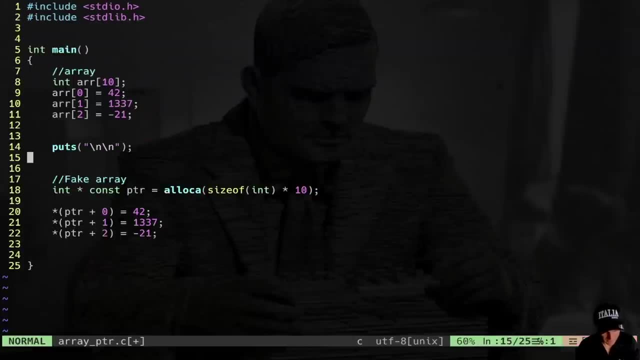 But now I will show you that this is not quite the case. Uh, so let's start from the beginning and let's watch all the similarities between the two. First of all, I'm going to print off the address of the array, and I do person P. okay, 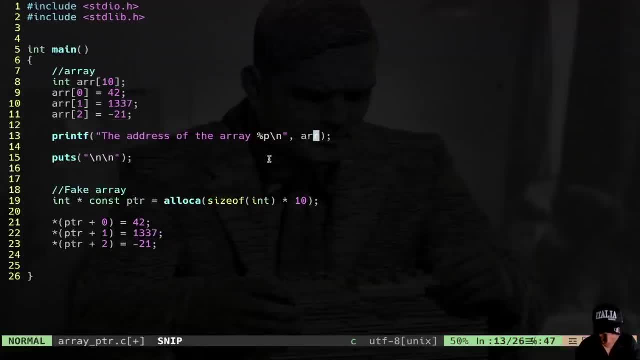 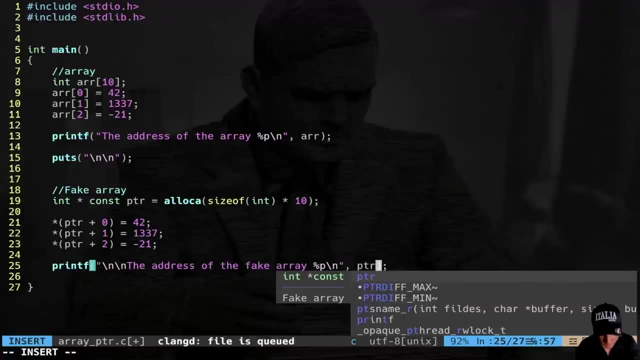 So I use the array identifier, which is array, that you know. that is basically a pointer to the first element, So I can do that. Okay, Here I put this time my pointer. I compile and, as you can see, um, they're pretty close. 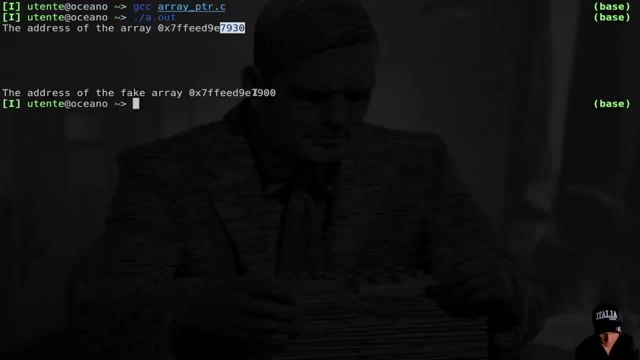 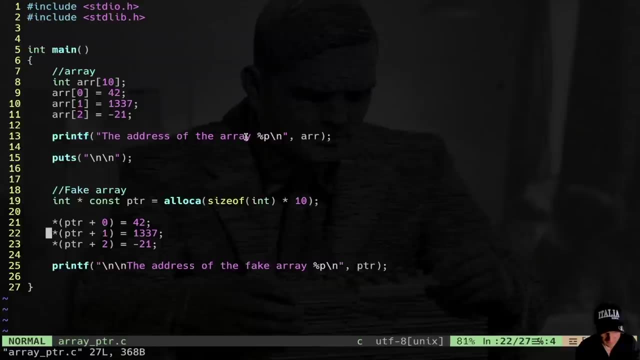 Okay, They are equal 7, 9, 3, 0, 7, 9, 0, 0.. They both live in the stack. Okay, They point in the stack. Okay. So this is the first point. these array, uh, and all these elements are living inside the stack. 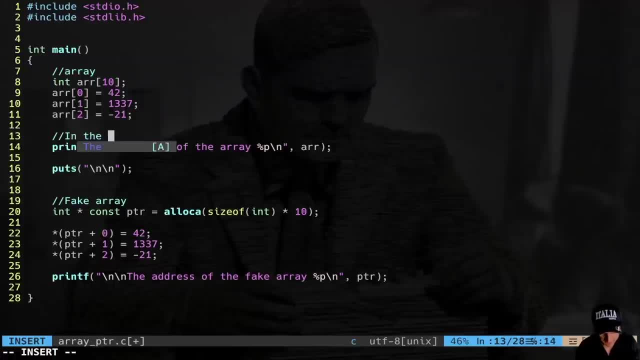 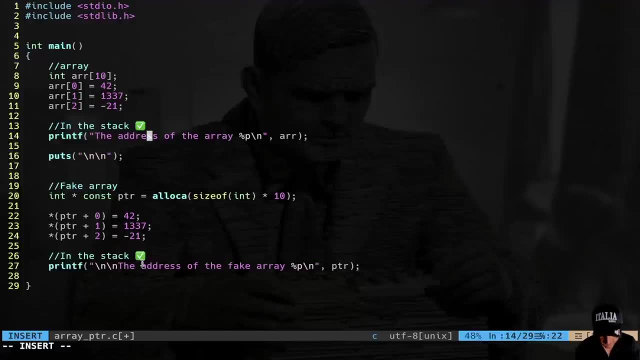 First thing, which is equal in the stack, Okay, As well here in the stack. the other thing that you just saw is that, um, we cannot, we cannot increase, cannot increase Are as well as we cannot increase, um, these custom pointer. 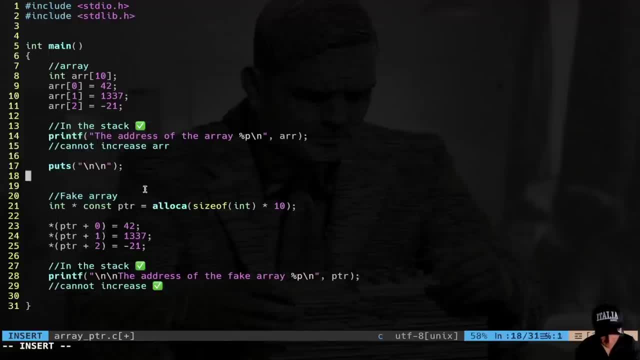 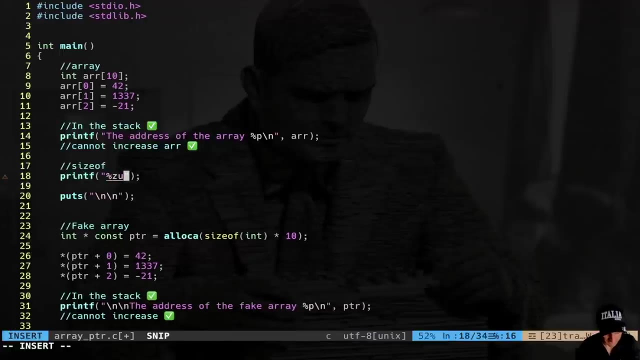 So cannot increase. So this is the same. Okay, We have two things which are equal. Now let's find something which is not equal, And here we're going to do: uh, sides off operator, I'm going to use the sides of operator and I'm going to print off percent, zoo, the size of, of array. 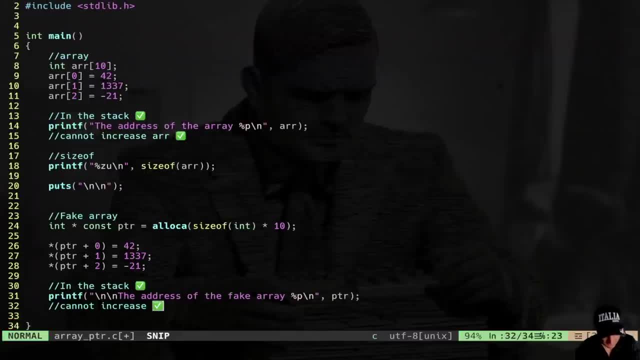 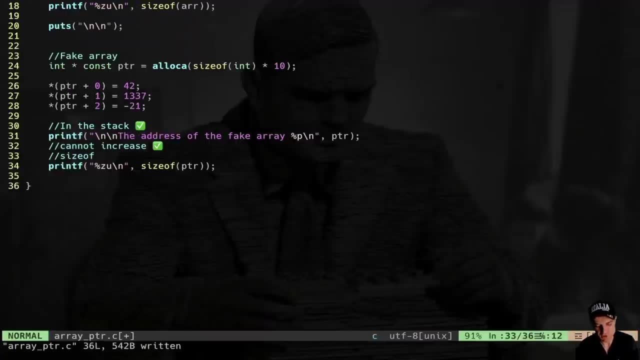 So the size of R- I'm going to do the same here for my pointer- So size of PTR. So let's try to launch this time the code and let's watch if it is exactly the same. I'm going to compile OPA here. 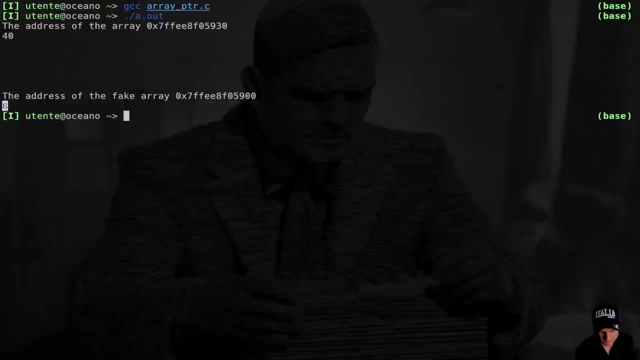 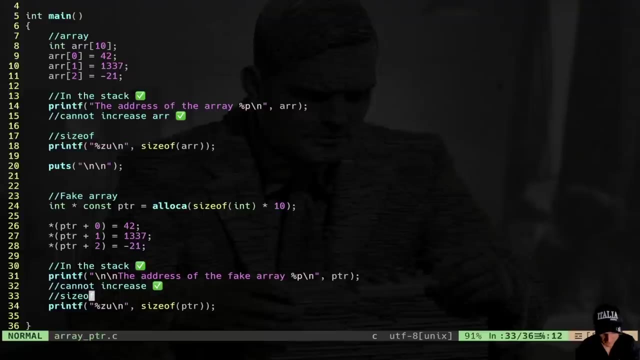 I get something different: here I get 40 and here I get eight. Hmm, So this is a big difference. What is happening? Well, when I call here the size off on my constant pointer, what am I getting? Well, I'm getting the size of a pointer that you know by now that, uh, this is eight bites, right? 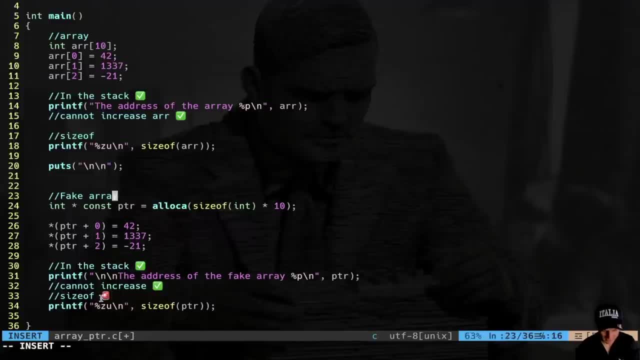 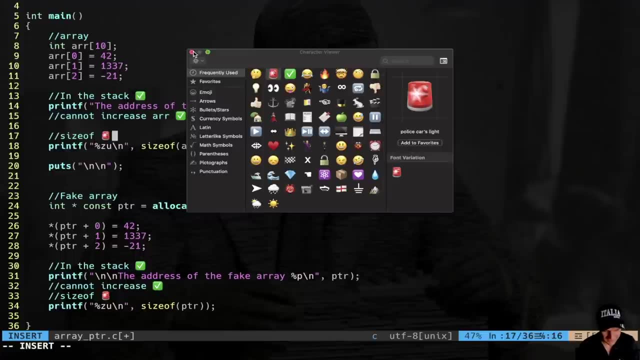 Depending on the machine. in my machine is eight bites. On the contrary, when I call here size off on the array, what is happening? Well, I am getting the size of the entire array. I'm not getting the size of a pointer. 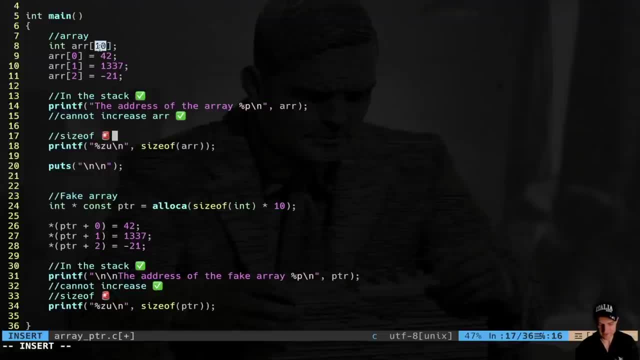 You see the catch and get in size off array, which is 10 per four, because this is the size of all the objects. So I have an object in memory which is 40 bites. Here I have a pointer: I don't have an object of 40 bytes. 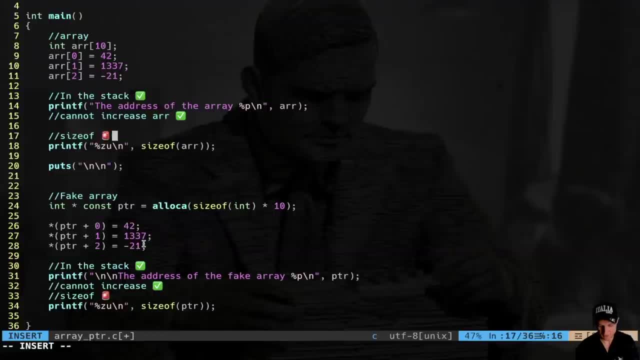 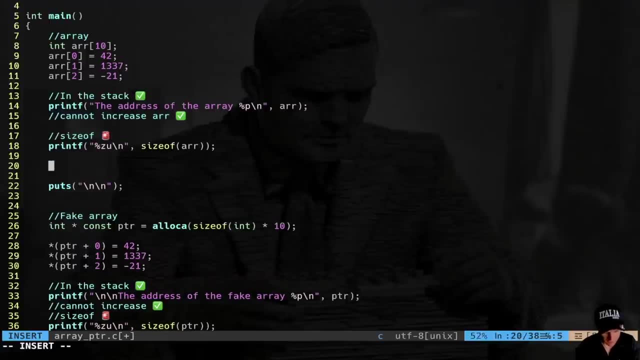 I have a pointer And uh, in every location in my stack I'm going to put manually all these values. I see this is a big difference already. Now let's try uh with another operator, which is uh, the ampersand operator. 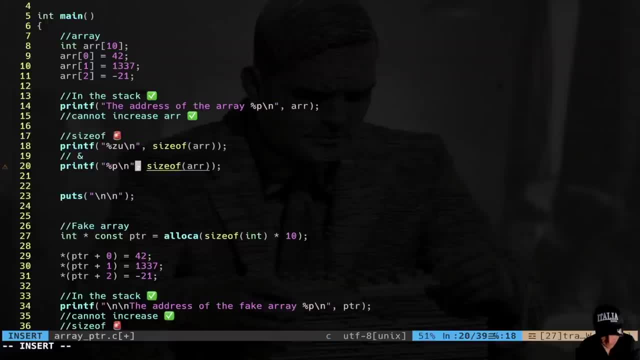 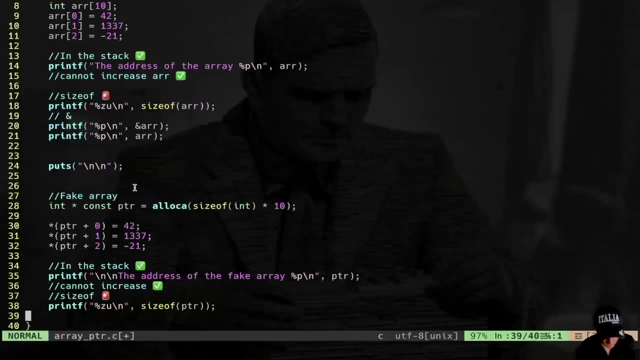 So I'm going to copy this, I'm going to print a pointer to the address of array and then, just beneath, I'm going to do a pointer to array. So I want to do the same operation with my fake array. So, using the ampersand, I'm going to do print. 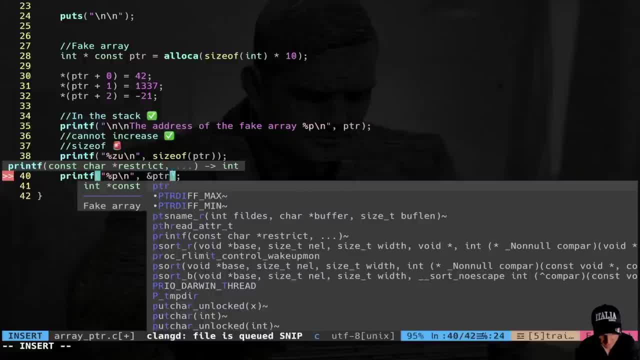 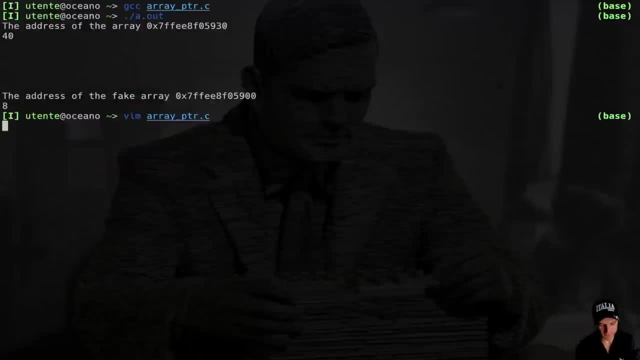 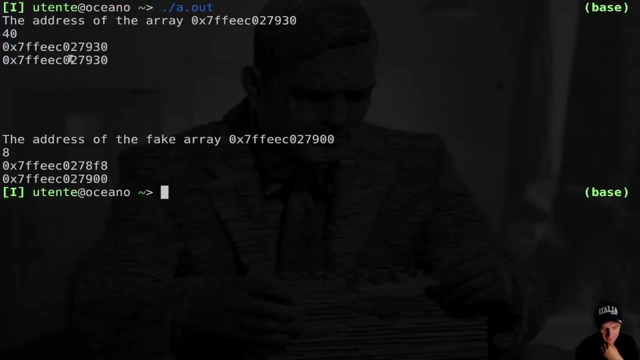 In-step percent P. Uh, so the address of PTR and as well PTR by himself. Why didn't it happen here, my friend, let's watch carefully, compile and just launch. You see something peculiar with the array: I get the same address both when I use the ampersand year. 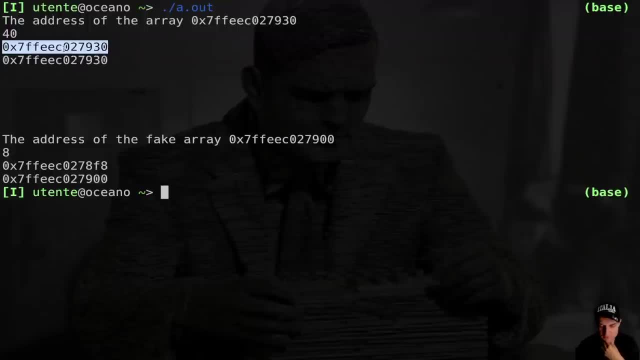 And when I don't use it. these are the same pointer, the same address, but they are of different types. here I have a pointer to array type. in this case I have a pointer to an array of 10 integers. and here I just have. 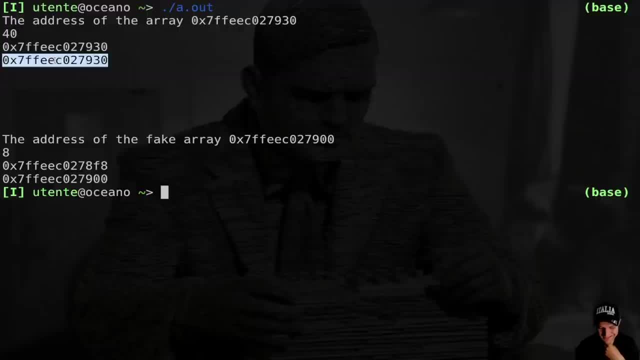 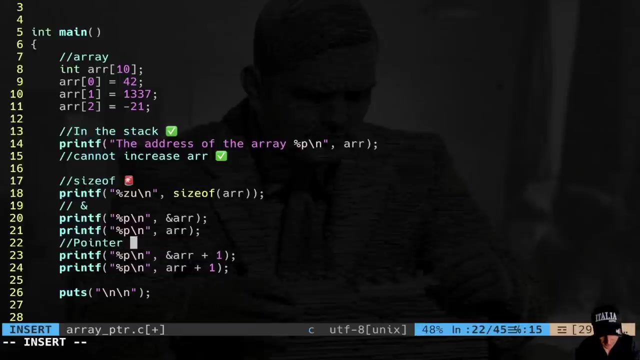 a normal pointer to an integer. so they of course point to the same memory location, but they have a different type. what does it mean? well, it means that if I perform pointer arithmetic with this, I get a different result, respecting to this one. let's try. so I'm gonna do that pointer arithmetic, and this time as you. 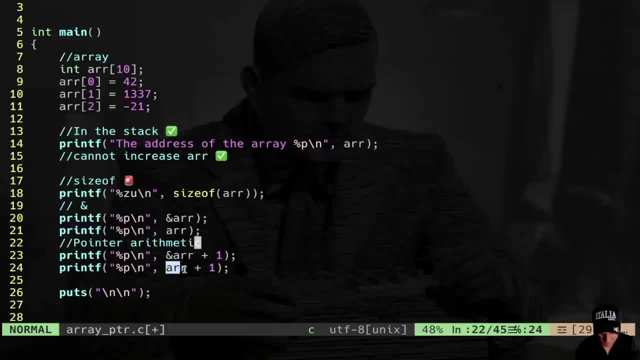 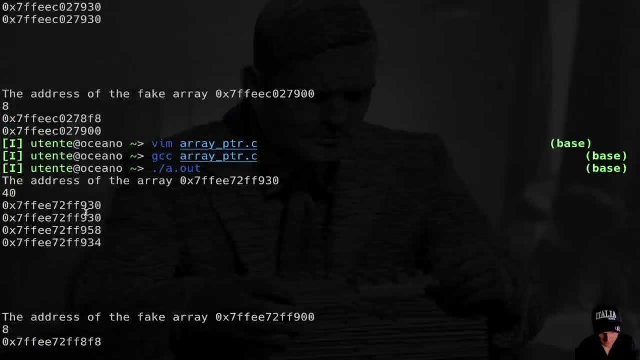 can see I'm doing pointer arithmetic to this pointer and to this pointer which you just saw. they are the same. let's try out gonna compile a launch. look at that, my friend. what do you see? they, of course, point out the same address. but when I perform a plus one, I don't advanced equally here, I only advance for a. 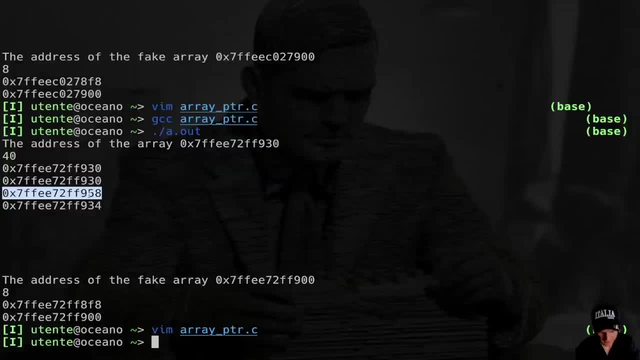 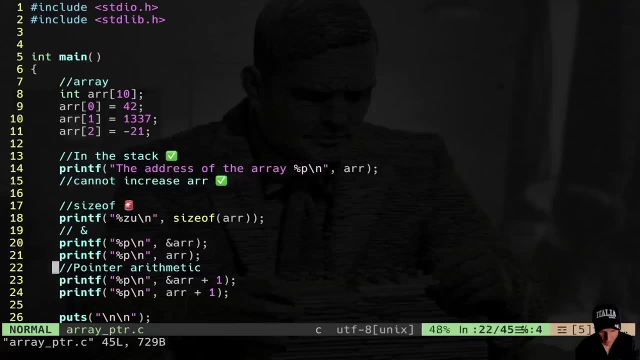 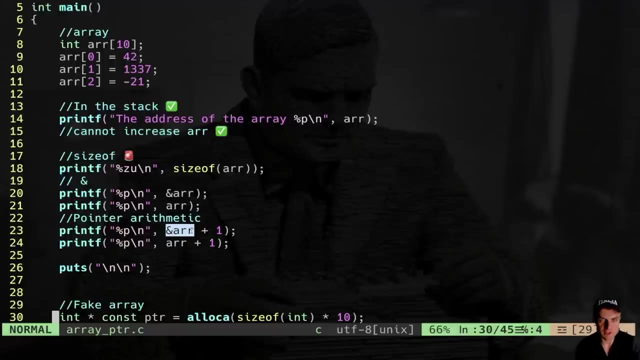 position. on the contrary, here I advance much more. indeed, here I jumped one array position. this is of course hexadecimal notation, so pay attention to that. so when I do this, I'm going to do a pointer arithmetic to this pointer I'm going to, I use the ampersand on the name of the array. I get a pointer which is of a. 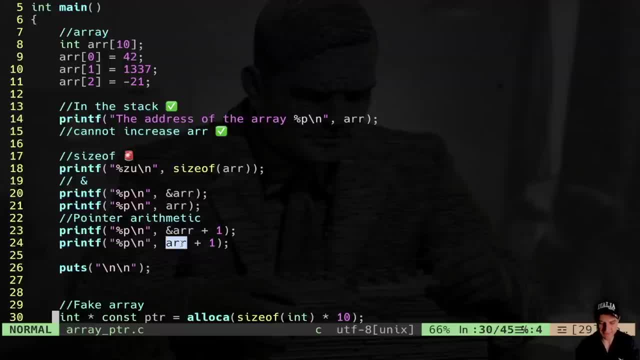 different type, respecting to this name of the array alone. so I get a different pointer arithmetic. you recall from the previous videos I told you that the data type of the pointer is going to imply the way by which we read data in the respective memory pointed and the pointer arithmetic itself. this is what is. 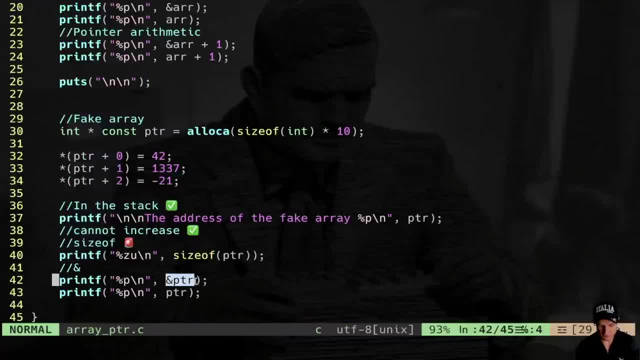 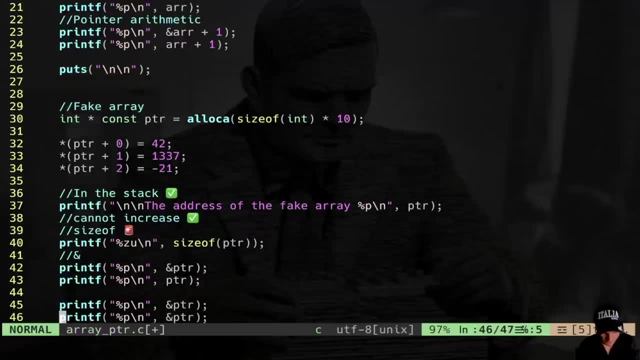 happening. on the contrary, Here what do I have? I have a pointer to a pointer, and here I have a simple pointer. So if I do the same trick, So I'm gonna do this and that, and here I'm gonna say plus one, and here plus one. 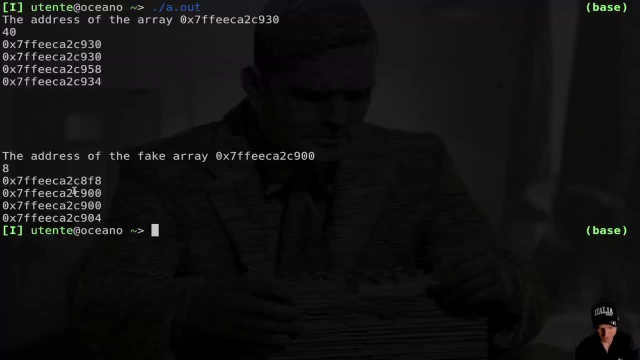 What is going to happen? Compile So I get those results. So this is the address of the pointer. This is the pointer itself. This is the address of the pointer plus one. and this is the pointer plus one. Of course, this is not very well written. I should have written the output better, but 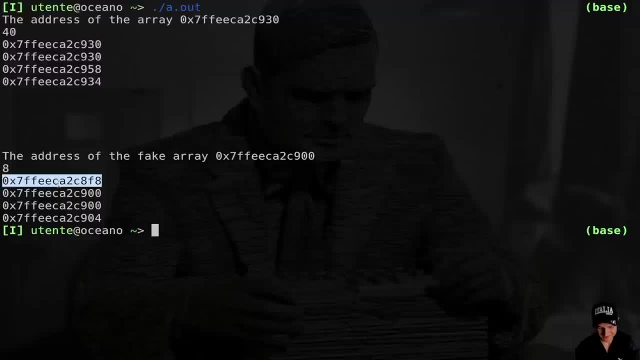 but you get the point. I guess This is the address of the pointer. When I say pointer plus one, I jump. here I jump eight because a pointer is eight bytes. Here, on the contrary, I say pointer plus one, I jump four because an integer is four bytes. So let's not dig too much into this technical. 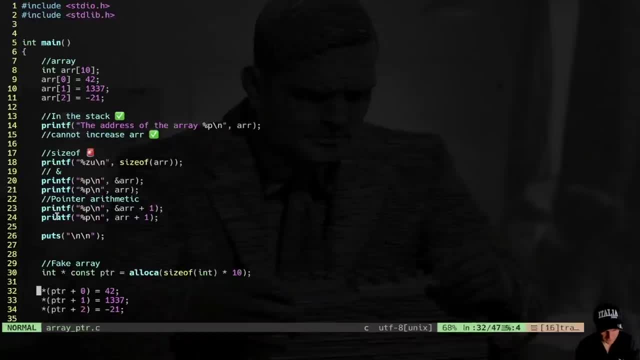 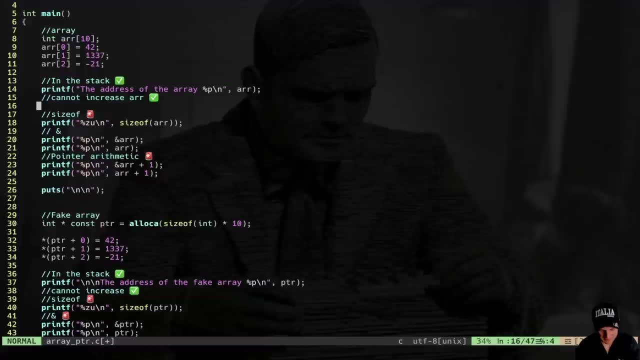 stuff, which is not easy, and let's understand the overall idea. So I have these two objects, an array and a fake quote-unquote array that I created. They are basically the same. They both allocate memory In the stack. this is happening because this is an array. You know how it works, You have a location. 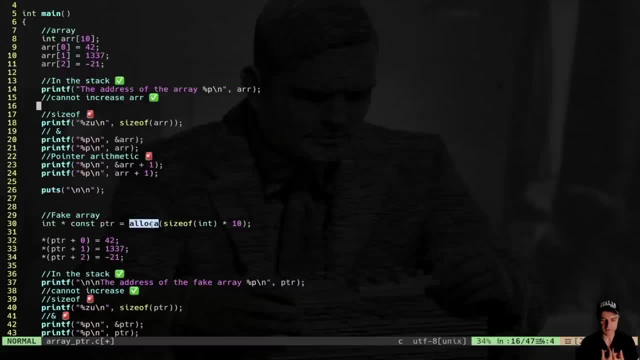 in memory. Here, on the contrary, I perform myself the allocation using this function, which is not suggested, but that's how it works. So it's gonna allocate 40 bytes in the stack. This is a constant pointer to an integer, Almost like this. So both are in the stack. Okay, I cannot increase array as 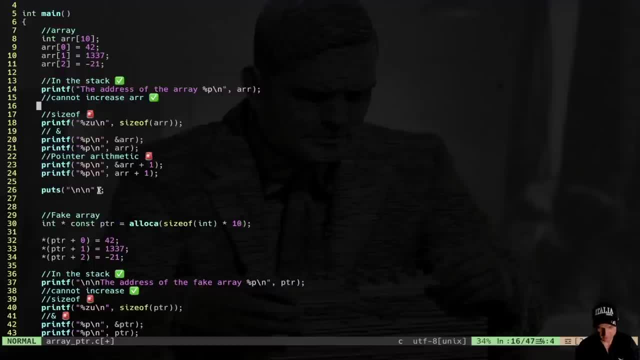 well, as I cannot increase ptr because this is a constant. The difference is that when I use size of, I'm gonna get the size of all the object, of all the array. When I use size of on my pointer, I get the size of my pointer, because this is just a pointer. When I use the ampersand, I get the address. 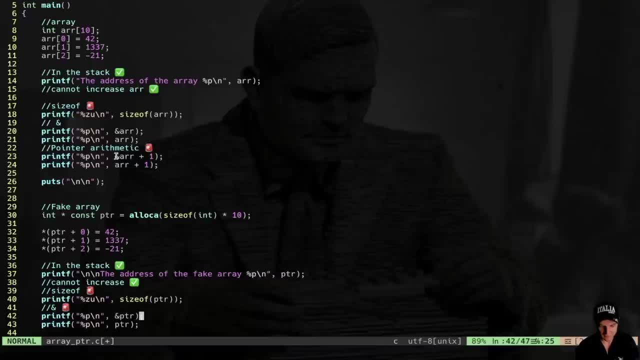 of the pointer. On the contrary, when I use the ampersand on an array, I get the address of the array that's typed. So I get a pointer of a specific data type. In this case, I get an address to an array int 10.. So we get these. 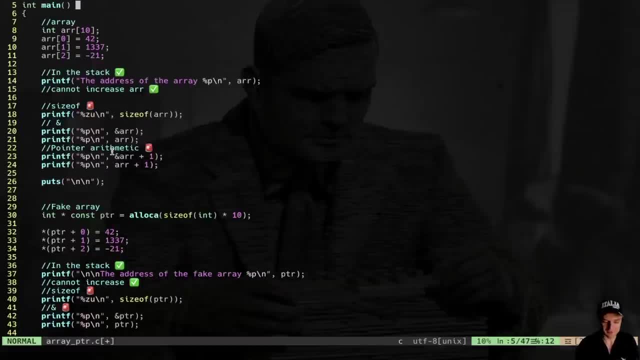 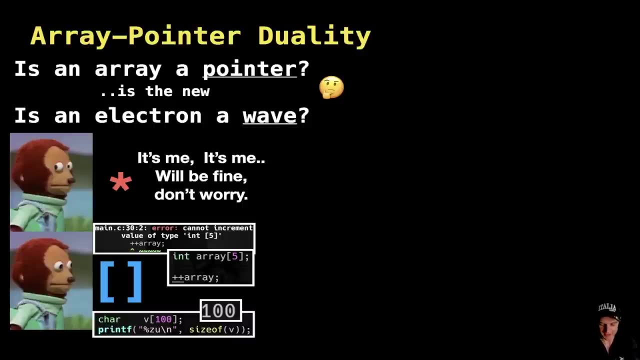 things which are not equal. And now let's understand why. Let's understand what is going on. We have this array, pointer duality. The best analogy that comes to my mind is the wave particle duality right of quantum mechanics. We don't actually know if a particle is a wave or a. 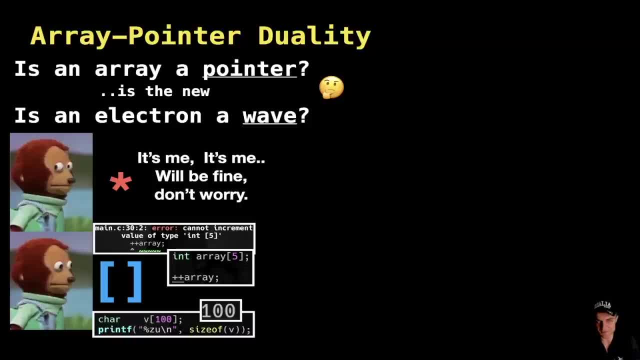 particle, because sometimes it behaves like a particle, Sometimes it behaves like a wave, and that's all confusing. So in the same way we have arrays and pointers. Sometimes they are arrays when I use the size of operation. Sometimes they are arrays when I use the size of operation. 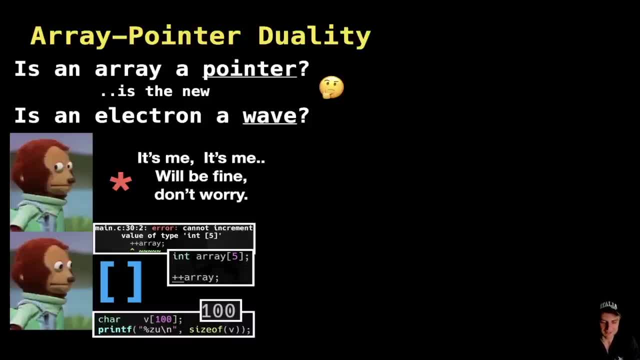 And sometimes they are just pointers. when I just dereference the first element, It is just a pointer at the end of the day. So this is confusing. Indeed, my friend, there is this phenomenon which is called array decay, in which the array, basically, is a pointer You can perceive. 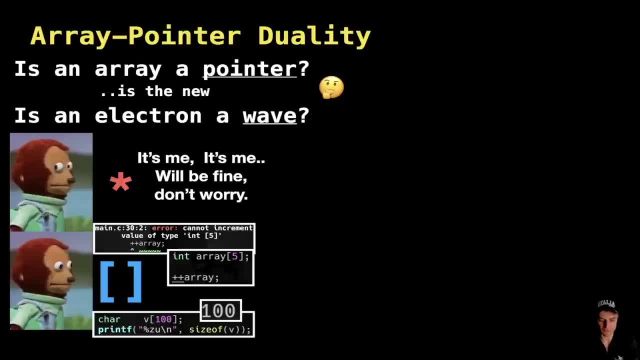 the array as a pointer, And this is the message I want to convey to you. We don't want to get bogged down into technical details, We just want to write code. So my suggestion to you is that when you work with an array identifier- much probably that is just a pointer to the first- 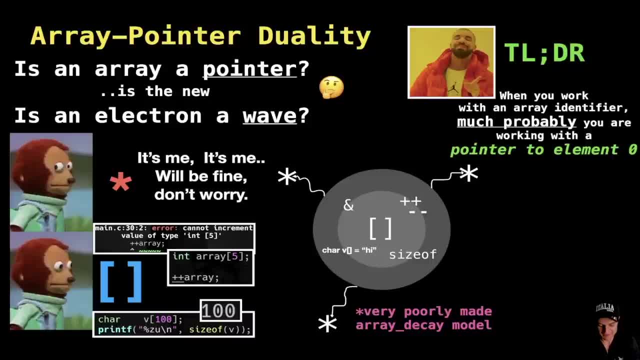 element Here. I just created this stupid model, standard model of arrays and pointers, by which we have an array that always decays into a pointer to the first element, but not in all situations, For example, when we want to increment the name of the array you just saw. we cannot do. 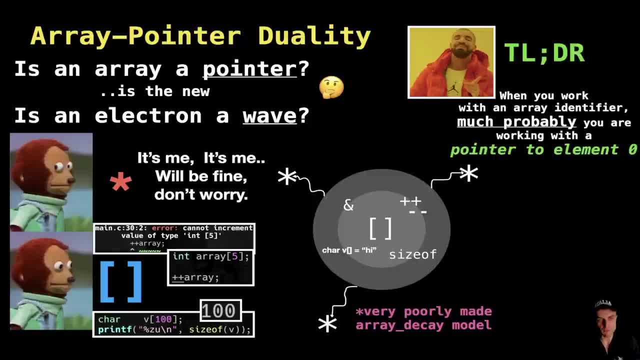 that We cannot increase the name of an array. When we use the ampersand operator with an array, we get the address of the array that's typed. We don't get an address of a pointer. We get an address that has a specific type. that is the type of the array: Int, array 10 in the case. 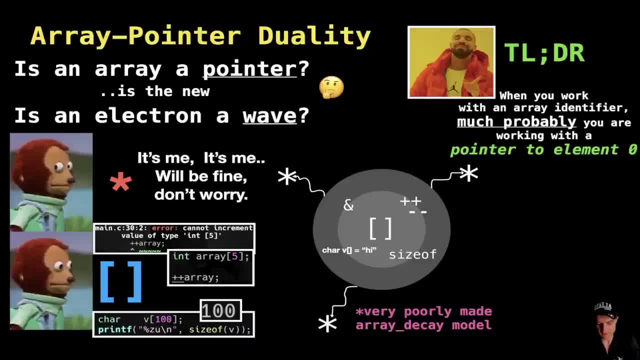 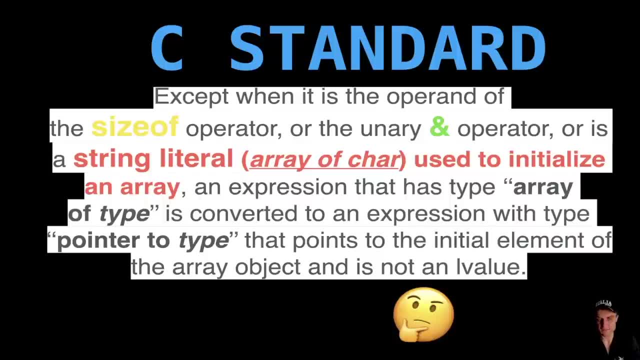 before. So it's kind of tricky right. This array decaying is kind of a tricky beast to master. Now let's see what is written in the C standard. So, except when I use the size of operand or the initialize an array, an expression that has type, array of type, we have a conversion to an expression. 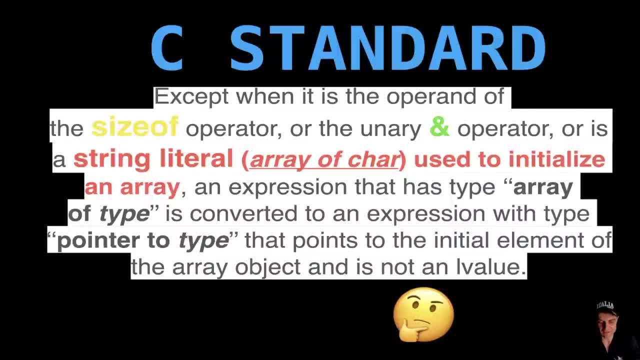 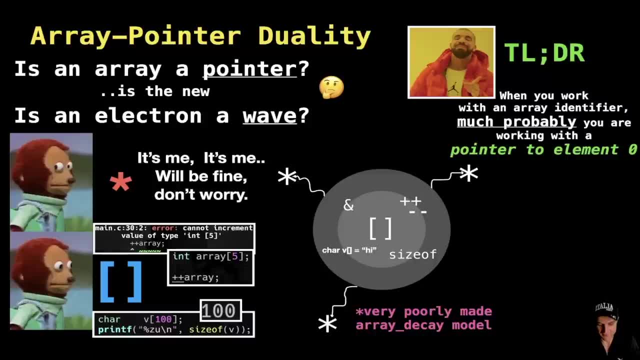 of pointer to type. So the array is decaying into a pointer that points to the initial element of the array. Okay, so this is essentially what is happening. Keep in mind the stupid model I've created, because I think it's fairly useful. It gives you the idea of what is going on. So let's. 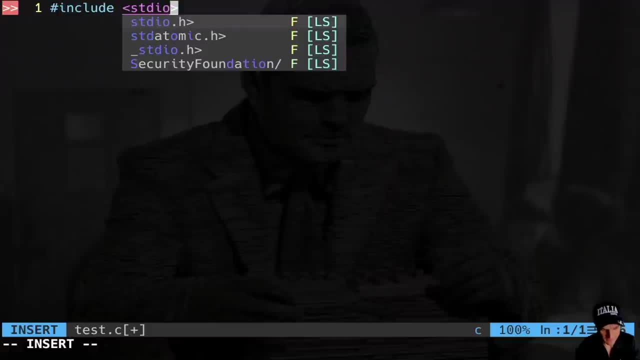 write together a little piece of code so we can understand better this idea. So, as usual, my main function at the top and then I create an array of 10 elements to integer, like always. So I know that every time the array identifier is going to decay into a pointer to the first element, but not. 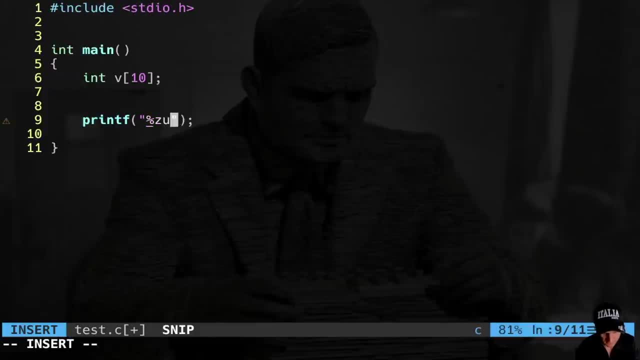 always Like: if I do printf- you saw before zoo size of v. we don't have a decay Here. the value is going to be 40 and not 8, right? But if I do something like that, I do ptr and then I do ptr. 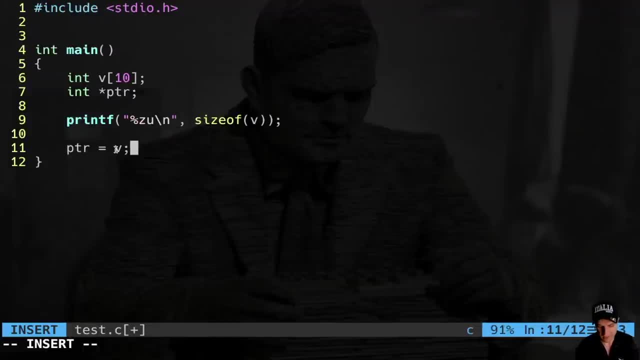 is equal to ptr. What is happening here? Well, I'm not assigning an array to the pointer, I'm assigning a pointer to the first element. You see. So here, if I say v in position 0 is equal to 42. Here I can see that. 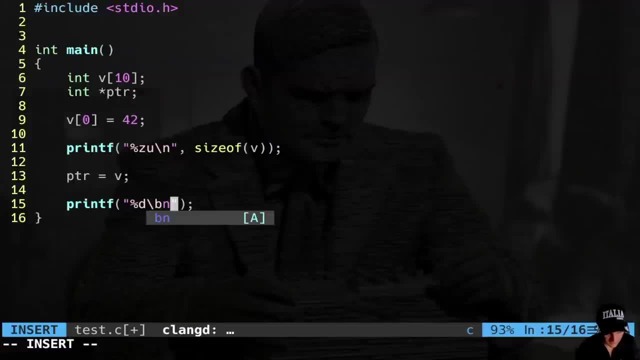 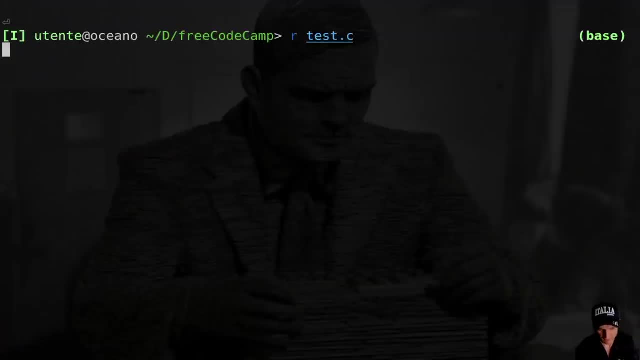 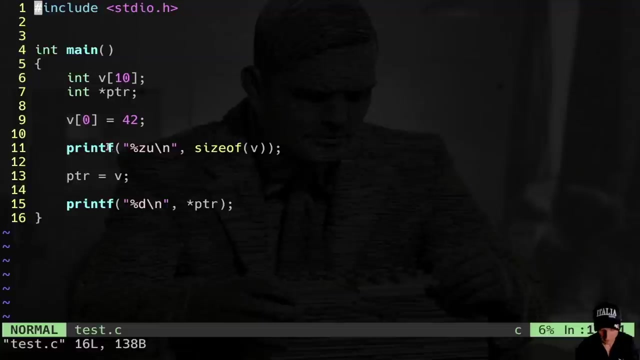 value, just with the printf, and I say: at ptr, This is exactly the same right? So I'm gonna run, As you can see. this is the size of the object and this is the element in the first position Accessed through the pointer. See, Because here I have a decay, Here I don't have a decay. Why? 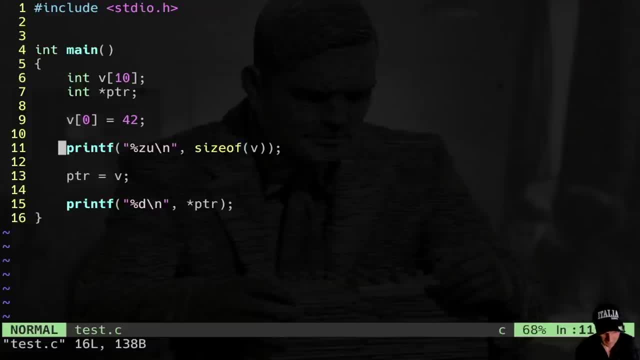 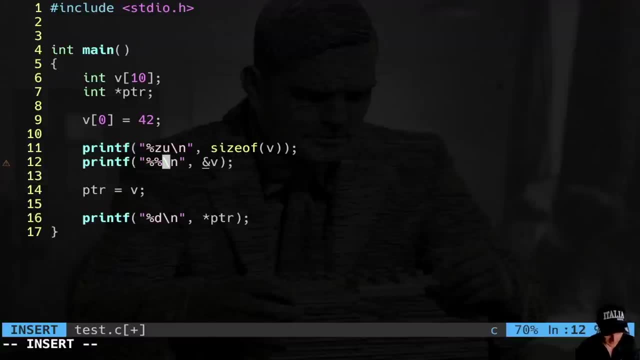 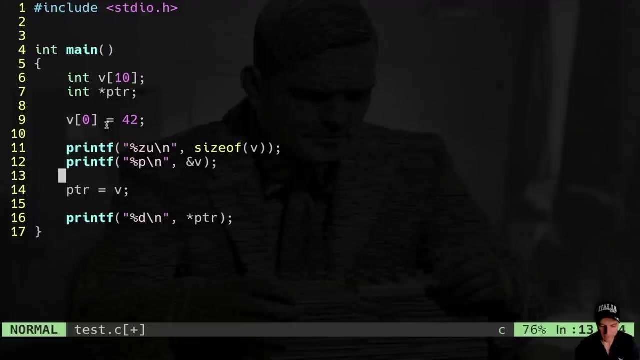 Because I'm using the sizeof operator, So the decay as well doesn't hold if I'm using the ampersand operator You saw before, So I just remove this. Here I'm getting the address of the array, which is equal to the pointer to the first element, but is of a different type. This is the key difference. 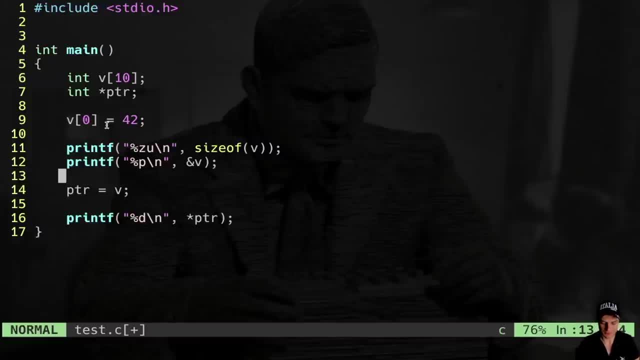 And basically that's it. I don't want to give you too many details because at a certain point, you don't need to stress out too much. When you work with arrays, you have an object allocated in the stack and this is different from a pointer, An. 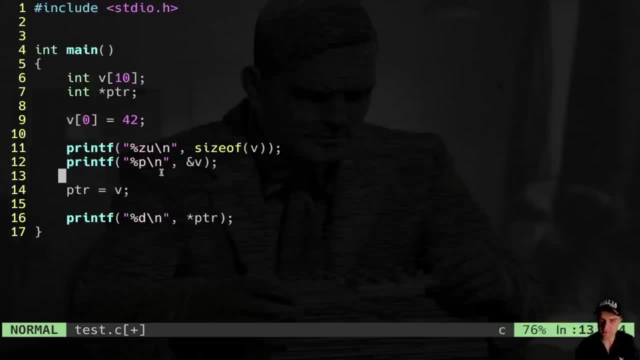 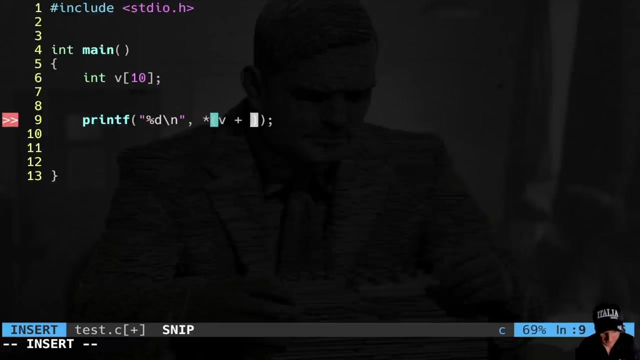 array is not a pointer. The trick is that very often an array decays into a pointer, So we can basically consider an array like a pointer. The thing is so intertwined that basically I can use pointer notation like that to access elements inside My array. I want the object at position v plus one. Okay, So I'm gonna do: v1 is equal to 42. 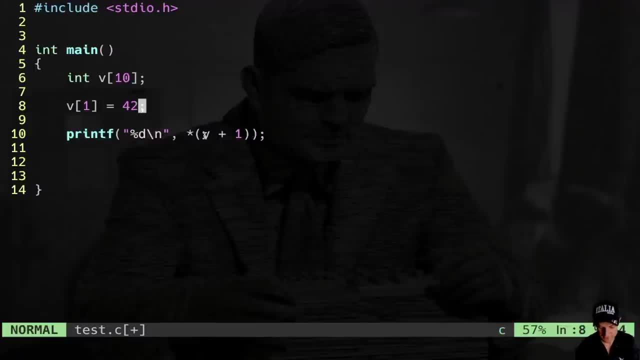 But I access with pointer notation. Why? Well, because this is a pointer, My friend, This is a pointer, So I'm gonna run, That's the same, You see. So what is, at the end of the day, the difference between array accessing in this fashion or in this fashion, Like that? Well, there is no. 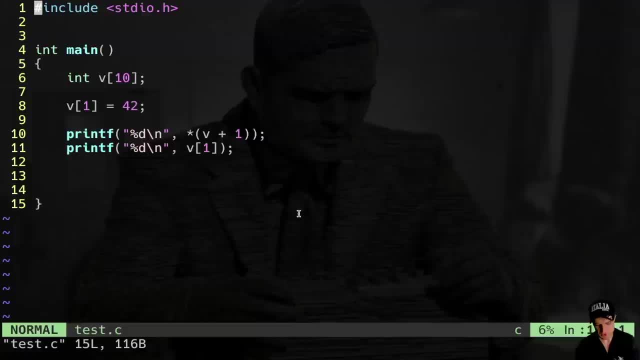 difference. indeed, They are the same. The square bracket notation at the end of the day is just syntactic sugar. It is easier to perceive what is going on with this way of typing, But underneath the hood, what is happening is that we get the reference of a pointer. 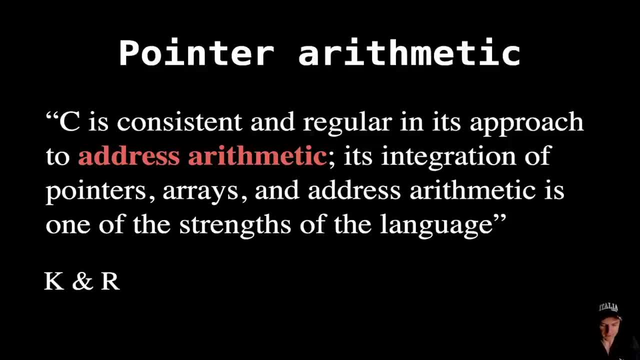 You see, Coming back to a previous principle that I explained in a previous video, We have C, which is consistent and regular in its approach to address arithmetic. Right Its integration of pointers, arrays and address arithmetic is one of the strengths of the language. That's why pointer 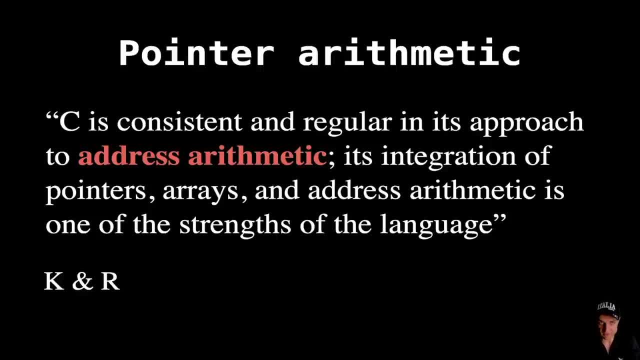 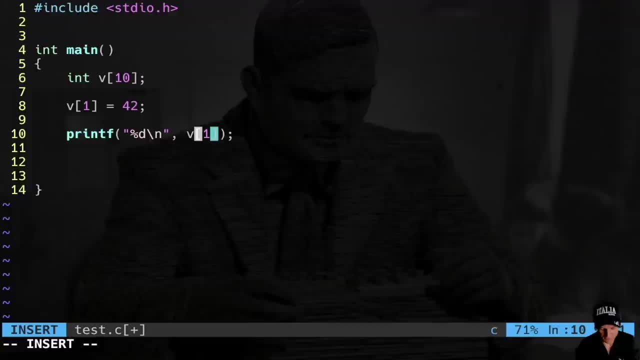 index works the way it works. It's basically array indexing Right. When I increase by one, I'm pointer to a short. I'm increasing by two positions because I want to access the following short, The following object. So when the compiler sees this v square bracket one, what is happening? 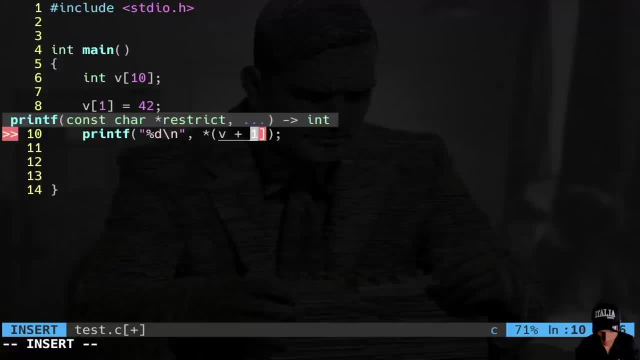 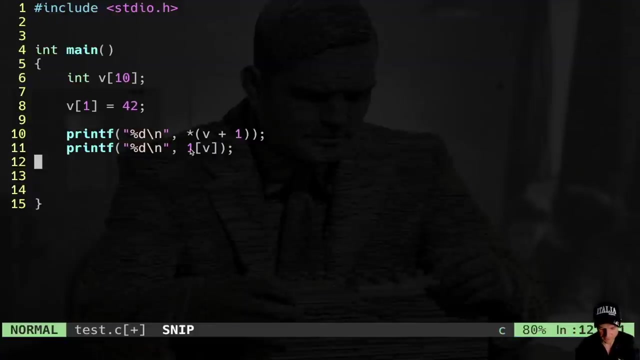 is that it converts this to that. Okay Plus one, So we can do something really murky. now We can do that. We can do printf The same, But this time I'm gonna do one in position v. Oh my god, Do you think it's gonna work? 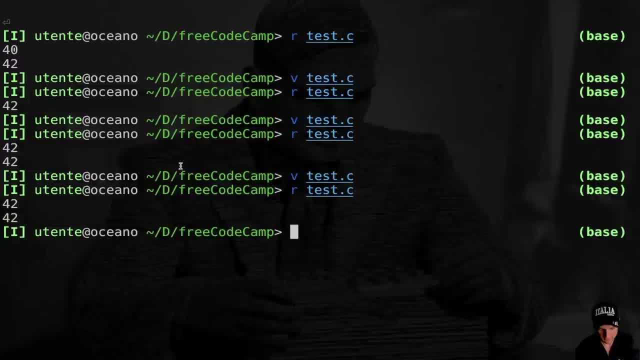 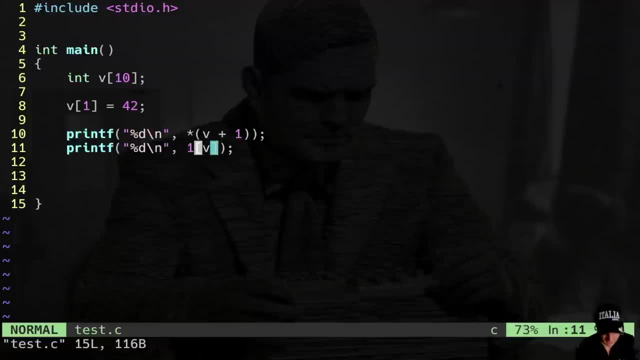 One in position v. This doesn't make any sense, but let's try. Well, you see, it works as well, because what is this thing here? At the end of the day, the compiler is gonna translate this into this, So it's the same. Right At the end of the day, this is commutative. This is the same thing, So we can. 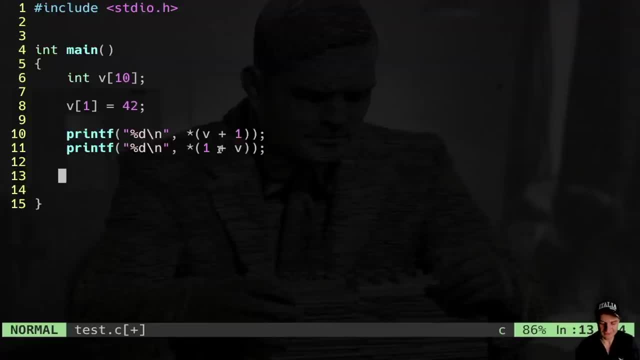 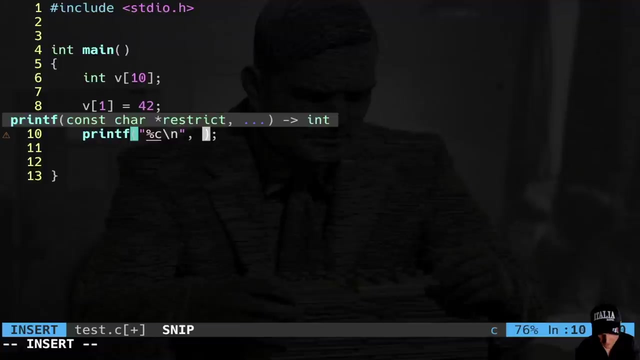 do really strange stuff because at the end we have the referencing of a pointer. Now let me show you other quirks, just to have fun, not to learn this stuff, because it's very bad programming. But you can do printf, for example the char in a string literal, In a string literal that: 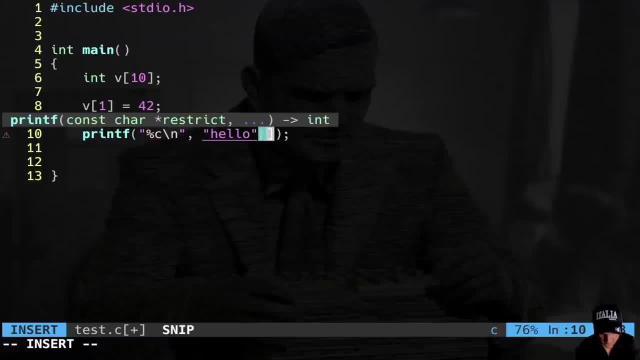 it is an array of char in C. So I do hello and I take the one in position three. or let's do the one in position zero. Let's take the h. Do you think it's gonna work? Let's run. So it's gonna give me back the h because this string, literal, is an array. 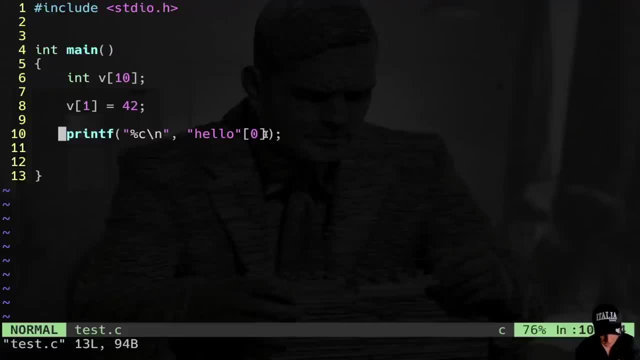 Underneath the wood, And this is array indexing. But I told you that this is just like pointer dereferencing, So we can do this. Okay, let's try. As you can see, I get two h's The same, Or I can do something like that At two, And it's gonna be so bad to see. This is gonna give me back. 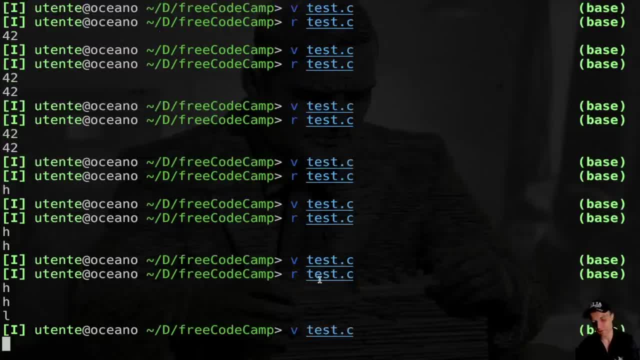 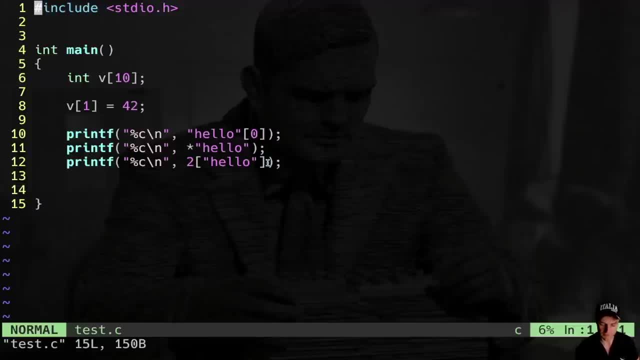 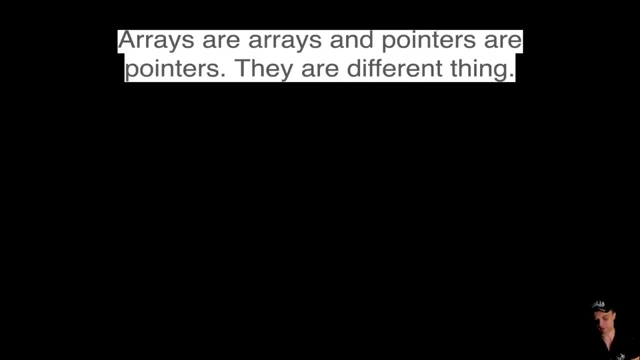 an l Hhl. as you can see Right Now, you understood the trick right. We don't have to go any deeper. We can do super strange stuff given the nature of reality in C. So the message I want to convey to you is that arrays are arrays And pointers are pointers. 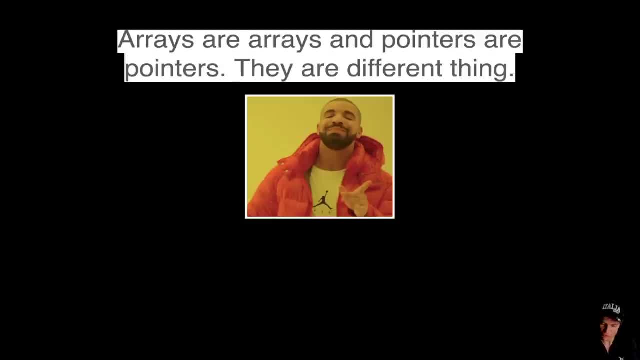 They are indeed different things, But, as Drake is telling us, To Drake, that's just a pointer. End of the story. Be Drake, Be cool, Because when you're working with arrays, Unless you're using the sizeof operator or the ampersand operator or so forth, You are handling a pointer. 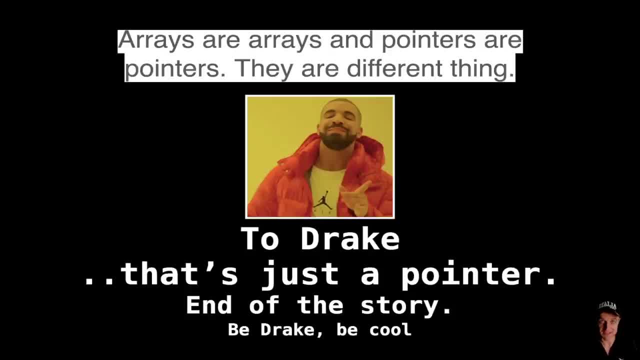 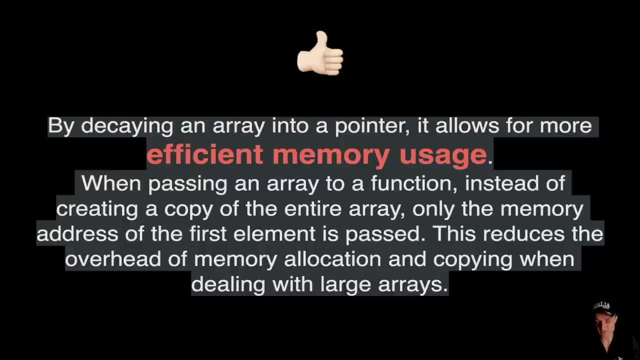 to the first element. So in your mind you can think: Okay, this is a pointer to the first element, End of the story. So now let's try to respond to some questions, And the first one is: Why is this array decay? Well, it's fairly simple, right? If you reach this level of the course, You know that when 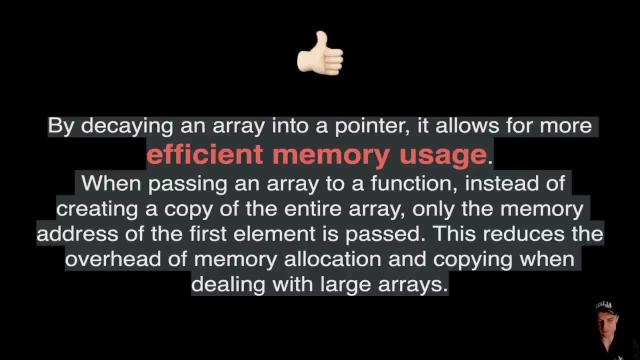 an object is decaying to a pointer, We have a reference to it. So let's pretend we have a very, very big array And we are passing to a function. Well, we are not passing a copy, So the function doesn't have to copy all the the thing, But it just have a reference to it. So it's efficient. 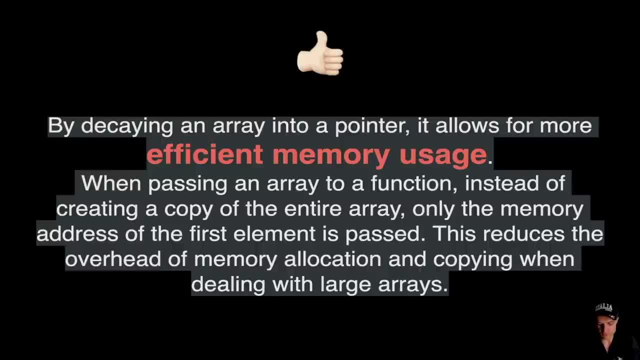 In memory usage When passing an array to a function, Instead of creating copying. So when passing an array to a function, We are not creating a big copy And this improves performance overall. Right, So you see this little stupid program. I have my main Inside my main. I'm going to declare: 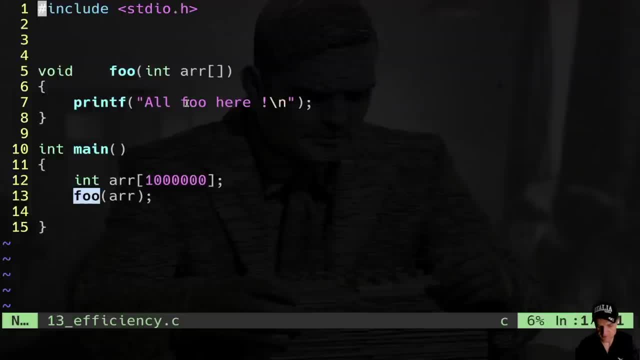 a big array. And then I pass to foo. Foo is going to receive just a pointer, Even though here I write a square bracket, This is a pointer. When I write a square bracket I just say, Hey, keep in mind that main, I have an array and not a pointer. But they are the same, Right, You can do like that or like. 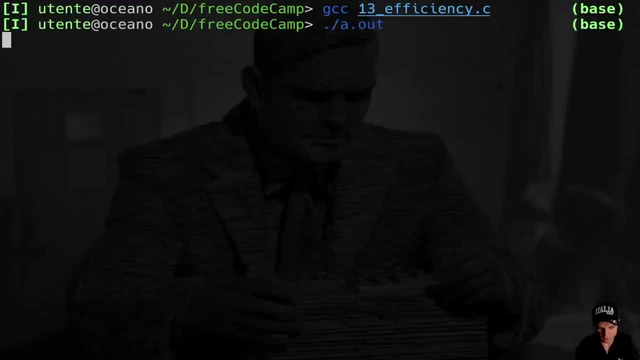 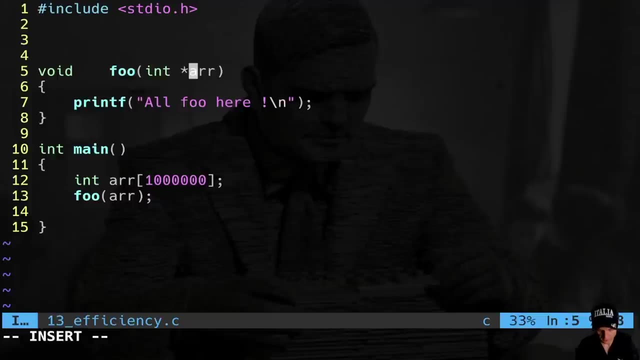 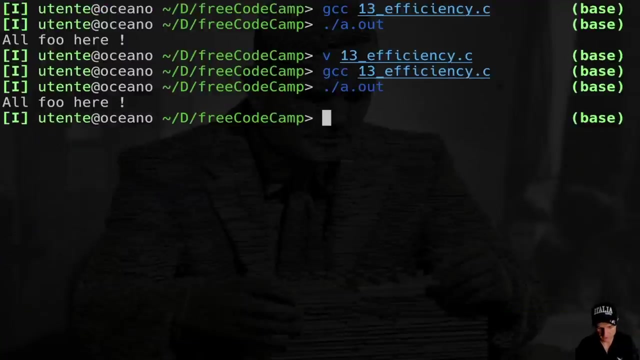 that. So the foo function is going to receive only a pointer to the array. It's not going to receive a copy of that. It's not going to copy all the array in its local frame. Of course. here I can write in these two fashions: It's totally the same. So I compile and launch. You see Cool. 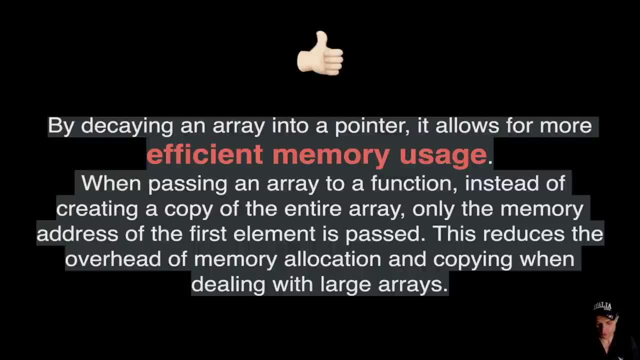 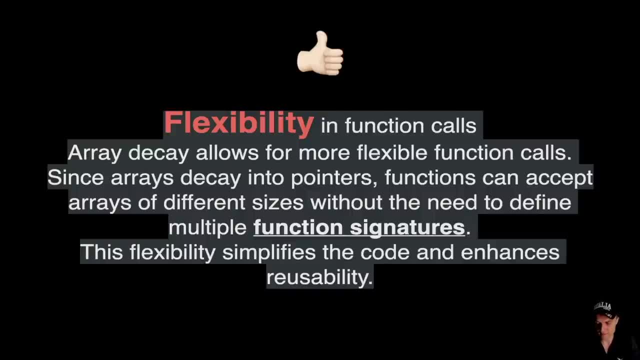 So having this decay is going to improve your memory usage. This is flexible, Of course, Because every array has a specific data type. I can have, in the examples of before I have: array int 10.. Array int 15.. Array double 30. You know. So for every array I would need an adoc. 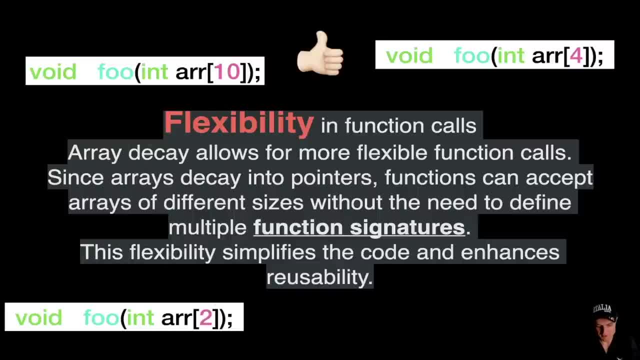 function. I don't want to have many, many functions that are dealing with specific array types. I have an array that is decaying to a pointer, So a pointer is a pointer, So I can have a generic function that is able to perform a specific function. So I can have a generic function that is able to. 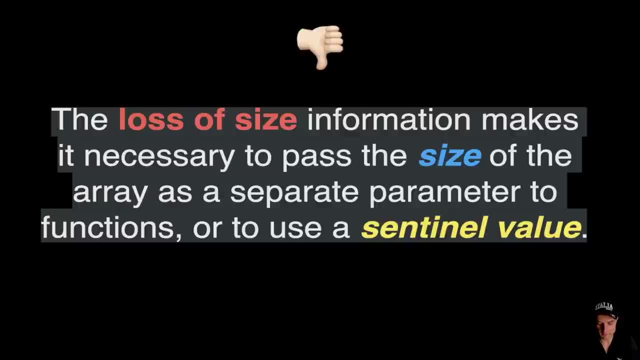 perform its operation to every kind of array. The bad part is that I have loss of size information. Basically, when I pass an array to a function, I don't know anymore how big is this array. So I need all the time to bring with me an anchor value which is the size right Every time I call a. 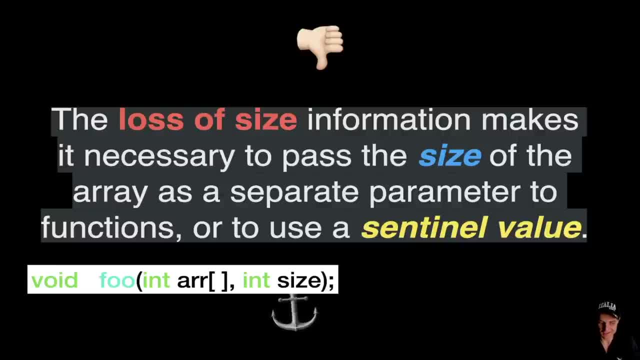 function. I have this cumbersome size that I need to pass, Or I can use a sentinel value, For example, interleaved inside the values in my array. I can have a value, for example a negative value. given that my array has only positive values, that is will apply as a. 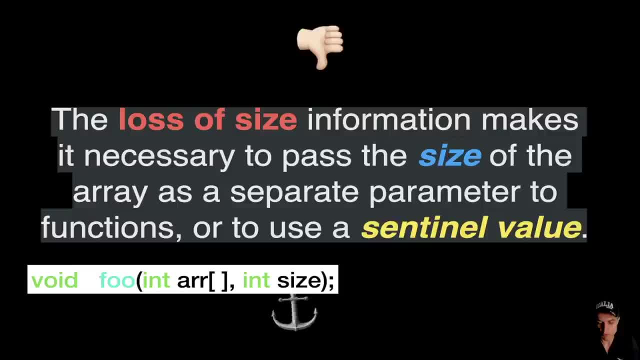 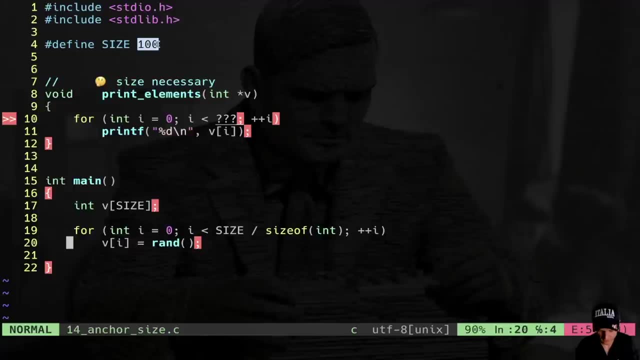 sentinel value. But you know you have to engineer a way to communicate to the cool function that this is an array of a specific type. What is the deal here? Let's try with the code to explain why this is important. You see, here I have my little code with the symbol in constant with the value. 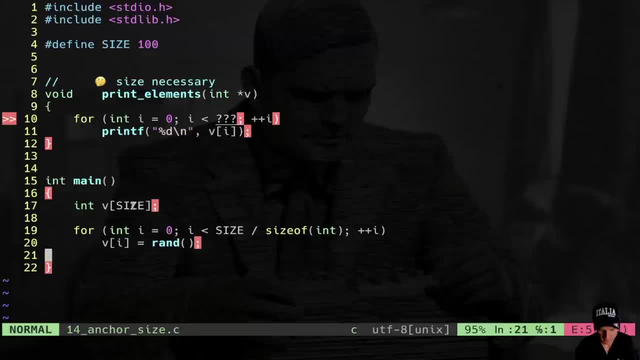 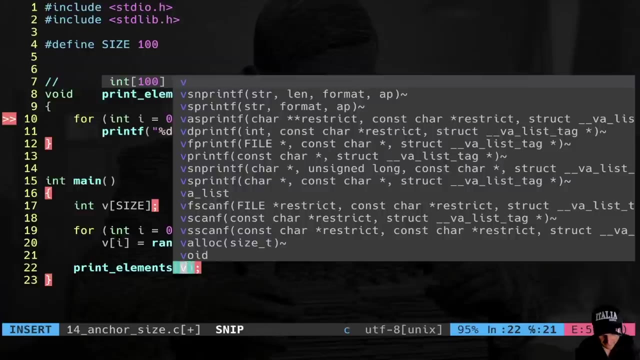 100. Size symbol in constant. So I create my array which has 100 elements. Then I go to populate my array with random values. Then I want to call my function, which is printElements, and I give as an input my array v. okay, Now printElements would like to. 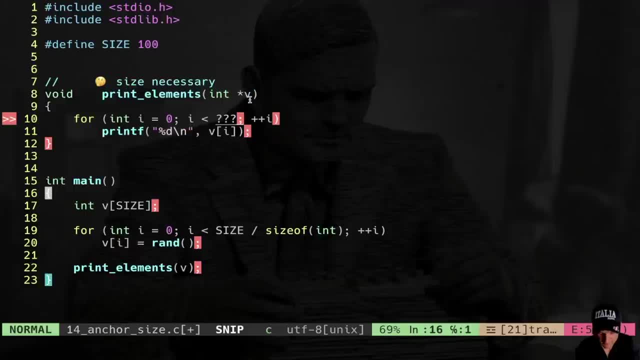 print the values inside my array, all the values. but it doesn't know how, You see, Because I have my for loop which has the exit condition when i is minor than what, Given that v. here is only a pointer. You see The catch. So here I need to pass a function which is going to give me a value. 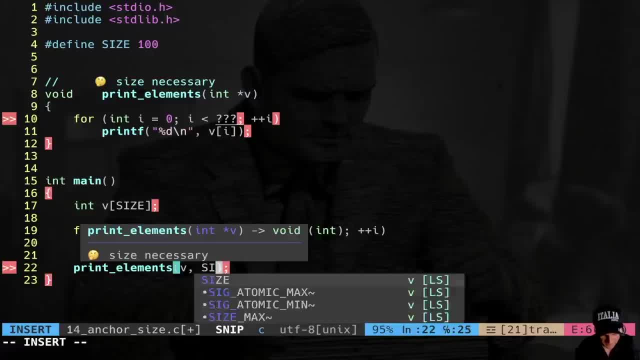 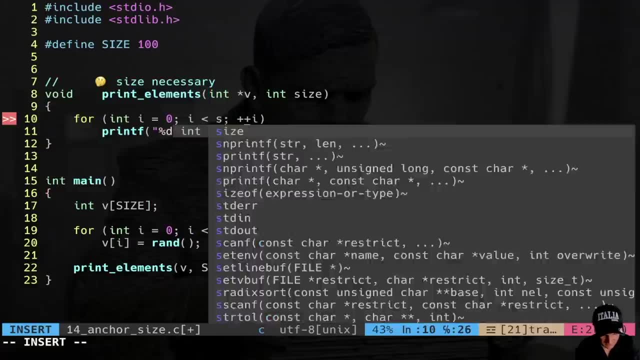 So I'm going to pass the size, so we are going to pass size, and here I'm going to put int size, okay, So here I do is minor, then size. Now we can work. you see, To make it crystal clear If I do printf. 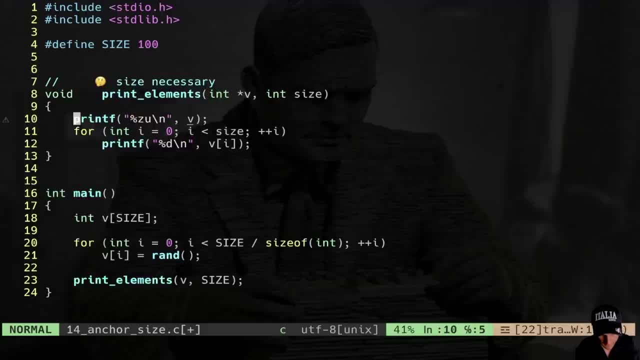 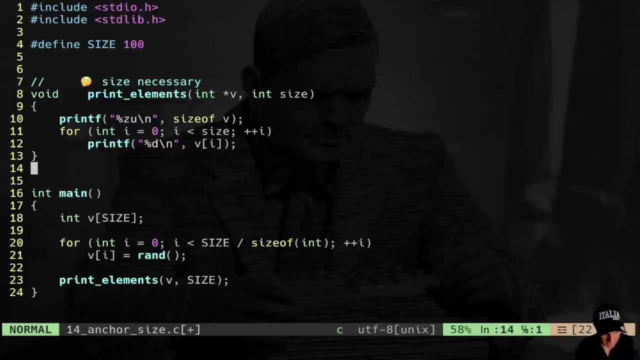 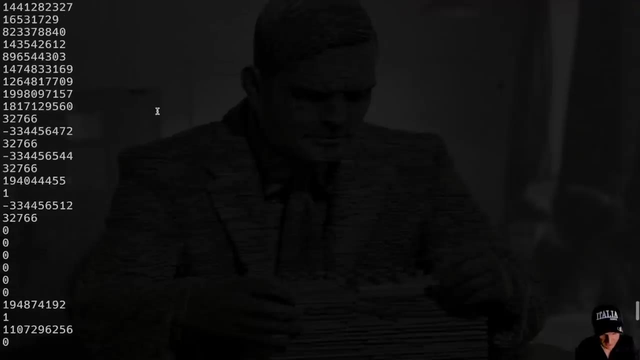 zoo of v. here I'm. I'm going to get um like that size of v. Here I'm going to get 8 and not the size 100.. So let's run this code and let's try to see how it works. what is going on? 14 anchor size, and here i have all the random values which are inside my array. 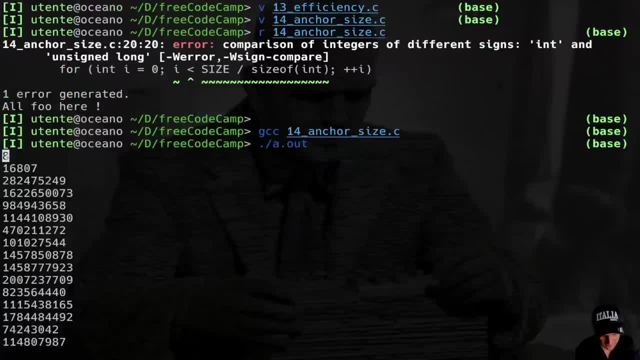 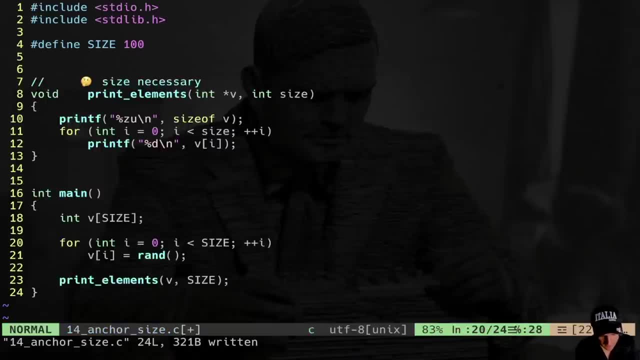 the first one, of course, is the value 8, which is the size of the pointer received. here there is a little mistake. there shouldn't be size off of int. so let's try to launch again. and then here i want to tweak a little bit the code to make it more readable. let's do modulo. 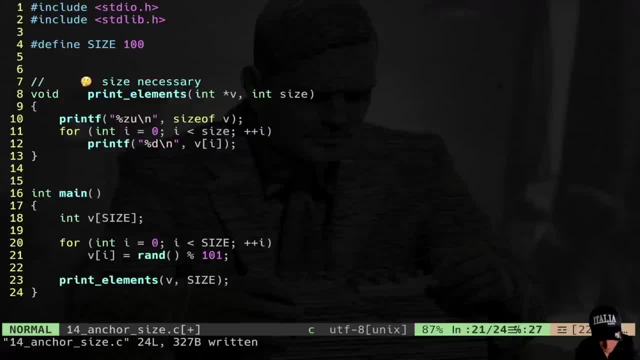 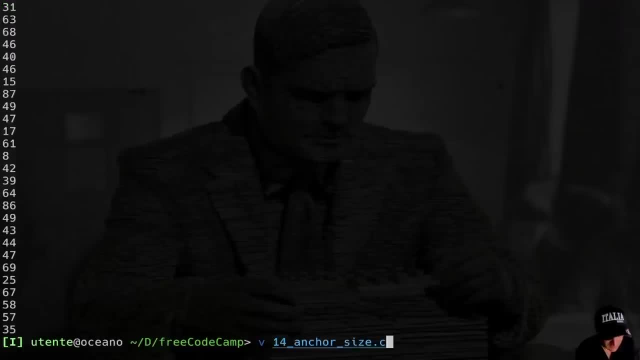 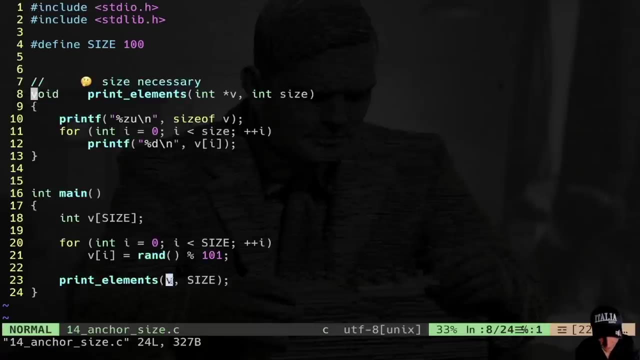 101. so i have numbers ranging from 0 to 100 by launch. okay, now i have all the numbers that i want and here at the beginning of my eight, which is the size of the pointer, basically the name of the array that, at this level, has decayed into a pointer. so i guess you understand what. 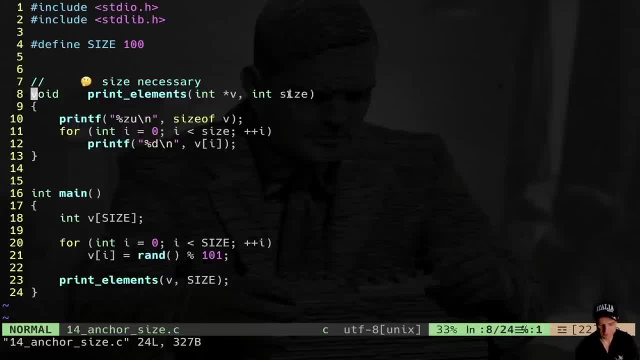 is going on. okay, all the times i need to bring with me this size, uh value, otherwise the code function doesn't really know how big the array is. so, like all the things, we have pros and cons, trade-offs. now the the question that you just saw before, so i'm 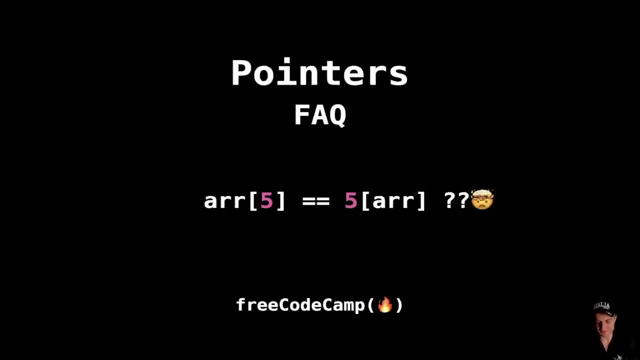 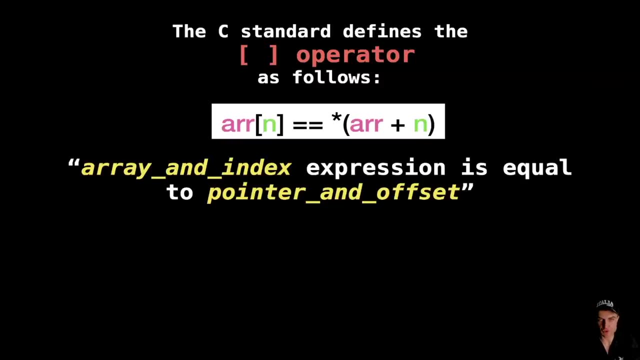 not going to repeat why array index five is equal to five index array. You know because at the end of the day we are dereferencing a pointer. So very shortly, the C standard defines the square bracket operator, like the referencing right. 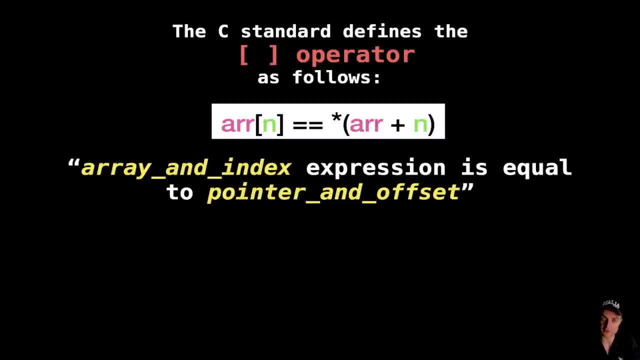 So array and index expression is equal to pointer and offset. That's totally the same. So if I say array five, I'm saying at array plus five, And if I say five array, I'm saying at five plus arrays. So you see, I'm just inverting the values. 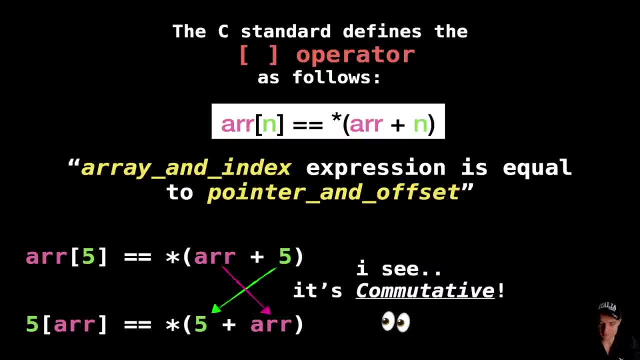 and, of course, this is commutative and that's no problem at all, But you understand this idea right? Okay, we are finished with this duality array and pointers. I tried to explain as the best as I can, but I understand that this is tricky. 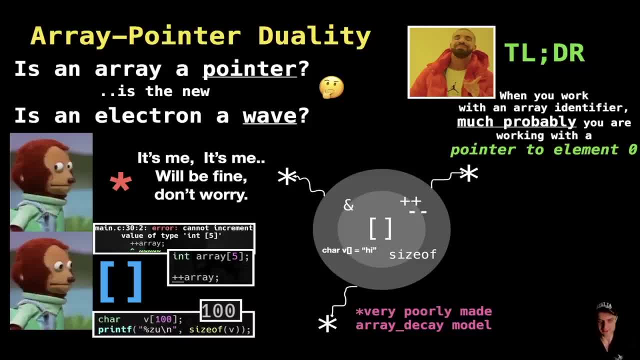 This is tricky. Keep in mind this idea: An array is an array, but most probably it's gonna decay into a pointer to its first element. So you have this standard model of array and pointers by which an array is just a pointer in your mind. 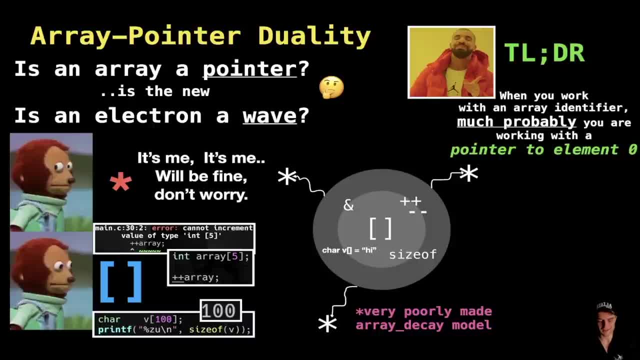 And, believe me, every time I write code, I think I basically forget that an array is an array at the end of the day. So for any practical purpose, they are the same. Now, pedantically speaking, you understand that they are not. 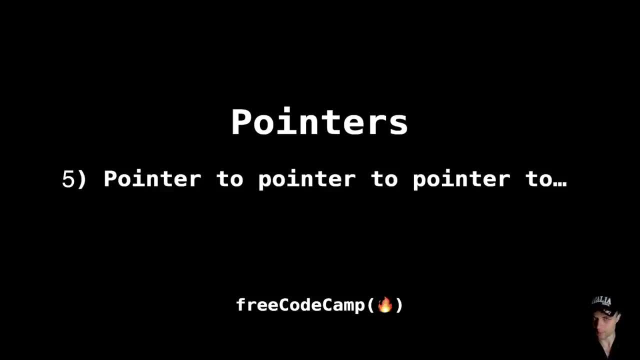 Okay, my friend, now we understood all the big principles related to pointers. Now we go a little deeper, So we're gonna do now pointers to pointers, to pointers to pointers and so forth. right, We are gonna understand how these work, okay. 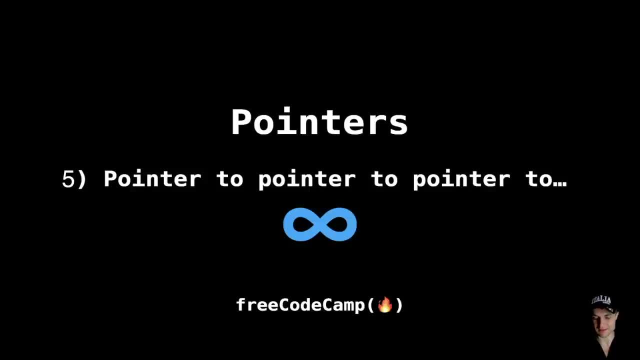 The thing is that, basically, you can create arbitrary complex objects, right? Arbitrary complex pointers. Let me tell you that in real code, you don't very often stumble upon more than three levels pointers. On the contrary, double pointers are totally normal. 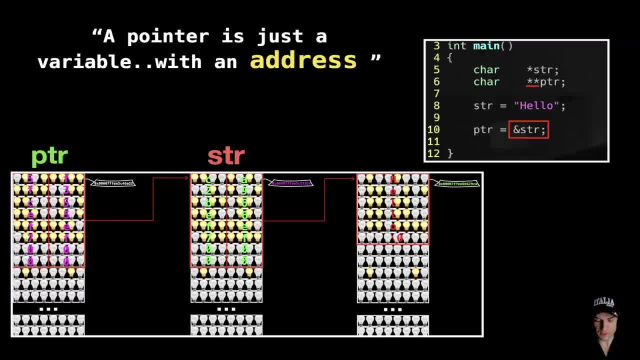 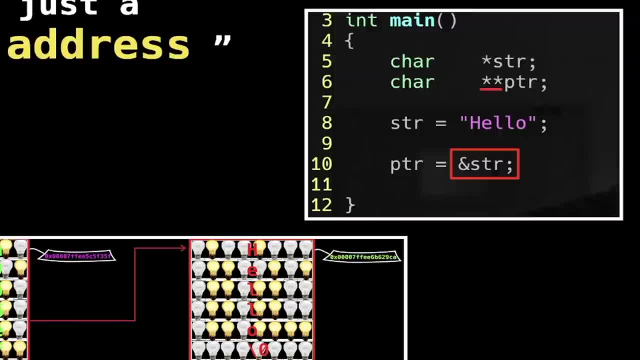 So let's just watch this stupid program that contains a string and a pointer to a string. I have a string- char star- and then I have a pointer to that string that I call ptr. As you can see, this is a double pointer. 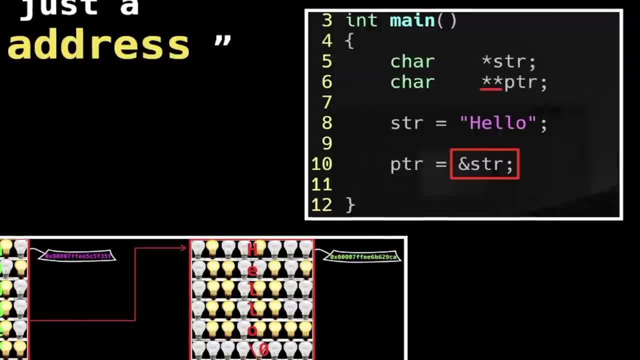 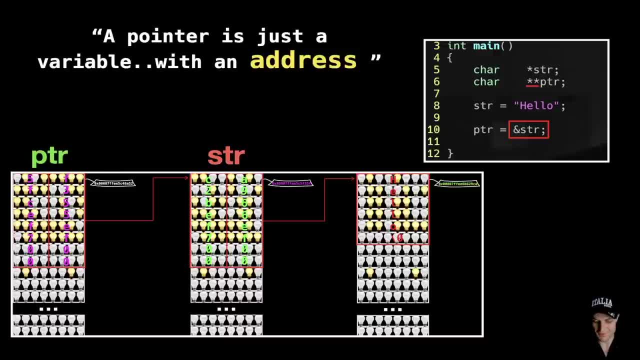 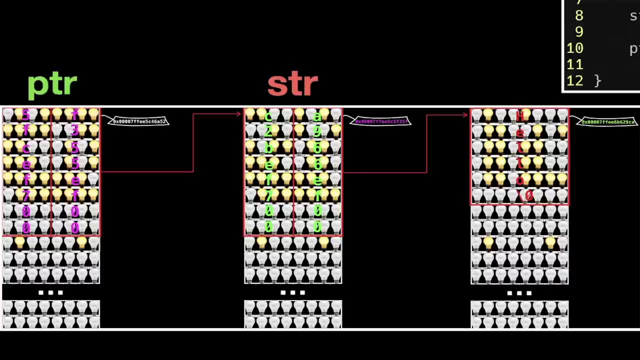 Right, because the string is itself a pointer. So ptr is a pointer to a pointer. So when you declare a pointer to a pointer, you have this structure. This is a visual representation of what is going on. As you can see, pointer is an eight byte in my system. object: 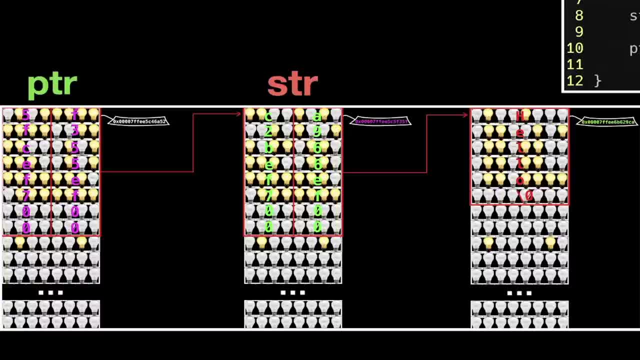 that is pointing to another eight byte object. str as well is pointing to the first char of the string hello. So if you watch carefully you can see that inside these two pointers you have the address. right inside str. you have the address of the letter H inside my string. 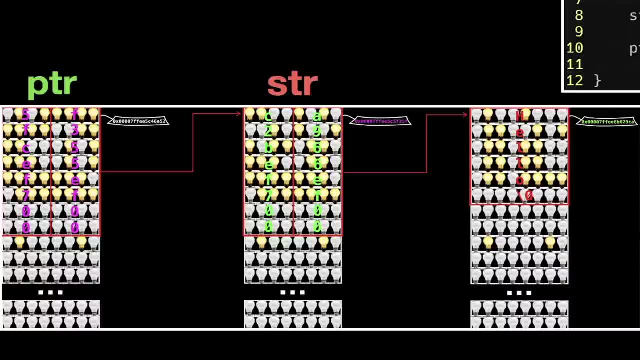 And inside my PTR I have the address of str right you can clearly see, thanks to the color and thanks to the hexadecimal notation. Indeed, we use hexadecimals because they're very cozy when we want to very clearly see groups of nibbles. 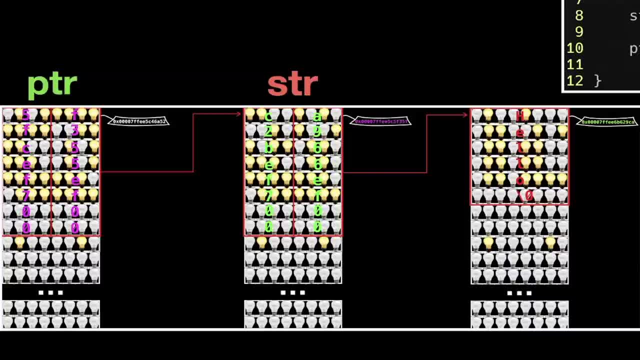 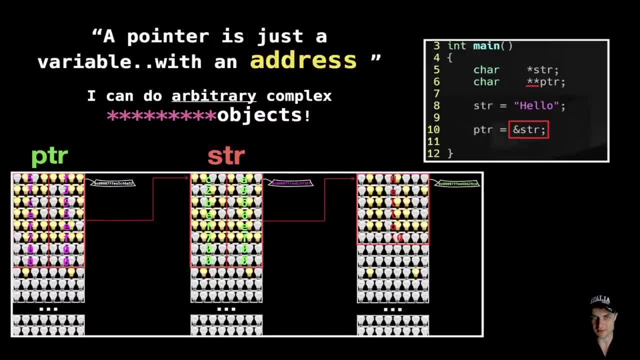 So at the end of the day, that's what it is- you can have a pointer to a pointer to a char, Easy right. Of course. let me repeat to you, you can create arbitrary, complex objects, a very deep, multi level pointer. 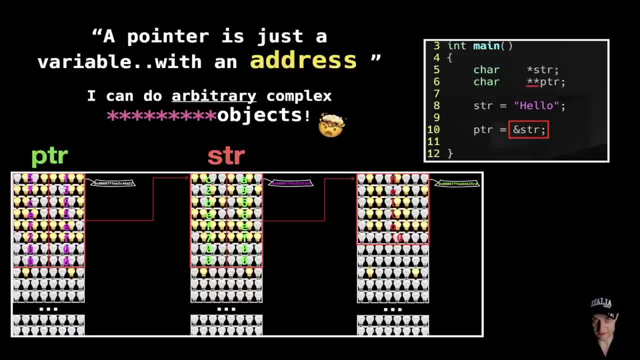 Of course this is not recommended because more than three level pointers, I would say- the code starts to become unreadable And this is super bad, especially for you, that you have to read again the code that you wrote. you won't be able to understand your own code. 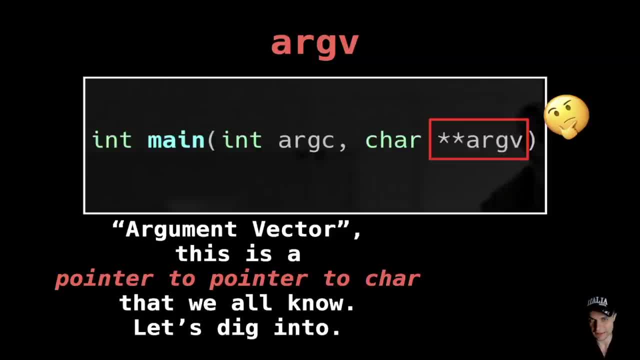 Now let's watch an example which is crystal clear, because we use on a daily basis. So these inputs are argument counter and argument vector. you have seen many, many times. right, You can also have environment variables, but now it's not the point. 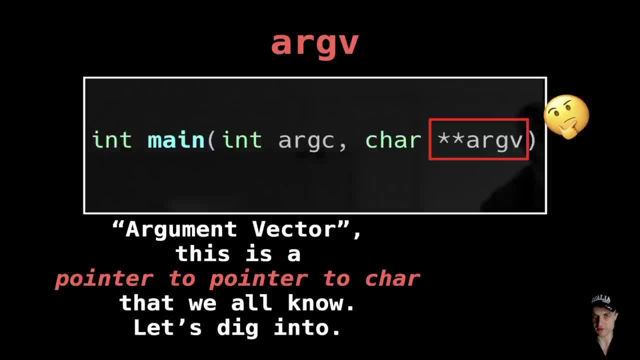 So I have this argument vector, which is a pointer to a pointer to a char. So that's perfect. we can analyze this idea of pointers to pointers thanks to these argument vector, So we are not going to talk about something which is poorly theoretical. 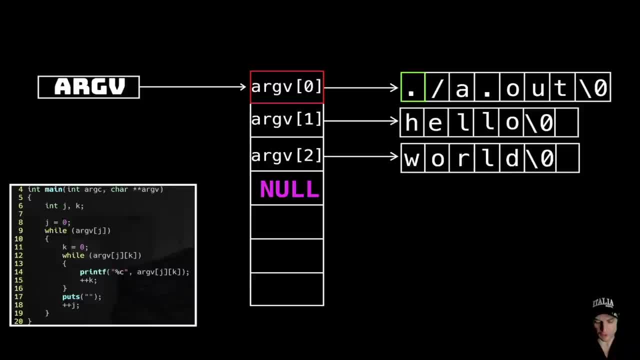 we are going to talk about something which is pretty useful on a daily basis. So here, my friend, I have a little algorithm that is able to print all the chars inside argument vector, And this is a very good representation of what argument vector is. 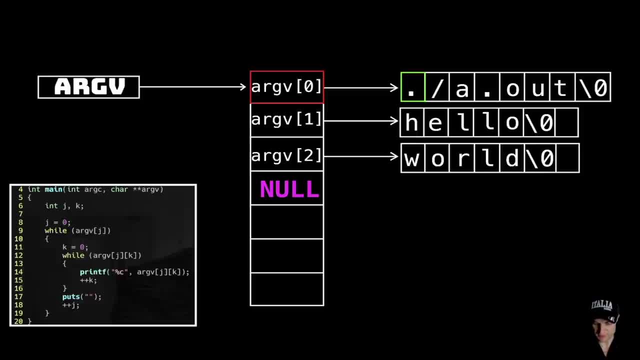 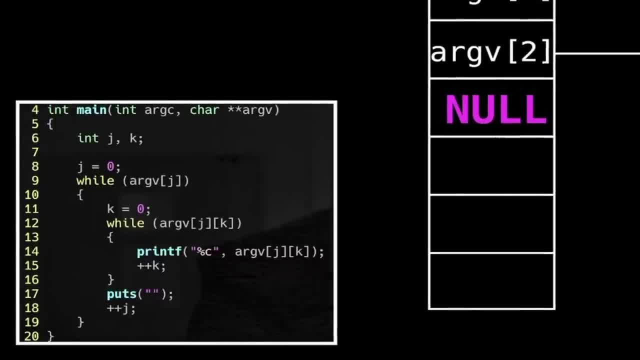 And then I simply do a nested while loop. With this nested while loop, I'm able to print all the chars. Of course, I want to print char by char, because I want to make extremely clear how the structure works. So let's start a loop. 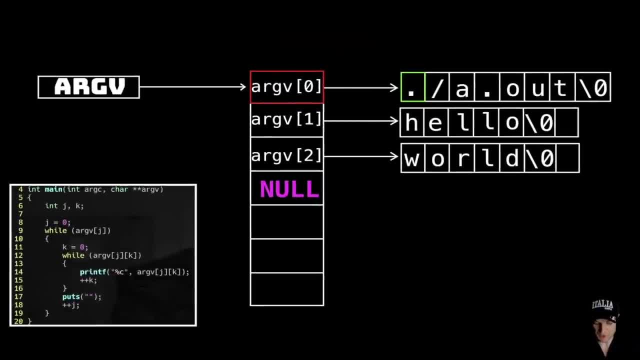 I want to make with you very visually. We have initially J, which is equal to zero. So I have argv. that is pointing to the first pointer. the one in position zero, After that I have a K is equal to zero. This is a refresh operation. 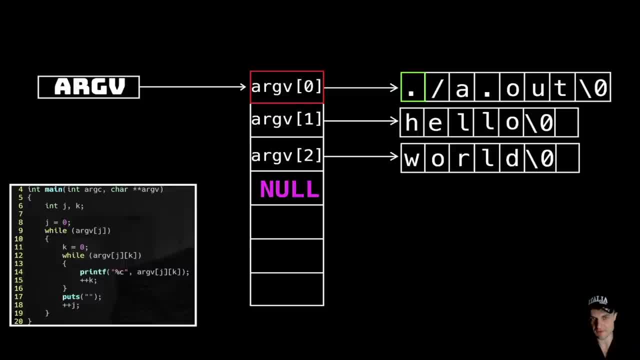 I want K every time to be zero, So this is going to work. It's going to be the first char of my string. Then I simply do a loop, while argv, J, K print that char. Okay, So initially I'm going to print the point. 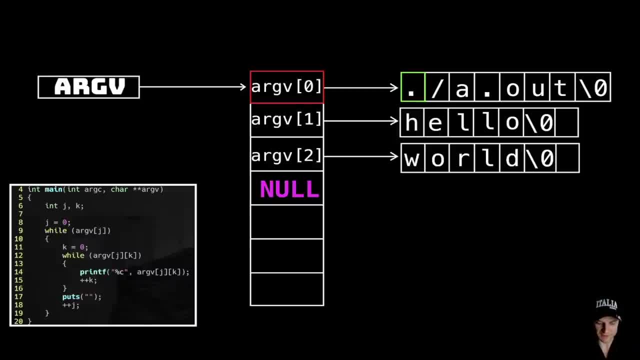 Of course, here I don't use is different from zero, because this is redundant. I'm going to use directly the backslash zero as a boolean value. So this is the inner while loop that is working. So I'm going to do while argv J in position K. 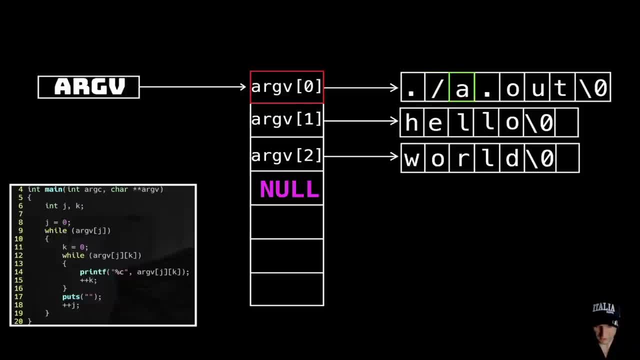 I'm going to loop. I go in the first position of the string, Then I go in the second, then in the third, and so forth Right, Until I reach the final backslash zero. This final backslash zero is going to act as a boolean value. 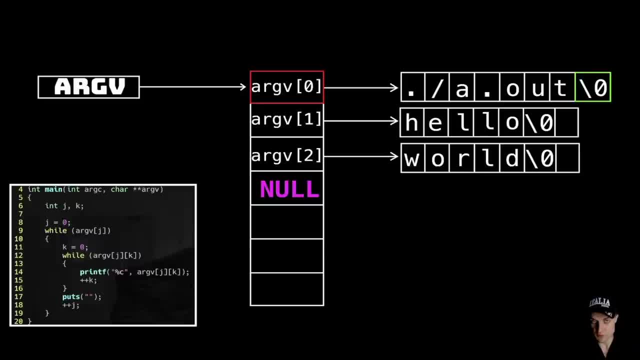 You know that in C zero is equal to false, So this while loop is going to break. I have a put S, So this is going to print a new line. I go in the following line And then I just increase J. 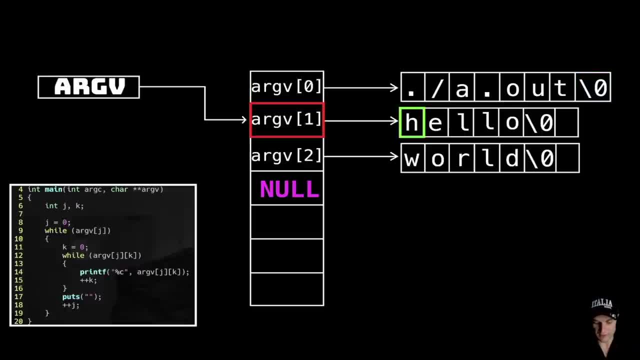 So I go in the following pointer: Boom. You see K is going to be refreshed. And then I do again the same thing. You see, I loop inside all the chars until I stumble upon the backslash. Here the condition is going to become false. 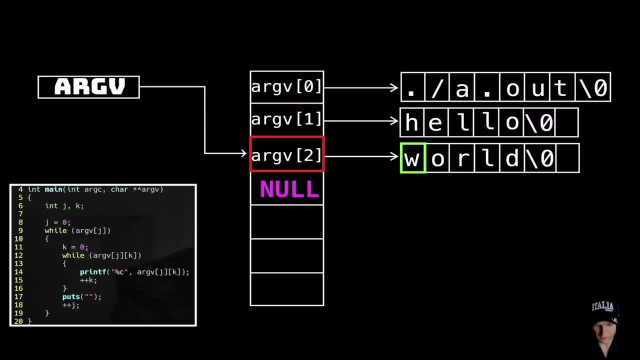 So again, the while loop is going to break. I print a new line And then boom, I go in J, equal to You see, And then I do the same thing. I'm going to print all the string until at the end. I'm going to stumble upon this null. 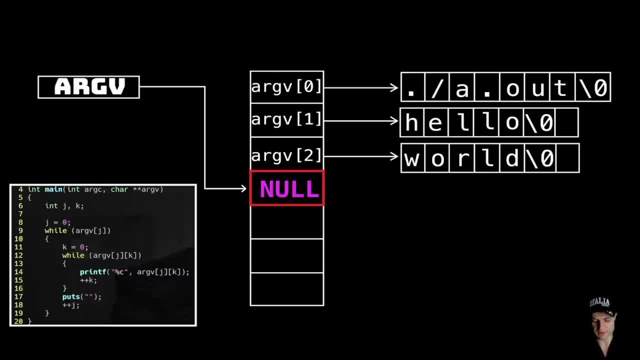 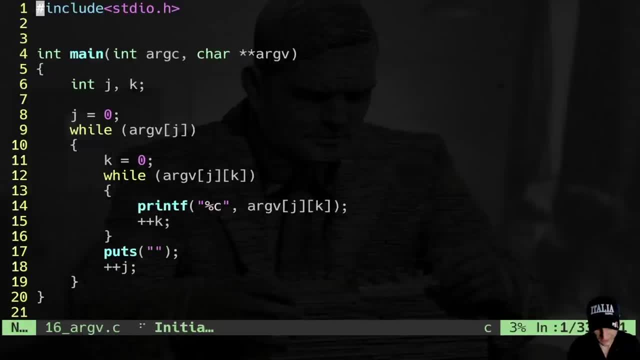 This null, my friend, is a sentinel value, So thanks to this null I can say: OK, I don't have any more strings in my argument vector. So here, my friend, we have the actual program That you just saw. 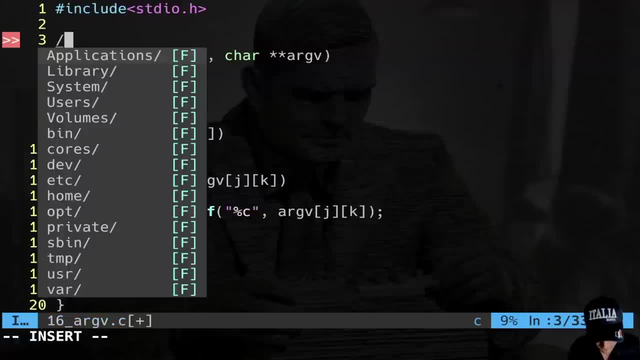 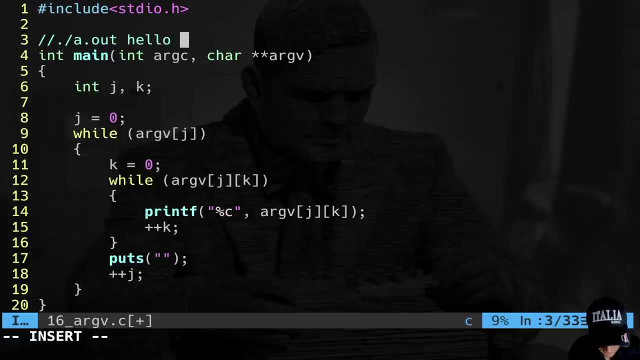 So here, for example, I have my program that I'm going to launch, For example, I don't know. I'm going to have a dot out and some inputs, For example: hello there, OK, These are going to be the strings that are going to be written. 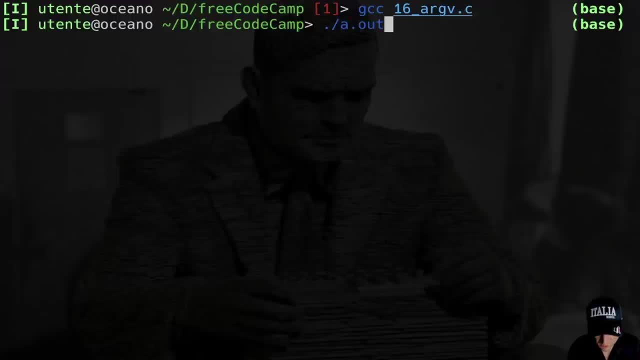 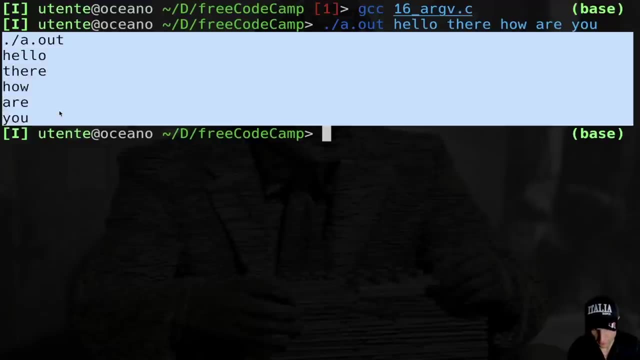 So let's try to compile and launch. I'm going to launch with an input, For example: hello there, How are you? Boom. And as you can see, I have in my standard output all these strings. You see, Cool. 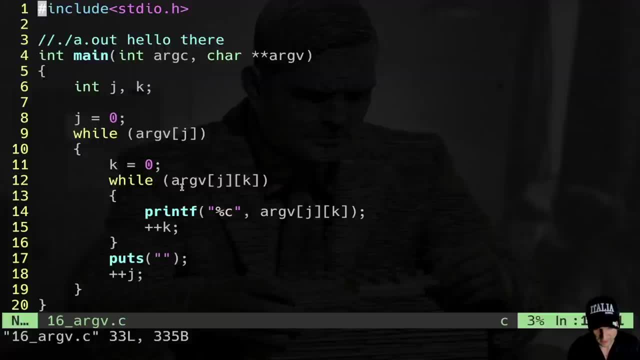 So this is a little algorithm that is going to loop inside the strings pointed by argv. Here, of course, I used the square bracket notation because it is more intuitive, Do you agree? But you know that this is just at the end of the day, syntactic sugar. 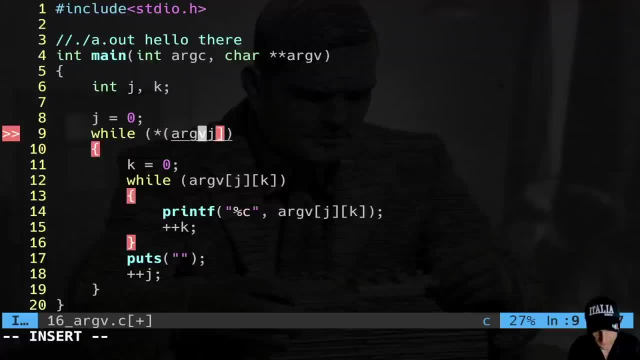 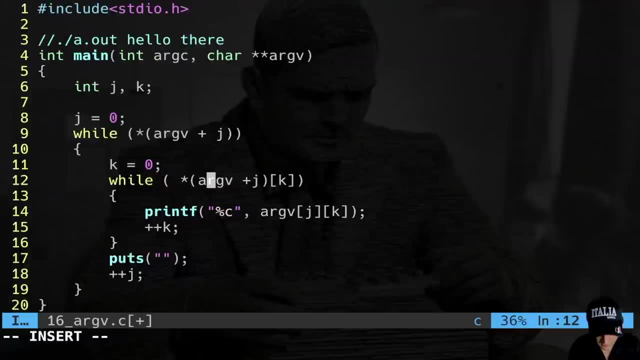 I can do also like that. Let's try I can do at argv plus j, right, And here I can do. These are more complicated, but it's going to be at argv plus j, And then I'm going to do. 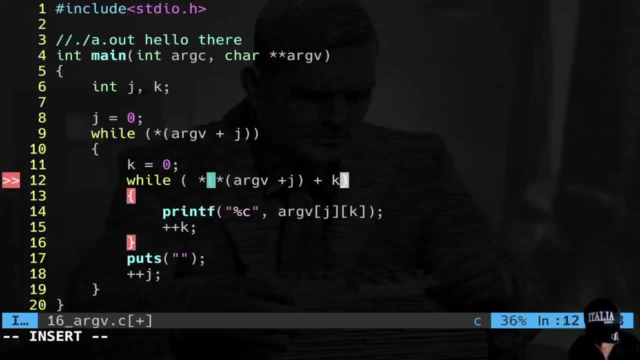 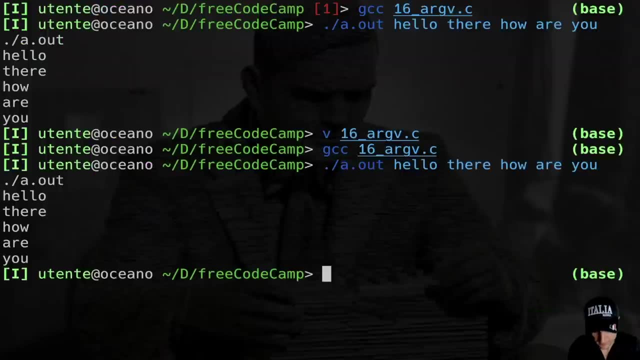 At argv plus j is going to be the reference plus k, like that. Cool. Let's try to launch again the code and let's watch if it's going to work again. As you can see, it works exactly the same, because I did exactly the same thing. 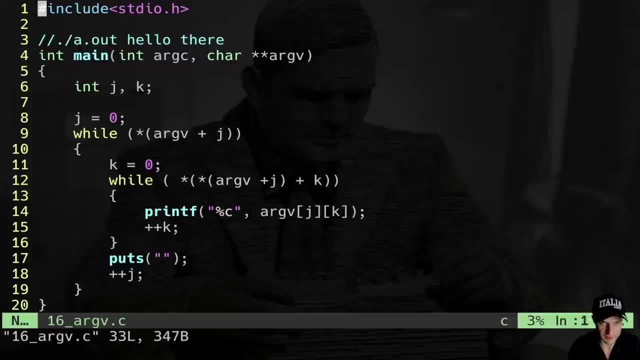 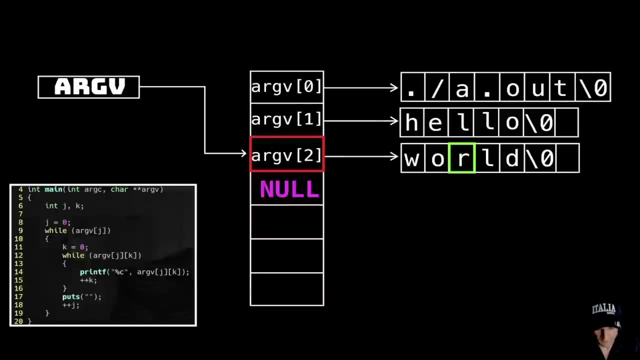 I'm sure you agree that the square bracket notation is far, far better, far, far more intelligible than this one, right? So it's far better to use this. and the square bracket notation, if you watch carefully, really recalls the cell right inside our vector, our array. 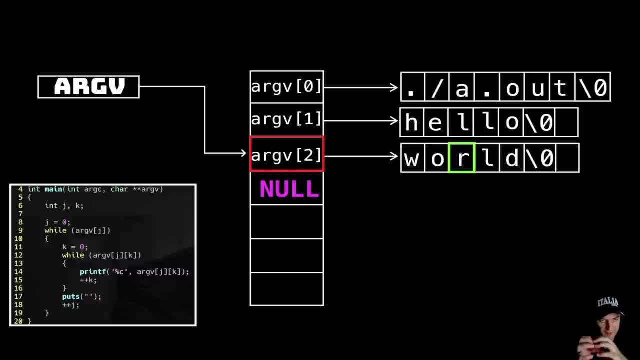 We have the first cell, the first level, and then the second level, which is the chart itself. You see, it's fairly intelligible to see what is going on If you have a clear diagram in your mind. with the first j, I'm selecting the string. with the k, I'm selecting the chart itself. 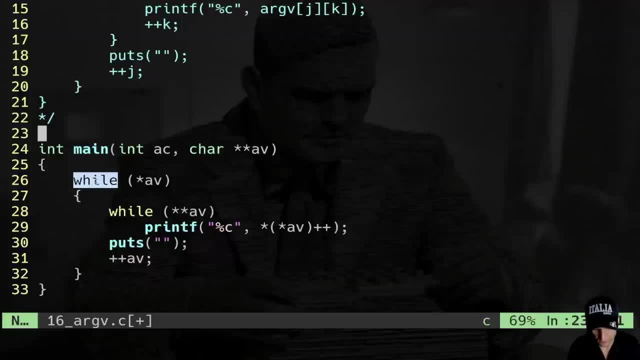 Now here I have the pro version of the program. Basically I say while at argv and while at av right. You remember, Yeah, from the previous video when i told you that when i double the reference this i get the chart because i can see in its signature right i have. if i double the reference this object here i get the. 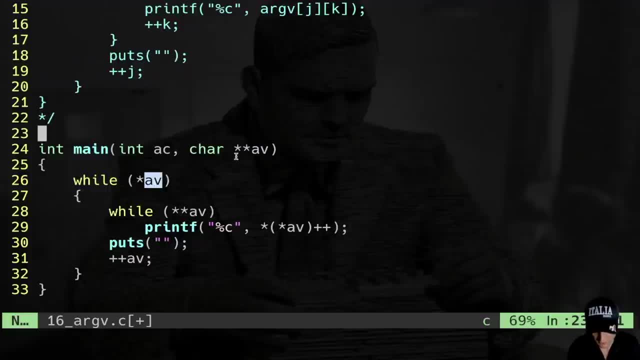 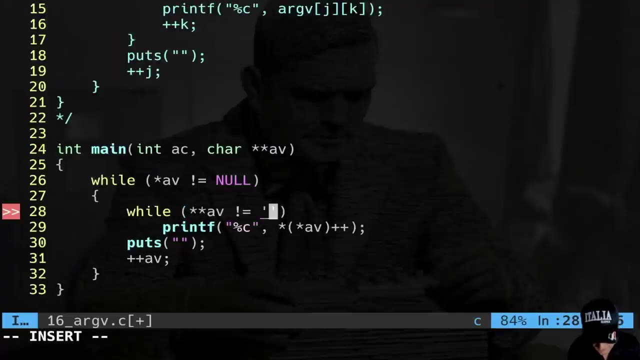 chart. if i single the reference this object, what do i get? well, i get a pointer to hr. so here is written, while i have a pointer to hr- and here i just omitted this- it's different from null right and while v is different from zero. you print all the stuff here. i use the. 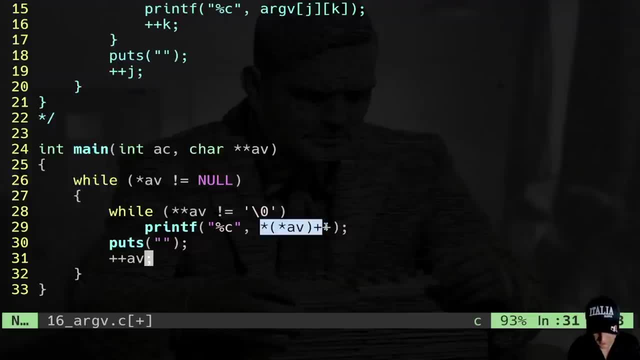 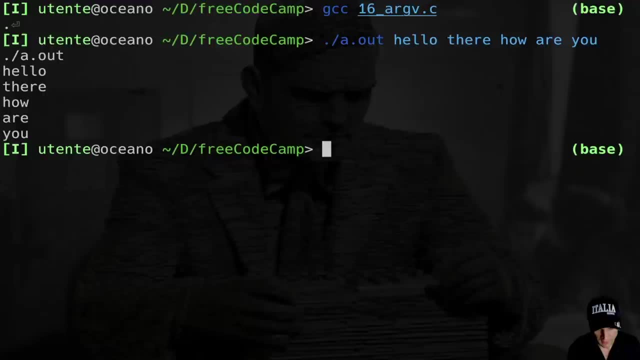 the pointer notation to your reference. you see how cryptic it is. it's far better to use the square bracket notation when we have multi-level pointers. anyway, let's try to launch this and see if it works. and, as you can see, it works exactly like the previous one. cool now, my friend, i'm sure. 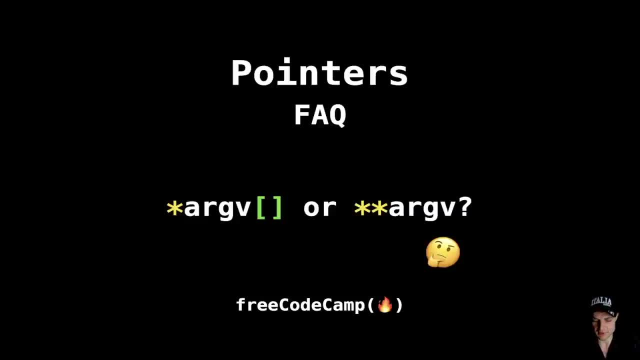 you many times have seen this signature in the main right. so you can have a star or v array, or you can have a double star, argv. what is the difference here? now, given that you understand this array pointer duality from the previous video, i'm sure you now understand what is going on well. 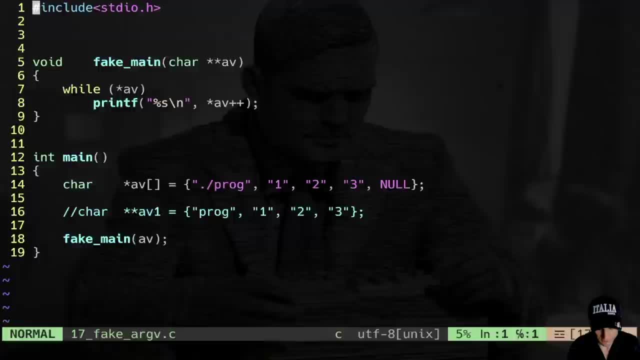 my friend, the problem is always the same: array, the k. so here, my friend, i have a little program that is creating a fake main. you see, that is taking an argument vector and here i'm creating in my main function an argument vector. so this is what thanks to the right left. 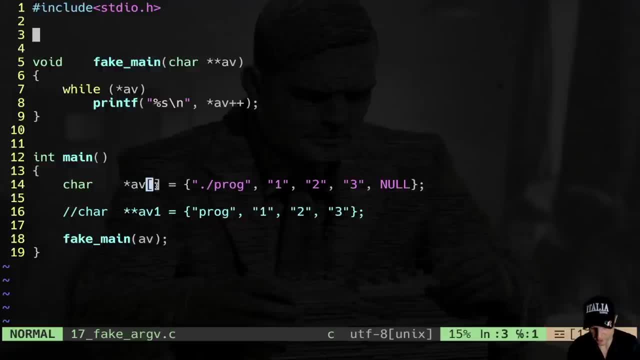 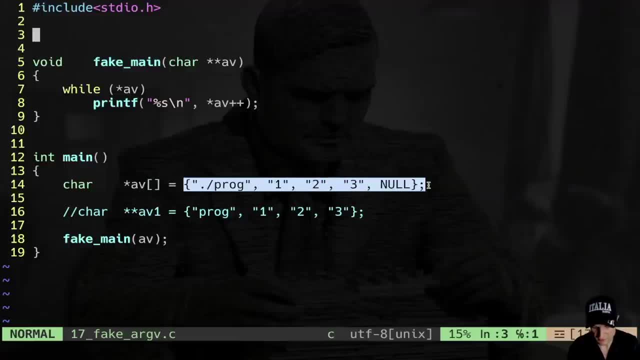 pointers to char. so this is the initialization of the array. i'm going to insert directly the strings. right, given that this is an array of strings, at the end i'm going to put an all. then what do i do? i call the fake main function and i pass av. but you remember right that arrays have this. 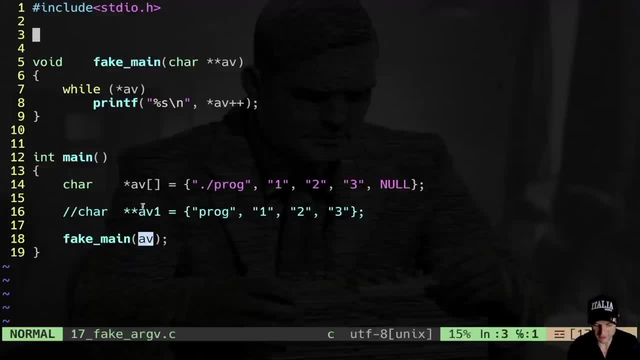 peculiarity that are going to decay to a pointer, to the first element. so we don't really care if the objects inside the array are pointers themselves. they could have been integers, floats, doesn't really matter. the thing is that we have an array, so you know that when we pass an 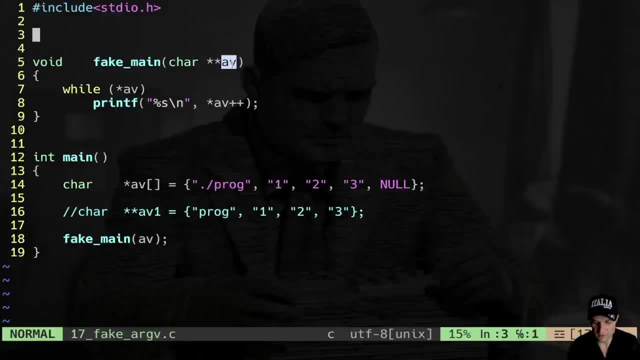 array, the function fake main is going to receive a pointer, a pointer to what? a pointer to a pointer? because this array contains pointers. that is what is going on. let's try this code and let's convince ourselves that this is true. so i'm going to run the code and, as you can see, i have the inputs. 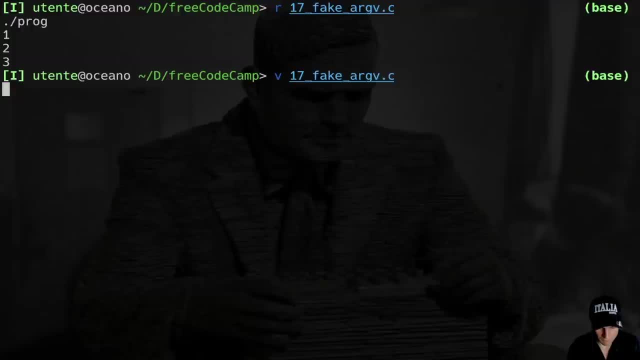 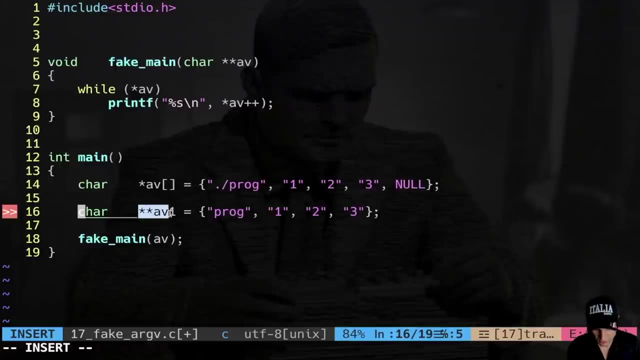 that i've given inside my array. now we have to understand a point here. i want to do this operation, creating a v1 which is a pointer to a pointer, and then i do the same thing as here. i initialize this pointer to pointer like here. but i cannot do that. let's try to compile this. 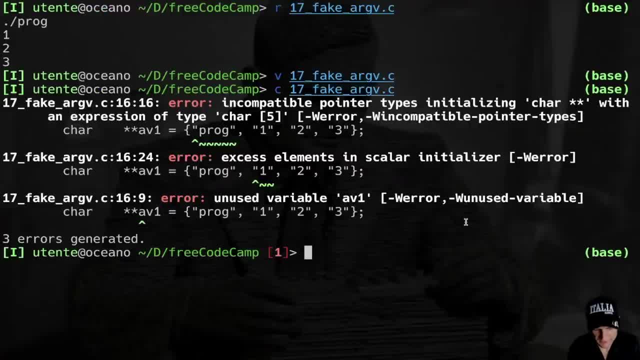 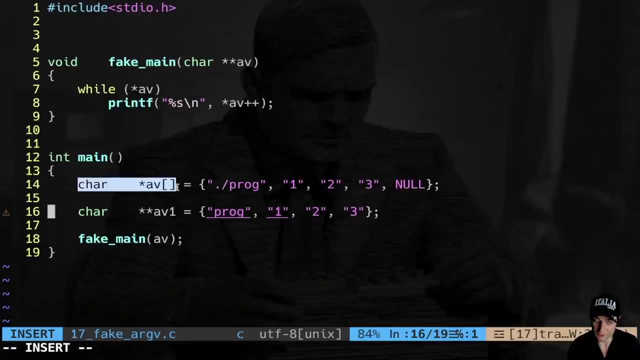 code and let's see the mistake. so i'm going to compile. as you can see, i cannot do this operation. incompatible pointer types initializing char star star with an expression of type char star star five. the thing is that at this level, this is an array of pointers, an array, so we have an. 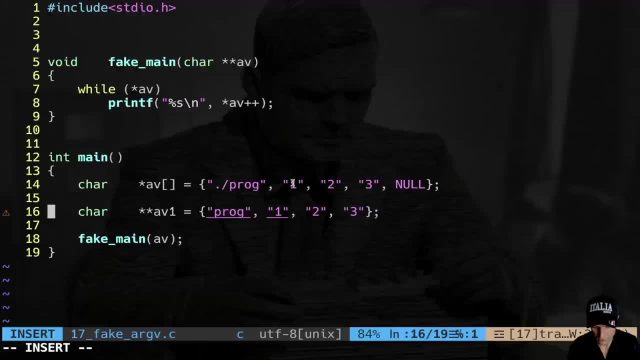 allocation of space. in this case we have an allocation of one, two, three, four, five pointers, so 40 bytes. and, as i told you, this is an array. array and pointers are not the same thing. they behave similarly in certain conditions, but they are not the same. here i just have a pointer, so 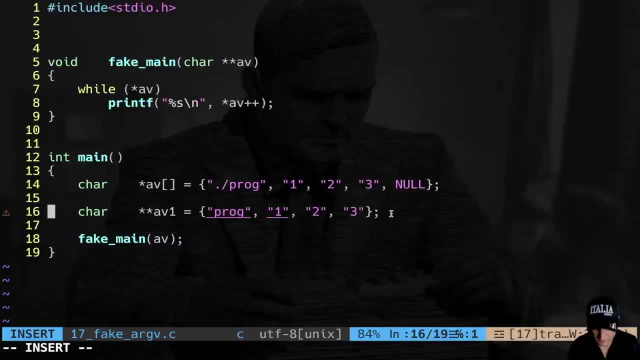 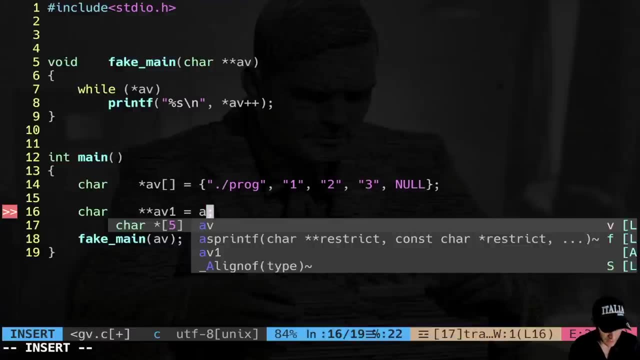 what? what am i doing here? i'm assigning this thing to this object. this is not. this is not possible. this is not feasible. this makes no sense. i can do that here. i can do. this is equal to av. this is legal. and why it is legal? well, because you know that the identifier of an array is going to 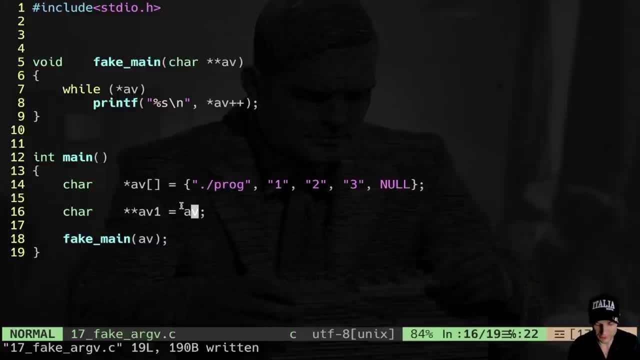 decay to a pointer, to the first element. so here i have a pointer to a pointer. okay, that's all there is, i think. uh, you understand super well what is going on. so here of course, i can write like this or like that. it's exactly the same here when we write in the cold function an array, it is just to. 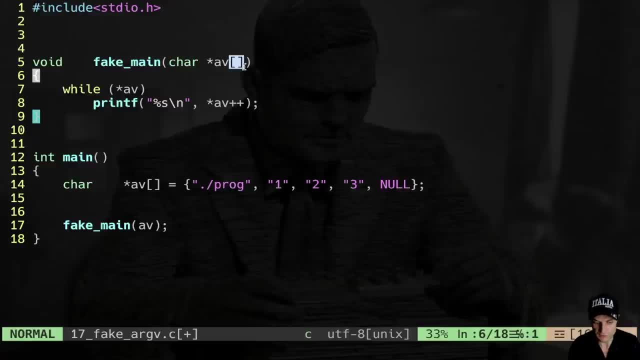 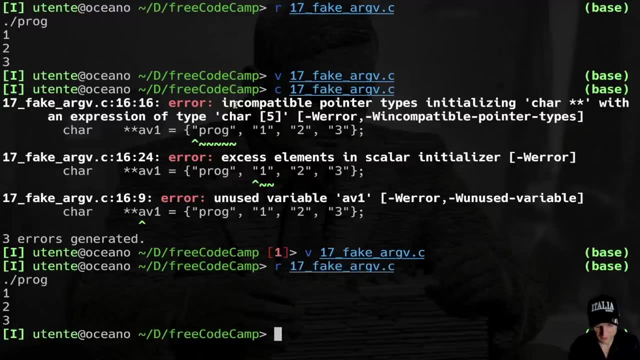 stress out that in the coley function we have an array, we are manipulating an array, and what we are using, the cold function, is just a pointer. so let's run again. as you can see, it works perfectly. okay, i think you understand what is going on, right? so my humble suggestion is always the same. just 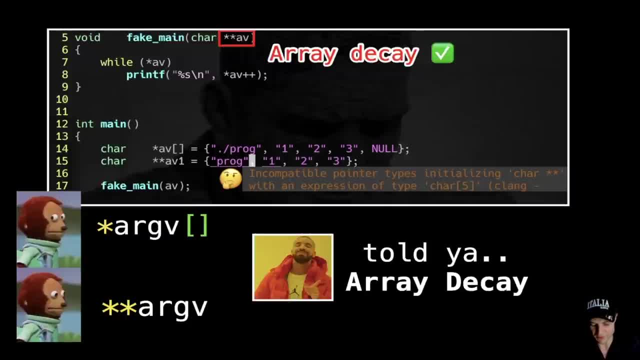 keep in mind that an array, probably in your code, is just a pointer. if something bad happens, just remember that array are arrays, so probably it is an exception. the array hasn't decayed. so if you want to train a little bit with these pointers to pointers, you can come here in ctuser and do some. 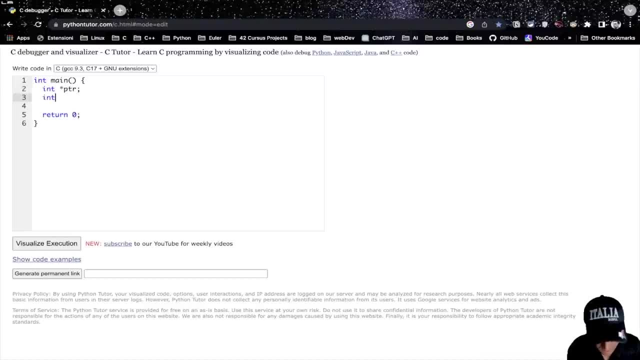 code. for example, you can do ptr, you do int and equal 42. double ptr, triple ptr- okay, so you do many level pointers. you see, let's do till four ptr- okay, so we do. yeah, although with the same name: ptr one, two and three. and then i say ptr is equal to the address. 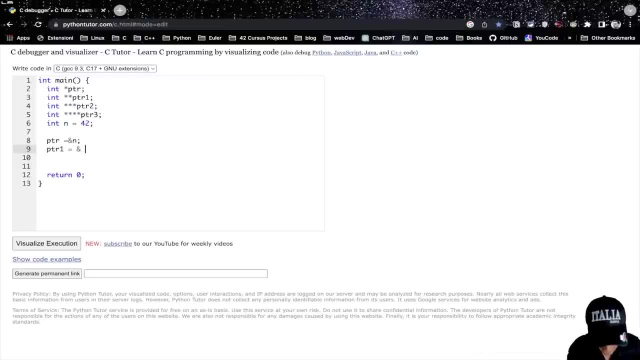 of n. ptr1 is equal to the address of ptr. you see, ptr2 is equal to the address of ptr1. ptr3 is equal to the address of ptr2. okay, let's try to launch this code, and here you see, you have a bit of a. 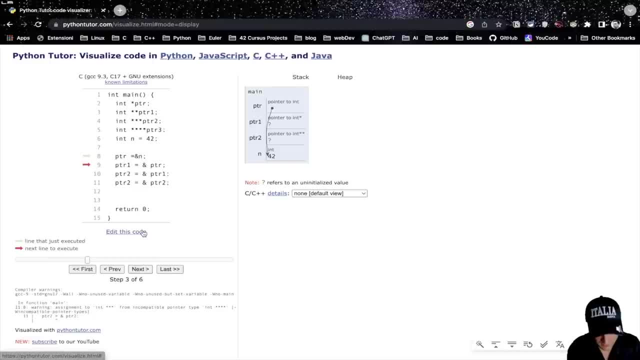 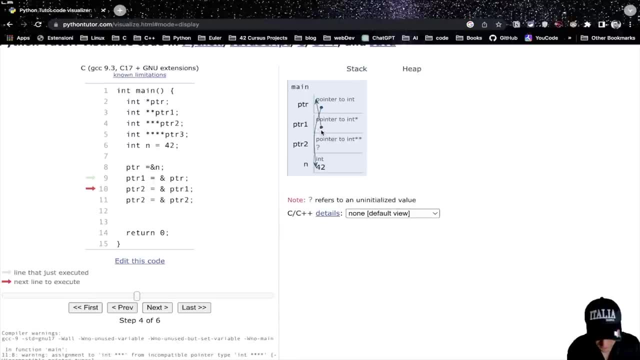 beautiful representation. you have the number and you have ptr here that is pointing to 42. then what do you have? you have ptr1 that is pointing to here- i made a mistake- ptr3 i want, like that. okay, let's launch again. so i have 42, i have a pointer to 42, then i have pointer one that is: 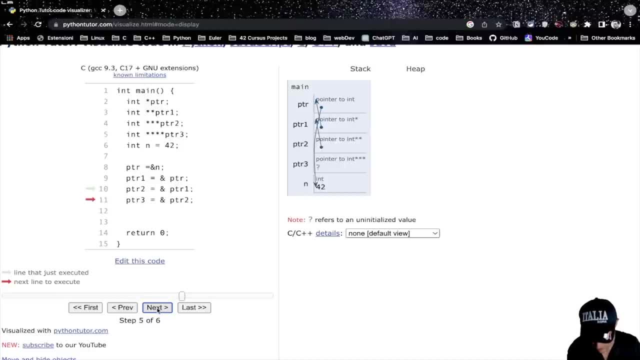 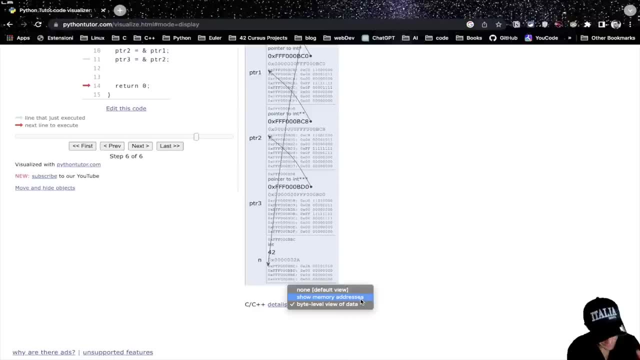 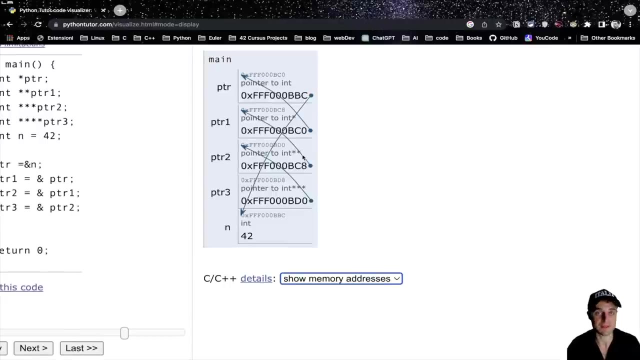 pointing to ptr, then i have pointer two that is pointing to ptr1, and then i have pointer three. that's the structure that you can expect. here we can also see the memory addresses, so we can have a better understanding of what is going on and you can create all the mess that you want with. 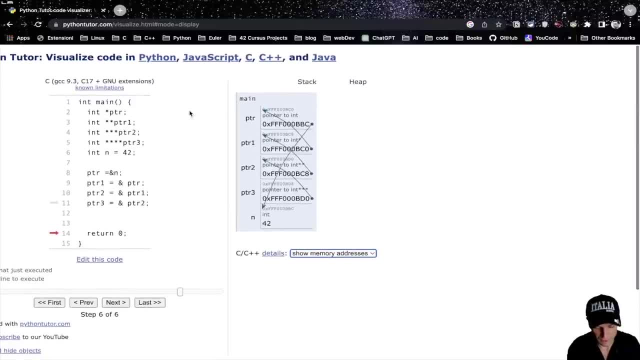 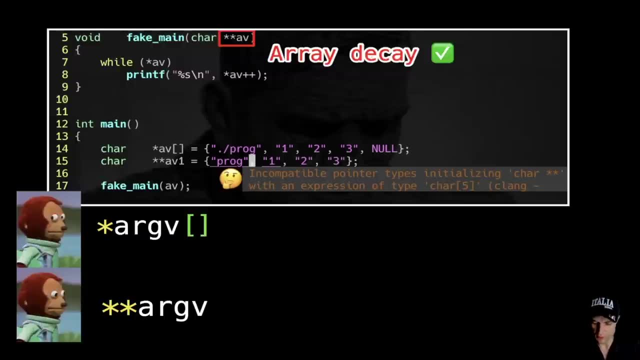 these pointers. okay, just, i highly suggest you to come to this website and work out a little bit these ideas. okay, that's all there is with these double pointers. i don't want to dig too down because these can become very complex. so, my friend, here we are in the last chapter of this mini course. 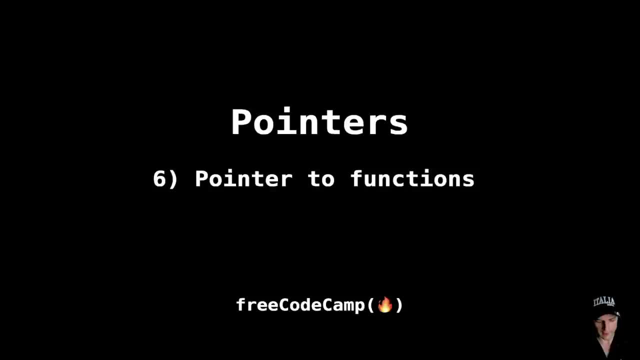 we're going to talk about pointer to functions. i'm not gonna go very deep, first of all because this starts to be a little complicated and, generally speaking, pointer to functions are not super used. of course, this boils down to the type of code you're writing, but i would say initially: 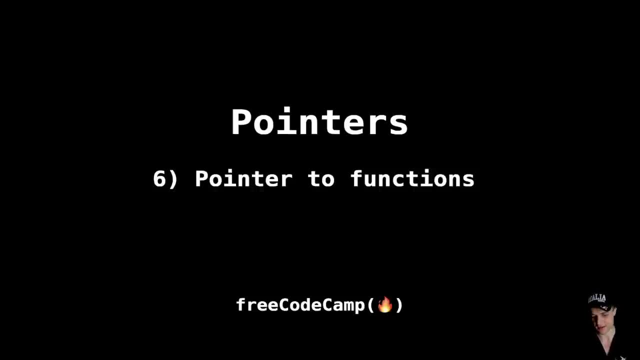 if you are a beginner and if you are watching these kind of videos, you are not gonna really use pointers to functions anyway. this is just a gentle introduction. i would like you to understand what is going on with pointer to functions and i'm not going to go into too much detail on this. 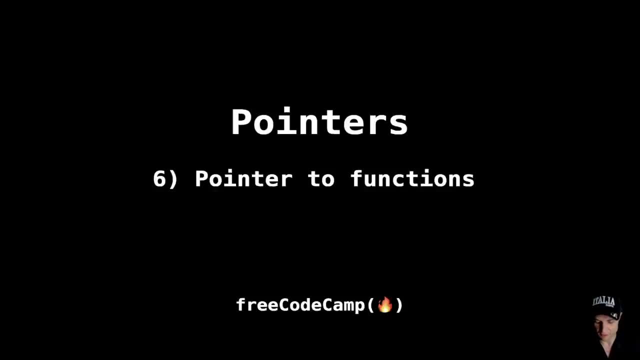 but i'm going to start with the first part of the video and i'm going to start with the first part of the video, and i'm going to start with the first part of the video and take home the overall ideas, the overall principles. so you know that a function is a symbol. 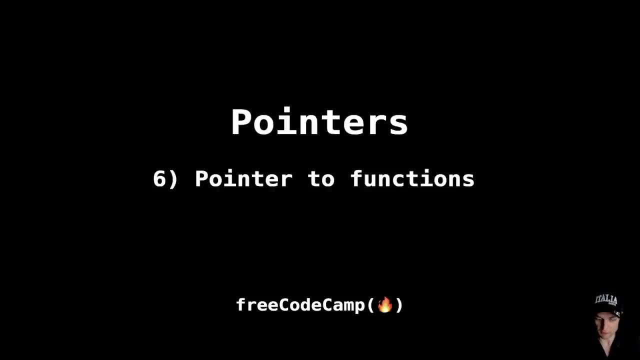 that you can call to get some action right, to perform some, perform a specific task, for example the printf. when you call the printf you would like to see on the terminal something written, and indeed that's what it is. but functions can be also pointers. so let's read together this line: 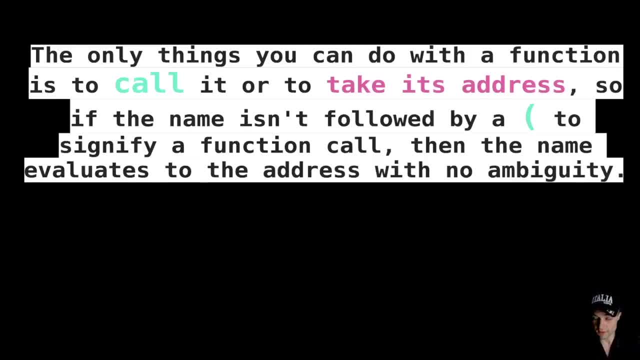 the only things you can do with a function is to call it or to take its set. so if the name is not followed by the brace- the round brace- well, it means that i don't want the function to be called. but i want something different. indeed, i want the address of the. 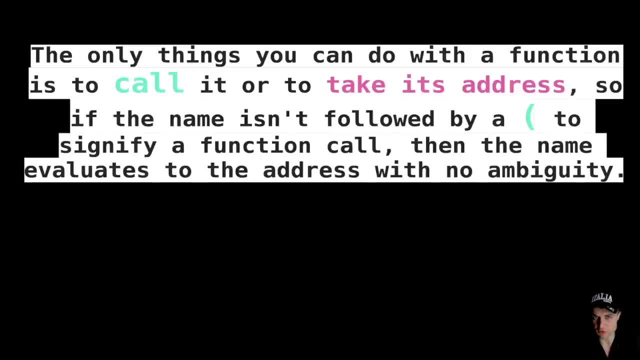 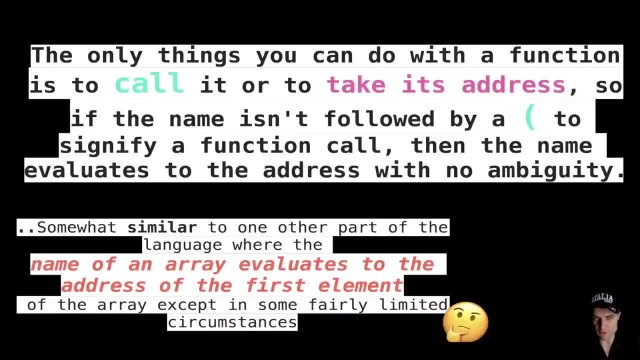 function. so take home message: if you write the name of the function without the round brace, it means that you want the address. it is kind of similar. if you want to, the array decay right when you use the name of the array is going to decay to the pointer, to the first element. well, 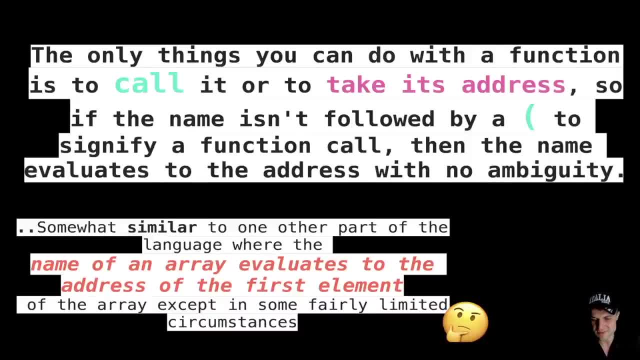 in this case it's similar if you want to call it the address of the function. so if you write the name of the function, the principle is similar. if you use the name of the function is gonna quote, unquote, decay into the address to the function. so let's understand better this idea. 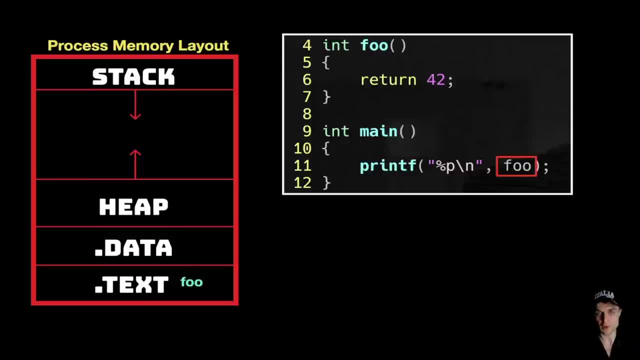 here, as you can see, i have my process memory layout, so when you launch your program, you know that the operating system is giving you a space in memory which has this shape. now where, in my process memory layout, the function foo, in this case a stupid function that is returning me the 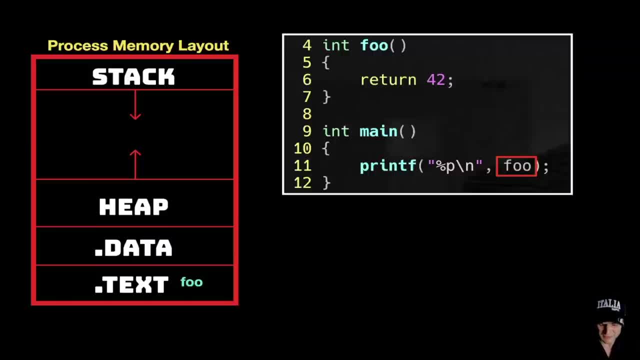 value for the tube lives in the stack in the heap. where is it in the stack in the heap? where is it, this function? well, it turns out that the function lives in the text area. indeed, the text, also called the code segment, contains the instructions of your program. instructions are bare bone binaries that. 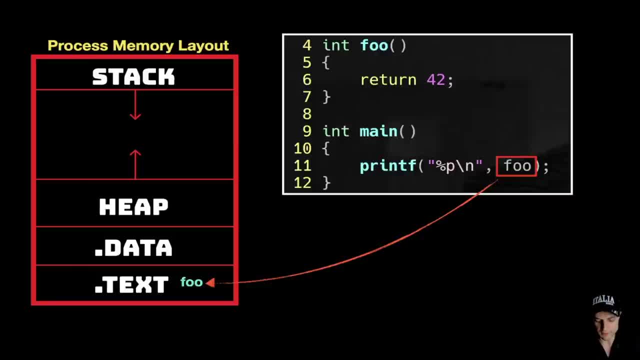 are telling to the computer to do something. you don't have to go too deep into this stuff, or better, if you want, that would be marvelous, but it's low level stuff. so the binary of the function foo, the instruction, live in this section in my process memory layout. so if you watch carefully, the printf is trying to print a pointer. 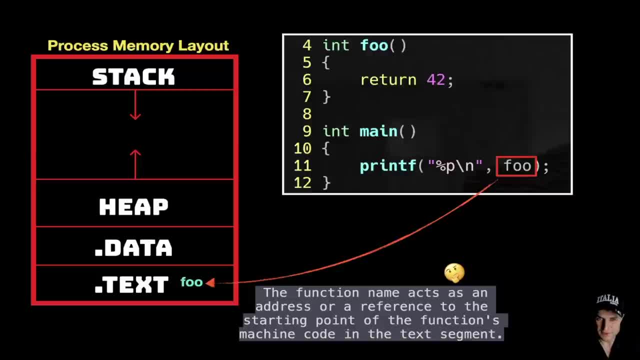 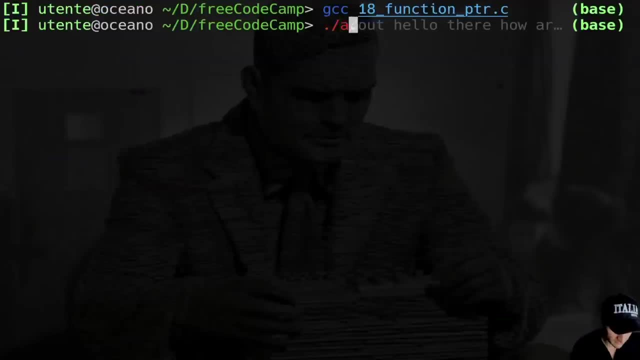 you see from the identifier p, foo is a function, but i'm not using with the round brace, so you know from before that this is the address of the function foo. so this is the program, my friend, and now we're gonna launch. so i'm gonna compile and now i'm gonna launch. okay, here comes. 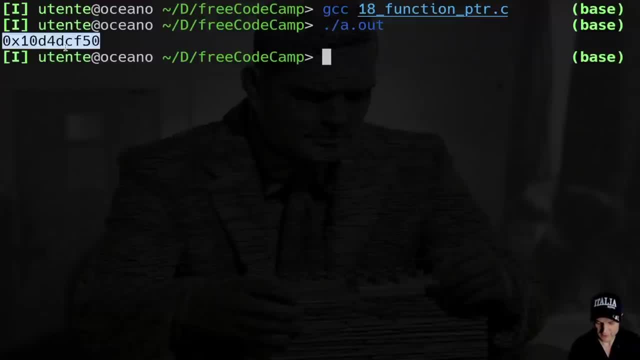 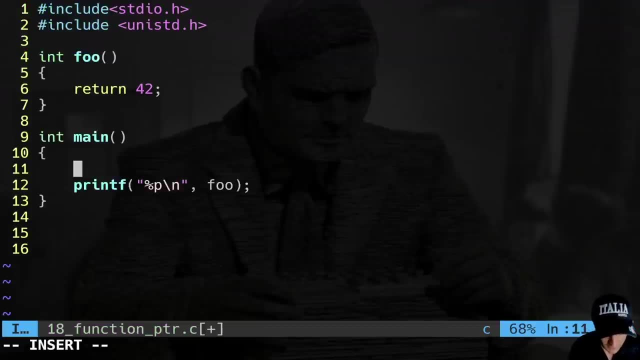 i have this address, which is kind of peculiar, right, it's very different from the kind of address that we get from a variable. let me explain better. if here i do int and b and b equal 13 and i print the two addresses, okay, so p and p, here is foo and here i use the address of mb. 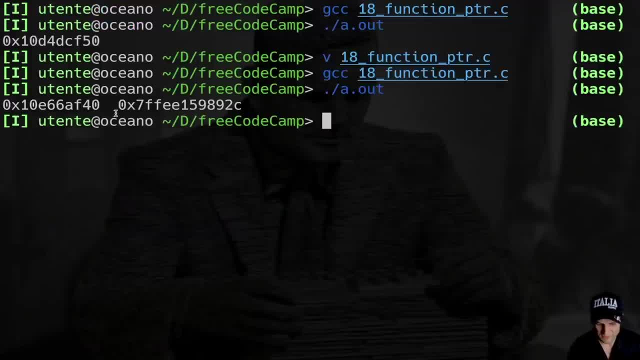 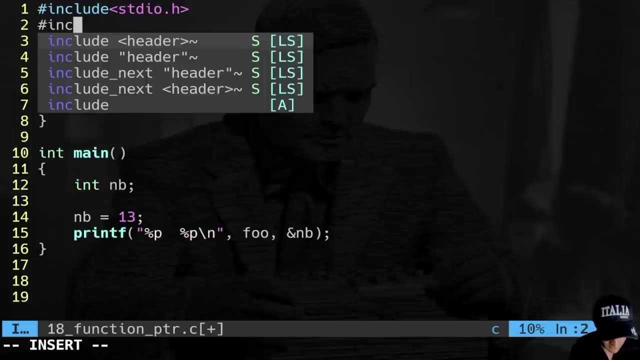 so i'm going to compile and launch. you see, they are very different. very, very different one is this: quote unquote: little number. on the contrary, our variable lives here. now i want to explain you something. to do that, i use the slip function. so include uni std. 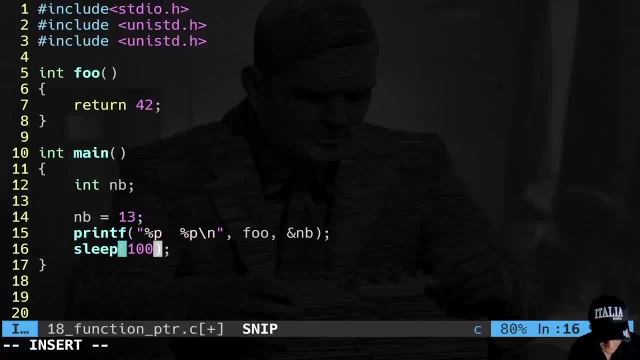 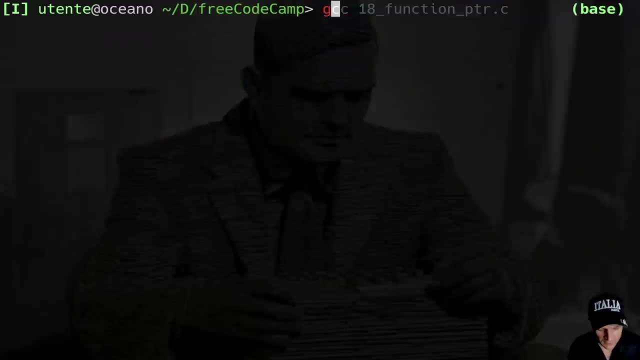 and here i do a sleep 100, okay. so i want my process to not die, to stay alive, because i want to check this process, memory layout. so i'm gonna compile and then just launch with the number cent so i have the terminal. i can use the terminal even though the process is running on. 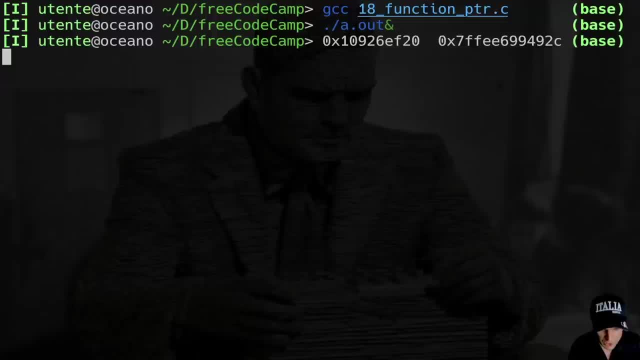 the background. so enter. now. i check ps here immediately. you can see the, the addresses right. the printf has worked, so i say ps. you can see that the process is running. now i do virtual memory map of the process and then i pipe this into less. this is just a way to see better what is inside. 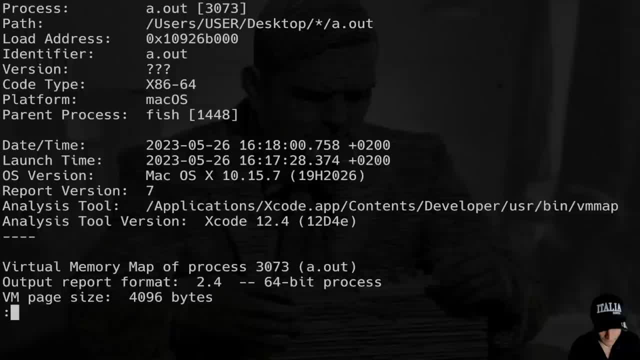 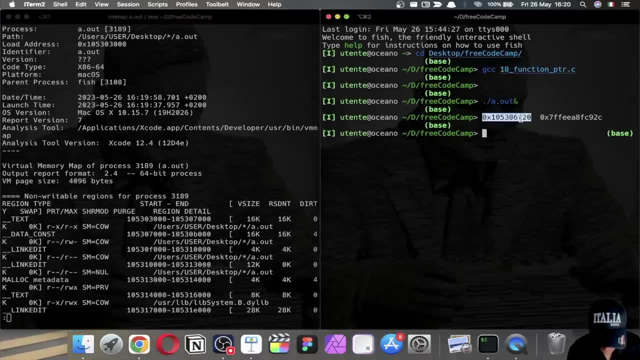 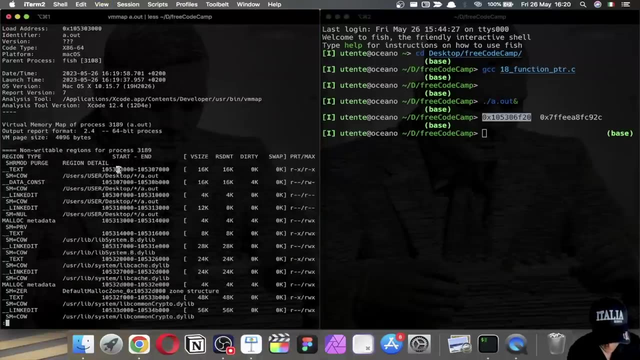 the output of the command: virtual memory map. okay, enter now with this command. i can see the virtual memory layout, which is this one. now we have this address, which is this one: 105, 30, 6f, 20.. let's see if we can find here 105, 30, 36, f. so here we go, from 30 to 105, 30, 70.. so you see that, um the address of. 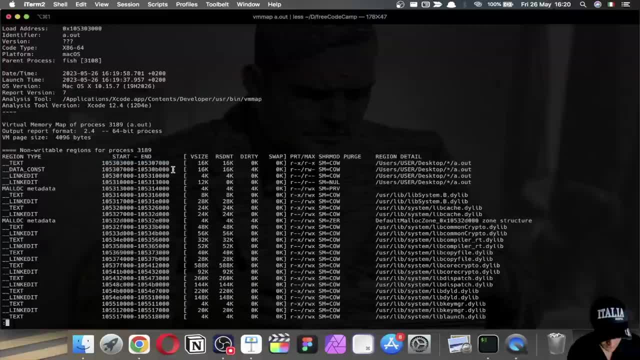 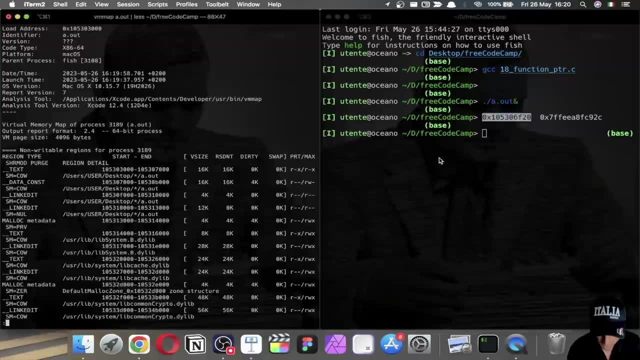 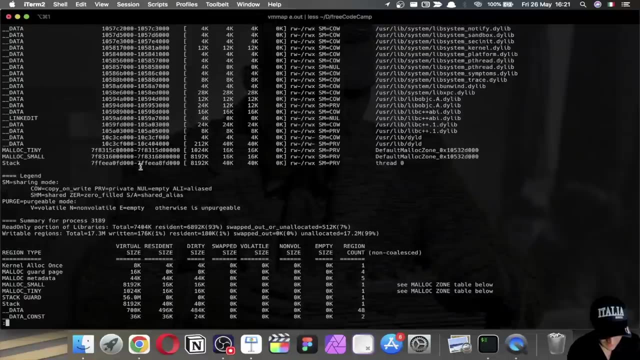 a function is here, is in this range and, if you watch carefully, this is the text range. here it is a non-writable region. of course, we cannot change the values inside the text here. on the contrary, we have this value 7ff. i already know that this is the stack, of course, so let's search for the stack, as you can see here. 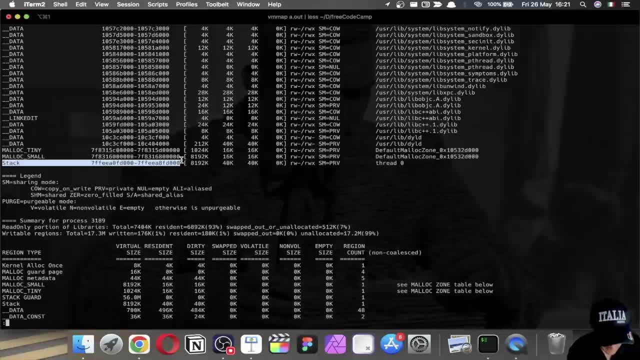 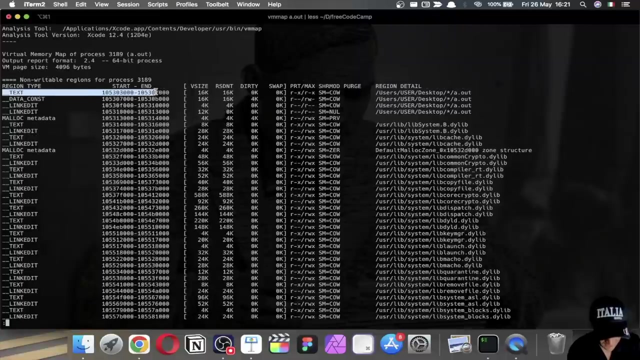 maybe is in this range here: seven f e, e, a zero, seven f e, e, a eight. so here i have a eight fd zero, zero f c, nine two c. you see. so i have the variable which leaves in this range. so i have one range here. on the contrary, i have the um function that is living in this range. okay, so 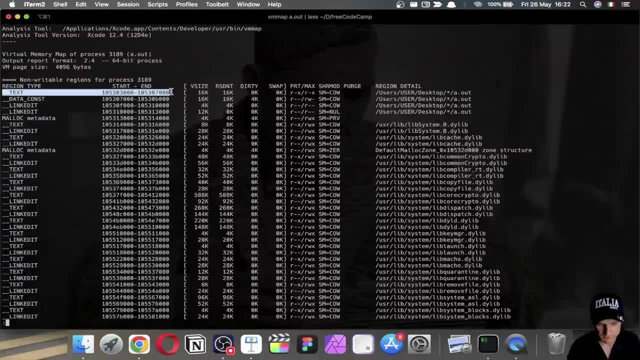 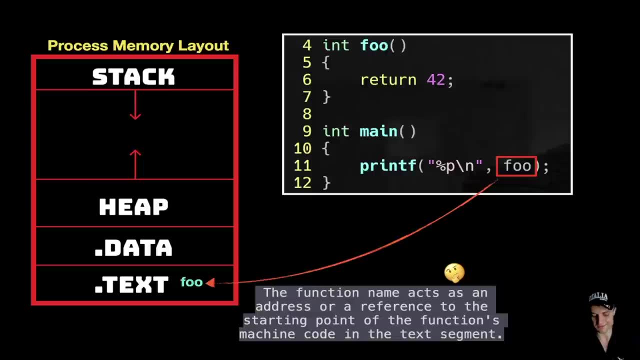 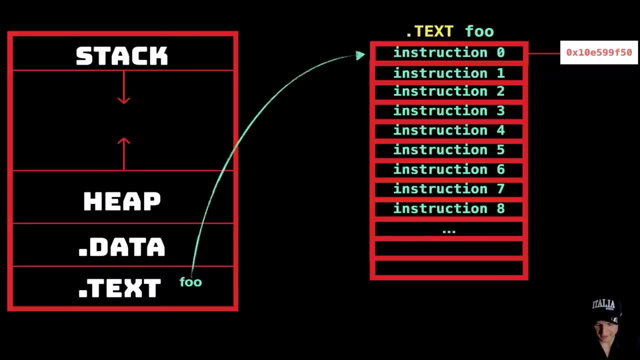 this is low level stuff, technical stuff, but just to give you a glimpse. so this is, uh, the abstract view that i um proposed to you, in which we have our function that lives inside this place. now let's zoom in a little bit so we have our function foo that lives inside the text segment, and 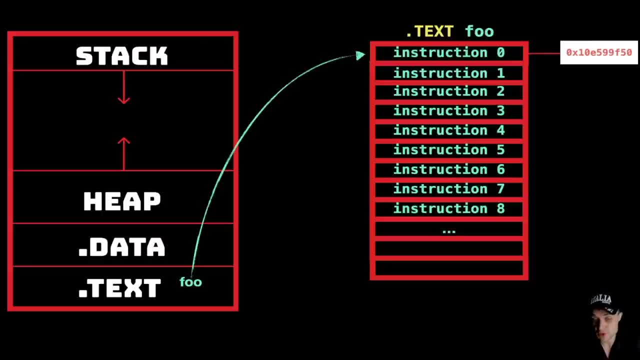 basically, this foo is a pointer to instruction zero if you want of that function. foo is a pointer to instruction zero if you want of that function. foo is a pointer to instruction zero if you want of the function foo. so instruction zero of the function foo has that specific address inside. 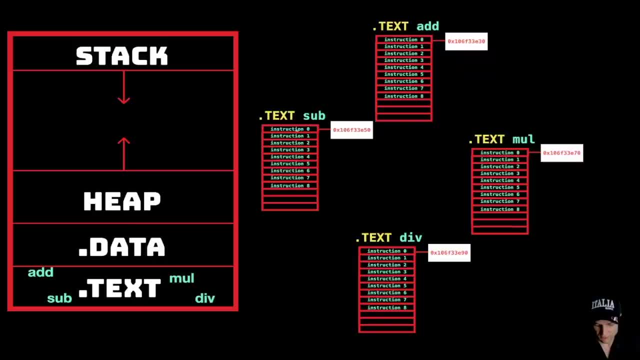 the text segment. you see, to make it clear, if we have more functions, for example, add, subtract, multiply, divide, we are going to have multiple pointers that are going to point to the instruction zero of the relative function. you see, that's what it is, my friend, that's what is going on. 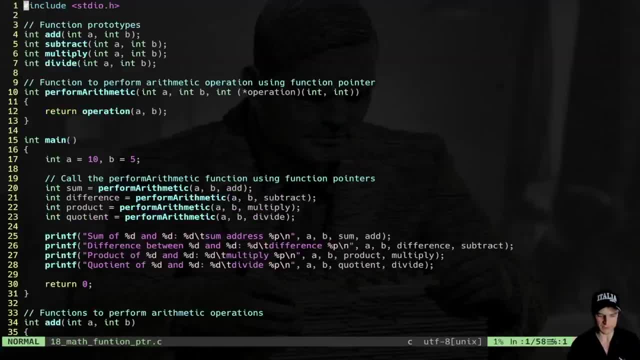 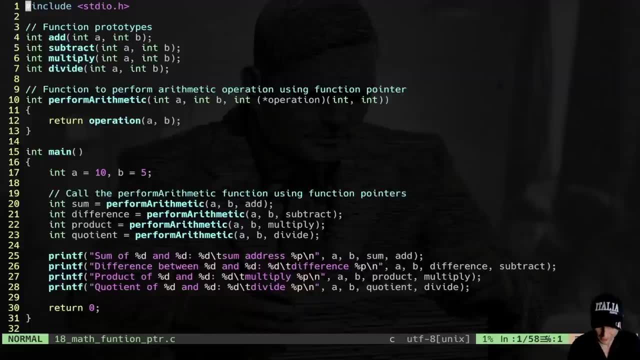 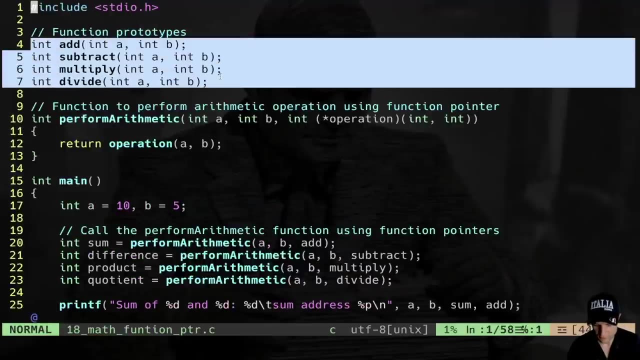 now, my friend, i have a little program to understand this concept of pointer to functions. okay, given the principle, given the knowledge that you now have, we're going to understand in this program. so here, immediately, you can see that i have, uh, four prototypes right for function: add, subtract, multiply and divide. you immediately notice that they all have the same. 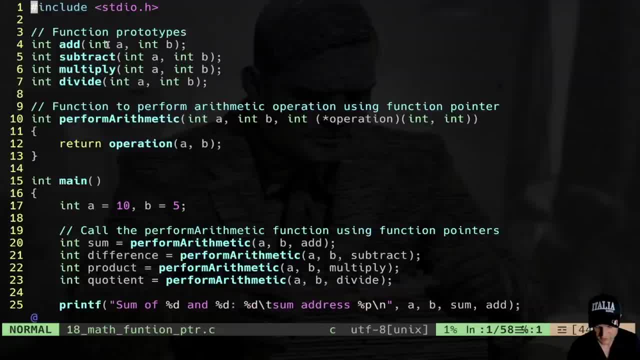 signature. they all have the same prototype because they give me back an integer and they take as an input an integer. okay, here i have another function that is called performed arithmetic special function because it's going to exploit function pointers. so the function is taking two integers and this strange thing here. you see this, my friend, is a pointer. 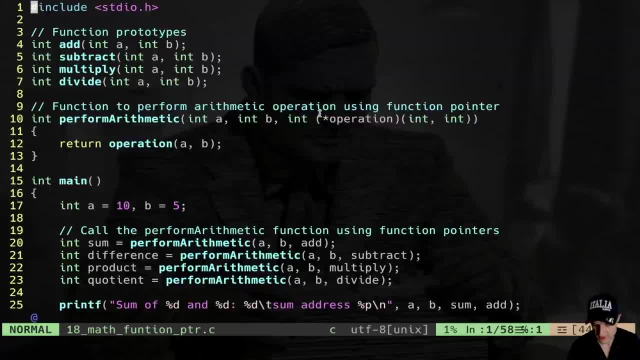 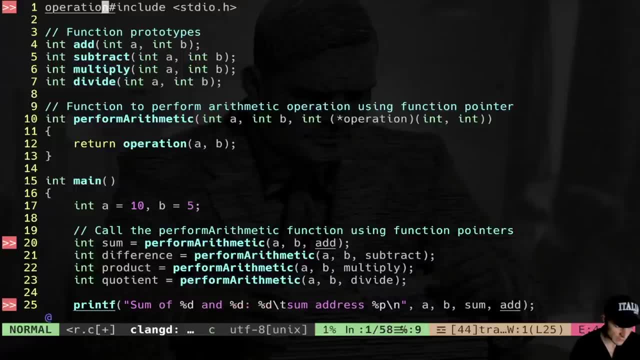 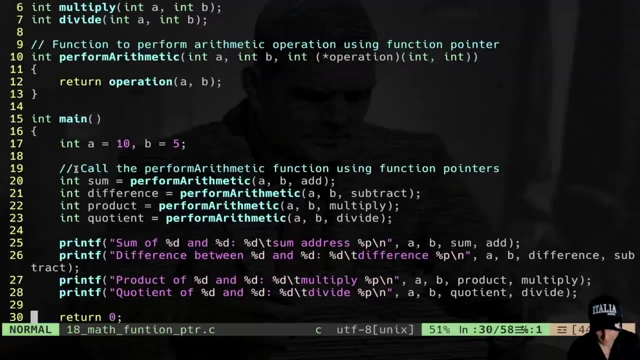 to a function, it has this way of writing. essentially it is almost like a prototype. the only difference is that we have these uh round braces here, and indeed, when it comes to uh pointer to functions, the syntax is not very simple. so now look there. in my main, i have, at the 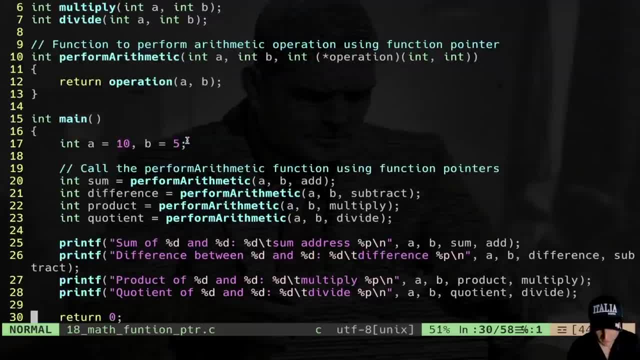 declaration of two variables, a and b, and here i want to perform arithmetic. in this case i want to perform the addition. so i call the function perform arithmetic and i give as an input: add. head is the name of a function, right is the name of this function. here i've 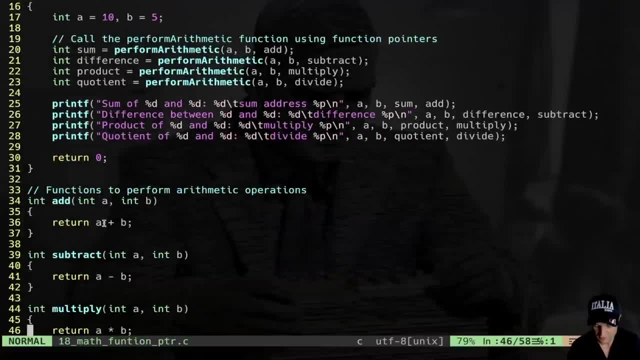 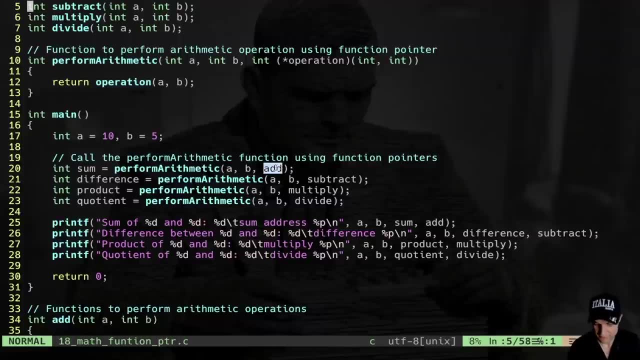 defined add here. this is a very silly function that is returning a plus b, but here i'm able to pass add. that now, you know, is just the address of the instructions in the text, it's just an address to the function. so here, every time i call, perform arithmetic. 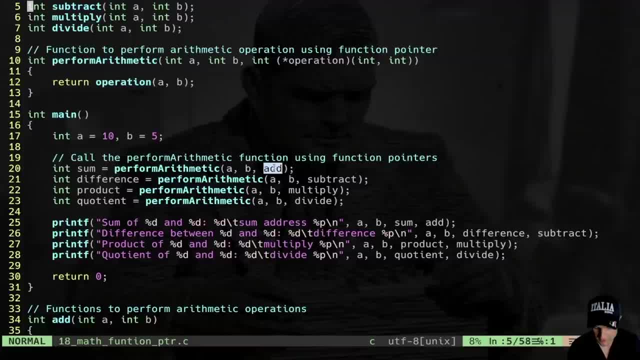 but with a different pointer right every time i change the pointer to the function perform, arithmetic only knows that it's gonna receive a function with a specific signature, and that's the important part. the thing is that a pointer has to be consistent. if you want to use in this fashion, all the pointers have to be an integer as a return. 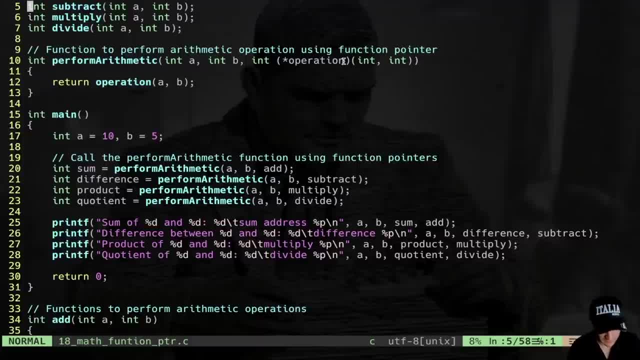 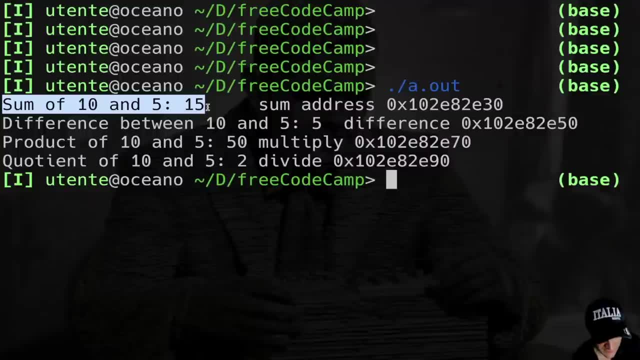 and two integers as an input. so let's try to launch this code and let's watch if it works. compile. so here i have the sum, which is 10 plus 5, is equal 15, of course, and the address of the sum function is this one. i have the difference, i get 5.. this is the 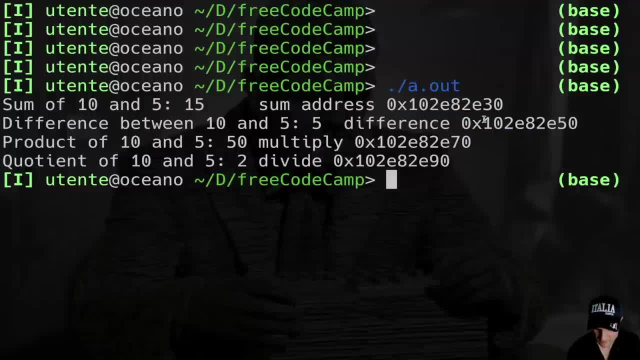 address of the difference. as you can see, it's fairly close. right, it's fairly close one each other. we have only a gap of 20, in hexadecimal of course, so it's going to be a gap of 32 bytes. here i have the multiplication and here i have the quotients, so the division okay. 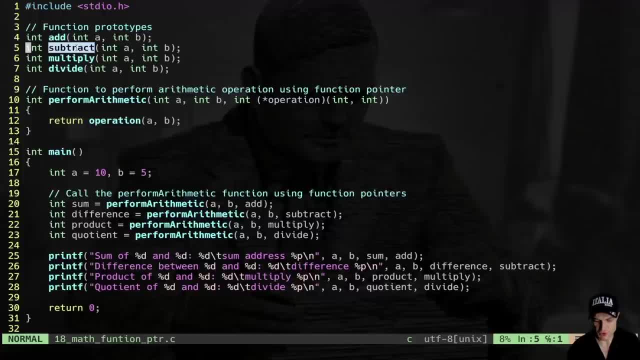 it works. so, at the end of the day, the name of a function is just an address, a spot in your memory in which you have the relative instructions to achieve the goal of the function itself. right here, with pointer to functions, we are exploiting this property. i repeat to you that it is important that the signature is the same. now let's try to change a. 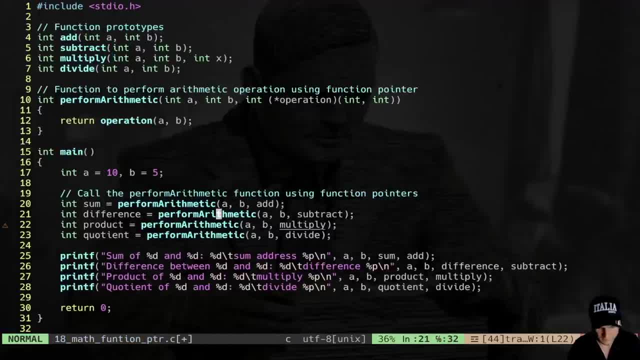 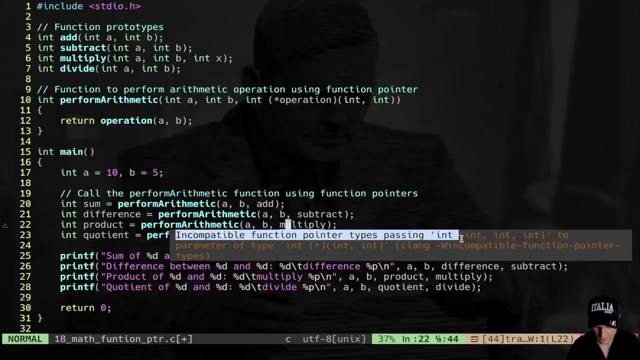 little bit. i'm gonna do another integer and this time immediately i get a warning and installing me incompatible um function pointer because you can see that this is another type. right, i have another type of pointer. so it's giving me a warning because i have a pointer to function that has another. 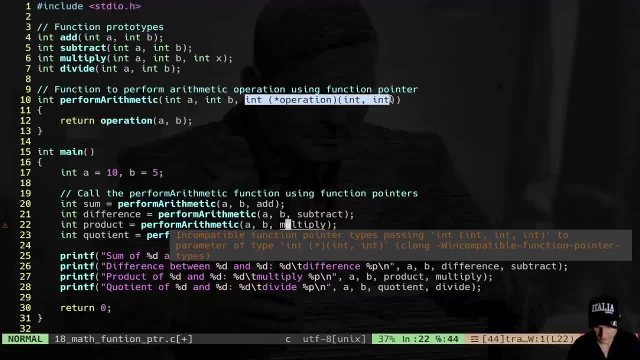 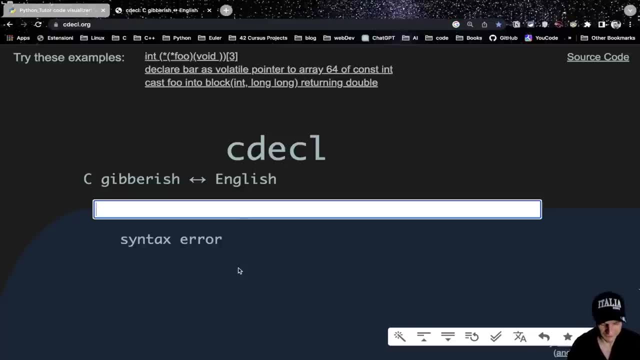 signature respective to the one that the function is able to take. the last thing we have to demystify is a little bit the syntax, which is kind of super tricky of pointers to function. so we go in the this website, which is gibberish to see, and we're gonna type, for example: int. 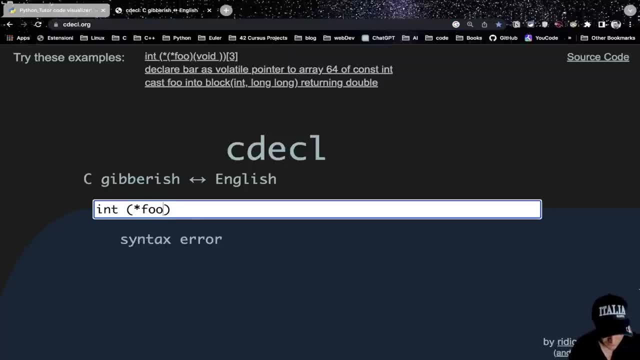 and then we are gonna do- i don't know- pointer to foo, and then we're gonna do int, int. as you can see, i have declare foo as a pointer to function that takes two integers and return an integer. now why it is important to use the round braces here. well, let's try to remove them. this is a. 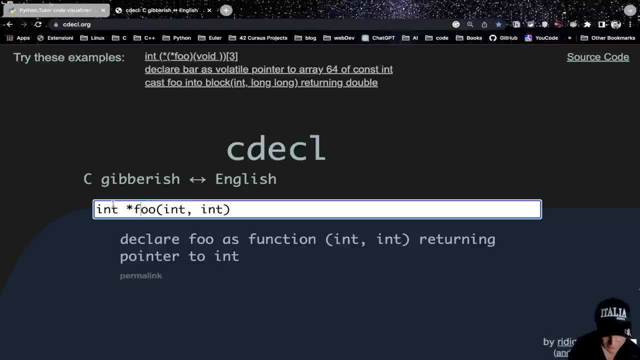 prototype. as you can see, we're declaring foo as a function, that is, returning a pointer to an integer. so that's the problem. on the contrary, if i say an hey, you have to read this together. I'm saying: oh, I see, So this foo is a pointer to a function. 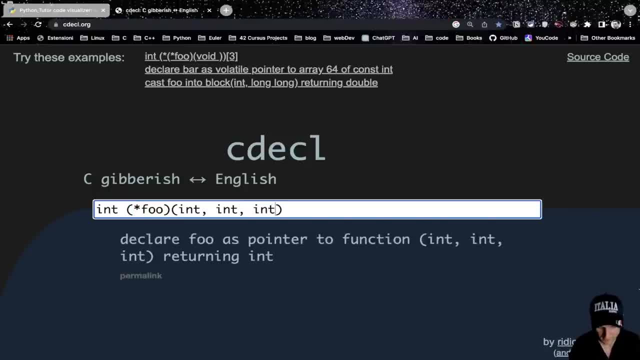 Get it Now, of course. here I have all the values that I can have, And that's all there is. This is the way by which you can declare a pointer to a function. I want to stress out that I don't use pointers to function. 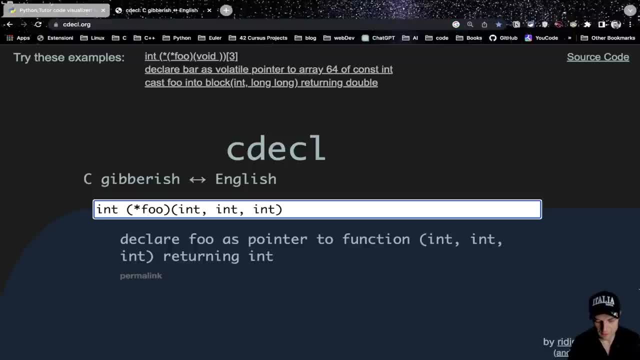 very often, but it's useful to know how they work. So I just gave you the overall principle, the overall idea. A function name is just a fancy way of talking about an address. in memory, I recall to you that all the names, all the variable names, 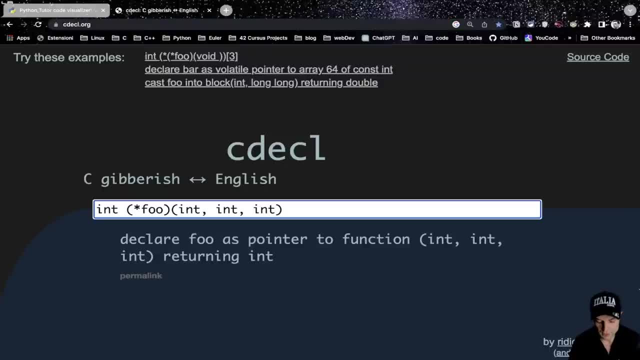 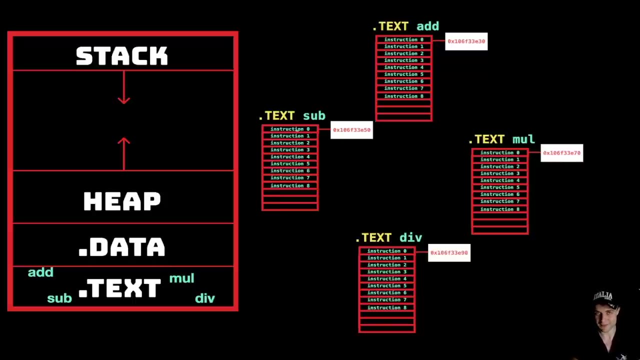 function names are just an abstraction for us to read the code. But at the end of the day, we have only numbers, We have only addresses, We have only binary values. All the symbols are just an abstraction for us. OK, my friend, I think that with this mini course, 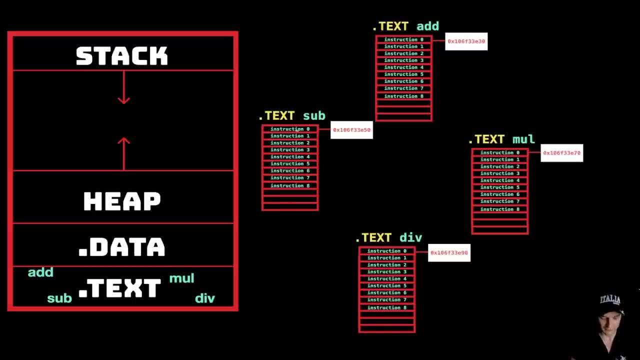 you have a better understanding of pointer pointers. hopefully, I really hope. Basically, this is the video I wanted to watch when I started to learn about the C programming language. Of course, there is a lot more to dig, to understand, to practice, because pointers are a tremendous bad beast. 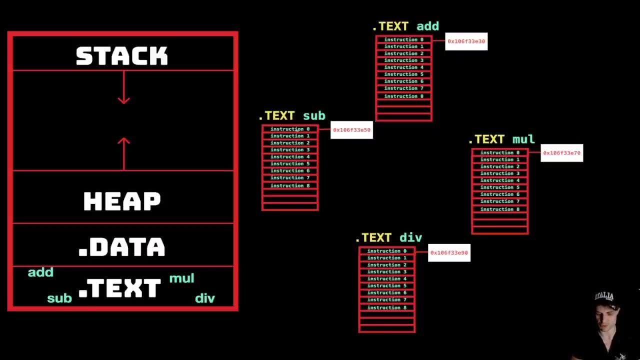 to tame, But this, I think, is a very good introduction. All right, my friend, thank you for watching. Take care. 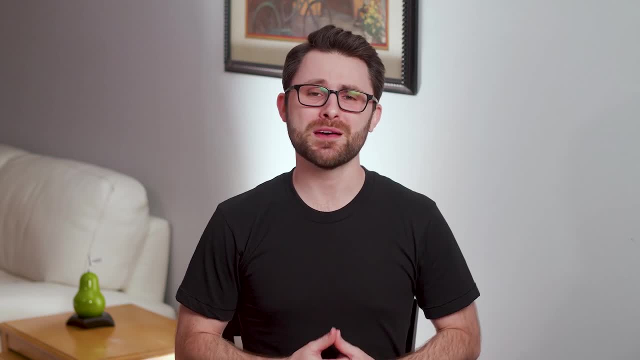 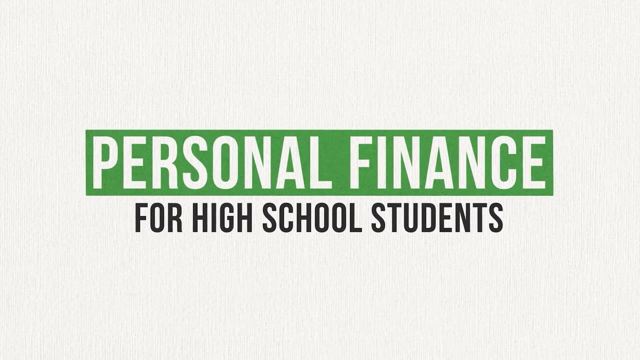 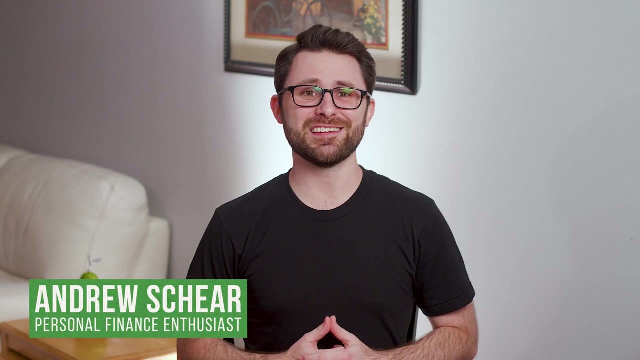 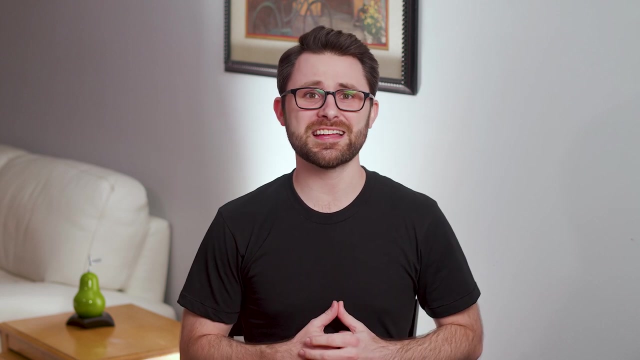 This is what you need to know about money and personal finance before graduating from high school. Hello and welcome to Practical Personal Finance, where you get the information you need to understand and succeed with money. Today, I'm going over five personal finance topics that you should be familiar with before walking across that stage and receiving your high school. 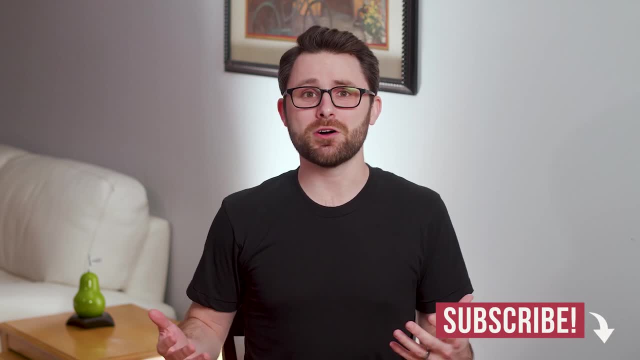 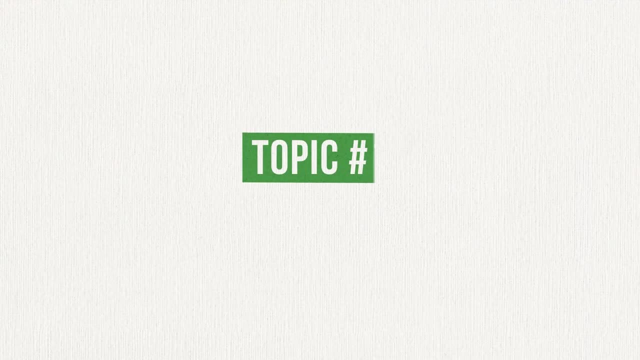 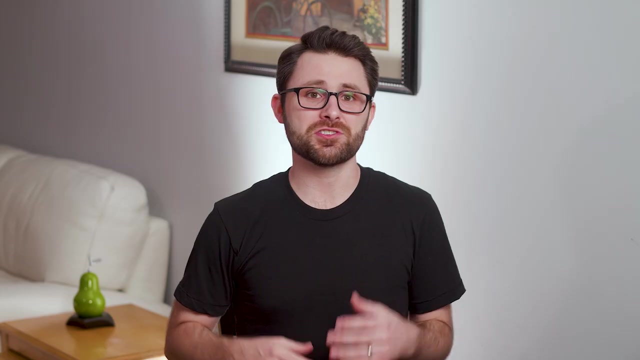 diploma. Money can be a pretty complex topic, so, as always, I'm going to do my best to break it down for you and explain each of these five topics in simple terms. Let's get started with topic number one: budgeting. If you listen to podcasts or watch a lot of YouTube videos, there's a good